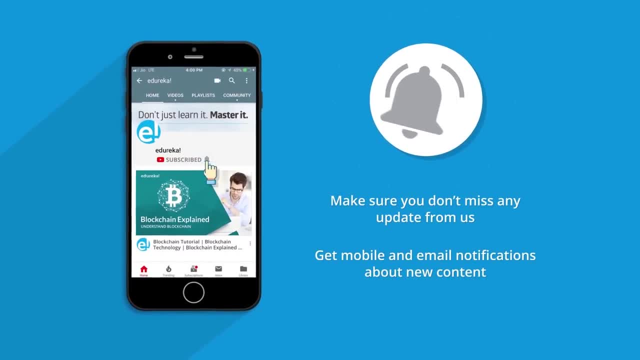 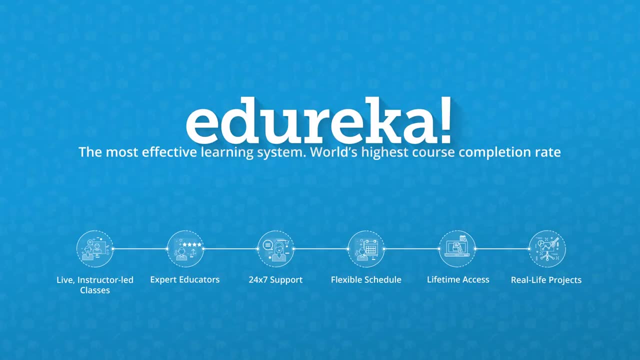 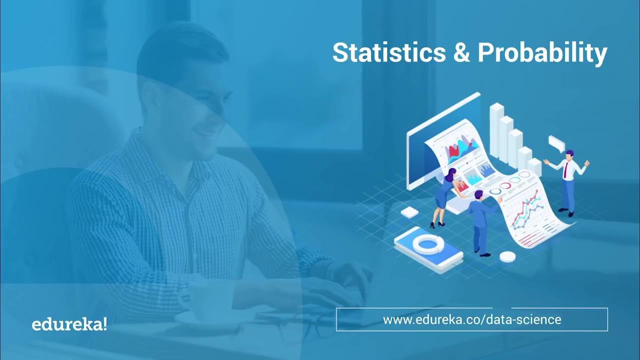 Statistics and probability are essential because these disciples form the basic foundation of all machine learning algorithms, deep learning, artificial intelligence and data science. In fact, mathematics and probability is behind everything around us, From shapes, patterns and colors to the count of petals in a flower. mathematics is embedded in each and every aspect. 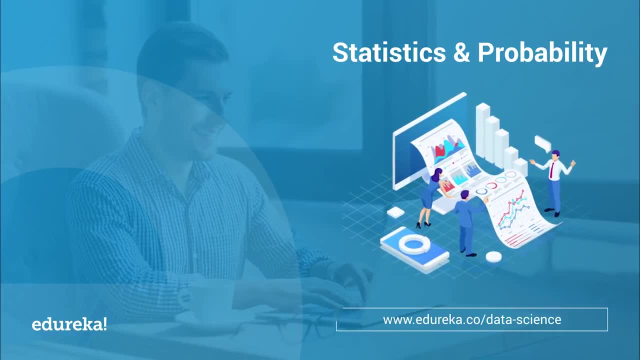 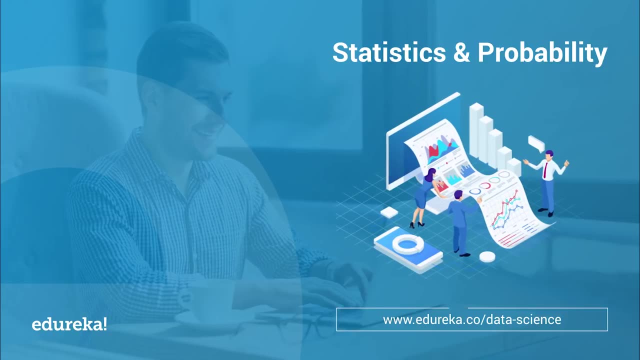 of our lives. With this in mind, I welcome you all to today's session. Hi everyone, I'm Zuleika from Edureka, and this session is all about statistics and probability, So I'm going to go ahead and discuss the agenda for today with you all. We're going to begin this session by 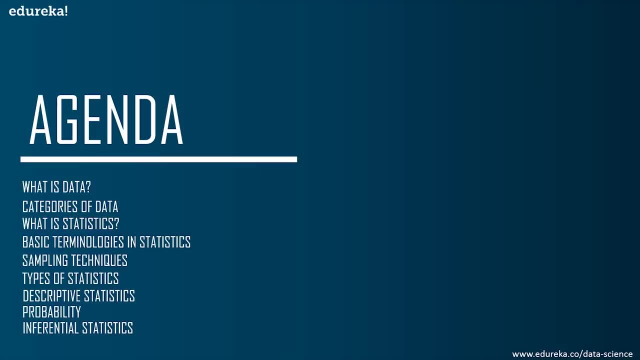 understanding what is data. After that, we'll move on and look at the different categories of data, like quantitative and qualitative data. Then we'll discuss what exactly statistics is, the basic terminologies in statistics and a couple of sampling techniques Once we're done, 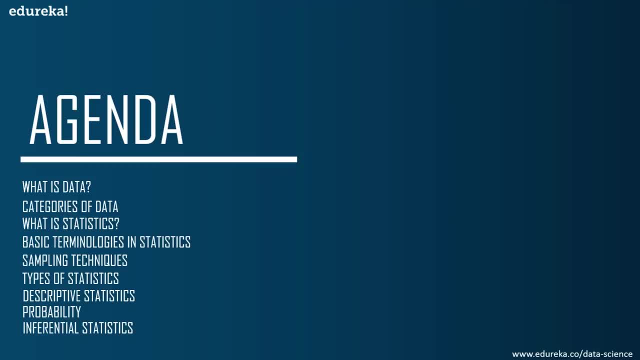 with that we'll discuss the different types of statistics, which involve descriptive and inferential statistics. Then in the next session we'll mainly be focusing on descriptive statistics. Here we'll understand the different measures of center, measures of spread information gain. 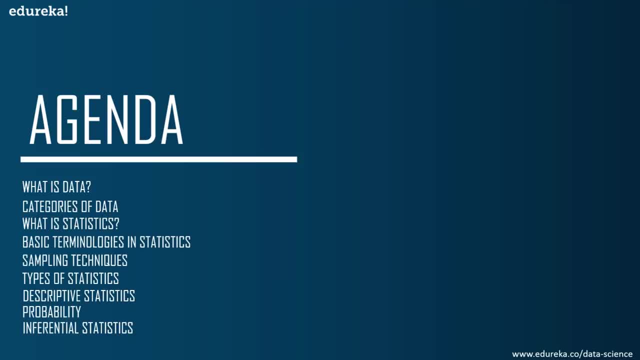 and entropy. We'll also understand all of these measures with the help of a use case. And finally, we'll discuss what exactly a confusion matrix is. Once we've covered the entire descriptive statistics module, we'll discuss the probability module. Here we'll understand what exactly. 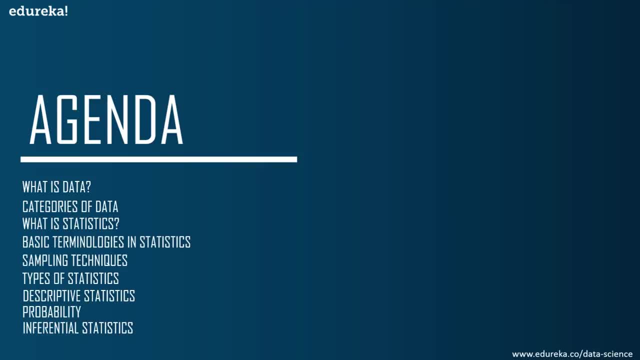 probability is the different terminologies in probability, We'll also study the different probability distributions and the different types of probabilities. So let's get started. First, we'll discuss the different types of statistics. First we'll discuss the different types of. 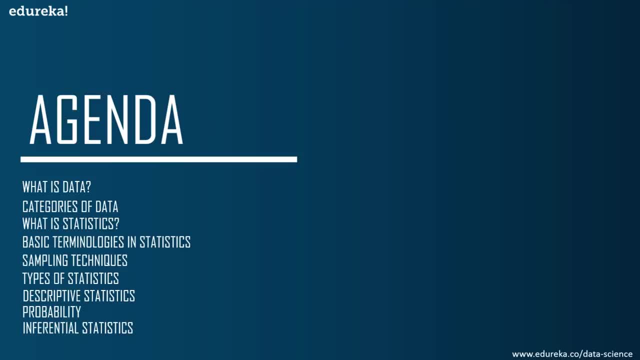 distributions. Then we'll discuss the types of probability, which include marginal probability, joint and conditional probability. Then we'll move on and discuss a use case wherein we'll see examples that show us how the different types of probability work. and to better understand Bayes theorem, we look at a 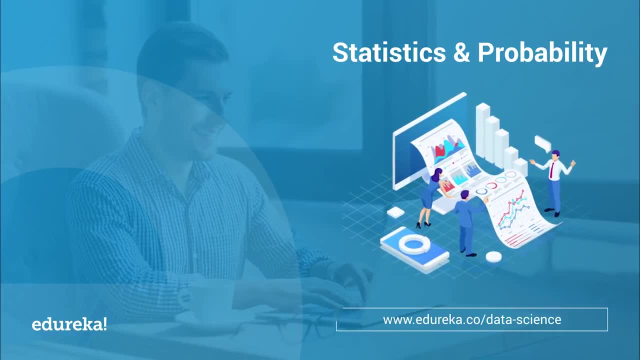 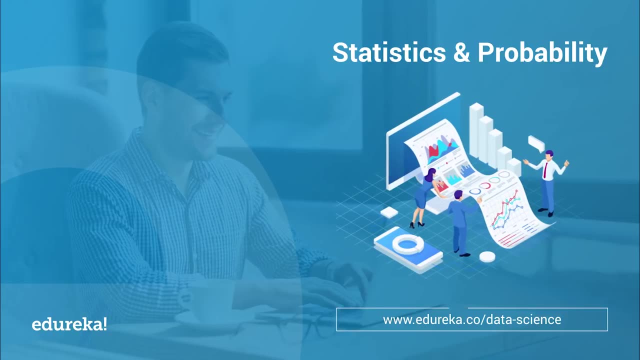 of our lives. With this in mind, I welcome you all to today's session. Hi everyone, I'm Zuleika from Edureka, and this session is all about statistics and probability, So I'm going to go ahead and discuss the agenda for today with you all. We're going to begin this session by 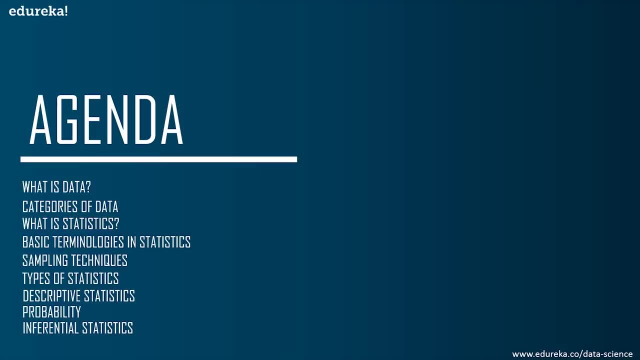 understanding what is data. After that, we'll move on and look at the different categories of data, like quantitative and qualitative data. Then we'll discuss what exactly statistics is, the basic terminologies in statistics and a couple of sampling techniques Once we're done, 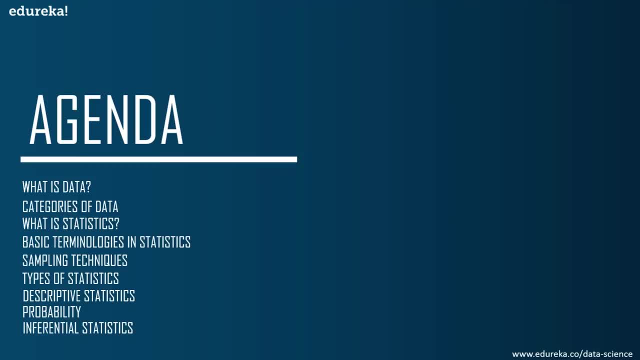 with that we'll discuss the different types of statistics, which involve descriptive and inferential statistics. Then in the next session we'll mainly be focusing on descriptive statistics. Here we'll understand the different measures of center, measures of spread information gain. 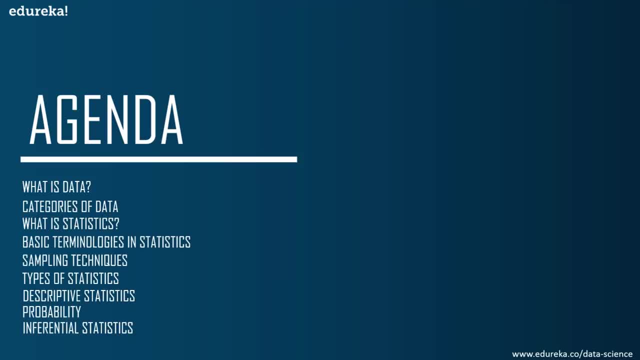 and entropy. We'll also understand all of these measures with the help of a use case. And finally, we'll discuss what exactly a confusion matrix is. Once we've covered the entire descriptive statistics module, we'll discuss the probability module. Here we'll understand what exactly. 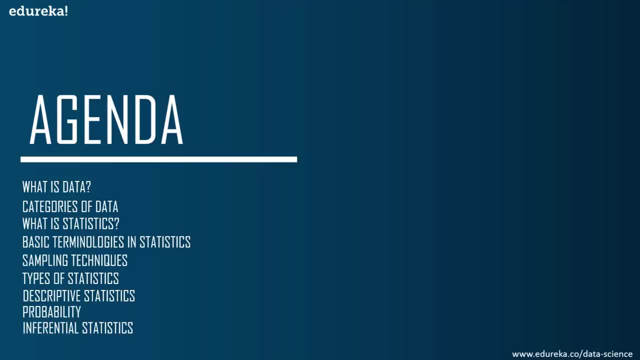 probability is the different terminologies in probability. We'll also study the different probability distributions And finally we'll discuss the different types of data. So let's start with the distributions. Then we'll discuss the types of probability, which include marginal. 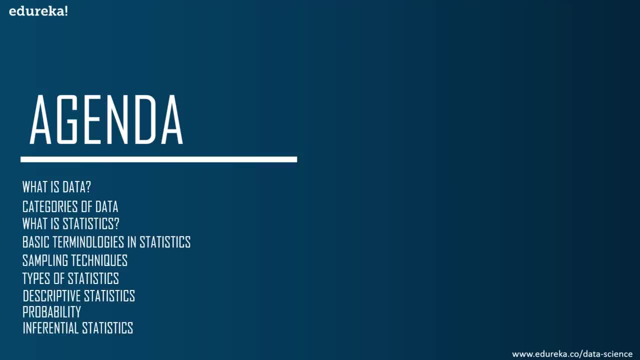 probability- joint and conditional probability. Then we'll move on and discuss a use case wherein we'll see examples that show us how the different types of probability work. And to better understand Bayes' theorem, we'll look at a small example. Also, I forgot to mention that at the end of the 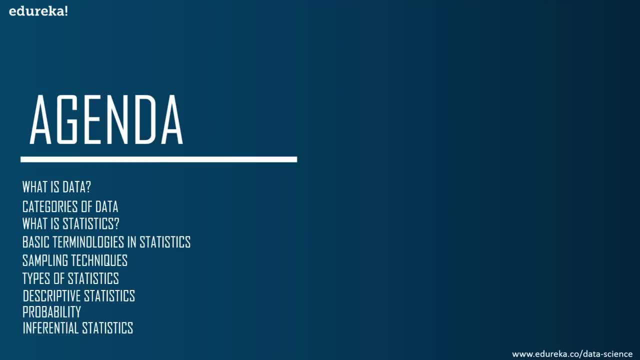 descriptive statistics module. we'll be running a small demo in the R language. So for those of you who don't know what descriptive statistics is, it's a small demo of the R language. So for those of you who don't know much about R, I'll be explaining every line in depth. But if you want to have 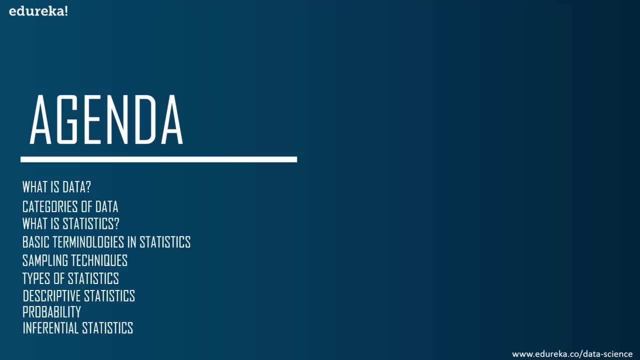 a more in-depth understanding about R. I'll leave a couple of blogs and a couple of videos in the description box. Y'all can definitely check out that content. Now, after we've completed the probability module, we'll discuss the inferential statistics module. We'll start this module by: 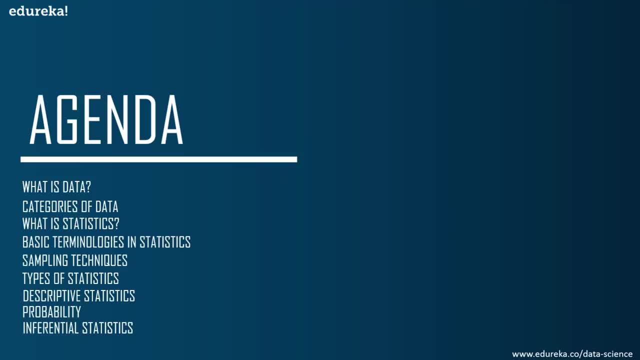 small example. Also, I forgot to mention that at the end of the descriptive statistics module will be running a small demo in the R language. So for those of you who don't know much about R, I'll be explaining every line in depth. but if you want to, 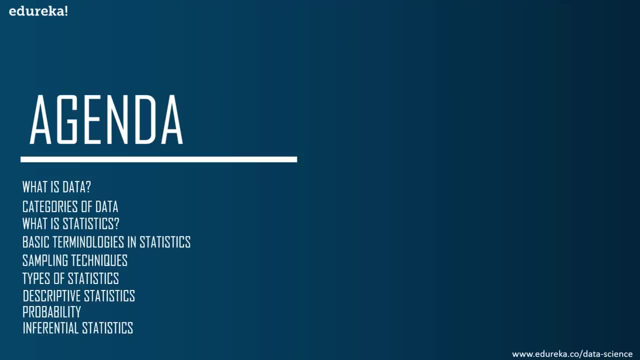 have a more in depth understanding about R, I'll leave a couple of blogs and a couple of videos in the description box. Y'all can definitely check out that content. Now, after we've completed the probability module, we'll discuss the inferential statistics module. 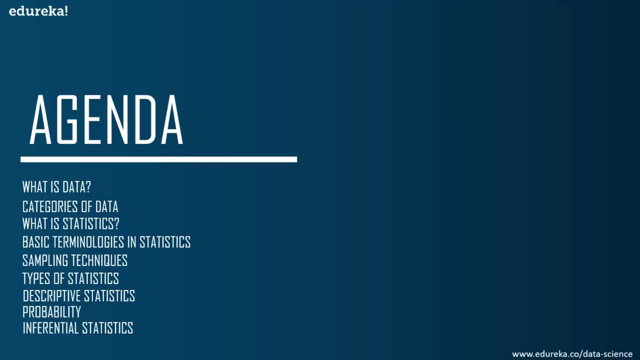 We'll start this module by understanding what is point estimation. We'll discuss what is confidence interval and how we can use it to determine the confidence interval. Now you can estimate the confidence interval. We'll also discuss margin of error and we'll understand all of these concepts by looking at a small use case. 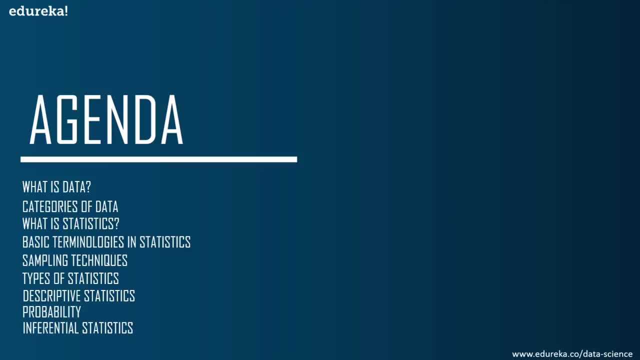 We'll finally end the inferential statistic module by looking at what hypothesis testing is. Hypothesis testing is a very important part of inferential statistics, so we'll end the session by looking at a use case that discusses how hypothesis testing works. and, to sum everything up, we'll look at 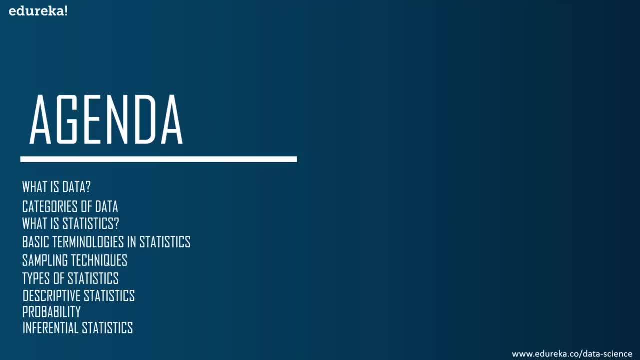 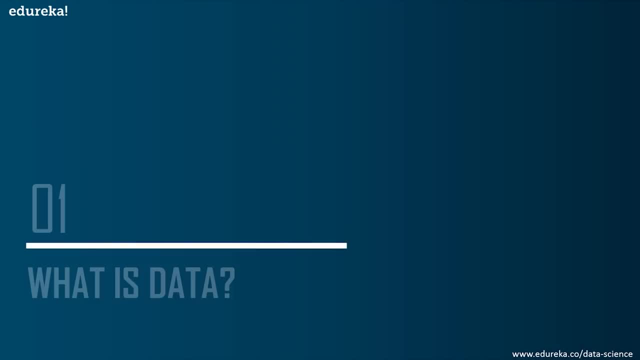 a demo that explains how inferential statistics work. So, guys, there's a lot to cover today, so let's move ahead and take a look at our first topic, which is: what is data? Now, this is a quite simple question. If I ask any of you what is data? 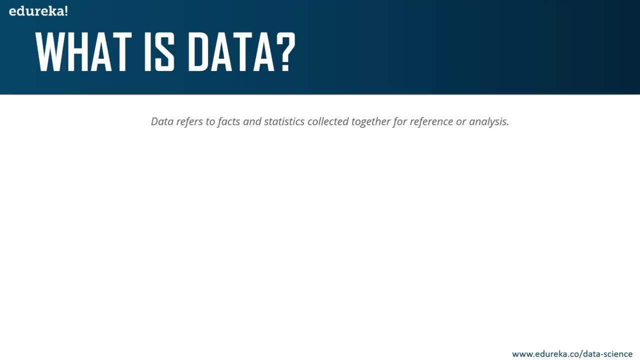 you'll see that it's a set of numbers or some sort of documents that I've stored in my computer. Now, data is actually everything. Alright, look around you. There is data everywhere. Each click on your phone generates more data than you know Now this: 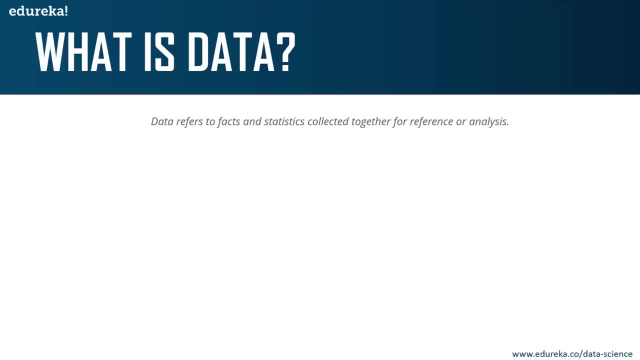 generated data provides insights for you to understand what is data. Data is used for analysis and helps us make better business decisions. This is why data is so important. To give you a formal definition: data refers to facts and statistics collected together for reference or analysis. Alright, this is. 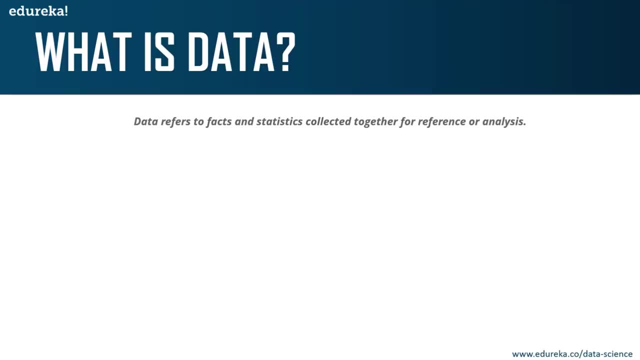 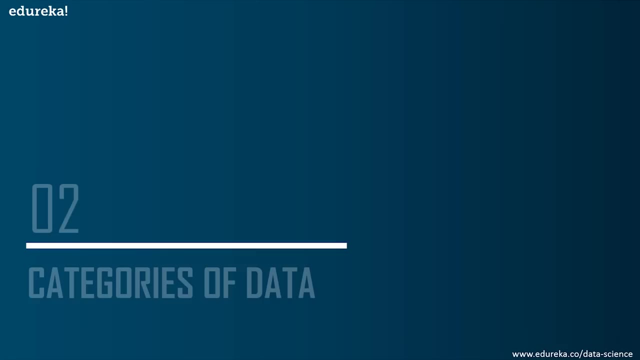 the definition of data in terms of statistics and probability. So, as we know, data can be collected, It can be measured and analyzed. It can be visualized by using statistical models and graphs. Now, data is not just a set of numbers, and data is divided into two major subcategories. Alright, so first, 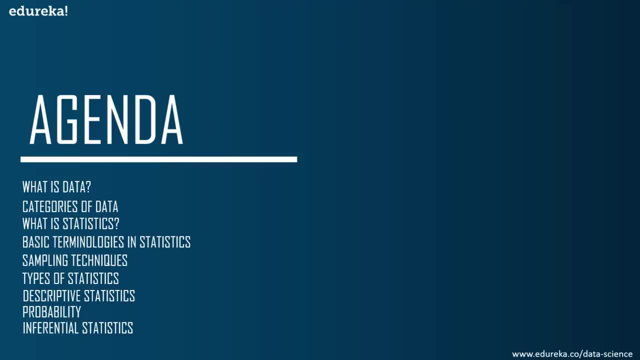 understanding what is point estimation. We'll discuss what is confidence interval and how you can estimate the confidence interval. We'll also discuss margin of error And we'll understand all of these concepts by looking at a small use case. We'll finally end the inferential statistic module by looking at what hypothesis 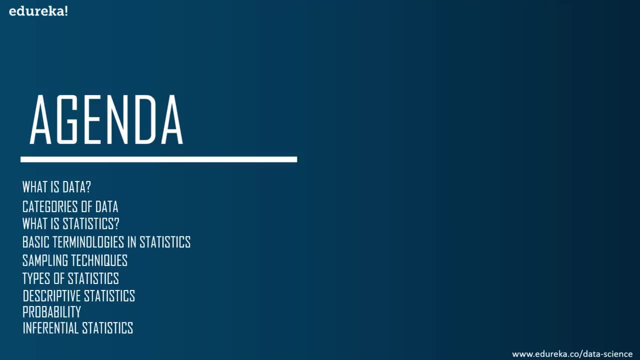 testing is. Hypothesis testing is a very important part of inferential statistics, So we'll end the session by looking at a use case that discusses how hypothesis testing works And, to sum everything up, we'll look at a demo that explains how inferential statistics works. Alright, so, guys, there's a. 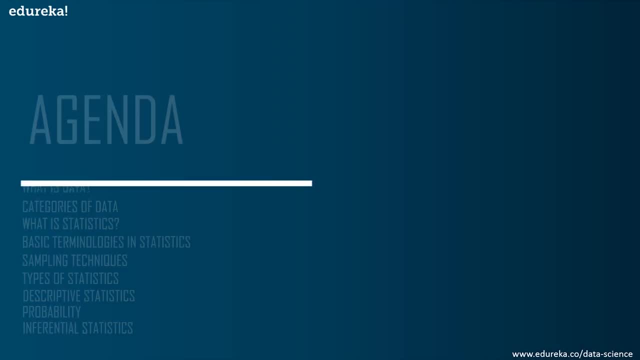 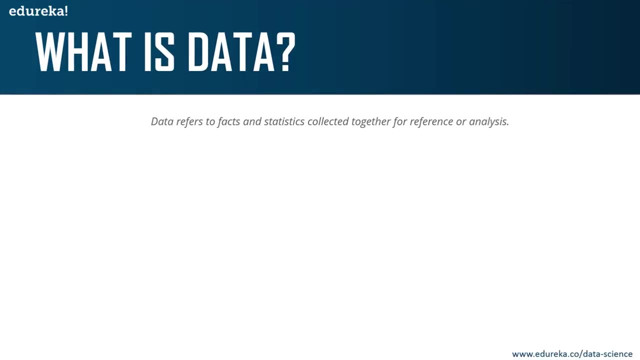 lot to cover today, So let's move ahead and take a look at our first topic, which is: what is data? Now, this is a quite simple question. If I ask any of you what is data, you'll see that it's a set of. 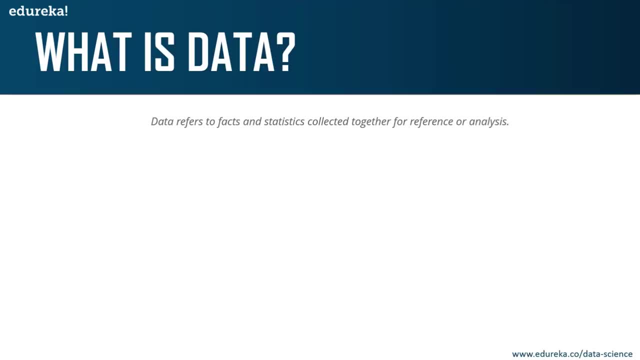 numbers or some sort of documents that I've stored in my computer. Now, data is actually everything. Alright, look around you. There is data everywhere. Each click on your phone generates more data than you know Now. this generated data provides insights for analysis and helps us make better. 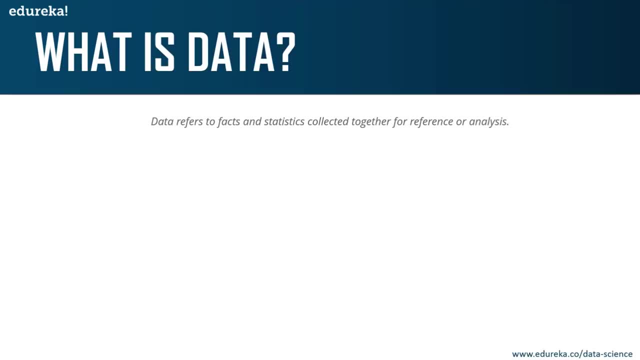 business decisions. This is why data is so important. To give you a formal definition, data refers to facts and statistics collected together for reference or analysis. Alright, this is the definition of data in terms of statistics and probability. So, as we know, 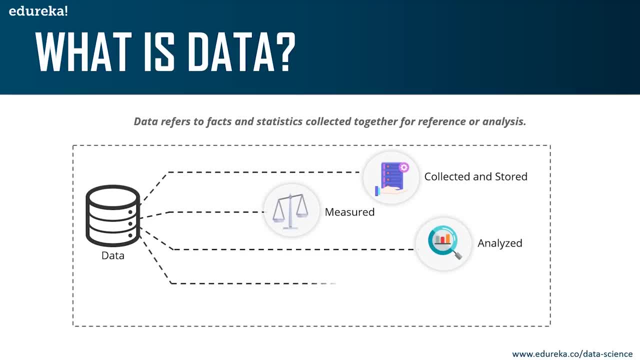 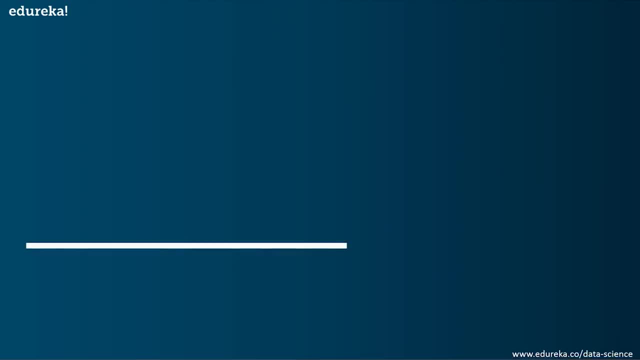 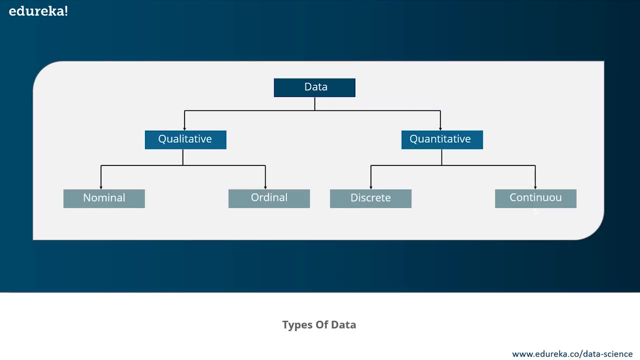 data can be collected, it can be measured and analyzed. it can be visualized by using statistical models and graphs. Now data is divided into two major subgroups. So data is divided into two major subgroups. Alright, so first we have qualitative data and quantitative data. These are the two different. 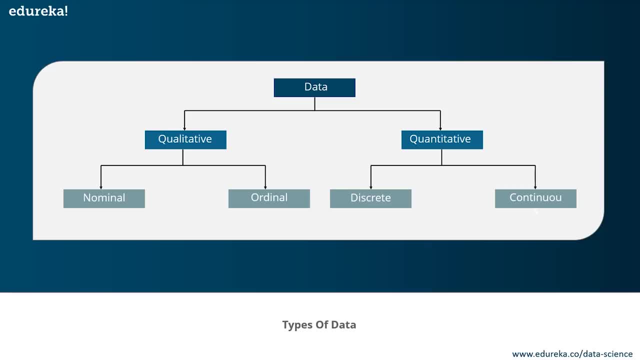 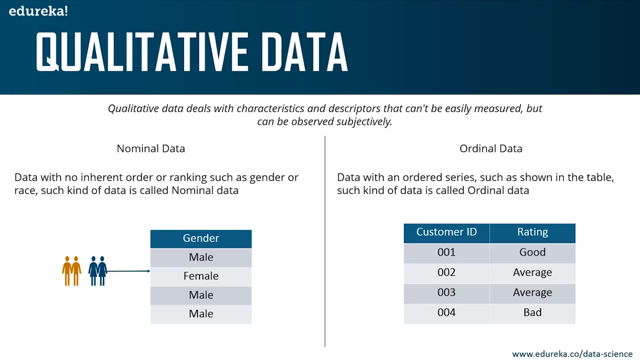 types of data. Under qualitative data, we have nominal and ordinal data, and under quantitative data, we have discrete and continuous data. Now let's focus on qualitative data Now. this type of data deals with characteristics and descriptors that can't be easily measured, but can be observed. 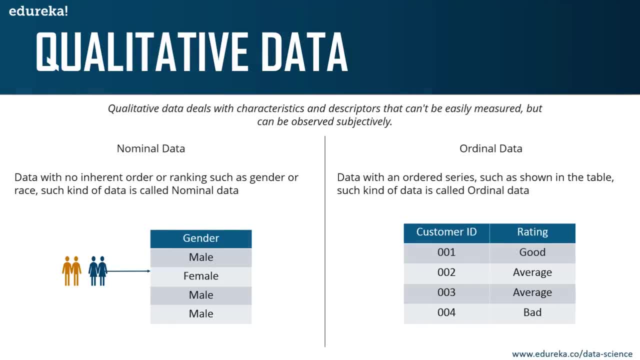 subjectively. Now qualitative data is further divided into two categories. So qualitative data is divided into nominal and ordinal data. So nominal data is any sort of data that doesn't have any order or ranking. Okay, an example of nominal data is gender. Now, there is no ranking in gender. 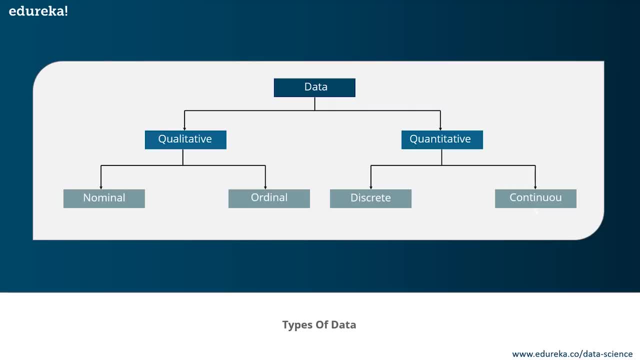 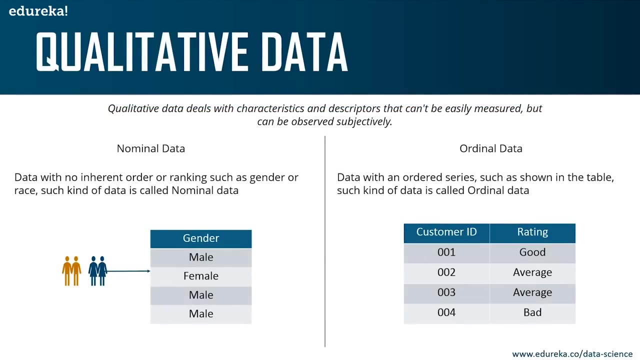 we have qualitative data and quantitative data. These are the two different types of data. Under qualitative data, we have nominal and ordinal data, and under quantitative data, we have discrete and continuous data. Now let's focus on qualitative data Now. this type of data deals with characteristics and 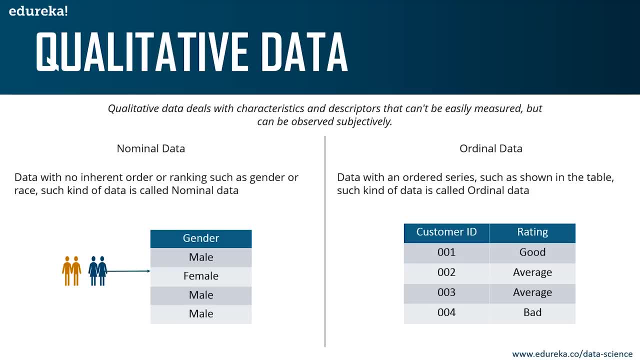 descriptors that can't be easily measured but can be observed subjectively. Now qualitative data is further divided into nominal and ordinal data. So nominal data is any sort of data that doesn't have any order or ranking. Okay, an example of nominal data is: 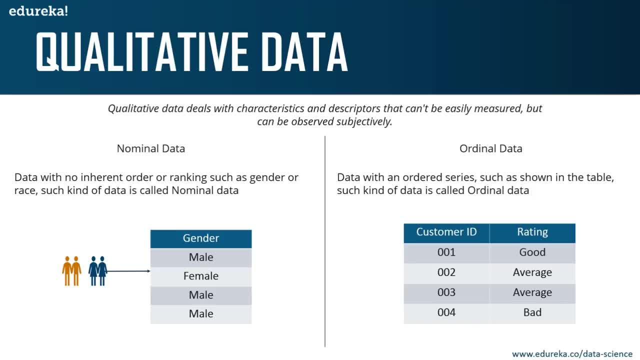 gender. Now, there is no ranking in gender. There's only male, female or other right. There is no one, two, three, four or any sort of ordering in gender. Race is another example of nominal data. Now, ordinal data is basically an ordered series of 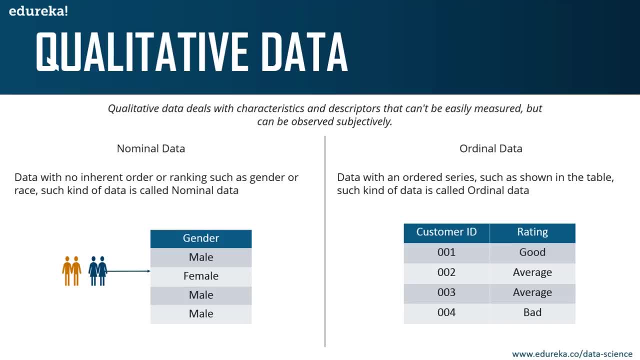 information. Okay, let's say that you went to a restaurant. Okay, your information is stored in the form of customer ID, Alright, so basically, you are represented with a customer ID. Now you would have rated their service as either good or average. Alright, that's how ordinal data is, And similarly, 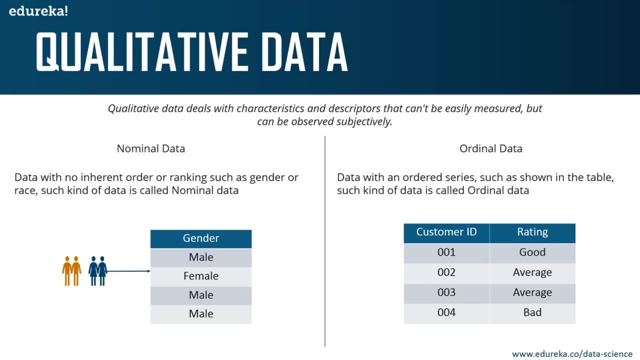 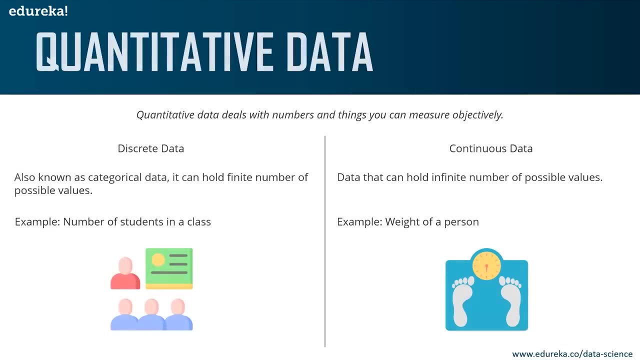 they'll have a record of other customers who visit the restaurant, along with their ratings. Alright, so any data which has some sort of sequence or some sort of order To it is known as ordinal data. Alright, so, guys, this is pretty simple to understand. Now let's move on and look at quantitative. 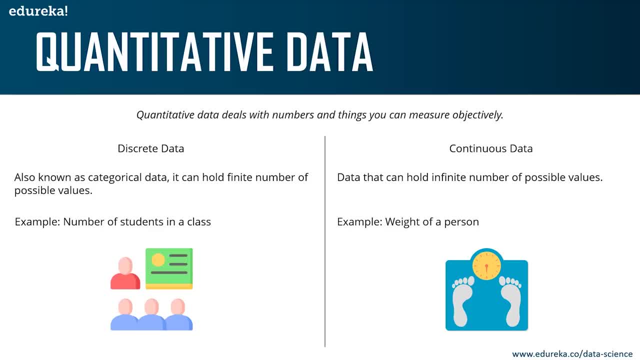 data. So quantitative data basically deals with numbers and things. Okay, you can understand that by the word quantitative itself. Quantitative is basically quantity, right? So it deals with numbers, it deals with anything that you can measure objectively. Alright, so there are two types of 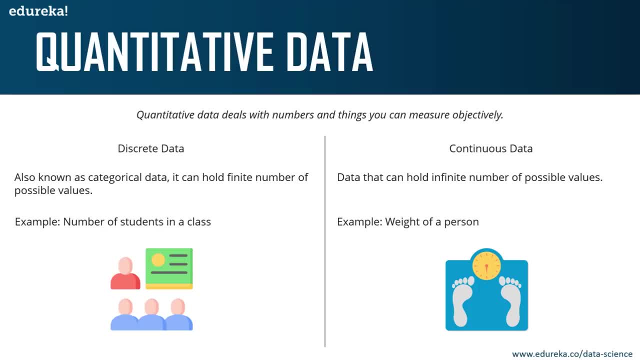 quantitative data, there is discrete and continuous data. Now discrete data is also known as categorical data, and it can hold a finite number of possible values. Now, the number of students in a class is a finite number. Alright, you can't have infinite number of students in a class. Let's say in your. 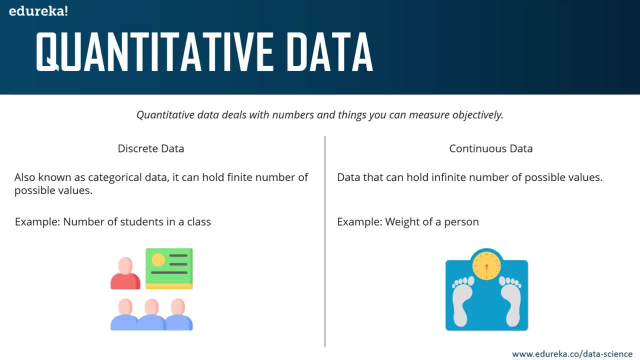 fifth grade, there were 100 students in your class. Alright, they weren't infinite number, but there was a definite, finite number of students in your class. Okay, that's discrete data. Next, we have continuous data. Now, this type of data can hold. 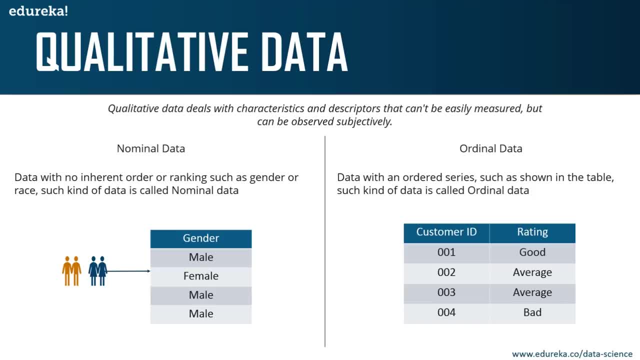 There's only male, female or other right. There is no 1,, 2,, 3,, 4 or any sort of ordering in gender. Race is another example of nominal data. Now, ordinal data is basically an ordered series of. 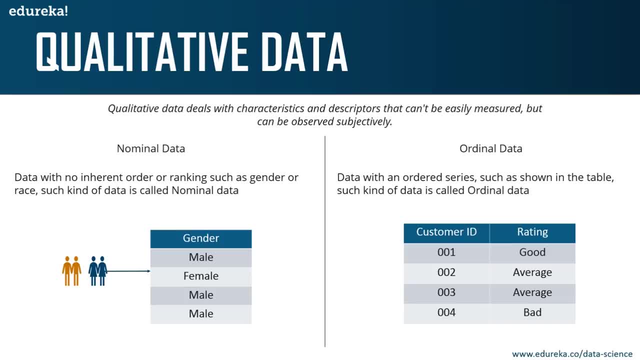 information. Okay, let's say that we have a number of data. We have a number of data, We have a number of data. Let's say that you went to a restaurant. Okay, your information is stored in the form of customer ID, All right. So basically, you are represented with a customer ID. Now you 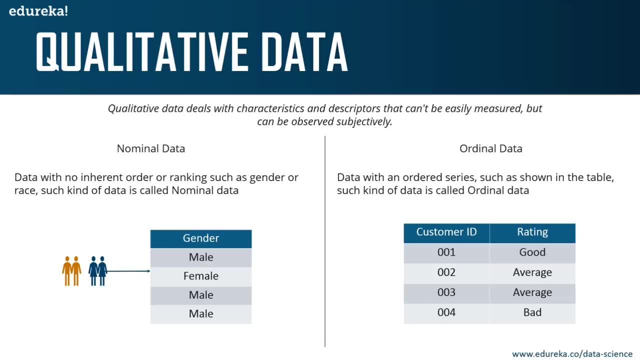 would have rated their service as either good or average. All right, That's how ordinal data is, And similarly, they'll have a record of other customers who visit the restaurant, along with their ratings. All right, So any data which has some sort of sequence or some sort of order to it. 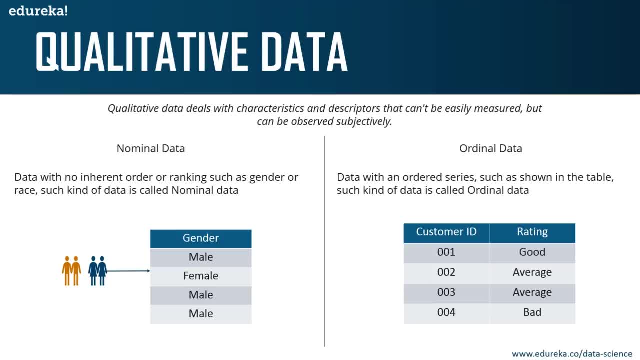 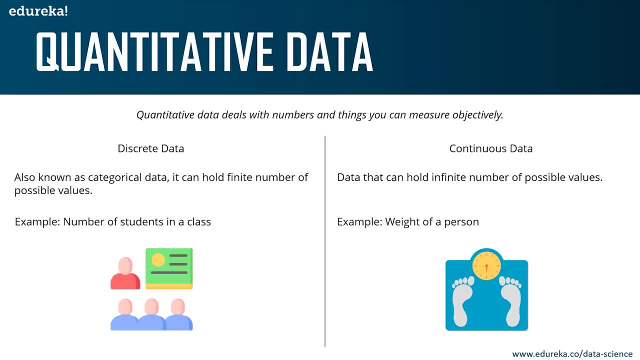 is known as ordinal data. All right, So, guys, this is pretty simple to understand. Now let's move on and look at quantitative data. So quantitative data basically deals with numbers and things. Okay, you can understand that by the word quantitative itself. Quantitative is basically quantity, right? So 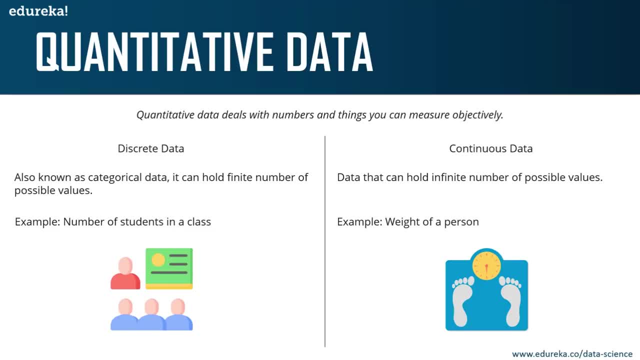 it deals with numbers. It deals with anything that you can measure objectively. All right, So there are two types of quantitative data. There is discrete and continuous data. Now, discrete data is also known as categorical data, and it can hold a finite number of possible values. Now the number. 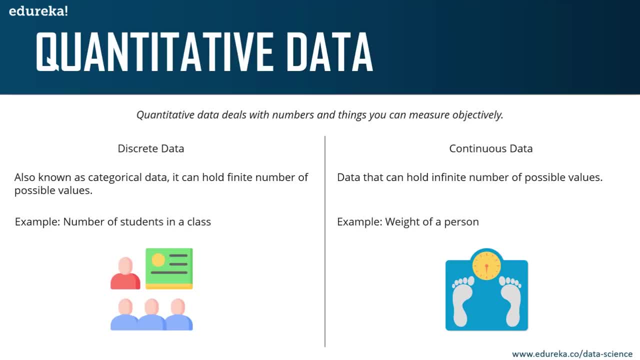 of students in a class is a finite number. All right, You can't have infinite number of students in a class. Let's say in your fifth grade, there were 100 students in your class. All right, There weren't infinite number, but there was a definite finite number of students in your class. Okay, 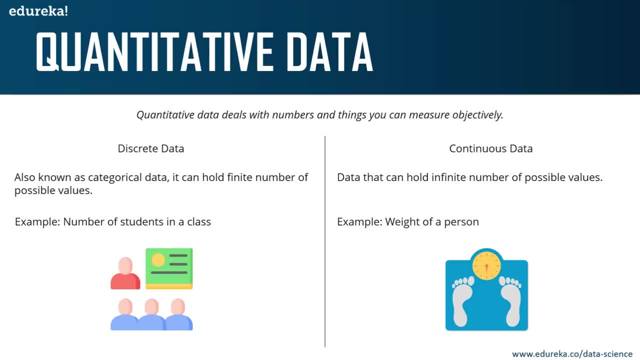 that's discrete data. Next, we have continuous data Now. this type of data can hold infinite number of possible values. Okay, So when you say weight of a person is an example of continuous data, what I mean to say is my. 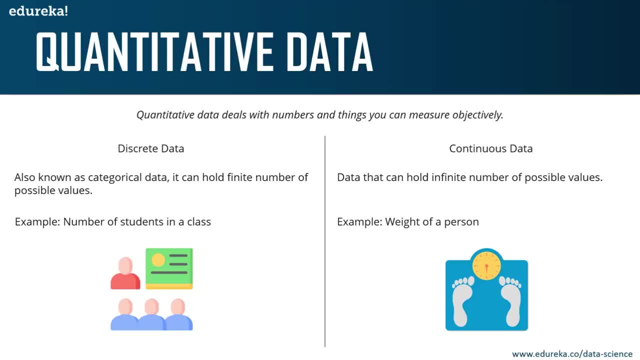 weight can be 50 kgs, or it can be 50.1 kgs, or it can be 50.001 kgs or 50.0001, or it's 50.023, and so on. Right, There are infinite number of possible values, Right? So this is what I mean by. 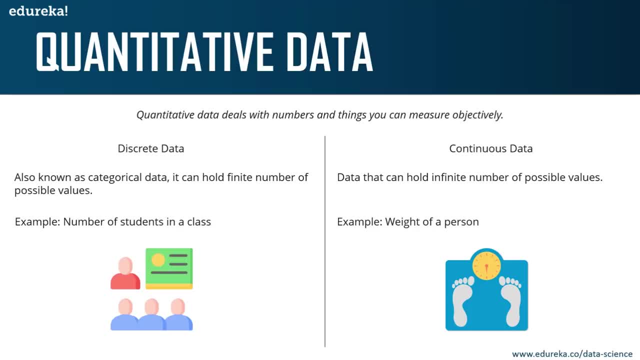 infinite of possible values. okay, so when you say weight of a person is an example of continuous data, what I mean to say is my weight can be 50 kgs, or it can be 50.1 kgs, or it can be 50.001 kgs or 50.0001 or 50.023 and so on. right, there are. 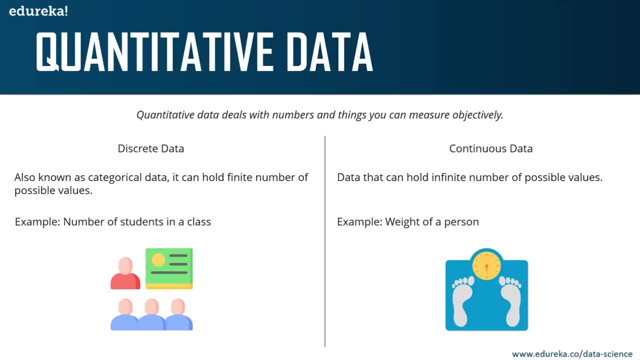 infinite number of possible values. right, so this is what I mean by continuous data. all right, this is the difference between discrete and continuous data, and also I'd like to mention a few other things over here. now, there are a couple of types of variables as well. all right, we. 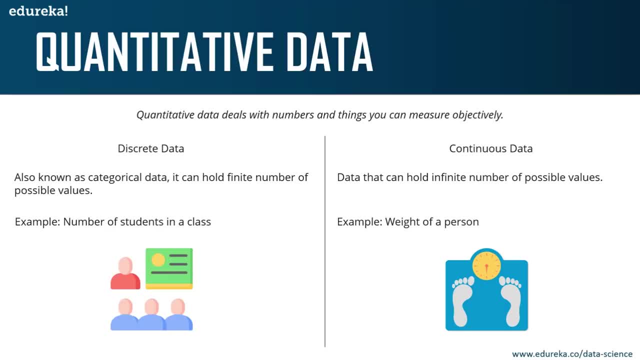 have a discrete variable and we have a continuous variable. discrete variable is also known as a categorical variable. all right, it can hold values of different categories. let's say that you have a variable called message and there are two types of variables that are called message and there are two types of. 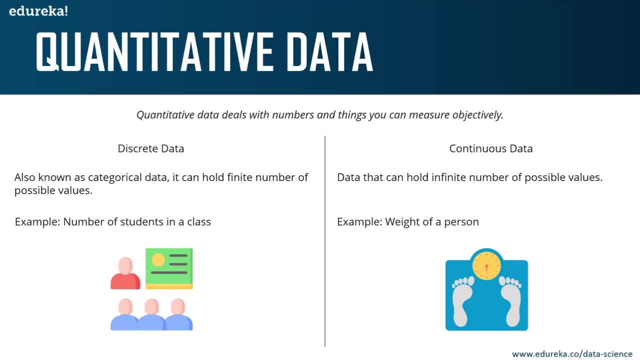 values that this variable can hold. let's say that your message can either be a spam message or a non spam message. okay, that's when you call a variable as discrete or categorical variable, all right, because it can hold values that represent different categories of data. now, continuous variables are basically: 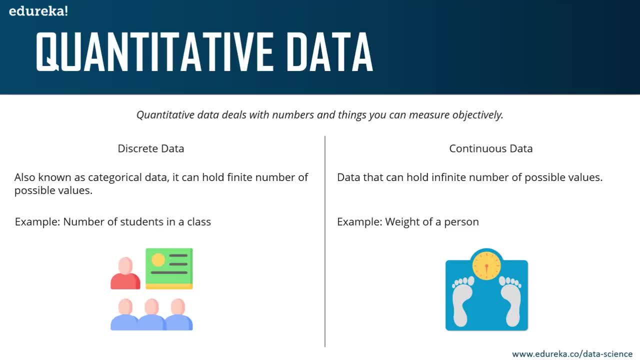 variables that can store infinite number of values. so the weight of a person can be denoted as a continuous variable. all right, let's say there is a variable and it can store infinite number of possible values. that's why we'll call it a continuous variable. so, guys, basically variable is anything that can store a. 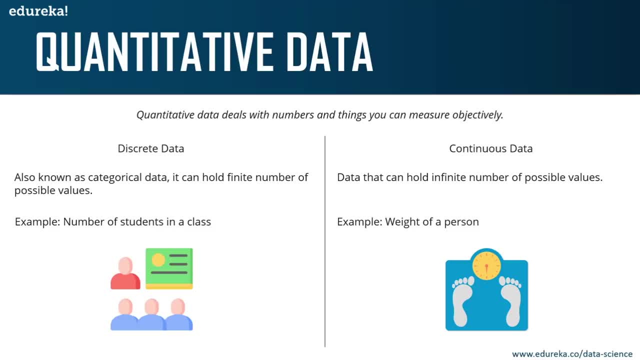 value right. so if you associate any sort of data with a variable, then it will become either discrete variable or continuous variable. there is also dependent and independent type of variables. now we won't discuss all of that in depth because that's pretty understandable. I'm sure all of you know. 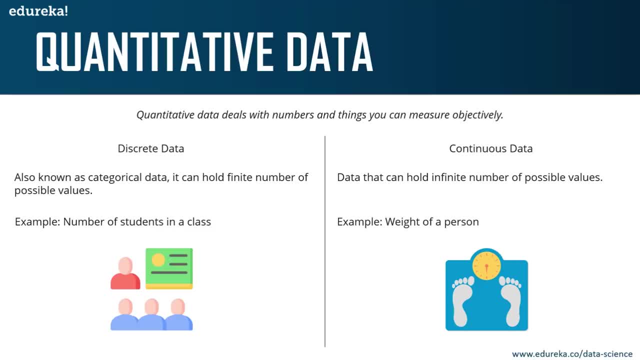 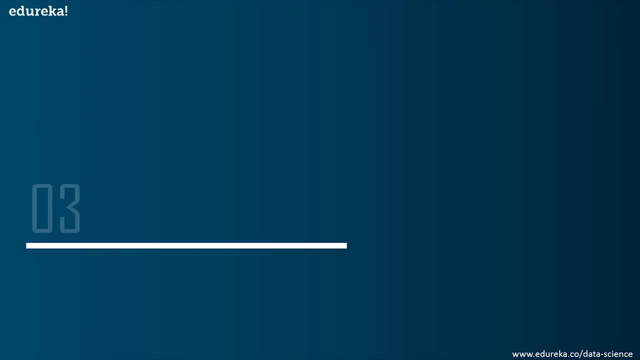 what is independent variable and dependent variable? right, dependent is any variable whose value depends on any other independent variable. so, guys, that much knowledge I expect all of you to have, all right. so now let's move on and look at our next topic, which is: what is statistics? now coming to the formal. 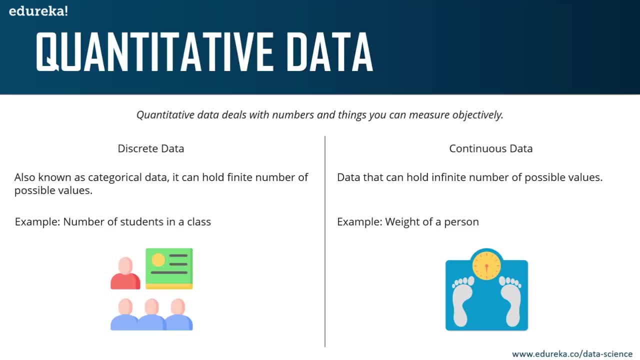 continuous data. All right, This is the difference between discrete and continuous data, And also I'd like to mention a few other things over here. Now, there are a couple of types of variables as well. All right, We have a discrete variable and we have a. 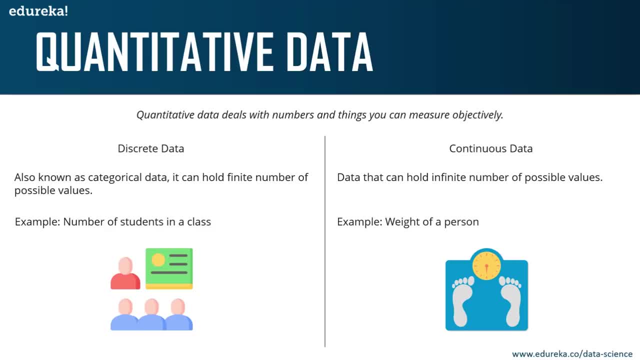 continuous variable. Discrete variable is also known as a categorical variable. All right, It can hold values of different categories. Let's say that you have a variable called message and there are two types of values that this variable can hold. Let's say that your message can either be a spam message or a non-spam message. Okay, That's when. 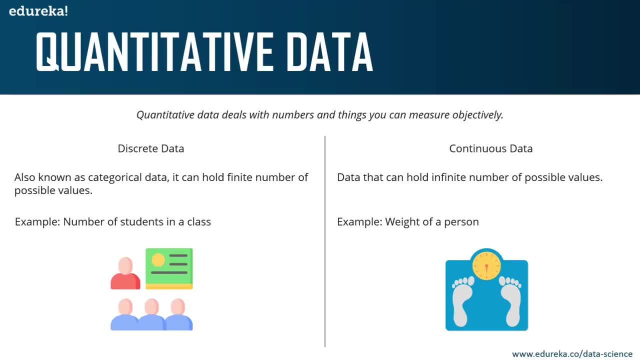 you call a variable as discrete or categorical variable. All right, Because it can hold values that represent different categories of data. Now, continuous variables are basically variables that can store infinite number of values, So the weight of a person can be denoted as a continuous. 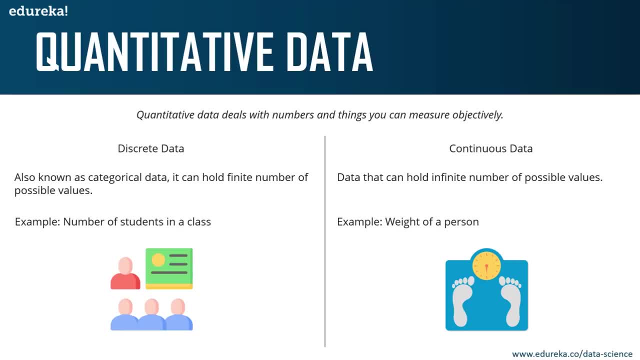 variable. All right, Let's say there is a variable called weight and it can store infinite number of possible values. That's why it's called a continuous variable. All right, So this is a continuous variable. So, guys, basically, variable is anything that can store a value, Right? So if 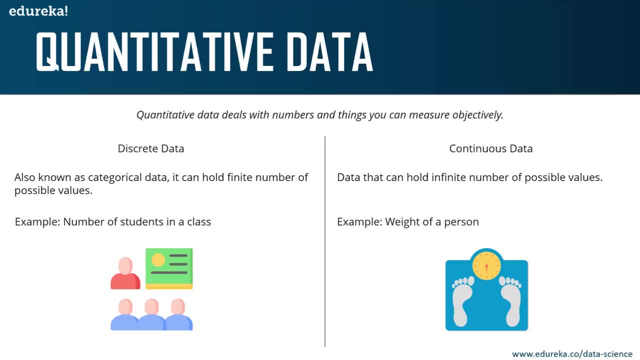 you associate any sort of data with a variable, then it will become either discrete variable or continuous variable. that is also dependent and independent type of variables. Now we won't discuss all of that in depth, because that's pretty understandable. I'm sure all of you know what is. 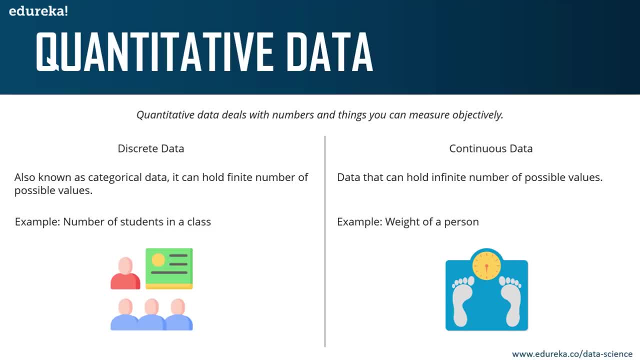 independent variable and dependent variable. Right, Dependent variable is any variable whose value depends on any other variable. All right. So if you associate any sort of data with a variable, independent variable. So guys, that much knowledge I expect all of you to have, All right. 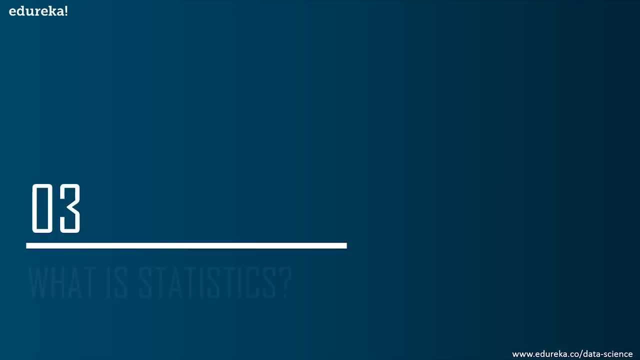 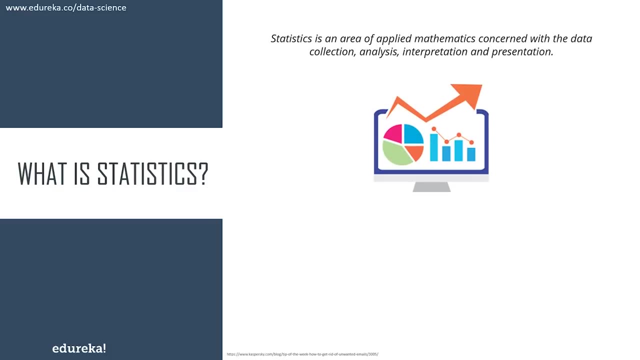 So now let's move on and look at our next topic, which is: what is statistics? Now coming to the formal definition of statistics: statistics is an area of applied mathematics which is concerned with data collection, analysis, interpretation and presentation. Now, usually when I speak about 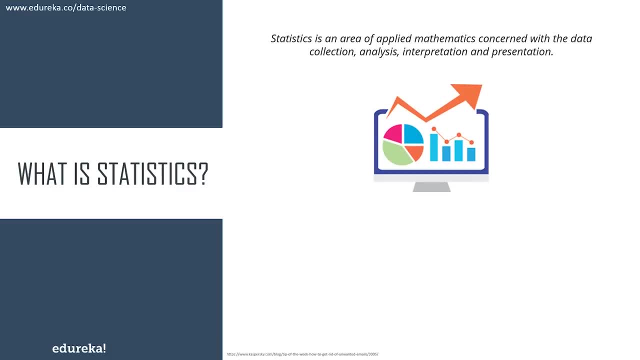 definition of statistics. statistics is an area of applied mathematics which is concerned with data collection, analysis, interpretation and presentation. now, usually when I speak about statistics, I'm not going to talk about statistics. I'm going to talk about data collection, analysis, interpretation and presentation. now, usually when I speak about statistics, 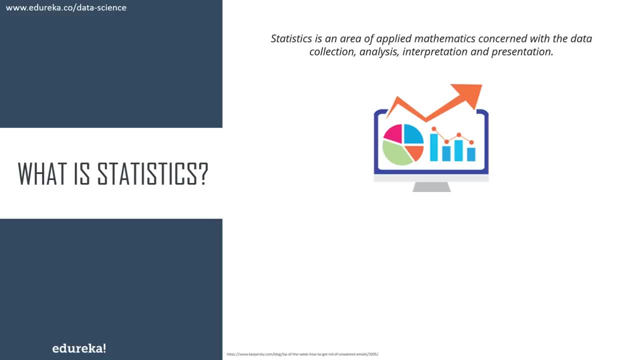 people think statistics is all about analysis. but statistics has other parts to it. it has. data collection is also a part of statistics. data interpretation, presentation, visualization- all of this comes into statistics. all right, you're going to use statistical methods to visualize data, to collect data, to interpret data, all right. so the area of mathematics deals with 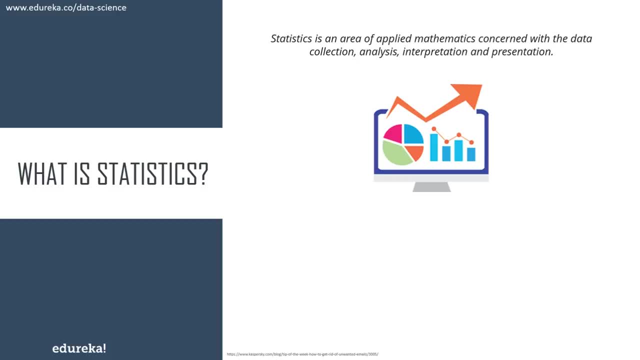 understanding how data can be used to solve complex problems. okay, now, as a, I'll give you a couple of examples that can be solved by using statistics. okay, let's say that your company has created a new drug that may cure cancer. how would you conduct a test to confirm the drugs effectiveness now, even though this 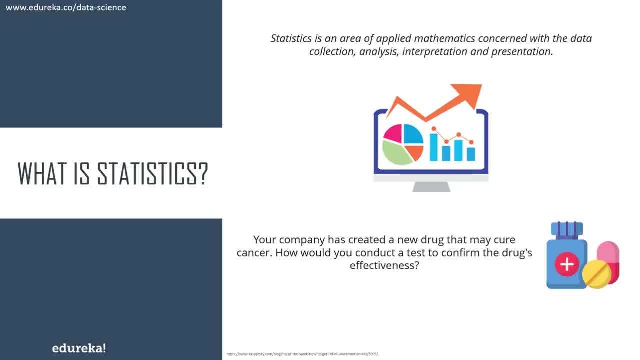 sounds like a biology problem. this can be solved with statistics. all right, you will have to create a test which can confirm the effectiveness of the drug. all right, this is a common problem that can be solved using statistics. let me give you another example. a friend are at a baseball game and out of the blue he offers you a bet that neither team will. 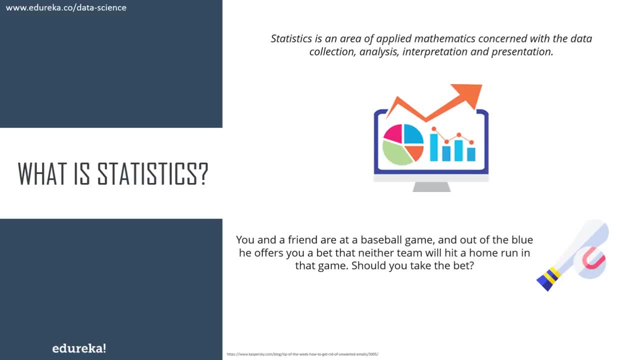 hit a home run in that game, Should you take the bet? All right. here you just discuss the probability of whether you'll win or lose. All right, this is another problem that comes under statistics. Let's look at another example. The latest sales data has just come in and your boss- 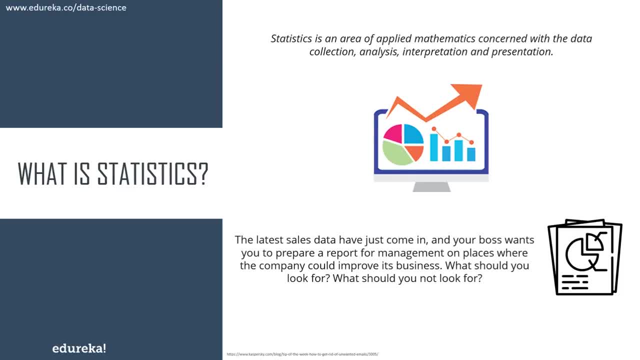 wants you to prepare a report for management on places where the company could improve its business. What should you look for and what should you not look for? Now, this problem involves a lot of data analysis. You'll have to look at the different variables that are causing your business. 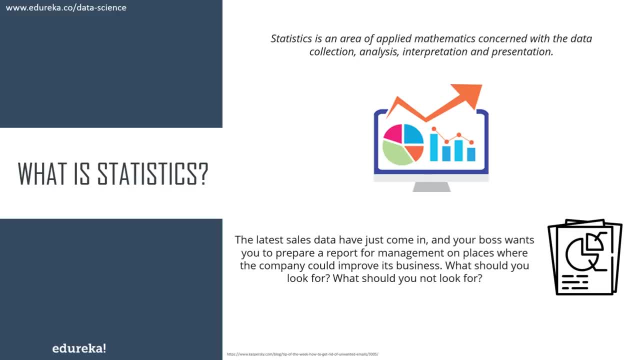 to go down, or that you have to look at a few variables that are increasing the performance of your models and thus growing your business. All right, so this involves a lot of data analysis, and the basic idea behind data analysis is to use statistical techniques in order to figure out the 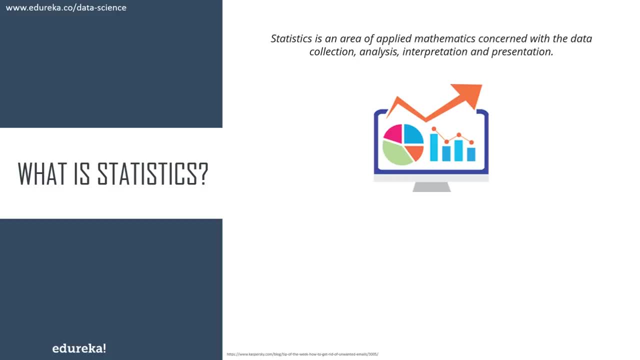 statistics. people think statistics is all about analysis, But statistics has other parts to it. It has. data collection is also a part of statistics. Data interpretation, presentation, visualization- all of this comes into statistics. All right, You're going to use statistical methods to visualize data, to collect data, to interpret data. 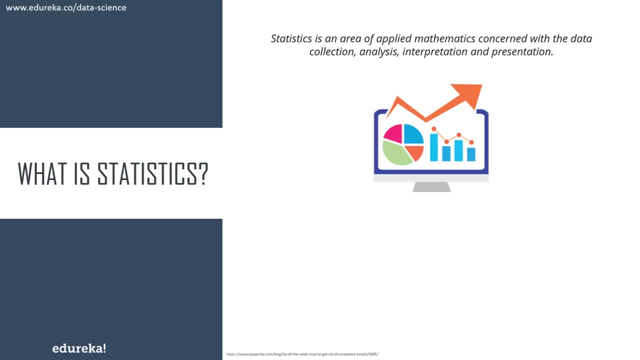 All right. So the area of mathematics deals with understanding how data can be used to solve complex problems. Okay, Now I'll give you a couple of examples that can be solved by using statistics. Okay, Let's say that your company has created a. 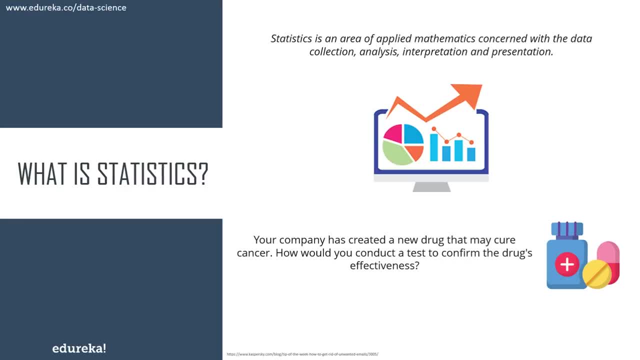 new drug that may cure cancer, How would you conduct a test to confirm the drug's effectiveness? Now, even though this sounds like a biology problem, This can be solved with statistics. All right, You will have to create a test which can confirm the effectiveness of the drug. 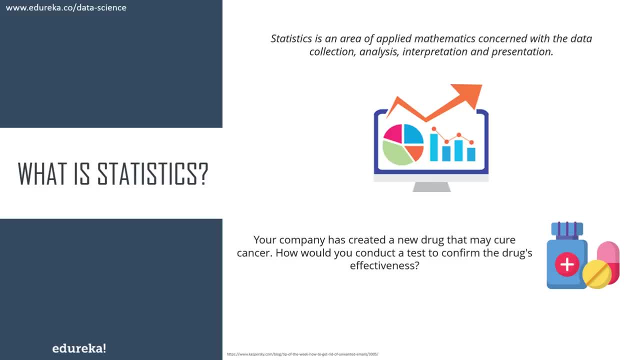 All right, This is a common problem that can be solved using statistics. Let me give you another example. You and a friend are at a baseball game And out of the blue, he offers you a- Virginia offers you a bet that neither team will hit a home run in that game. should you take the bet? 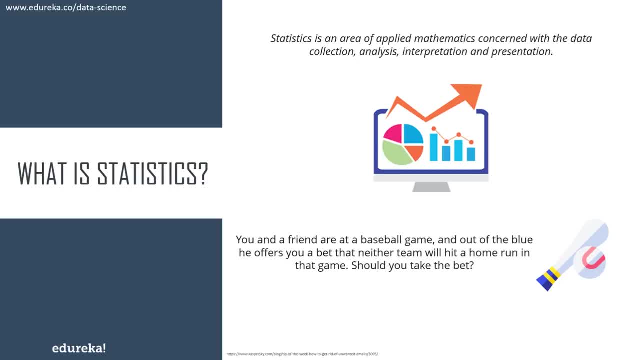 all right. here you just discuss the probability of whether you'll win or lose. all right, this is another problem that comes under statistics. let's look at another example. the latest sales data has just come in and your boss wants you to prepare a report for management on places where the company 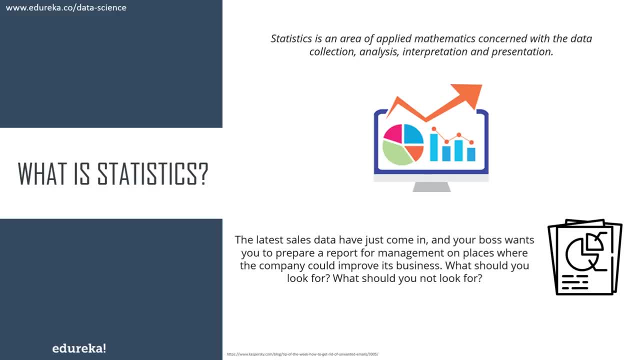 could improve its business. what should you look for and what should you not look for now? this problem involves a lot of data analysis. you'll have to look at the different variables that are causing your business to go down or that you have to look at a few variables that are increasing. 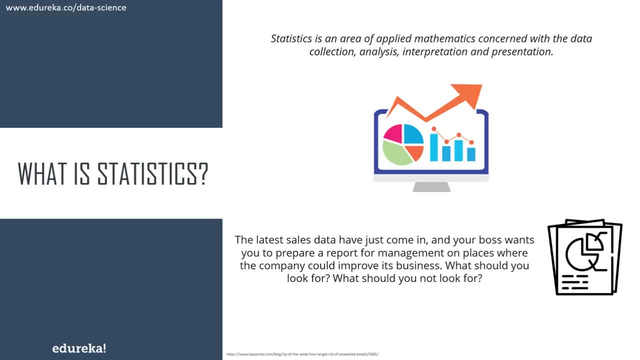 the performance of your models and thus growing your business. all right, so this involves a lot of data analysis, and the basic idea behind data analysis is to use statistical techniques in order to figure out the relationship between different variables or different components in your business. okay, so now let's move on. 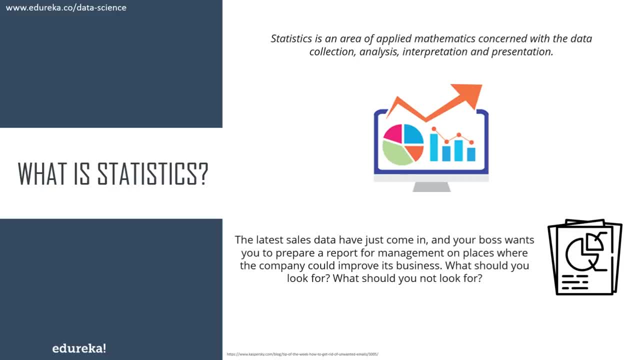 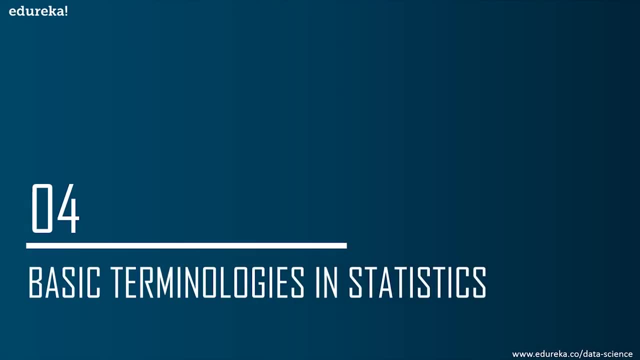 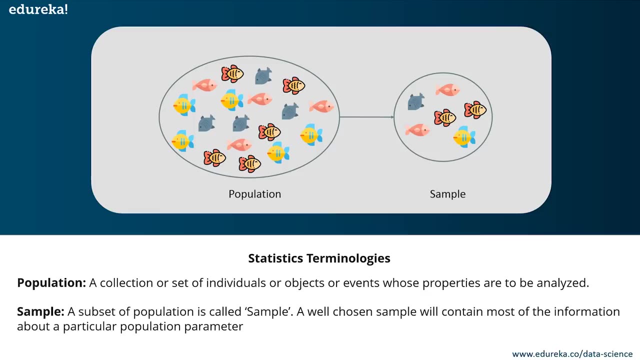 relationship between different variables or different components in your business. Okay, so now let's move on and look at our next topic, which is basic terminologies in statistics. Now, before you dive deep into statistics, it is important that you understand basic terminologies used in statistics. The two: 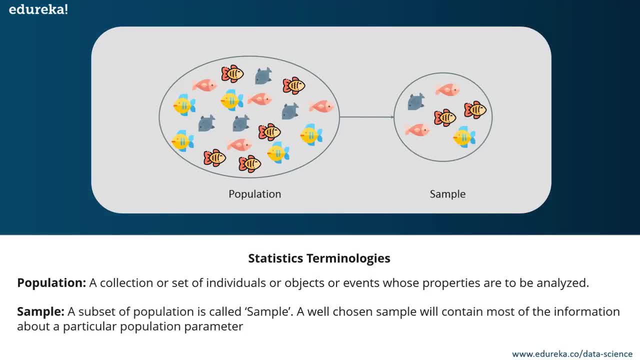 most important terminologies in statistics are population and sample. So throughout the statistics course, or throughout any problem that you're trying to solve with statistics, you will come across these two words, which is population and sample. Now, population is a collection or a set of individuals or objects or events whose properties are to be analyzed. 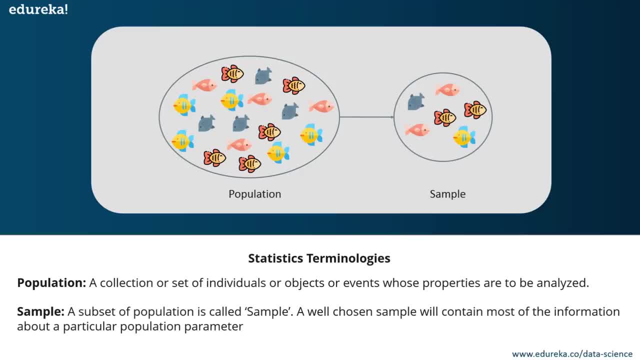 Okay. so basically, you can refer to population as a subject that you're trying to analyze Now. a sample is just like the word suggests: it's a subset of the population. So you have to make sure that you choose the sample in such a way that it represents the entire population. 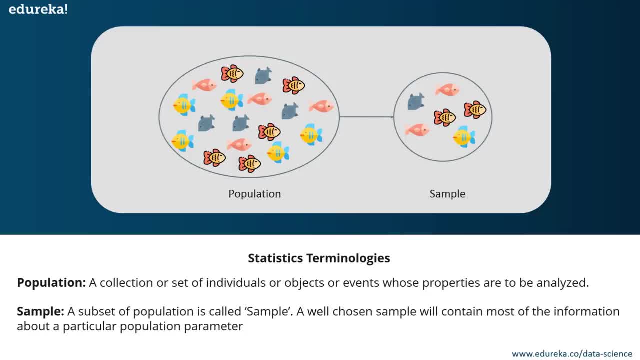 All right, it shouldn't focus at one part of the population. Instead, it should represent the entire population. That's how your sample should be chosen. So a well chosen sample will contain most of the information about a particular population parameter. Now you 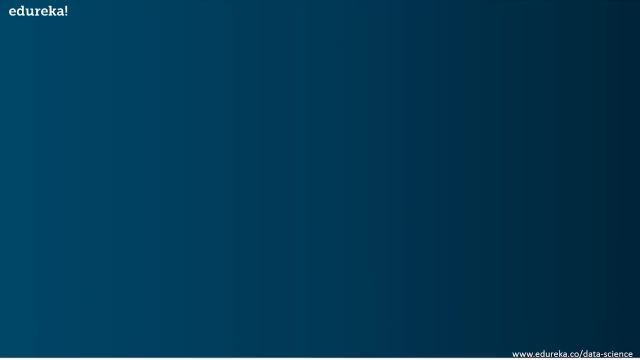 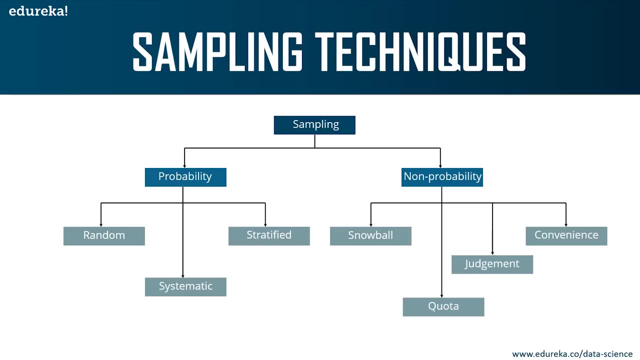 must be wondering how can one choose a sample that best represents the entire population. Now, sampling is a statistical method that deals with the selection of individual observations within a population. So sampling is performed in order to infer statistical knowledge about a population. All right, if you want to. 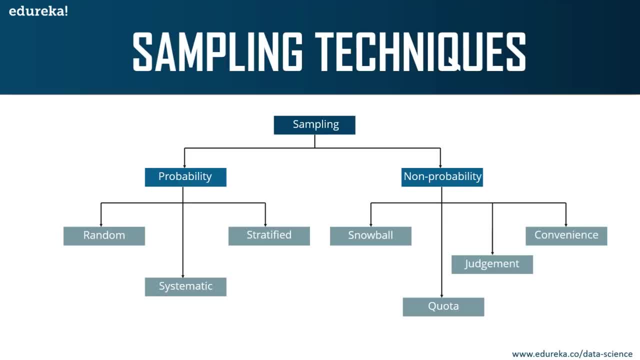 understand the different statistics of a population, like the mean, the median, the mode or the standard deviation or the variance of a population, then you're going to perform sampling, All right, because it's not reasonable for you to study a large population and find out the mean, median and 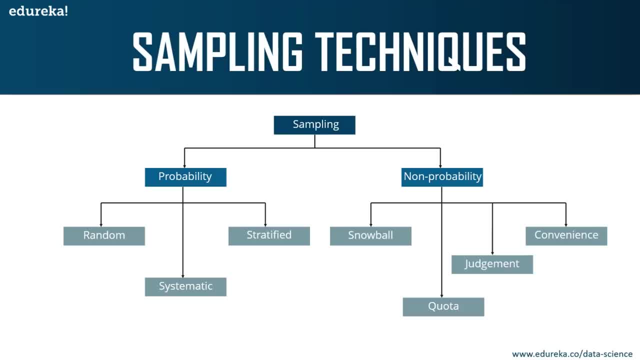 everything else. So why is sampling performed? You might ask. what is the point of sampling? we can just study the entire population. Now, guys, think of a scenario wherein you're asked to perform a survey about the eating habits of teenagers in the US. 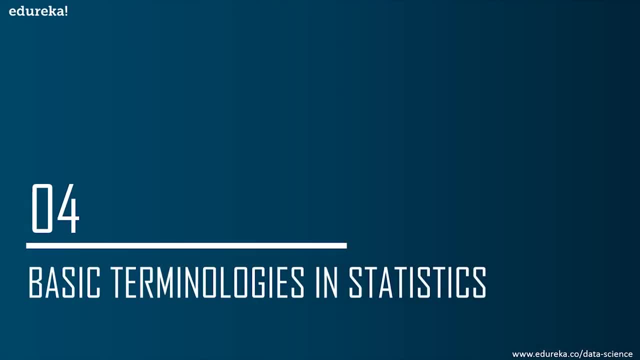 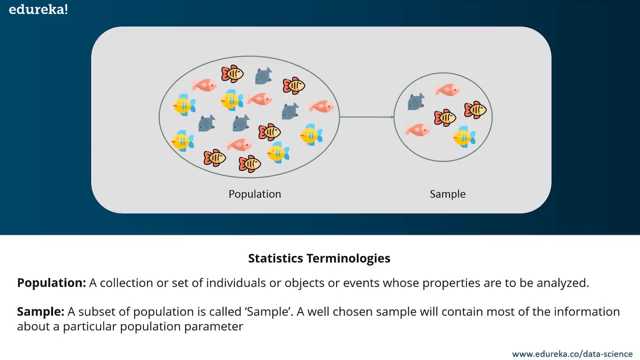 you and look at our next topic, which is basic terminologies in statistics. now, before you dive deep into statistics, it is important that you understand the basic terminologies used in statistics. the two most important terminologies in statistics are population and sample. so throughout the statistics course, or throughout any problem that you're trying 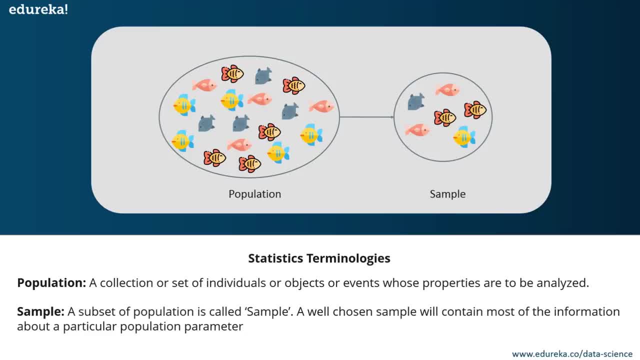 to solve with statistics. you will come across these two words, which is population and sample. now, population is a collection or a set of individuals or objects or events whose properties are to be analyzed. okay, so basically you can refer to population as a subject that you're trying to 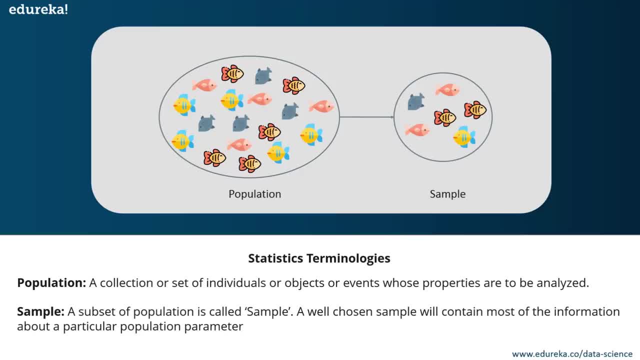 analyze now. a sample is just like the word suggests: it's a subset of the population. so you have to make sure that you choose the sample in such a way that it represents the entire population. all right, it shouldn't focus at one part of the population. instead, it should. 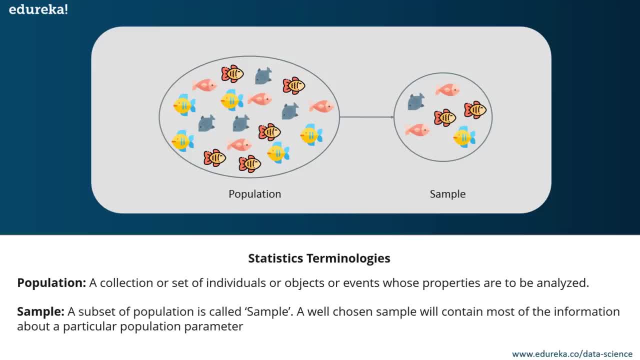 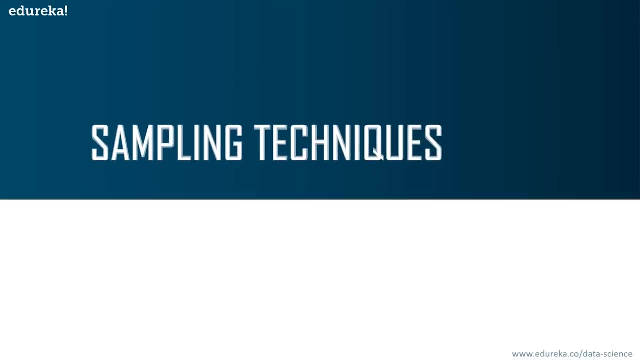 represent the entire population. That's how your sample should be chosen. So a well chosen sample will contain most of the information about a particular population parameter. Now you must be wondering how can one choose a sample that best represents the entire population? Now, sampling is a statistical method. 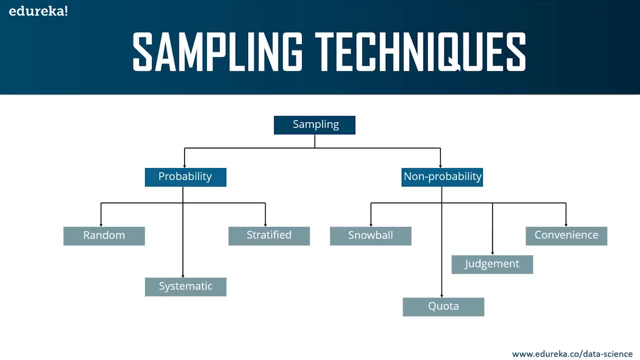 that deals with the selection of individual observations within a population. So sampling is performed in order to enforce statistical knowledge about a population. All right, if you want to understand the different statistics of a population, like the mean, the median, the mode or the standard deviation or the variance of a population. 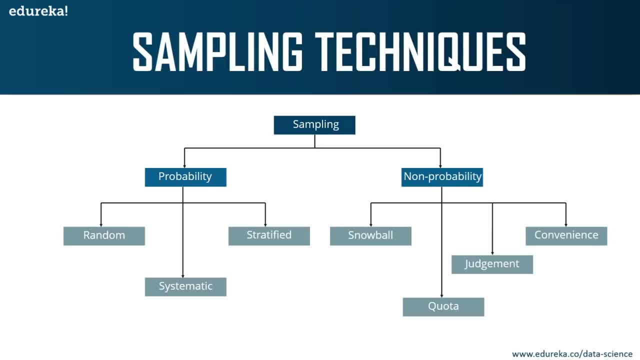 then you're going to perform sampling. All right, because it's not reasonable for you to study a large population and find out the mean median and everything else. So why is sampling performed? You might ask: what is the point of sampling? 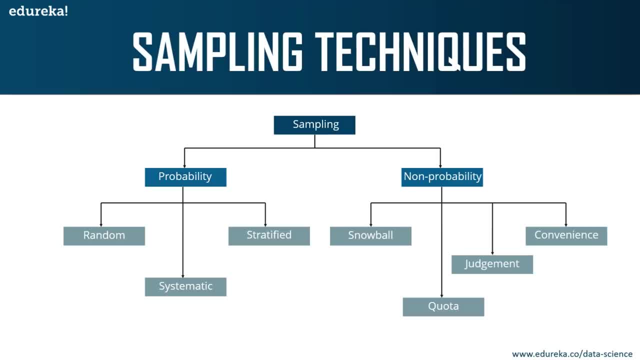 We can just study the entire population. Now, guys, think of a scenario wherein you're asked to perform a survey about the eating habits of teenagers in the US. So at present there are over 42 million teens in the US and this number is growing as we are speaking right now. 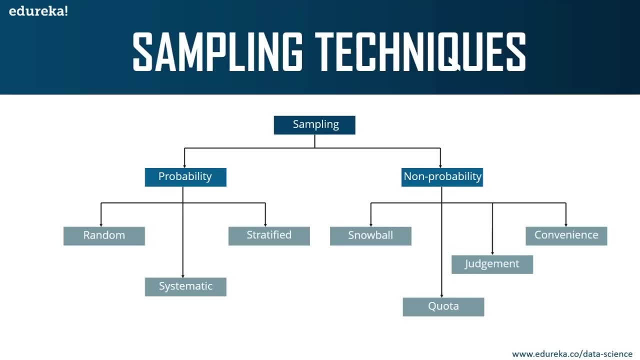 Correct. Is it possible to survey each of these 42 million individuals about their health? Is it possible? Well, it might be possible, but this will take forever to do Now. obviously it's not. it's not reasonable to go around. 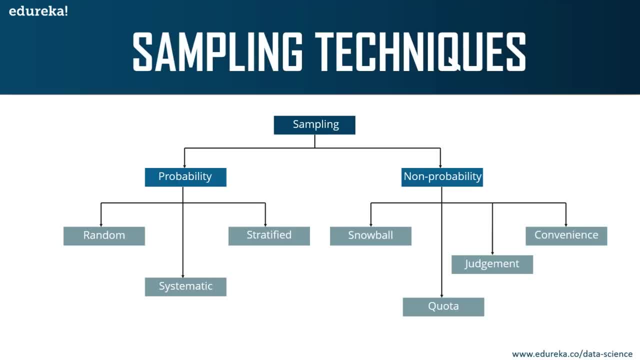 So at present, there are over 42 million teens in the US, and this number is growing as we are speaking right now. Correct? Is it possible to survey each of these 42 million individuals about their health? Is it possible? Well, it might be possible, but this will take forever. 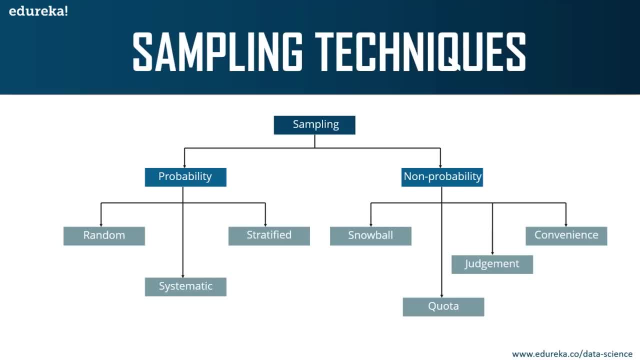 to do? Obviously it's not. It's not reasonable to go around knocking each door and asking for what does your teenage son eat? and all of that all right. This is not very reasonable. That's why sampling is used. It's a method wherein a sample of the population is studied. 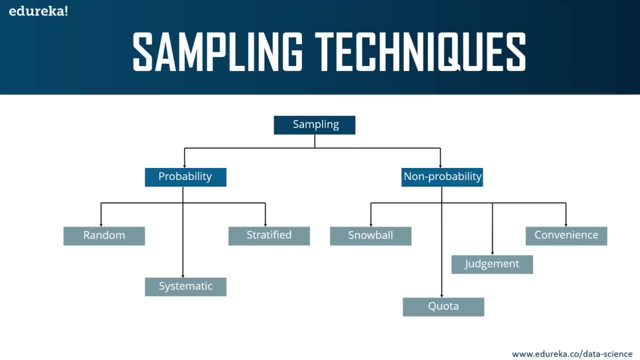 in order to draw inference about the entire population. So it's basically a shortcut to studying the entire population. Instead of taking the entire population and finding out all the solutions, you're just going to take a part of the population that represents the entire population. 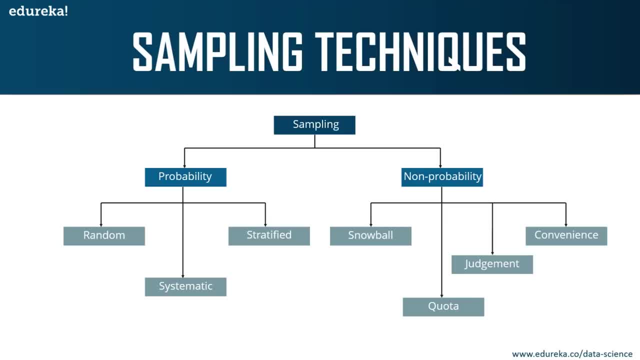 and you're going to perform all your statistical analysis, your inferential statistics, on that small sample, all right, And that sample basically represents the entire population, all right. So I'm sure I've made this clear to you all: what is sample and what is population. 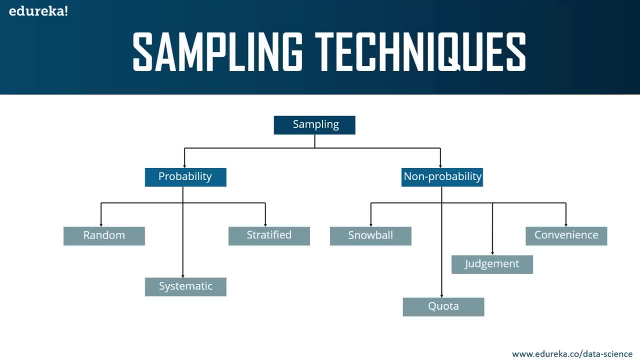 Now there are two main types of sampling techniques that I'll discuss today. We have probability sampling and non-probability sampling. Now, in this video, we'll only be focusing on probability sampling techniques, because non-probability sampling is not within the scope of this video. all right, 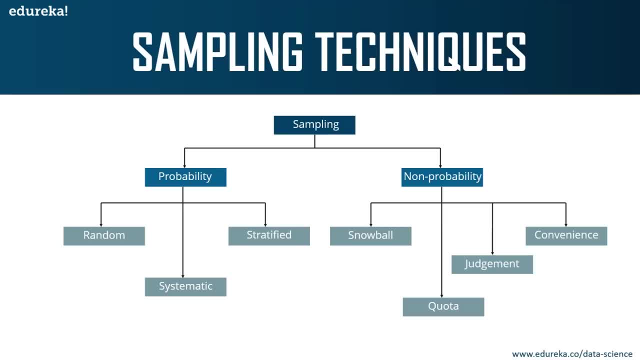 We'll only discuss the probability part, because we're focusing on statistics and probability, correct? Now again, under probability sampling, we have three different types. We have random sampling, systematic and stratified sampling. all right, And just to mention the different types. 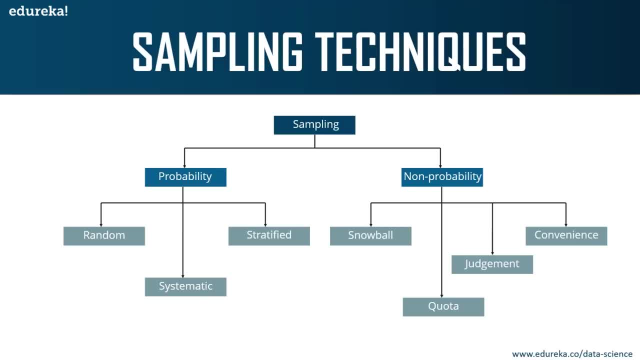 of non-probability samplings. we have snowball quota judgment and convenient sampling, all right. Now, guys, in this session I'll only be focusing on probability, So let's move on and look at the different types. 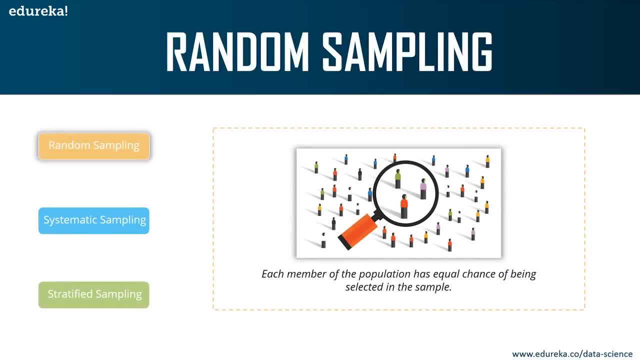 of probability sampling. So what is probability sampling? It is a sampling technique in which samples from a large population are chosen by using the theory of probability. all right, So there are three types of probability sampling, all right. First we have the random sampling. 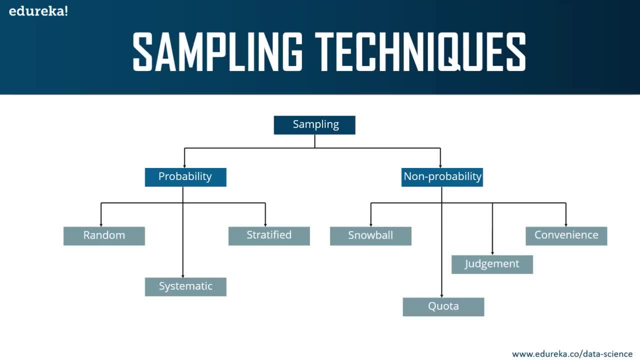 knocking each door and asking for what does your teenage son eat? and all of that all right. This is not very reasonable. That's why sampling is used. It's a method wherein a sample of the population is studied in order to draw inference about the entire population. 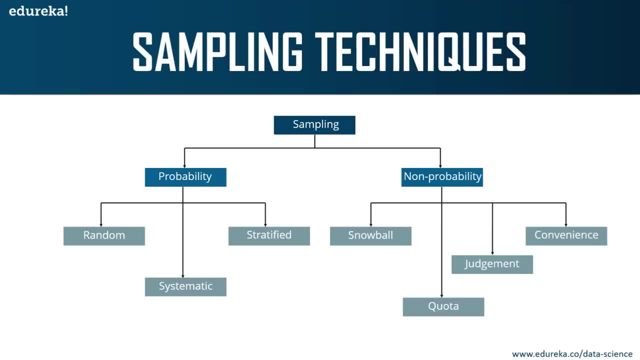 So it's basically a shortcut to studying the entire population. Instead of taking the entire population and finding out all the solutions, you're just going to take a part of the population that represents the entire population and you're gonna perform all your statistics. 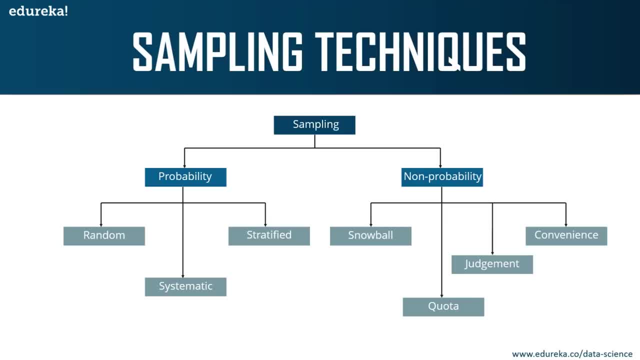 statistical analysis, your inferential statistics on that small sample, all right, and that sample basically represents the entire population, all right. so i'm sure i've made this clear to you all: what is sample and what is population. now there are two main types of sampling techniques: that 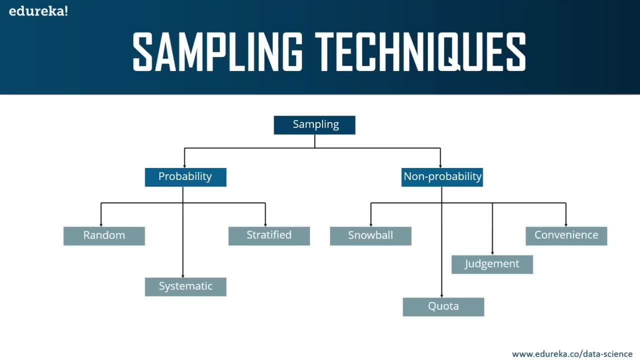 i'll discuss today. we have probability sampling and non-probability sampling now in this video we'll only be focusing on probability sampling techniques, because non-probability sampling is not within the scope of this video. all right, we'll only discuss the probability part, because we're 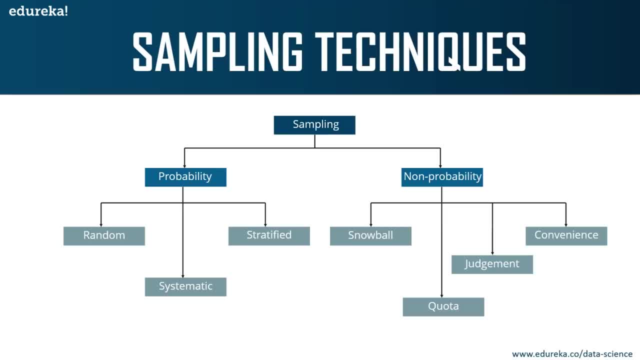 focusing on statistics and probability, correct. now again, under probability sampling, we have three different types. we have random sampling, systematic and stratified sampling- all right. and just to mention the different types of non-probability samplings, we have snowball, quota judgment and convenient sampling- all right. 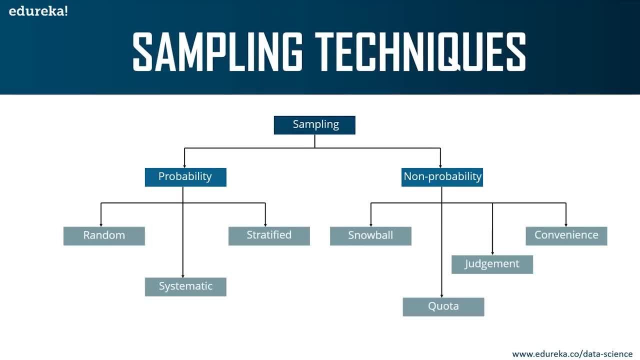 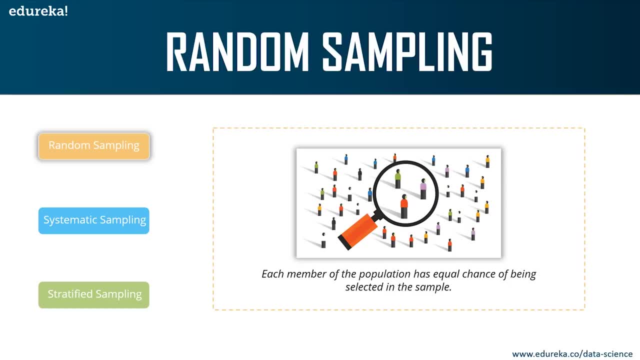 Now, guys, in this session, I'll only be focusing on probability, so let's move on and look at the different types of probability sampling. So what is probability sampling? It is a sampling technique in which samples from a large population are chosen by using the theory of probability. all right, 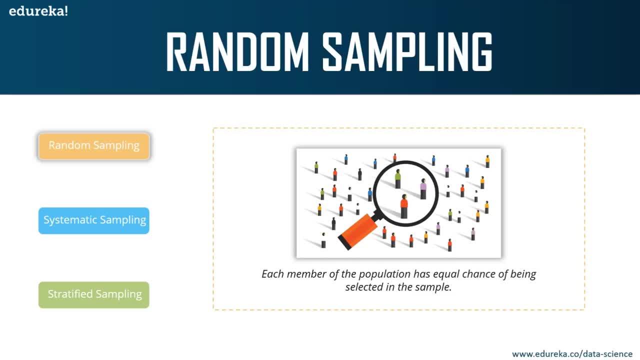 So there are three types of probability sampling. all right. First, we have the random sampling. Now, in this method, each member of the population has an equal chance of being selected in the sample. All right, so each and every individual or each and every object in the population. 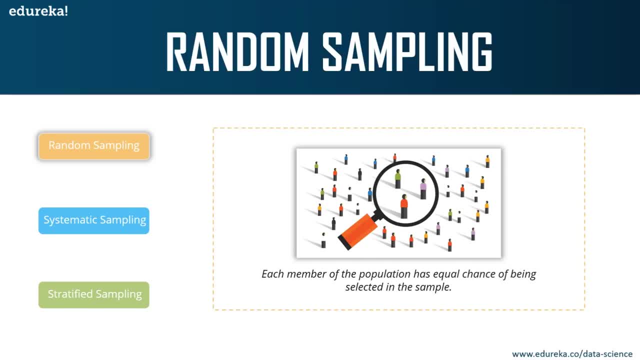 has an equal chance of being a part of the sample. That's what random sampling is all about. okay, You're randomly going to select any individual or any object, so this way, each individual has an equal chance of being selected, correct? 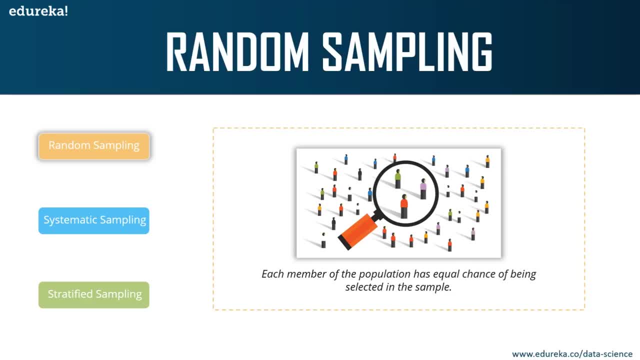 Now, in this method, every member of the population has an equal chance of being selected in the sample. all right, So each and every individual or each and every object in the population has an equal chance of being a part of the sample. That's what random sampling is all about, okay. 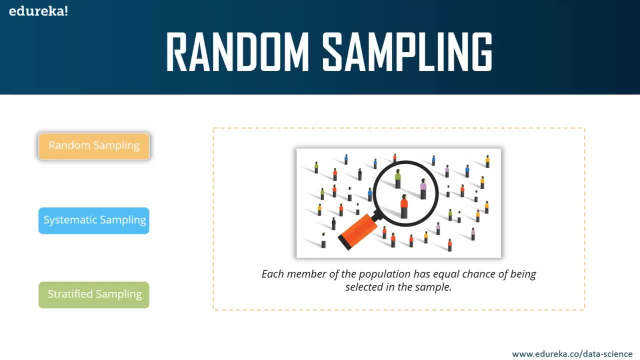 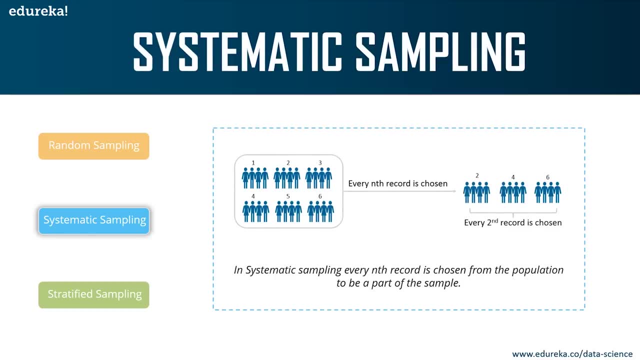 You're randomly going to select any individual or any object, So this way, each individual has an equal chance of being selected, correct? Next we have systematic sampling. Now, in systematic sampling, every nth record is chosen from the population to be a part of the sample. all right, 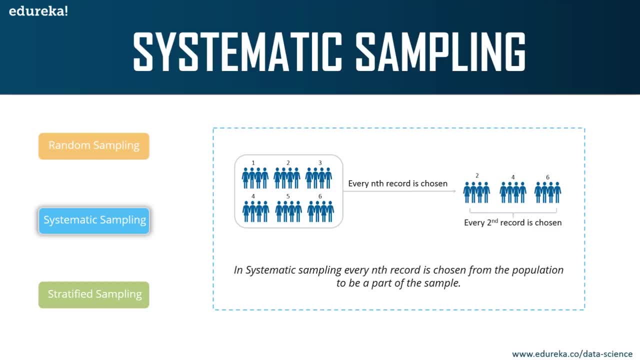 Now refer this image that I've shown over here. Out of these six groups, every second group is chosen as a sample. okay, So every second record is chosen here, and this is how systematic sampling works. okay, You're randomly selecting the nth record. 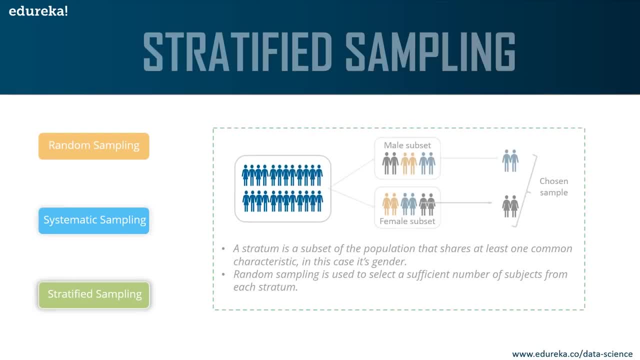 and you're going to add that to your sample. Next, we have stratified sampling Now. in this type of technique, a stratum is used to form samples from a large population. So what is a stratum? A stratum is basically a subset of the population. 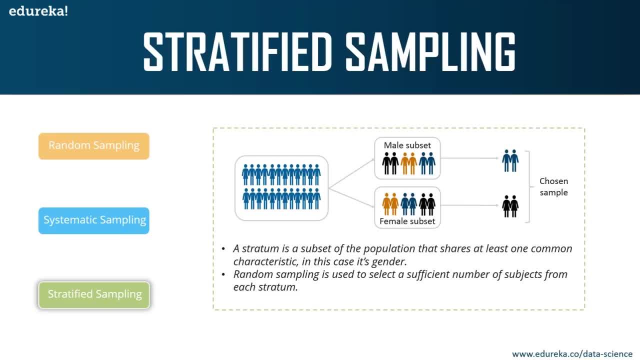 that shares at least one common characteristics. So let's say that your population has a mix of both male and female. So you can create two stratums out of this. One will have only the male subset and the other will have the female subset. all right, 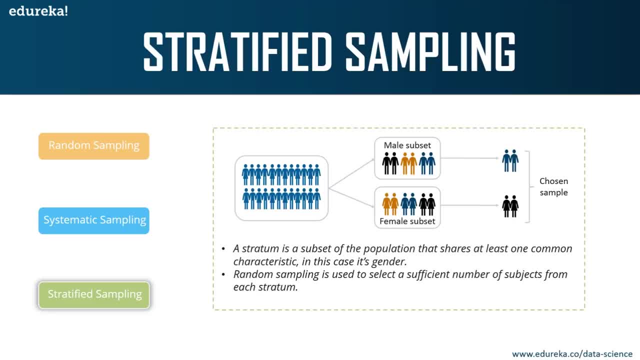 This is what stratum is. It is basically a subset of the population that shares at least one common characteristics. all right, In our example, it is gender. So after you've created a stratum, you're going to use random sampling on these stratums. 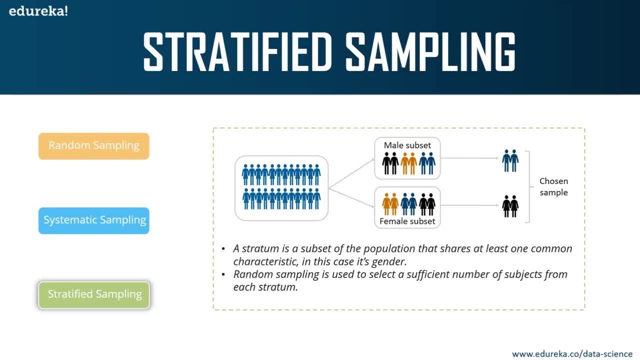 and you're going to choose a final sample. So random sampling, meaning that all of the individuals in each of the stratum will have an equal chance of being selected in the sample, correct? So, guys, these were the three different types of sampling techniques. 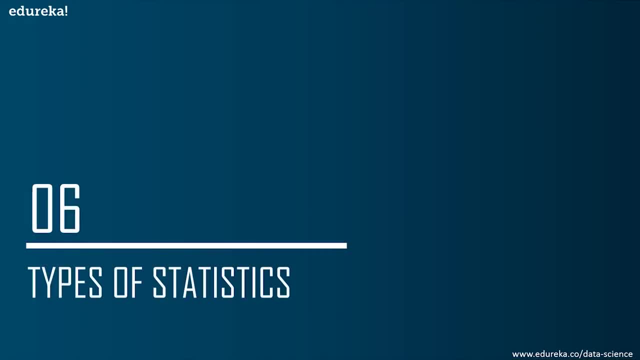 Now let's move on and look at our next topic, which is different types of statistics. So after this, we'll be looking at the more advanced concepts of statistics. all right, So far we discussed the basics of statistics, which is basically what is statistics? 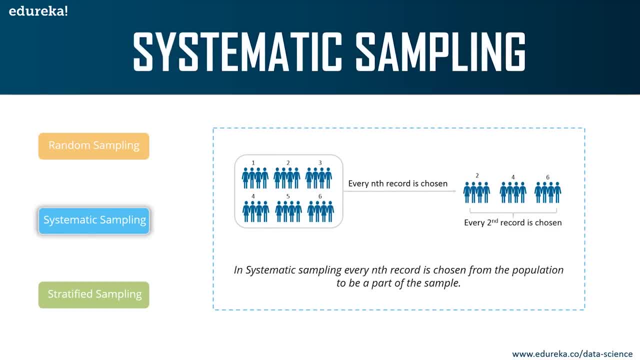 Next we have systematic sampling. Now, in systematic sampling, every nth record is chosen from the population to be a part of the sample. all right, Now refer this image that I've shown over here: Out of these six groups, every second group is chosen as a sample. okay, 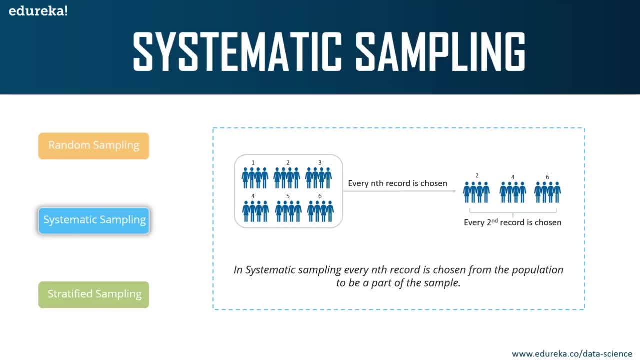 So every second record is chosen here, and this is how systematic sampling works. Okay, you're randomly selecting the nth record and you're going to add that to your sample. Next we have stratified sampling Now. in this type of technique, 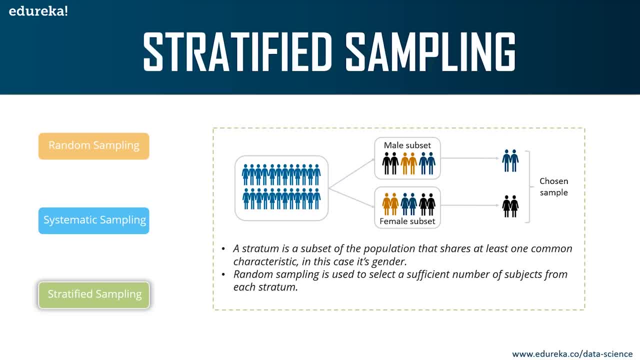 a stratum is used to form samples from a large population. So what is a stratum? A stratum is basically a subset of the population that shares at least one common characteristics. So let's say that your population has a mix of both male and female. 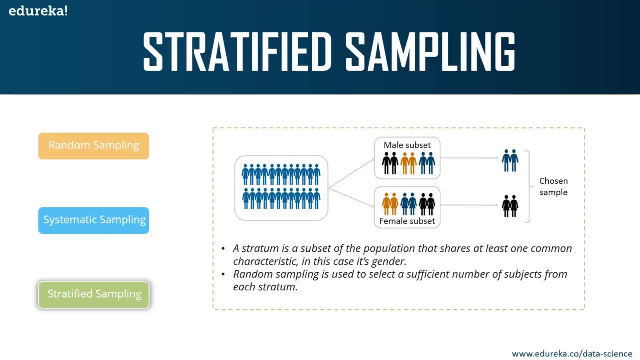 So you can create two stratums out of this. One will have only the male subset and the other will have the female subset. All right, this is what stratum is. It is basically a subset of the population that shares at least one common characteristics. all right, 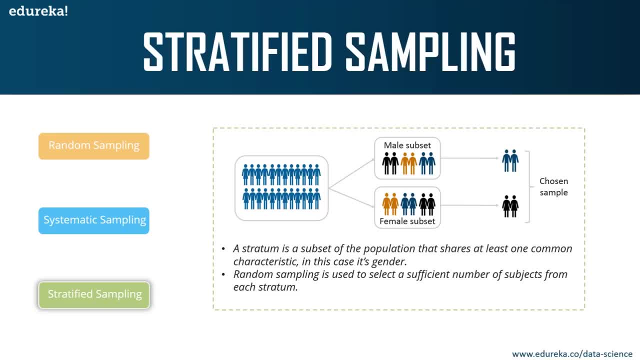 In our example it is gender. So, after you've created a stratum, you're going to use random sampling on these stratums and you're going to choose a final sample. So random sampling meaning that all of the individuals in each of the stratum will have an equal chance. 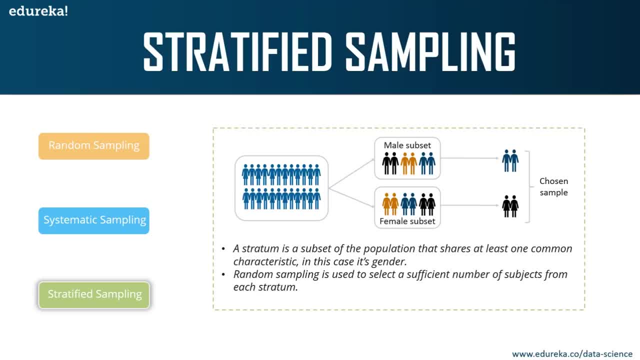 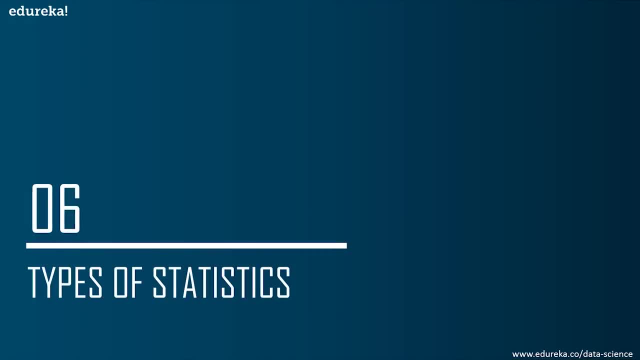 of being selected in the sample, correct? So, guys, these were the three different types of sampling techniques. Now let's move on and look at our next topic, which is the different types of statistics. So after this, we'll be looking at the more advanced 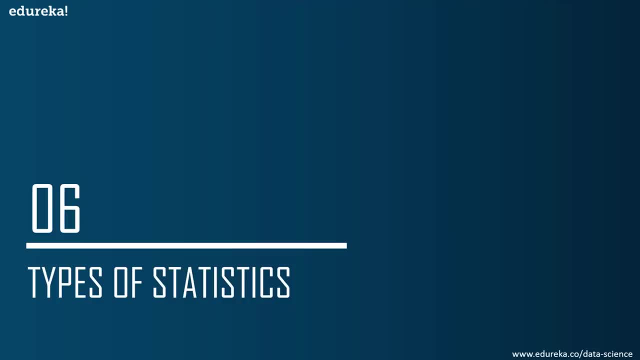 concepts of statistics. all right, So far we discussed the basics of statistics, which is basically what is statistics, the different sampling techniques and the terminologies in statistics. all right, Now we look at the different types of statistics. So there are two major types of statistics. 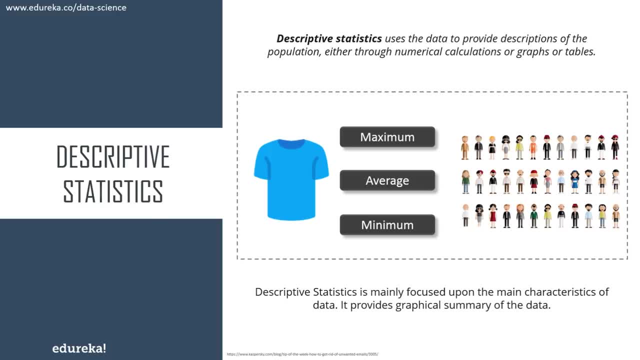 descriptive statistics and inferential statistics. In today's session, we'll be discussing both of these types of statistics in depth. all right, We'll also be looking at a demo, which I'll be running in the R language in order to make you understand what exactly. 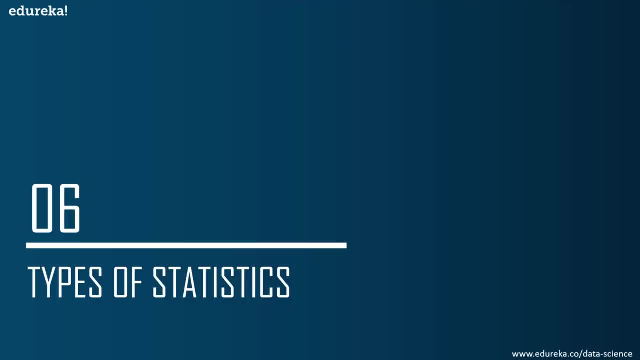 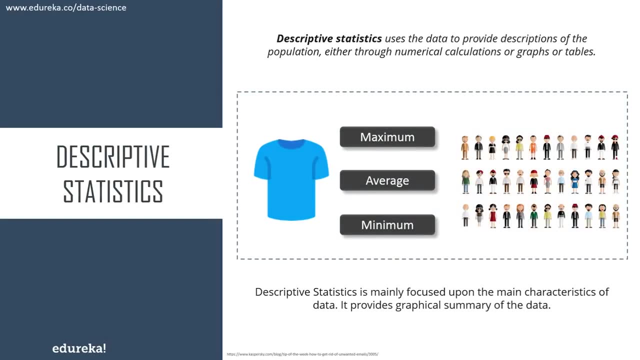 the different sampling techniques and the terminologies in statistics. all right, Now we look at the different types of statistics. So there are two major types of statistics: descriptive statistics and inferential statistics. In today's session we'll be discussing both of these types of statistics in depth. all right, 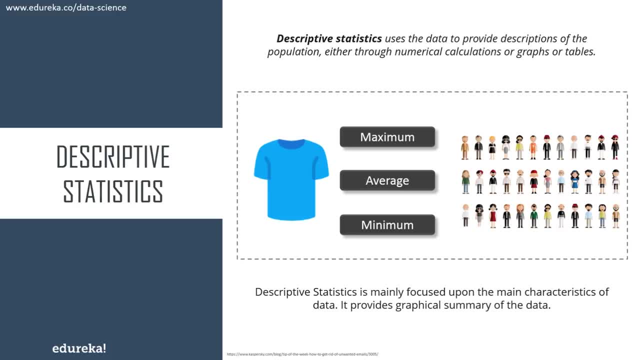 We'll also be looking at a demo, which I'll be running in the R language, in order to make you understand what exactly descriptive and inferential statistics is. So, guys, we're just going to look at the basics, so don't worry if you don't have much knowledge. 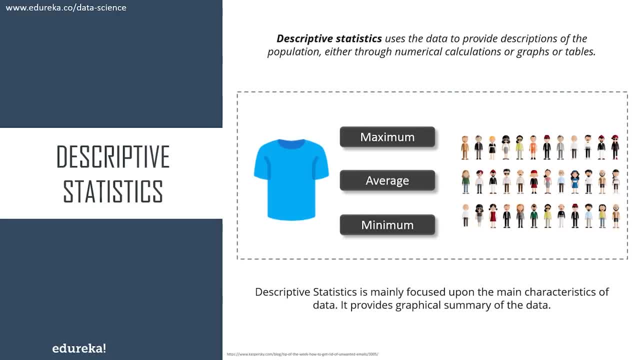 I'm explaining everything from the basic level, all right. So, guys, descriptive statistics is a method which is used to describe and understand the features of specific data set by giving a short summary of the data. Okay, So it is mainly focused upon the characteristics of data. 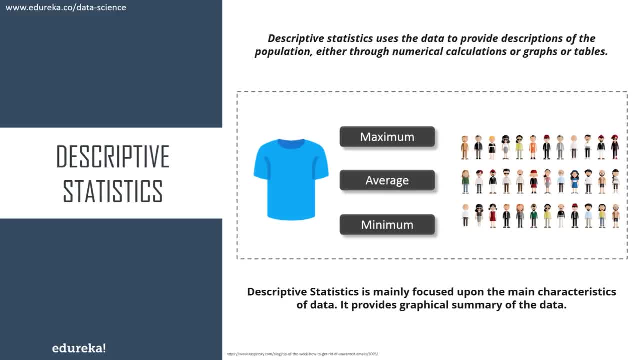 It also provides a graphical summary of the data. Now, in order to make you understand what descriptive statistics is, let's suppose that you want to gift all your classmates a T-shirt, So to study the average shirt size of a student in a classroom. 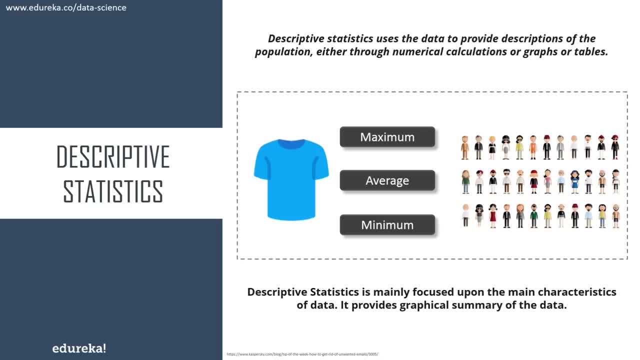 so if you were to use descriptive statistics to study the average shirt size of students in your classroom, then what you would do is you would record the shirt size of a student in your classroom. You would record the shirt size of all students in the class. 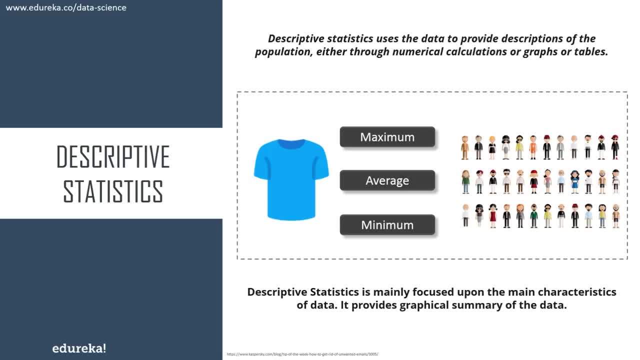 and then you would find out the maximum, minimum and average shirt size of the class. okay, So coming to inferential statistics, inferential statistics makes inferences and predictions about a population based on the sample of data taken from the population. okay, 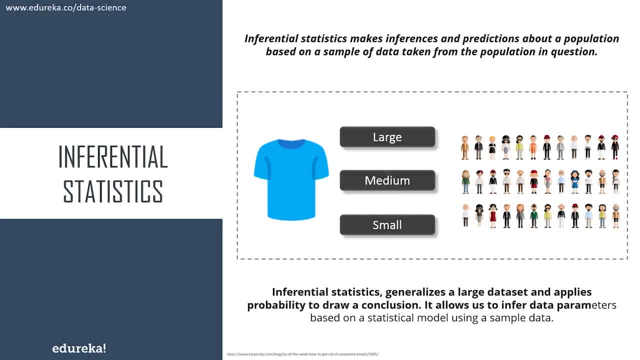 So, in simple words, it generalizes a large data set and it applies probability to draw a conclusion. okay, So it allows you to infer data parameters based on a statistical model by using sample data. So if we consider the same example of finding the average shirt size of students in a class, 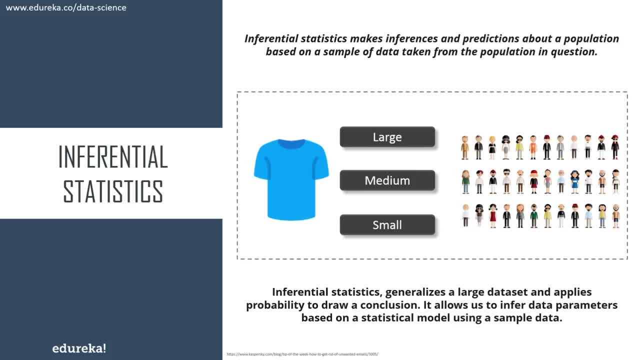 in inferential statistics you will take a sample set of the class, which is basically a few people from the entire class. all right, You already have had grouped the class into large, medium and small. all right, In this method, you basically build a statistical model. 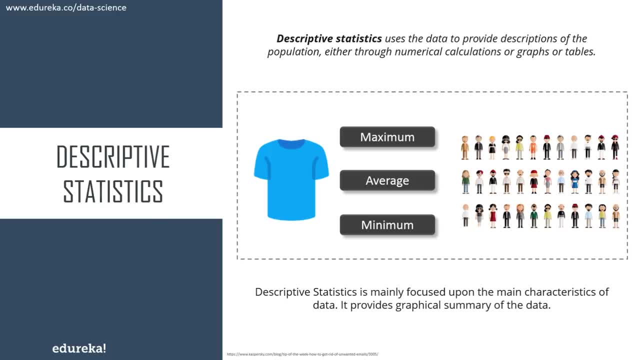 descriptive and inferential statistics is. So, guys, we're just gonna look at the basics, so don't worry if you don't have much knowledge. I'm explaining everything from the basic level, all right. So, guys, descriptive statistics is a method. 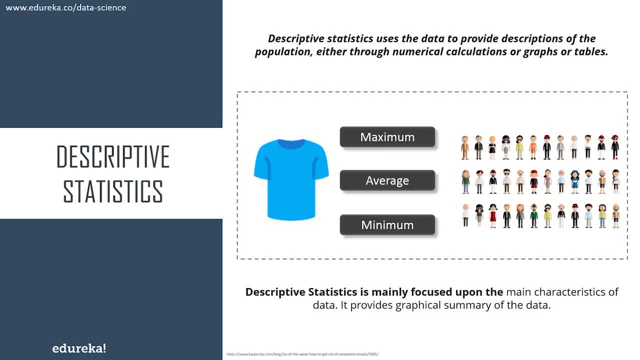 which is used to describe and understand the features of specific data set by giving a short summary of the data. okay, So it is mainly focused upon the characteristics of data. It also provides a graphical summary of the data Now, in order to make you understand. 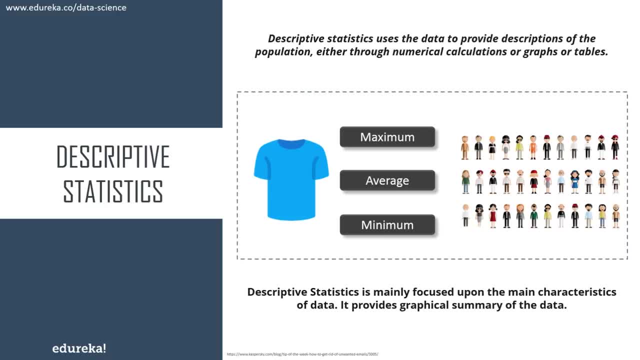 what descriptive statistics is. let's suppose that you want to gift all your classmates a T-shirt So to study the average shirt size of a student in a classroom. so if you were to use descriptive statistics to study the average shirt size of students in your classroom, then what you would do is: 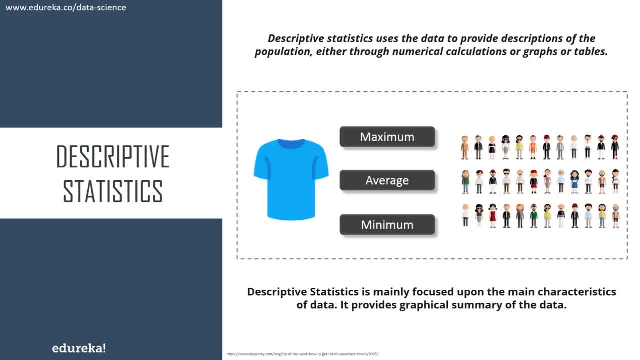 you would record the shirt size of all students in the class and then you would find out the maximum, minimum and average shirt size of the class. okay, So coming to inferential statistics. inferential statistics makes inferences and predictions about a population based on the sample of data. 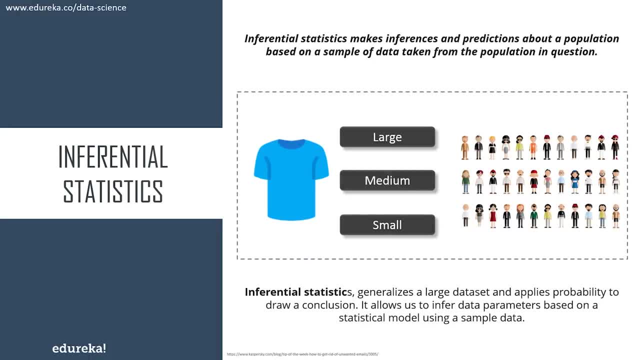 taken from the population. okay, So, in simple words, it generalizes a large data set and it applies probability to draw a conclusion. okay, So it allows you to infer data parameters based on a statistical model by using sample data. So, if we consider the same example, 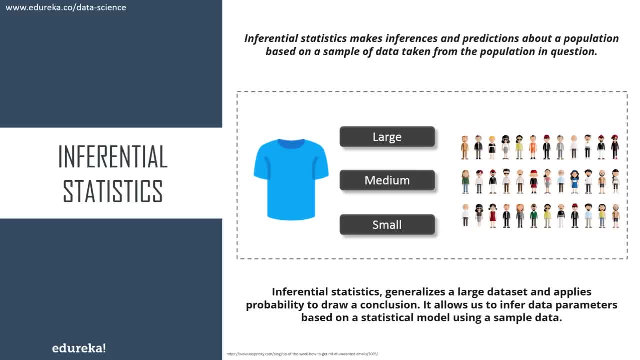 of finding the average shirt size of students in a class in inferential statistics. you will take a sample set of the class, which is basically a few people from the entire class. all right, You already have had grouped the class into large, medium and small, all right. 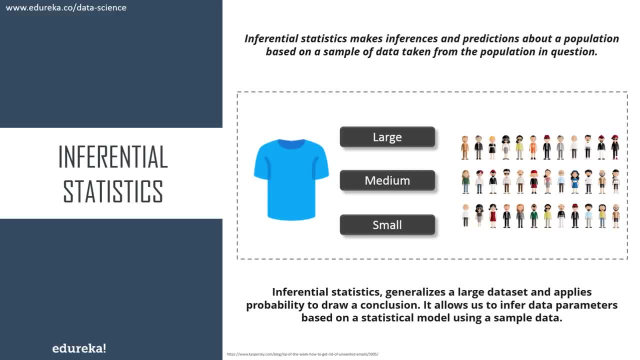 In this method, you basically build a statistical model and expand it for the entire population In the class. So, guys, that was a brief understanding of descriptive and inferential statistics. So that's the difference between descriptive and inferential. Now, in the next section, we'll go in depth. 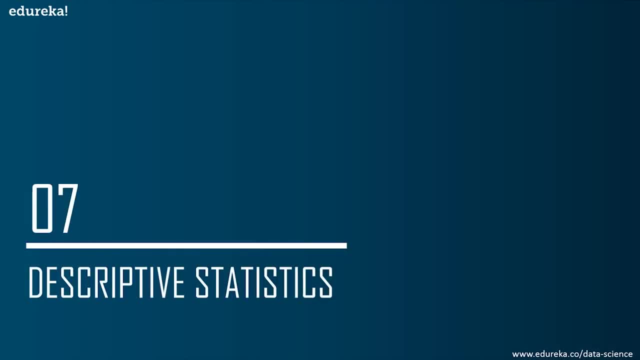 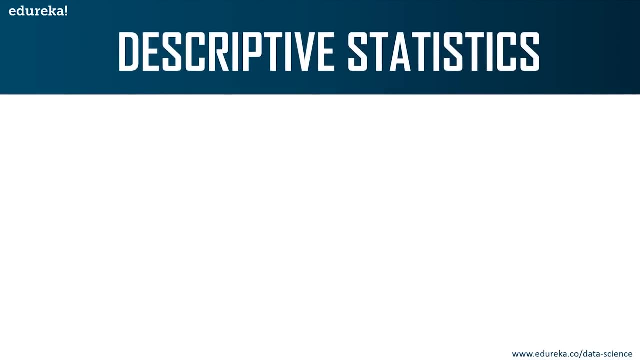 about descriptive statistics. all right, So let's discuss more about descriptive statistics. So, like I mentioned earlier, descriptive statistics is a method that is used to describe and understand the features of a specific data set by giving short summaries about the sample and measures of the data. 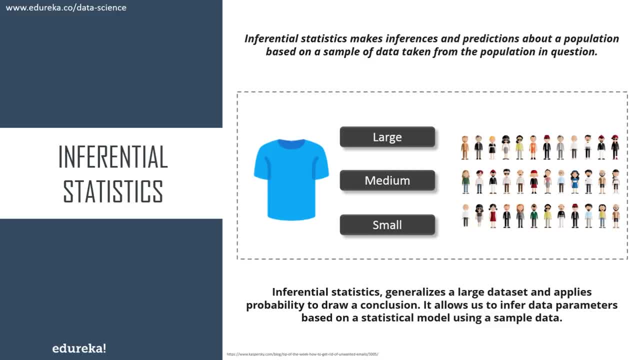 and expand it for the entire population in the class, Because there was a brief understanding of descriptive and inferential statistics. so that's the difference between descriptive and inferential. Now, in the next section, we'll go in-depth about descriptive statistics. all right, 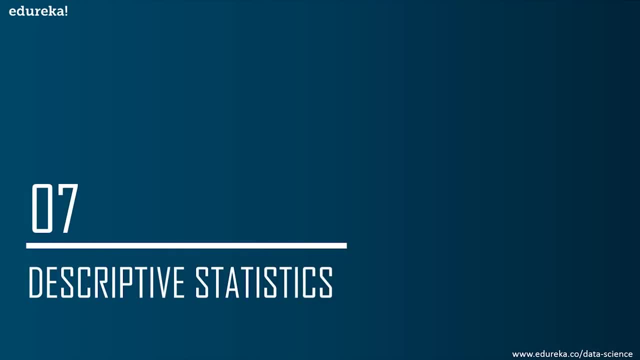 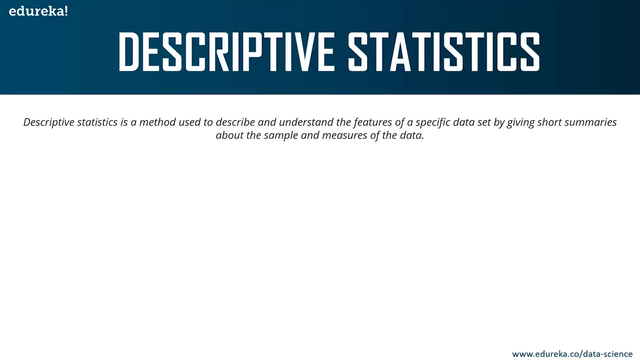 So let's discuss more about descriptive statistics. So, like I mentioned earlier, descriptive statistics is a method that is used to describe and understand the features of a specific data set by giving short summaries about the sample and measures of the data. There are two important measures in descriptive statistics. 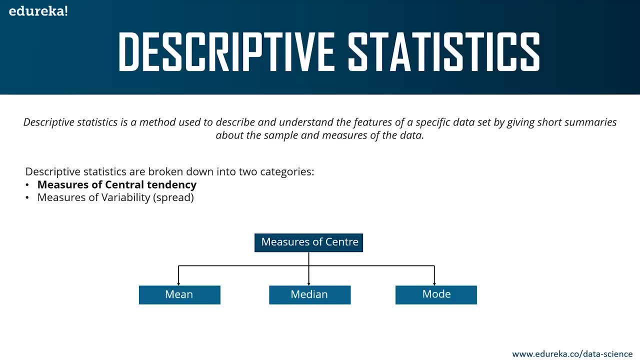 We have measure of central tendency, which is also known as measure of center, and we have measures of variability, This is also known as measures of spread. So measures of center include mean, median and mode. Now, what is measures of center? 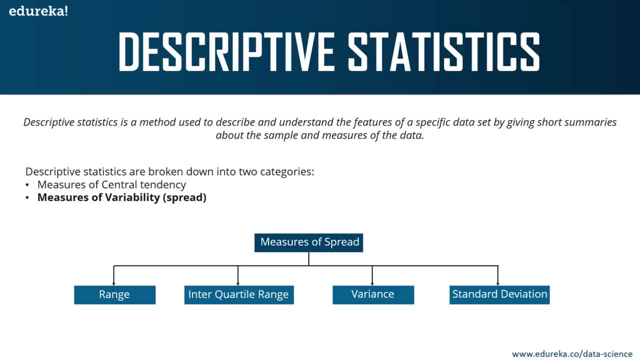 Measures of the center are statistical measures that represent the summary of a data set. Okay, the three main measures of center are mean, median and mode. Okay, the three main measures of center are mean, median and mode, Coming to measures of variability or measures of spread. 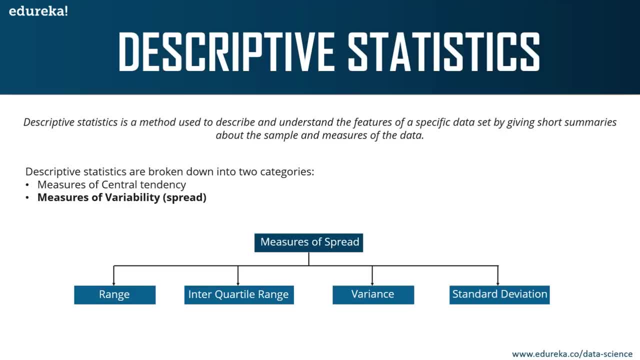 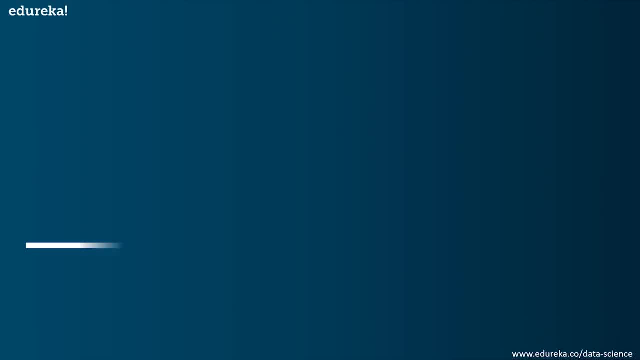 we have range, interquartile range variance and standard deviation- all right. So now let's discuss each of these measures in a little more depth, starting with the measures of center. Now, I'm sure all of you know what the mean is. 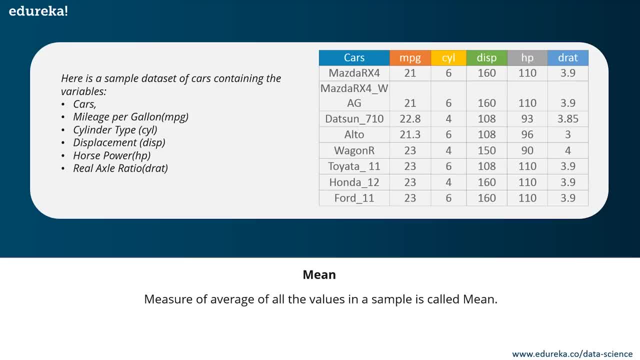 Mean is basically the measure of the average of all the values in a sample. okay, So it's basically the average of all the values in a sample. How do you measure the mean? I hope all of you know how the mean is measured. 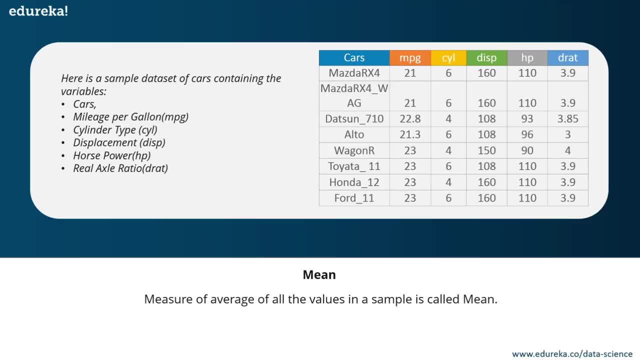 If there are 10 numbers and you wanna find the mean of these 10 numbers, all you have to do is you have to add up all the 10 numbers and you have to divide it by 10.. 10 here represents the number of samples in your data set. 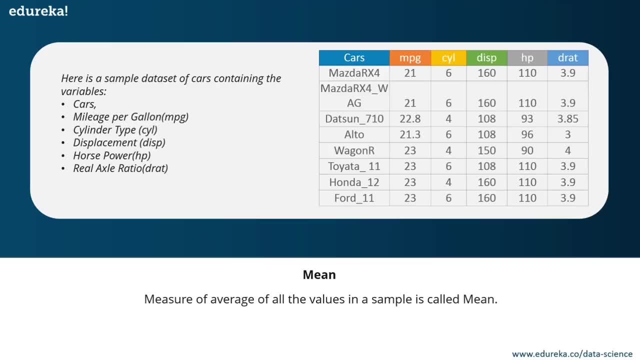 All right, since we have 10 numbers, we're gonna divide this by 10,. all right, This will give us the average or the mean. So to better understand the measures of central tendency, let's look at an example Now. the data set over here is based on the average of all the values in a sample. 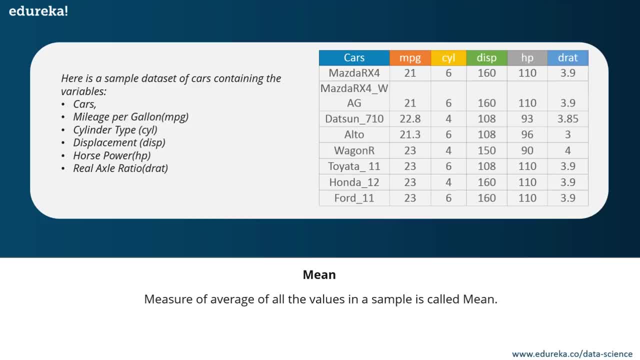 Now, the data set over here is based on the average of all the values in a sample. This is basically the CARS data set, and it contains a few variables. all right, It has something known as CARS. It has mileage per gallon, cylinder type. 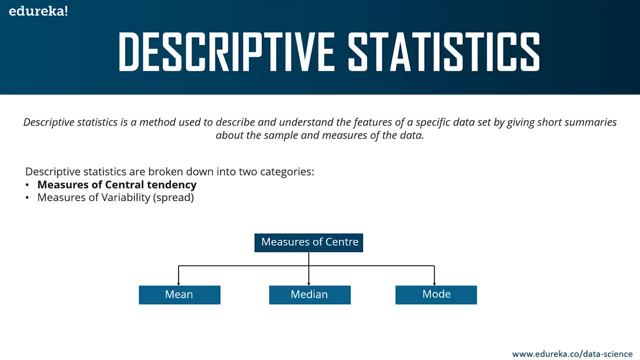 There are two important measures in descriptive statistics. We have measure of central tendency, which is also known as measure of center, and we have measures of variability- This is also known as measures of spread. So measures of center include mean, median and mode. 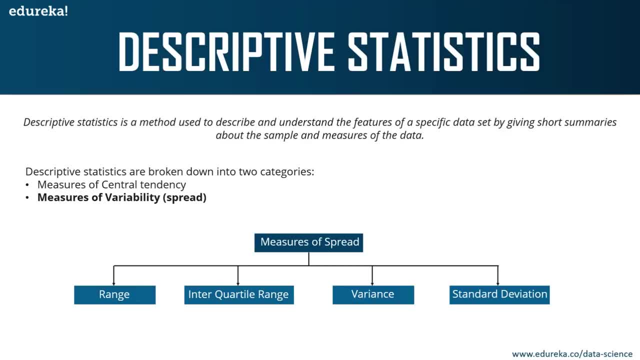 Now, what is measures of center? Measures of the center are statistical measures that represent the summary of a data set. okay, The three main measures of center are mean, median and mode. Coming to measures of variability or measures of spread, we have range, interquartile range. 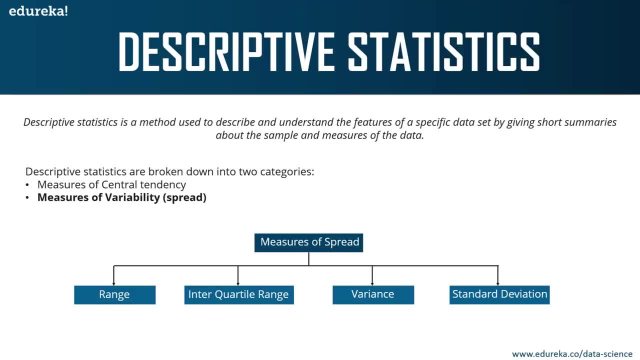 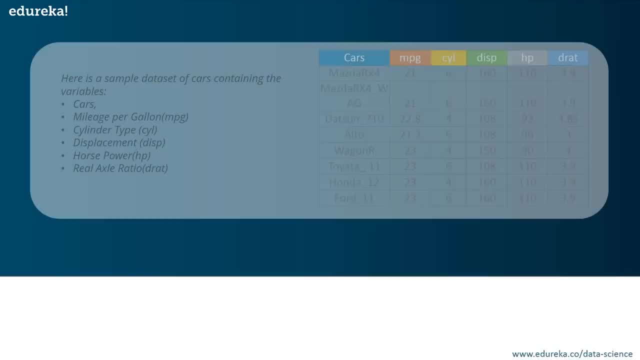 variance and standard deviation. all right, So now let's discuss each of these measures in a little more depth, starting with the measures of center. Now, I'm sure all of you know what the mean is. Mean is basically the measure of the average. 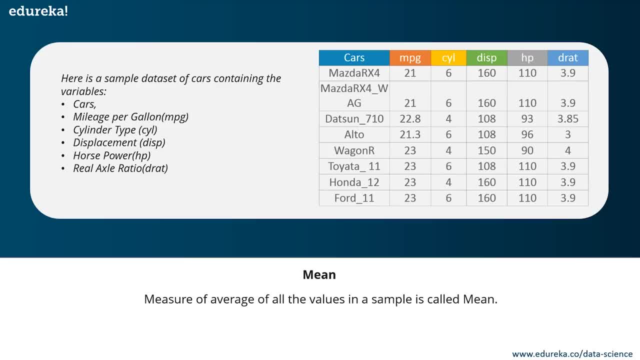 of all the values in a sample. okay, So it's basically the average of all the values in a sample. How do you measure? How do you measure the mean? I hope all of you know how the mean is measured. If there are 10 numbers and you want to find the mean, 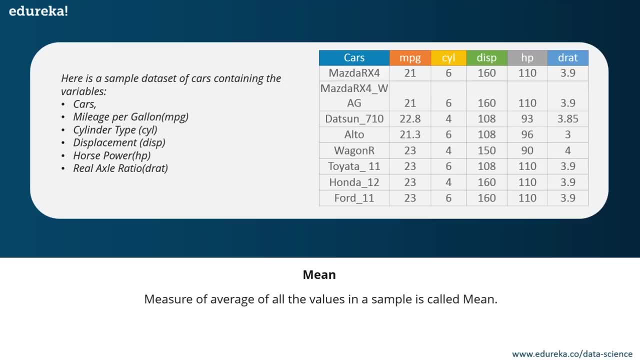 of these 10 numbers. all you have to do is you have to add up all the 10 numbers and you have to divide it by 10.. 10 here represents the number of samples in your data set. All right, since we have 10 numbers. 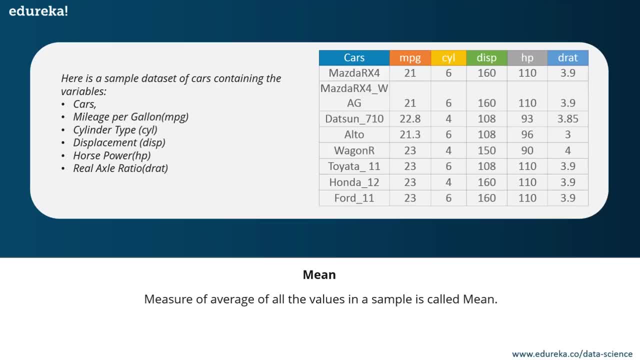 we're gonna divide this by 10,. all right, This will give us the average or the mean. So to better understand the measures of central tendency, let's look at an example Now. the data set over here is basically the CARS data set. 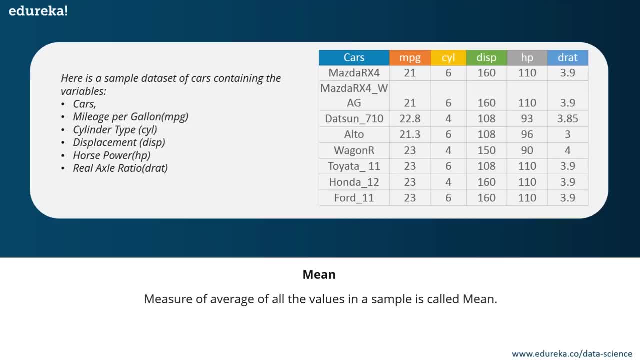 and it contains a few variables, all right. It has something known as CARS. It has mileage per gallon, cylinder type, displacement, horsepower and real axle ratio. all right, All of these measures are related to CARS, okay. 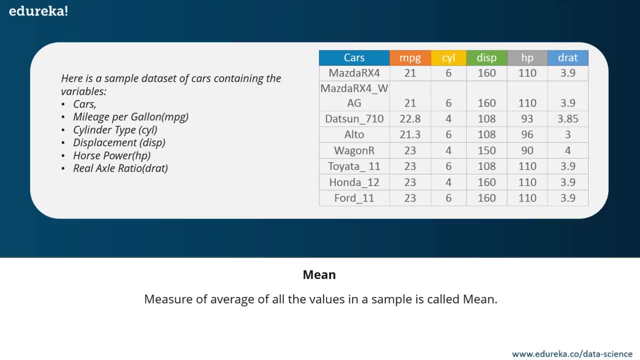 So what you're gonna do is you're going to use descriptive analysis and you're going to analyze each of the variables in the sample data set for the mean, standard deviation, median and so on. So let's say that you want to find out the mean. 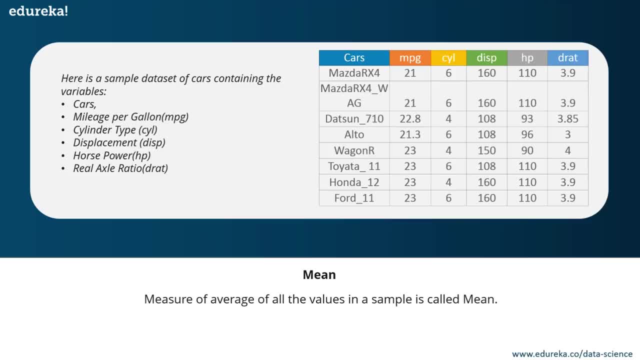 displacement, horsepower and real axle ratio. all right, All of these measures are related to CARS. okay, So what you're gonna do is you're going to use descriptive analysis and you're going to analyze each of the variables in the sample data set. 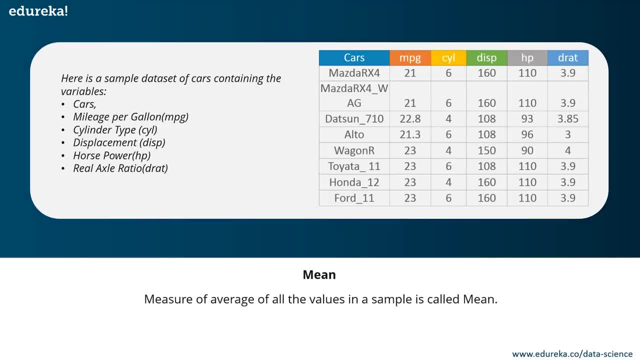 for the mean standard deviation, median, more and so on. So let's say that you want to find out the mean or the average horsepower of the cars among the population of cars, Like I mentioned earlier, what you'll do is: 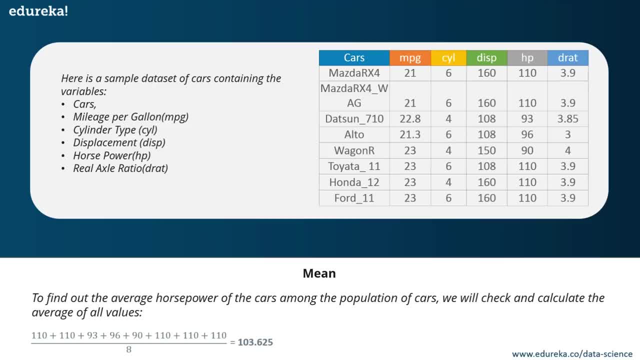 you'll check the average of all the values. So in this case we'll take the sum of the horsepower of each car and we'll divide that by the total number of cars. okay, That's exactly what I've done here in the calculation part. 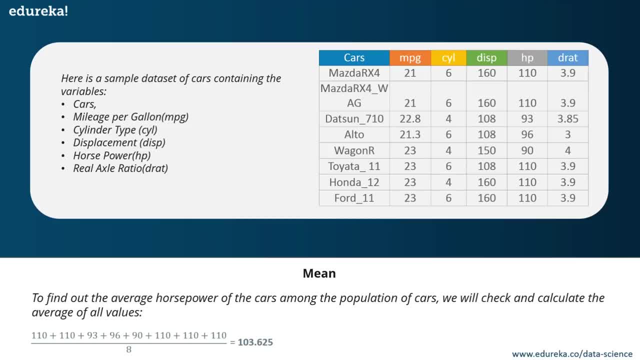 So this 110 basically represents the horsepower for the first car, all right. Similarly, I've just added up all the values of horsepower for each of the cars and I've divided it by eight. Now, eight is basically the number of cars in our data set. 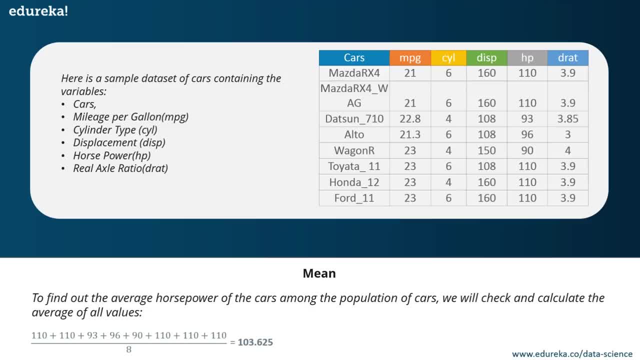 All right. so 103.625 is what our mean is, or the average of horsepower is all right. Now let's understand what median is with an example. okay, So to define median: median is basically a measure of the central value of the sample set. 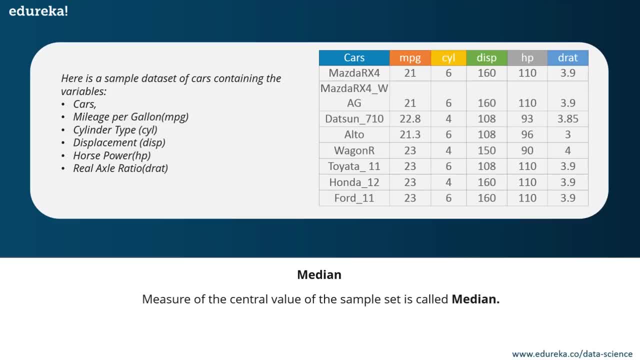 is called the median. all right, You can see that it is the middle value. So if you want to find out the center value of the mileage per gallon among the population of cars first, what we'll do is we'll arrange the mpg values. 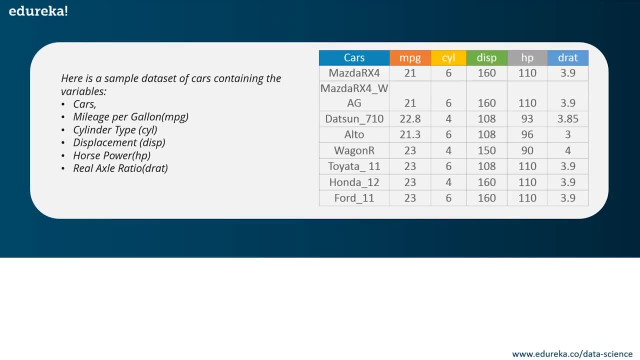 in ascending or descending order and choose a middle value. all right In this case, since we have eight values. right, We have eight values, which is an even entry. So whenever you have even number of data points or samples in your data set, then you're going to take the 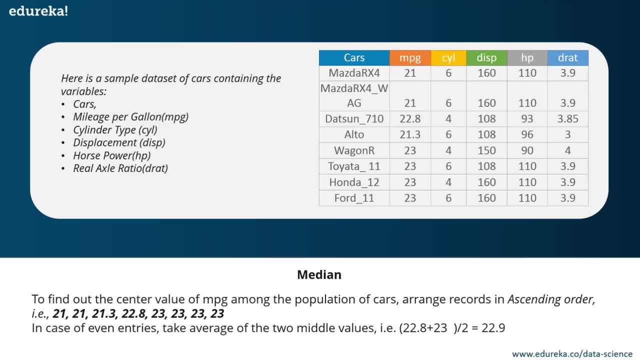 average of the two middle values. If we had nine values over here, we can easily figure out the middle value and, you know, choose that as a median. But since there are even number of values, we're going to take the average of the two middle values. 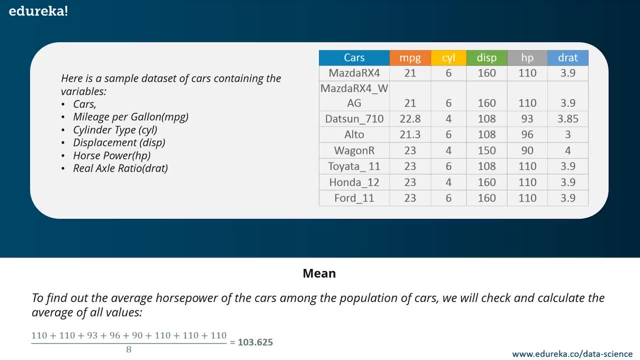 or the average horsepower of the cars among the population of cars. Like I mentioned earlier, what you'll do is you'll check the average of all the values. So in this case, we'll take the sum of the horsepower of each car and we'll divide that. 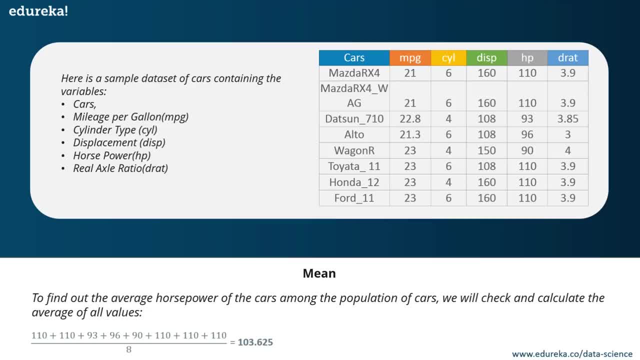 by the total number of cars. okay, That's exactly what I've done here in the calculation part. So this 110 basically represents the horsepower for the first car. all right, I've just added up all the values of horsepower for each of the cars and I've divided it by eight. 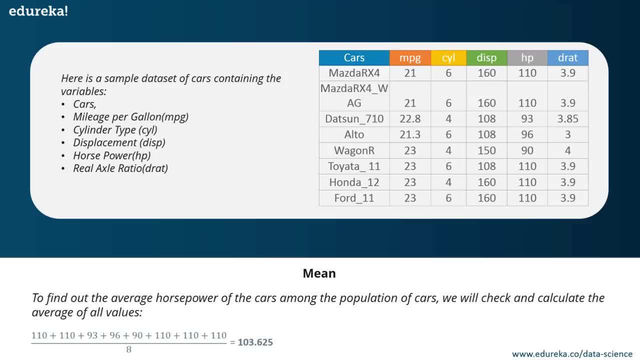 Now, eight is basically the number of cars in our data set. All right, so 103.625 is what our mean is, or the average of horsepower is all right. Now let's understand what median is with an example. okay, So to define median. median is basically a measure. 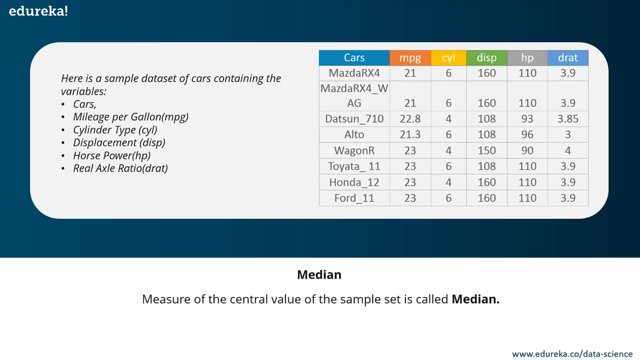 of the central value of the sample set is called the median. all right, You can see that it is a middle value. So if you want to find out the center value of the mileage per gallon among the population of cars first, what we'll do is we'll arrange the MPG values. 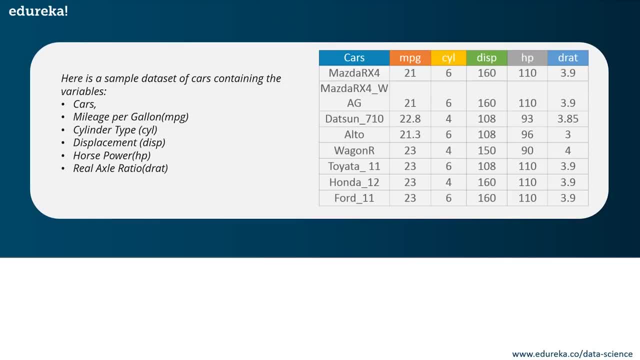 in ascending or descending order and choose a middle value. all right In this case, since we have eight values. right, We have eight values, which is an even entry. So whenever you have even number of data points or samples in your data set, then you're going. 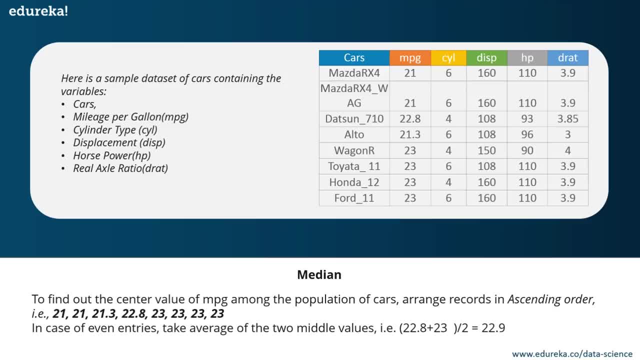 to take the average of the two middle values. If we had nine values over here, we can easily figure out the middle value and, you know, choose that as a median. But since there are even number of values, we're going to take the average of the two middle values. 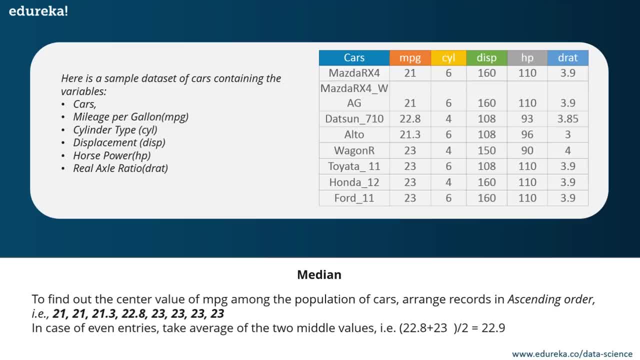 all right. So 22.8 and 23 are my two middle values and I'm taking the mean of those two and hence I get 22.9, which is my median, all right. Lastly, let's look at how mode is calculated. 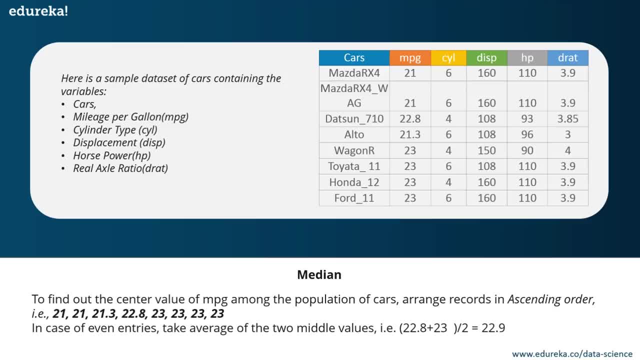 all right. So 22.8 and 23 are my two middle values and I'm taking the mean of those two and hence I get 22.9, which is my median, all right. Lastly, let's look at how mode is calculated. 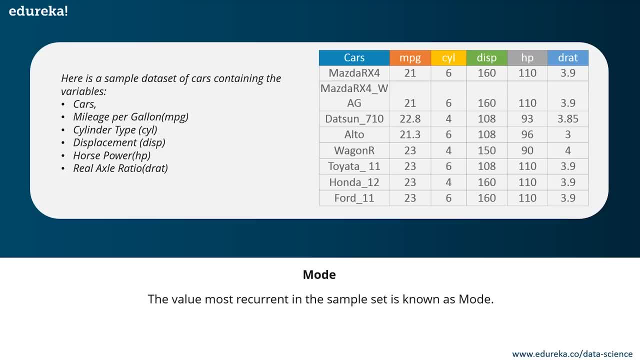 So what is mode? Now, the value that is most recurrent in the sample set is known as mode, Or basically, the value that occurs most often. okay, That is known as mode. So let's say that we want to find out the most common type of cylinder. 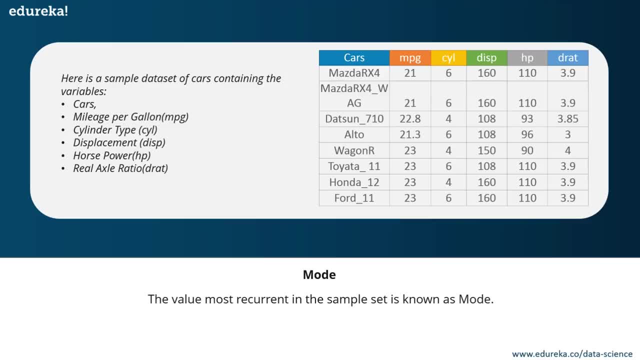 among the population of cars. What we have to do is we will check the value which is repeated the most number of times. Here we can see that the cylinders come in two types. We have cylinder of type four and cylinder of type six. right. 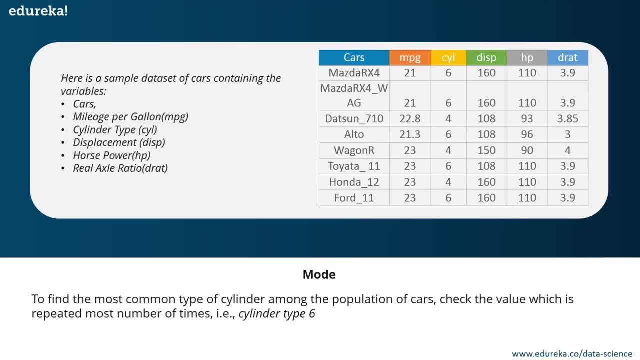 So take a look at the data set. You can see that the most recurrent type of cylinder is six, right. We have one, two, three, four and five. We have five, six and we have one, two, three. 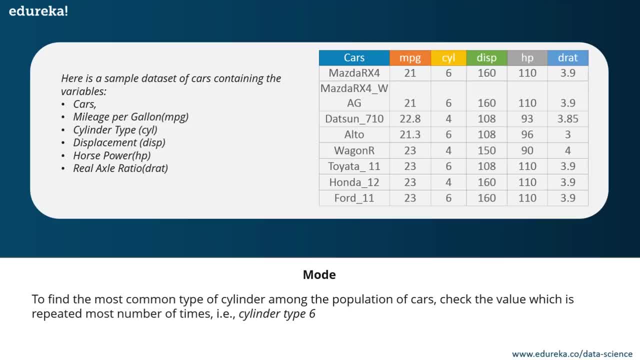 Yeah, we have three- four type cylinders and five- six type cylinders. So basically, we have three- four type cylinders and we have five- six type cylinders. all right, So our mode is going to be six, since six is more recurrent than four. 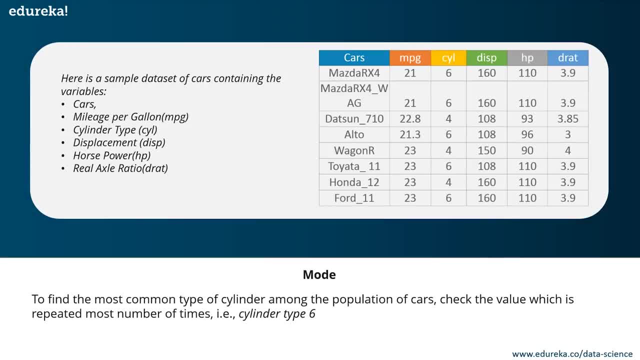 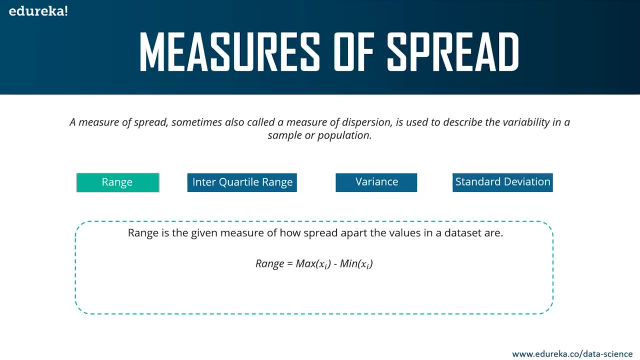 So, guys, those were the measures of the center, or the measures of central tendency. Now let's move on and look at the measures of the spread. All right, Now. what is the measure of spread? A measure of spread sometimes also called 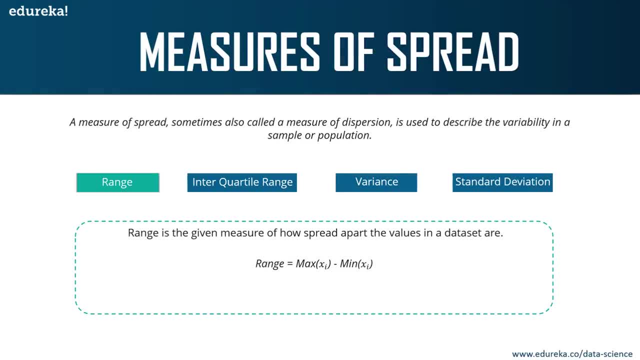 as measure of dispersion is used to describe the variability in a sample or population. Okay, you can think of it as some sort of deviation in the sample, all right, So you measure this with the help of the different measure of spreads. We have range interquartile range variance. 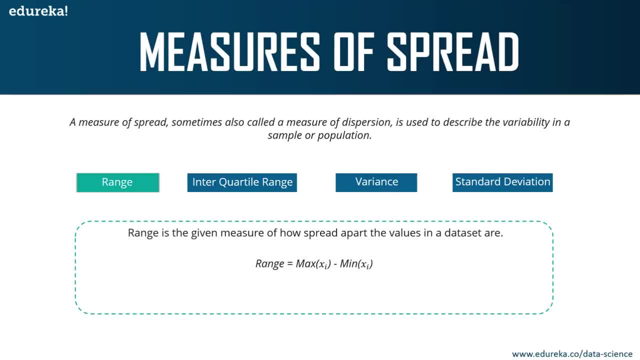 and standard deviation. Now, range is pretty self-explanatory, right. It is the given measure of how, spread apart, the values in a data set are. The range can be calculated as shown in this formula. So you're basically going to subtract the maximum value. 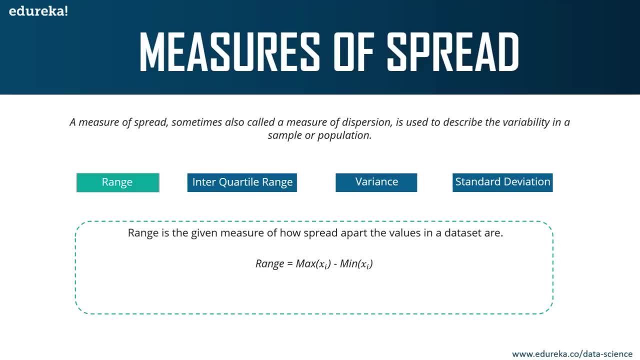 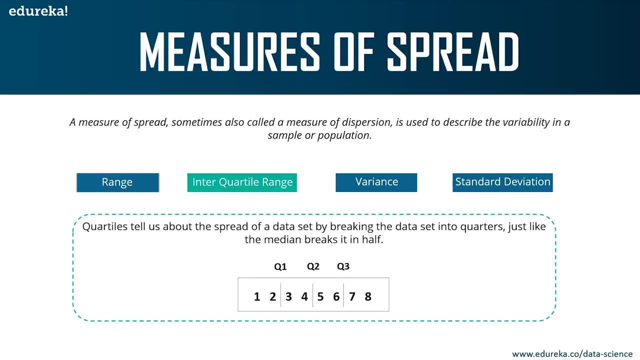 in your data set from the minimum value in your data set. That's how you calculate the range of the data. all right. Next we have interquartile range. So before we discuss interquartile range, let's understand what a quartile is. 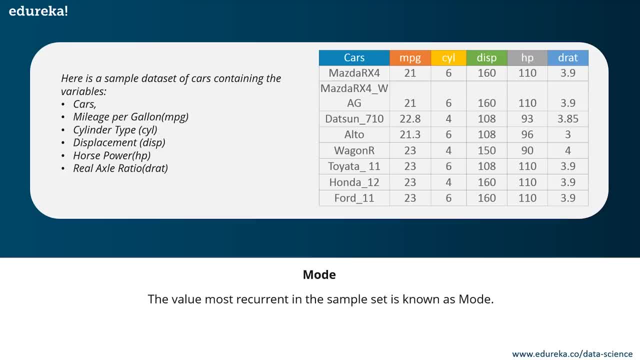 So what is mode? Now, the value that is recurrent in the sample set is known as mode, or basically, the value that occurs most often. okay, That is known as mode. So let's say that we want to find out the most common type of cylinder. 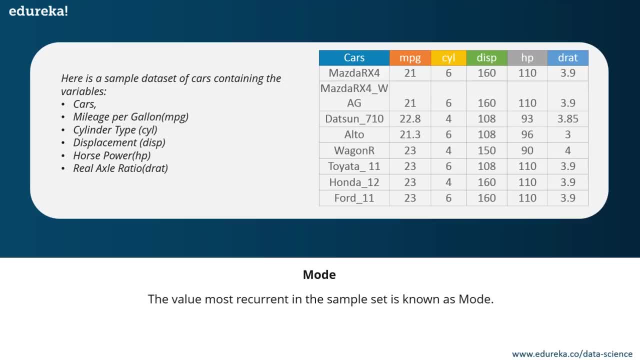 among the population of cars. What we have to do is we will check the value which is repeated the most number of times. Here we can see that the cylinders come in two types. We have cylinder of type four and cylinder of type six. right. 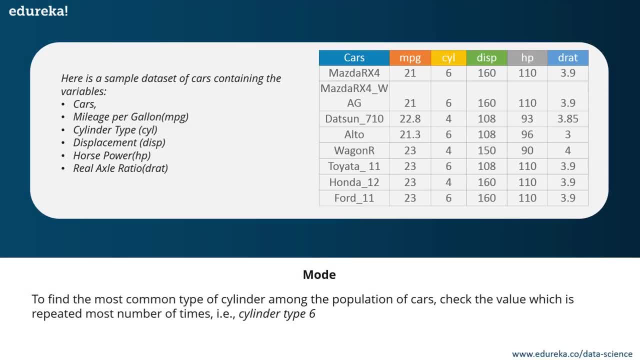 So take a look at the data set. You can see that the most recurrent value is six. right, We have one, two, three, four and five. We have five, six. and we have one, two, three. Yeah, we have three, four. type cylinders. 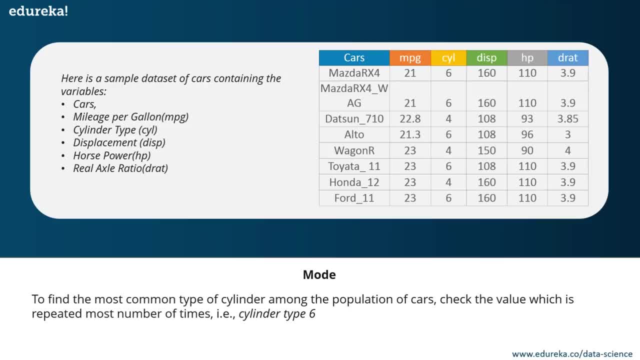 and five six type cylinders. So, basically, we have three four type cylinders and we have five six type cylinders. all right, So our mode is going to be six, Since six is more recurrent than four. So, guys, those were the measures of the center. 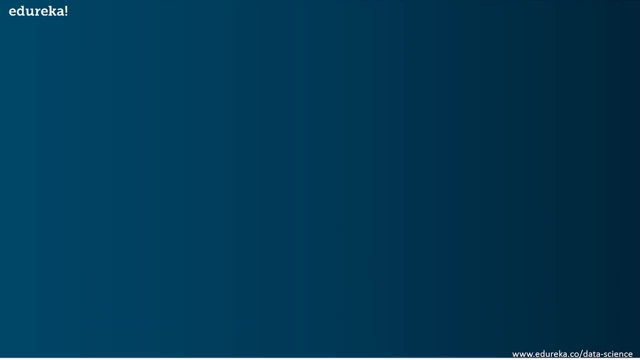 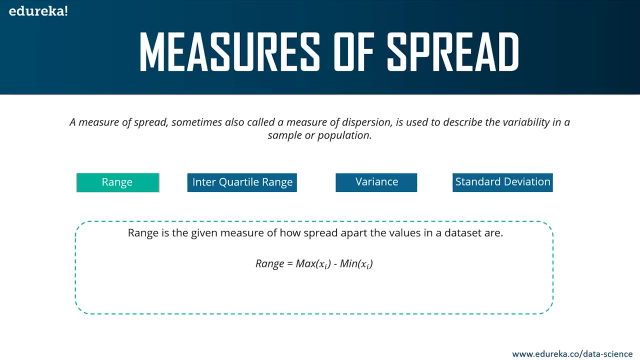 or the measures of central tendency. now let's move on and look at the measures of the spread. all right now, what is the measure of spread? a measure of spread, sometimes also called as measure of dispersion, is used to describe the variability in a sample or population. okay, you can. 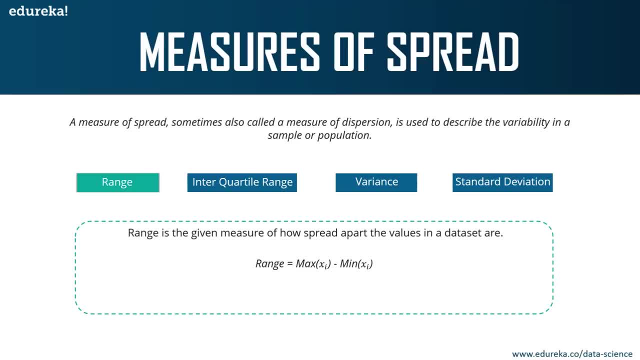 think of it as some sort of deviation in the sample. all right, so you measure this with the help of the different measure of spreads. we have range, interquartile range, variance and standard deviation. now, range is pretty self-explanatory, right. it is the given measure of how spread. 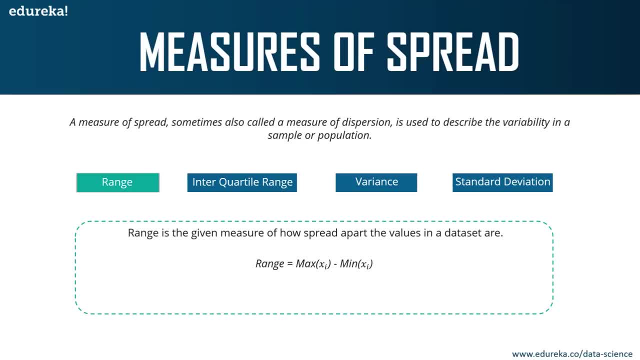 apart. the values in a data set are the range can be calculated as shown in this formula. so you're basically going to subtract the maximum value in your data set from the minimum value in your data set. that's how you calculate the range of the data. all right, 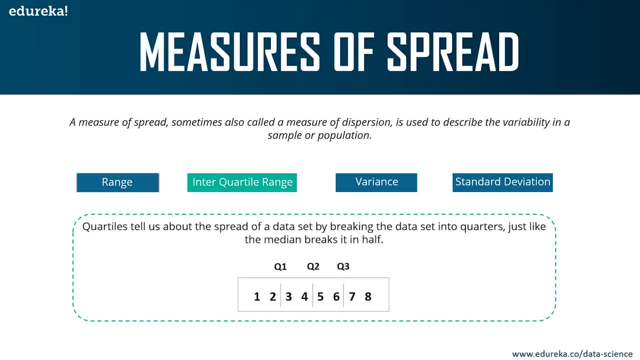 next we have interquartile range. so before we discuss interquartile range, let's understand what a quartile is. all right. so quartiles basically tell us about the spread of a data set by breaking the data set into different quarters. okay, just like how the median breaks the data into two parts. 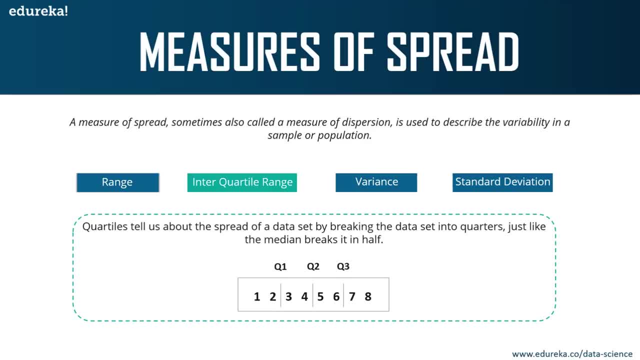 All right. so quartiles basically tell us about the spread of a data set by breaking the data set into different quartiles. Okay, just like how the median breaks the data into two parts, the quartile will break it into different quartiles. 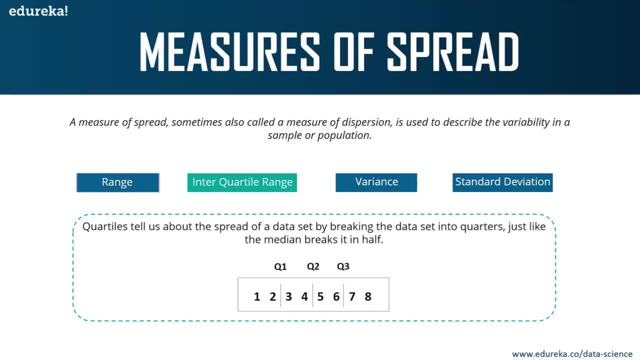 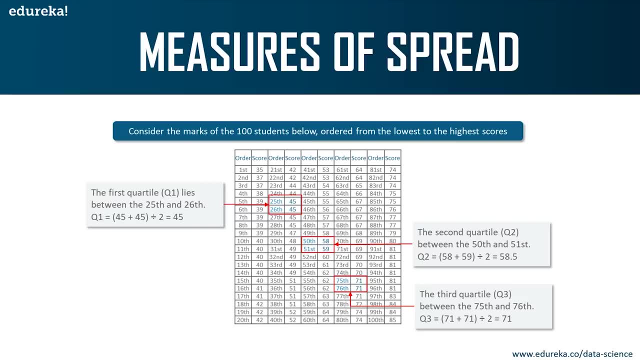 So to better understand how quartile and interquartile are calculated, let's look at a small example Now. this data set basically represents the marks of 100 students. Let's start from the lowest to the highest scores. All right, so the quartiles lie in the following ranges: 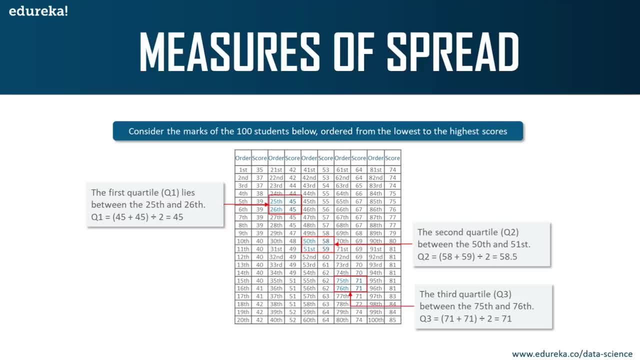 Now the first quartile, which is also known as Q1,. it lies between the 25th and the 26th observation. All right, so if you look at this, I've highlighted the 25th and the 26th observation. 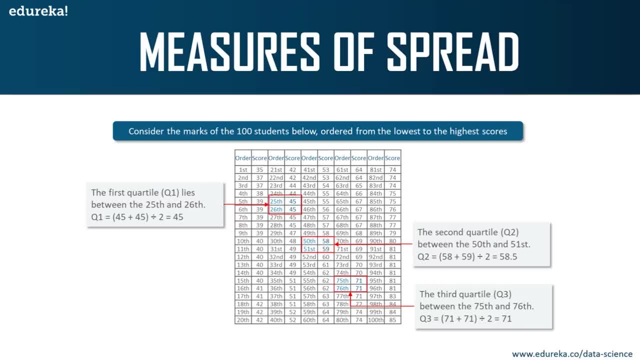 So how you can calculate Q1, or first quartile, is by taking the average of these two values. all right, Since both the values are 45, when you add them up and divide them by two, you'll still get 45.. 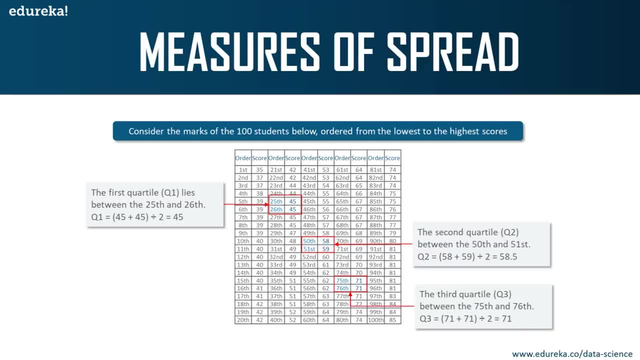 Now the second quartile, or Q2, is between the 50th and the 51st observation. So you're going to take the average of 58 and 59, and you'll get a value of 58.5.. Now this is my second quarter. 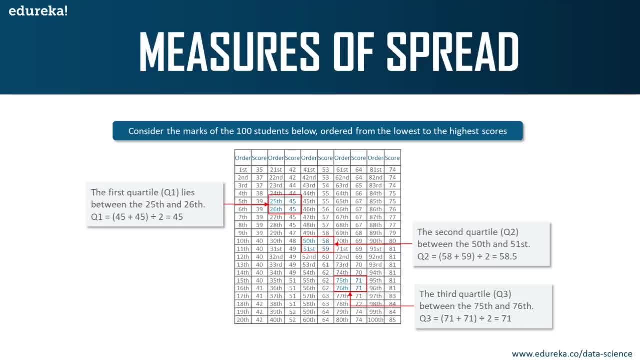 The third quartile, or Q3, is between the 75th and the 76th observation. Here again, you'll take the average of the two values, which is the 75th value and the 76th value. all right. 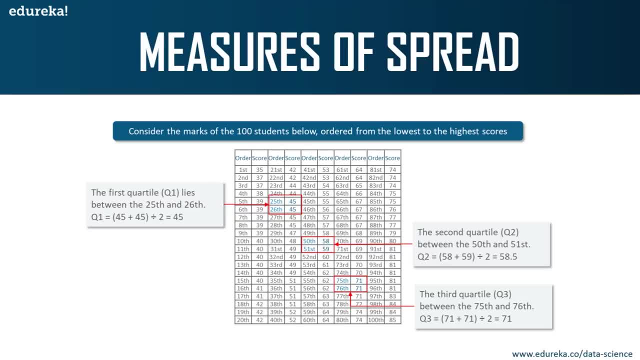 And you'll get a value of 71,. all right, So, guys, this is the first quartile or Q2, is between the 75th and the 76th observation. All right, So, guys, this is the first quartile or Q3,. 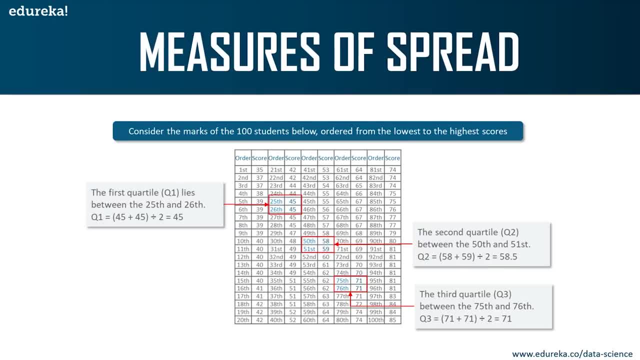 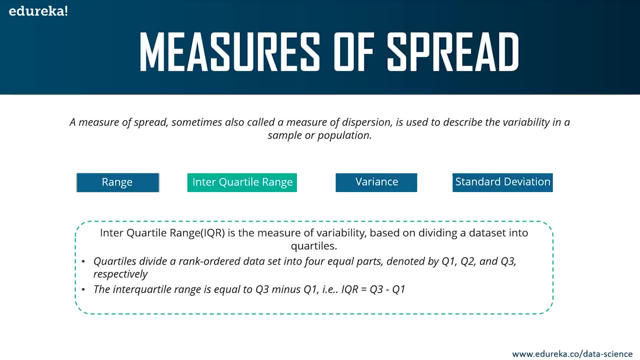 is between the 75th and the 76th observation. This is exactly how you calculate the different quartiles. Now let's look at what is interquartile range. So IQR, or the interquartile range, is a measure of variability based on. 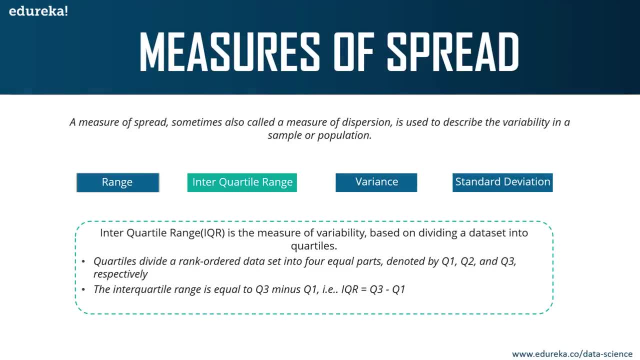 dividing a data set into quartiles. Now the interquartile range is calculated by subtracting the Q1 from Q3.. So basically, Q3 minus Q1 is your IQR. So your IQR is your Q3 minus Q1,. all right. 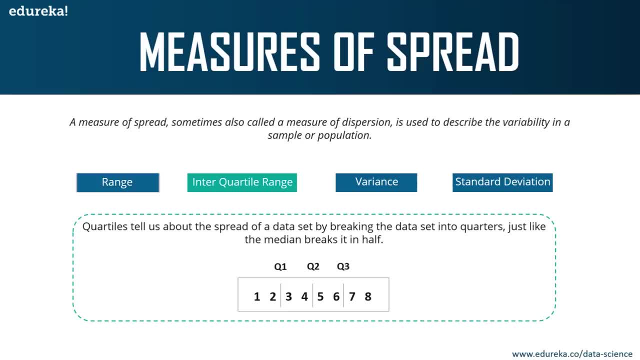 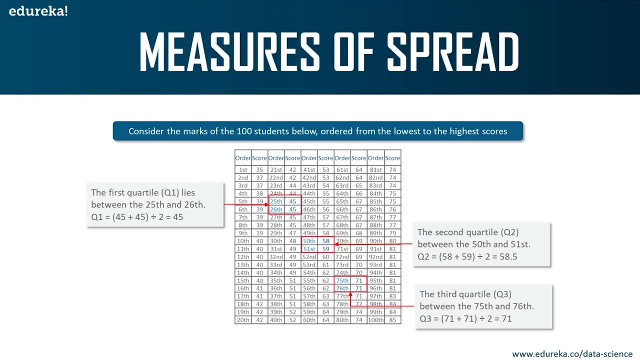 the quartile will break it into different quarters. so to better understand how quartile and interquartile are calculated, let's look at a small example now. uh, this data set basically represents the marks of 100 students, ordered from the lowest to the highest scores. all right, so the quartiles lie in the following ranges: now the first quartile, which 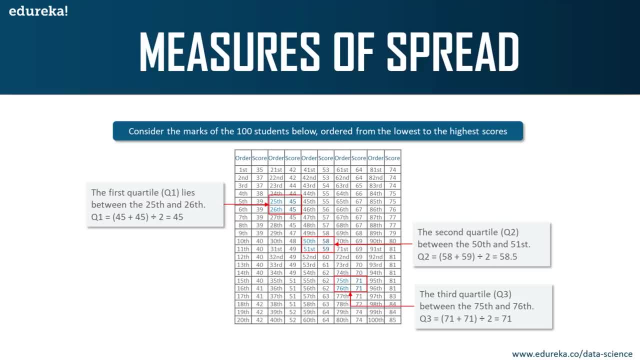 is also known as q1. it lies between the 25th and the 26th observation, all right. so, if you look at this, i've highlighted the 25th and the 26th observation. so how you can calculate q1, or first quartile, is by taking the average of these two values. all right, since both the 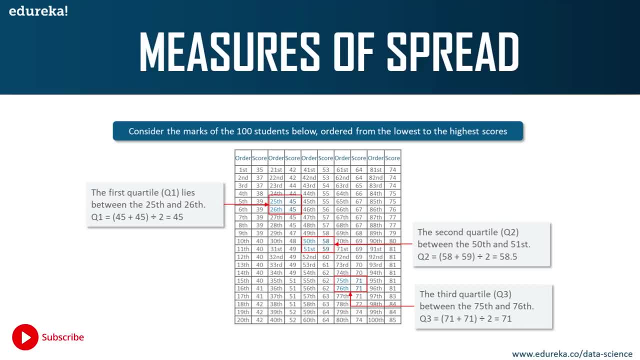 values are 45. when you add them up and divide them by 2, you'll still get 45.. now the second quartile, or q2, is between the 50th and the 51st observation. so you're going to take the average of 58 and 59 and you'll get a value of 58.5. now this is my second quarter. the third quartile, or q3, 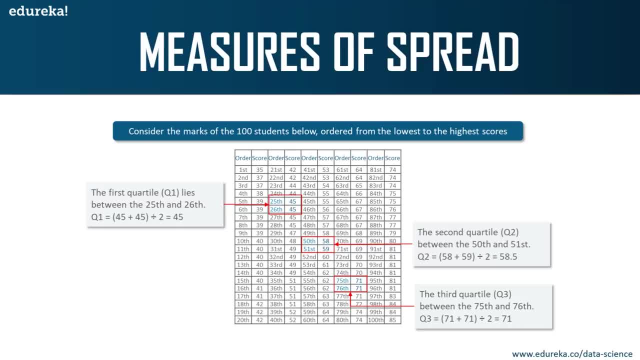 is between the 75th and the 76th observation. here again, you'll take the average of the two values, which is the 75th value and the 76th value, all right, and you'll get a value of 71, all right. so, guys, this is exactly how you. 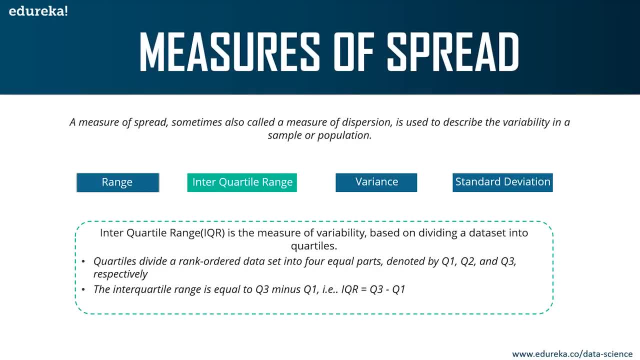 calculate the different quartiles. now let's look at what is interquartile range. so iqr, or the interquartile range, is a measure of variability based on dividing a data set into quartiles. now the interquartile range is calculated by subtracting the q1 from q3, so basically, q3-q1 is your iqr. 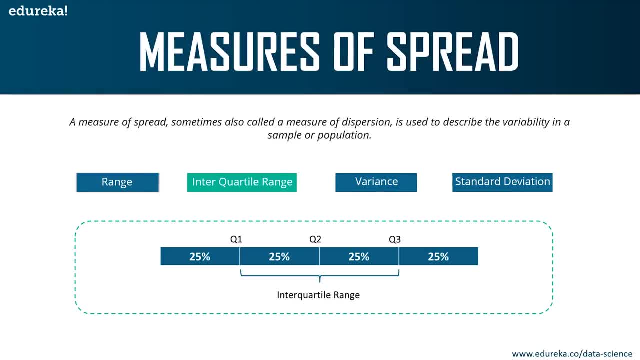 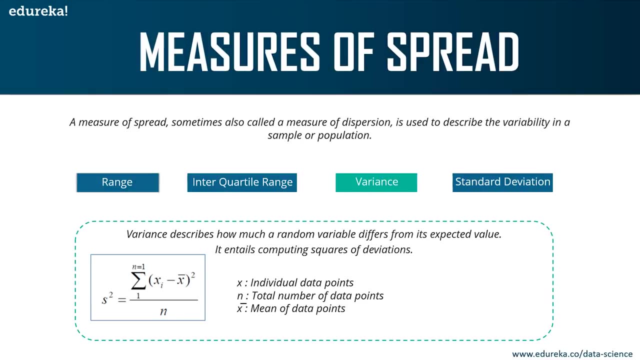 so your iqr is your q3-q1. all right, now. this is how each of the quartiles are. each quartile represents a quarter, which is 25 percent. all right. so, guys, i hope all of you are clear with interquartile range and what are quartiles. now let's look at variance. now. variance is basically: 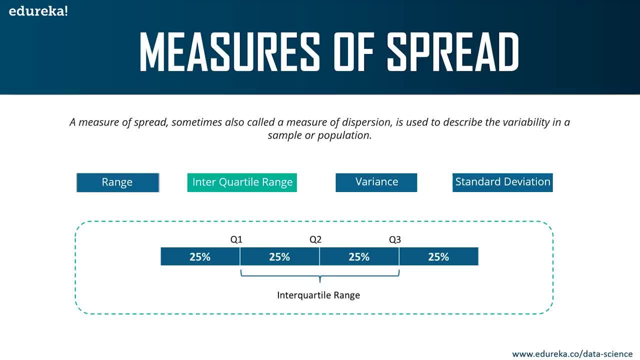 Now this is how each of the quartiles are. each quartile represents a quarter, which is 25%, All right, So, guys, I hope all of you are clear with interquartile range and what are quartiles. Now let's look at variance. 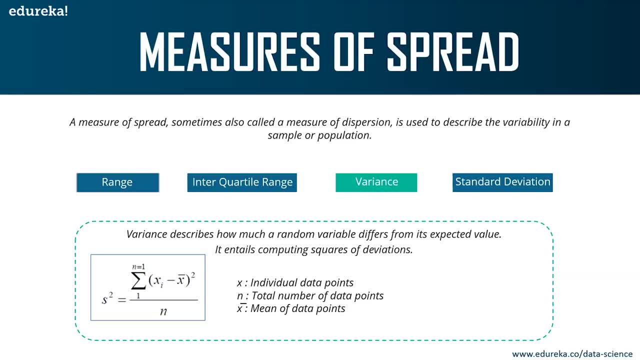 Now, variance is basically a measure that shows how much a random variable differs from its expected value. Okay, it's basically the variance in any variable. Now variance can be calculated by using this formula. All right here. X basically represents any data point in your data set. 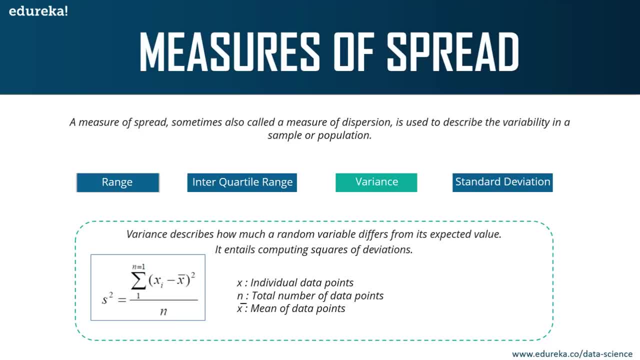 N is the total number of data points in your data set and X bar is basically the mean of data points. All right, This is how you calculate variance. Variance is basically computing the squares of deviations. Okay, that's why it says S squared there. 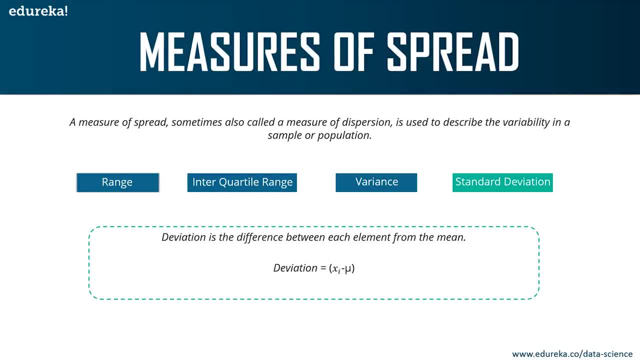 Now let's look at what is deviation. Deviation is just the difference between each element from the mean. Okay, so it can be calculated by using this simple formula, where Xi basically represents a data point and mu is the mean of the population. 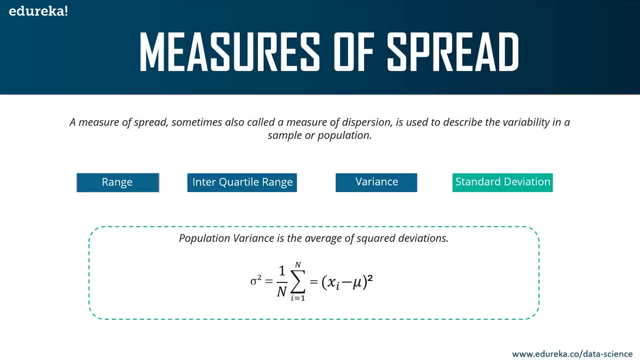 All right, this is exactly how you calculate deviation. Now, population variance and sample variance are very specific to whether you're calculating the variance in your population data set or in your sample data set. That's the only difference between population and sample variance, So the formula for population variance is pretty explanatory. 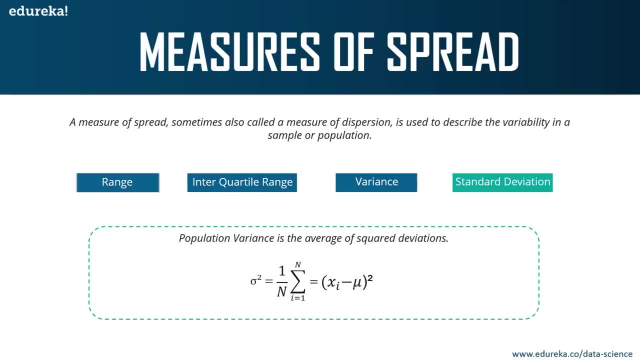 So Xi is basically each data point, Mu is the mean of the population, N is the number of samples in your data set. All right, Now let's look at sample variance. Now, sample variance is the average of square differences from the mean. 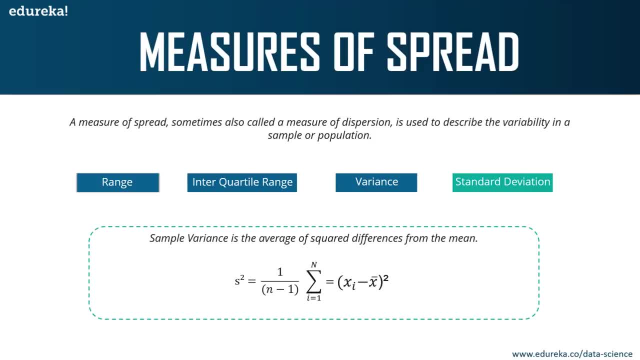 All right, Here Xi is any data point or any sample in your data set. X bar is the mean of your sample. All right, it's not the mean of your population, It's the mean of your sample. And if you notice N, here is a smaller N. 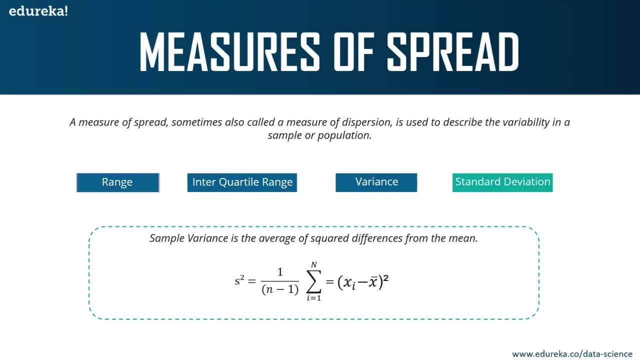 It's the number of data points in your sample And this is basically the difference between sample and population variance. I hope that is clear. Coming to standard deviation is the measure of dispersion of a set of data from its mean. All right, So it's basically the deviation from your mean. 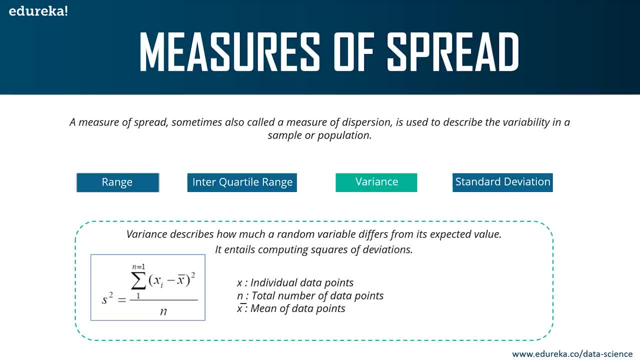 a measure that shows how much a random variable differs from its expected value. okay, it's basically the variance in any variable. now, variance can be calculated by using this one formula right here. x basically represents any data point in your data set, n is the total number of data points in your data set and x bar is basically the mean of data points. all right, 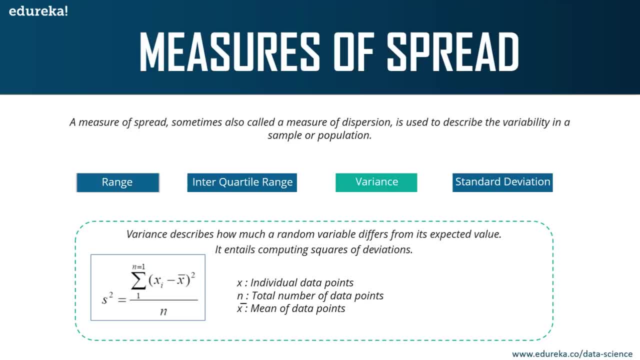 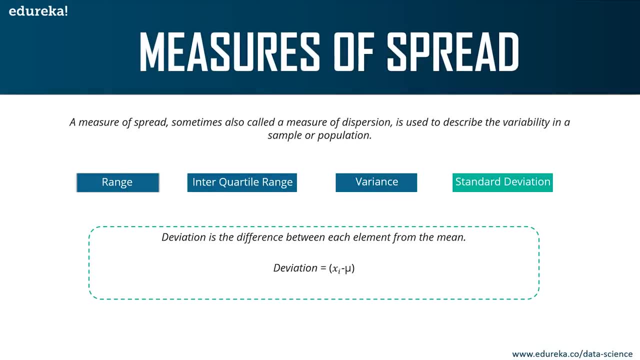 this is how you calculate variance. variance is basically, uh, computing the squares of deviations. okay, that's why it says s squared there. now let's look at what is deviation. deviation is just the difference between each element from the mean. okay, so it can be calculated by using. 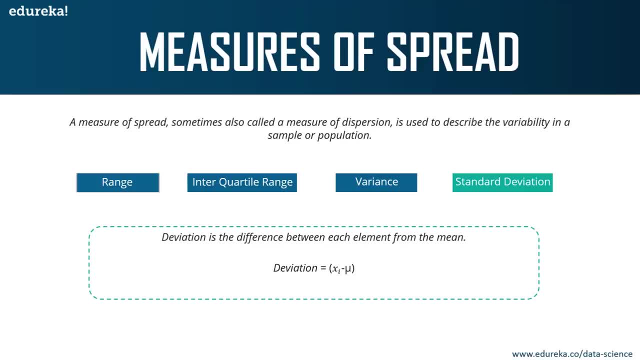 this simple formula, where x- i basically represents a data point and mu is the mean of the population. all right, this is exactly how you calculate deviation. now, population variance and sample variance are very specific to whether you're calculating the variance in your population data set or in your sample data set. that's the only difference between. 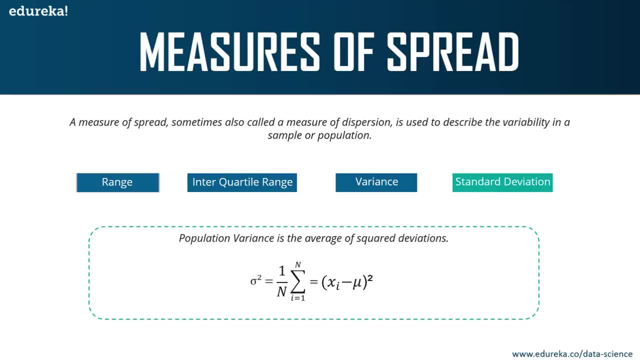 population and sample variance. so the formula for population variance is pretty explanatory. so xi is basically each data point, mu is the mean probability that the population var. the case where the variance is calculated for population- and while pilot is Essex, this might mean of the population, n is the number of samples. 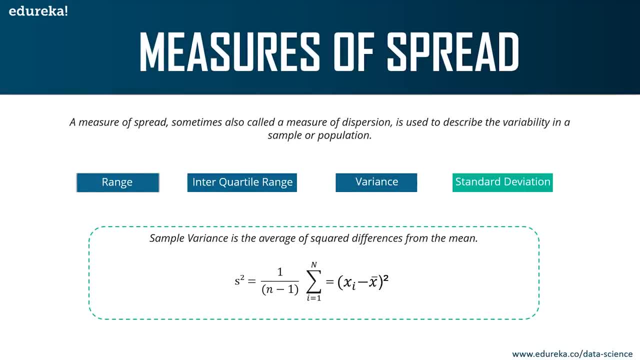 in your data set. all right. Now let's look at sample variance. Now, sample variance is the average of squared differences from the mean. all right. Here xi is any data point or any sample in your data set. X bar is the mean of your sample. all right. 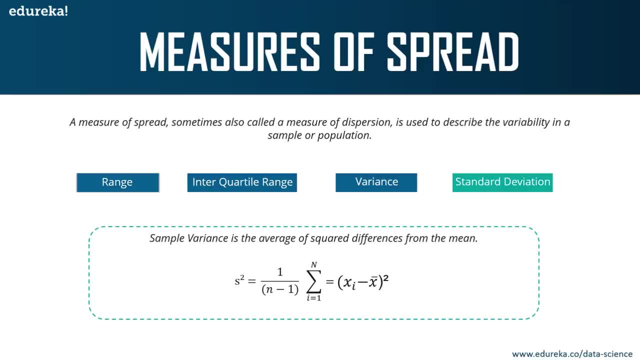 It's not the mean of your population, It's the mean of your sample And if you notice n, here is a smaller n, it's the number of data points in your sample And this is basically the difference between sample and population variance. 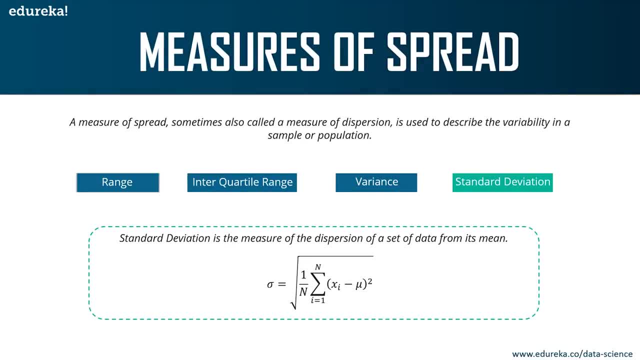 I hope that is clear. Coming to standard deviation is the measure of dispersion of a set of data from its mean. all right, So it's basically the deviation from your mean. That's what standard deviation is. Now to better understand how the measures of spread. 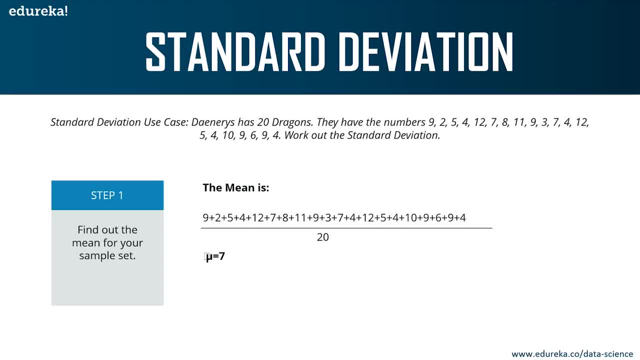 are calculated. let's look at a small use case. So let's say Daenerys has 20 dragons. They have the numbers nine, two, five, four and so on, as shown on the screen. What you have to do is you have to work out. 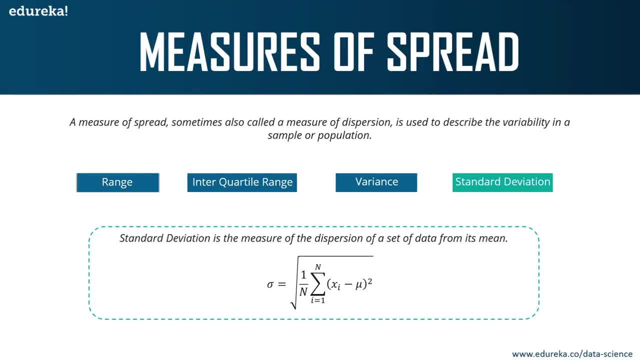 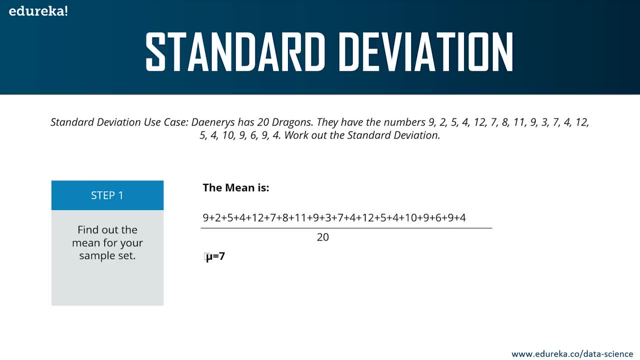 That's what standard deviation is. Now, to better understand how the measures of spread are calculated, let's look at a small use case. So let's say Daenerys has 20 dragons. They have the numbers nine, two, five, four and so on. 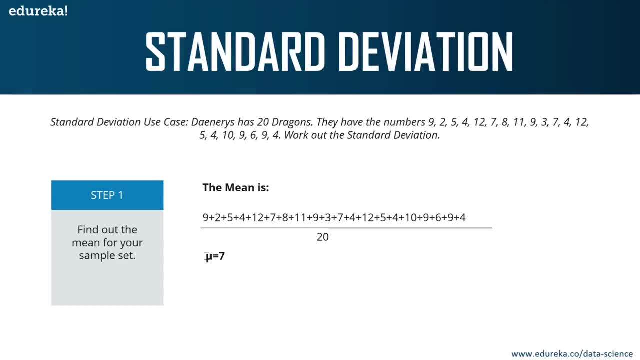 as shown on the screen. What you have to do is you have to work out the standard deviation. All right, in order to calculate the standard deviation, you need to know the mean right. So first you're gonna find out the mean of your sample set. 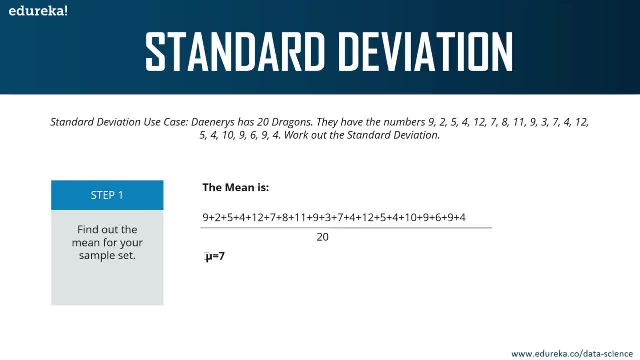 So how do you calculate the mean? You add all the numbers in your data set and divide it by the total number of samples in your data set. So you get a value of seven here. Then you calculate the RHS of your standard deviation formula. 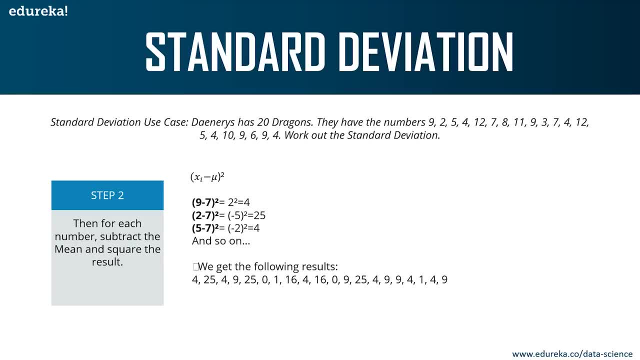 All right. so from each data point you're going to subtract the mean and you're going to square that. All right, so when you do that, you'll get the following result: You'll basically get this: 425,, 4925, and so on. 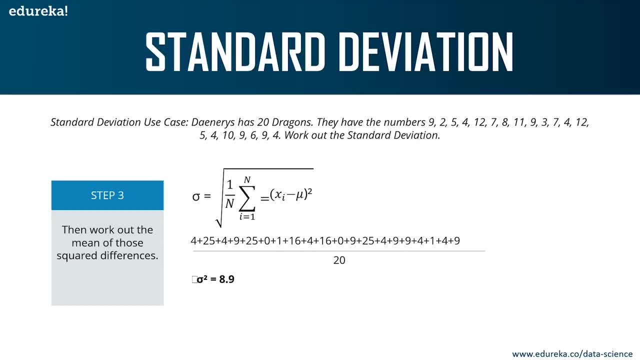 So, finally, you'll just find the mean of these squared differences, all right. So your standard deviation will come up to 2.983 once you take the square root. So, guys, this is pretty simple. It's a simple mathematic technique. 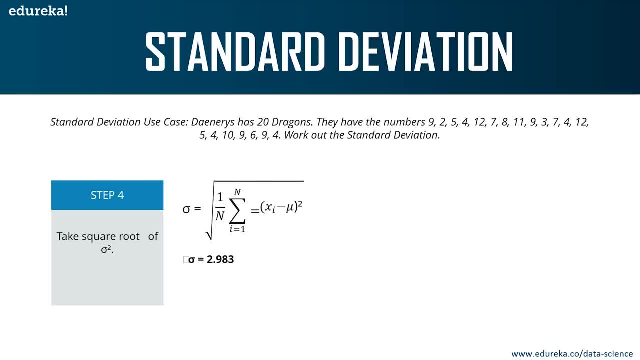 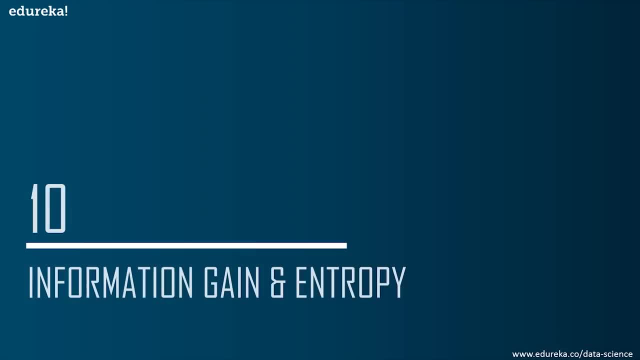 All you have to do is you have to substitute the values in the formula. all right, I hope this was clear to all of you. Now let's move on and discuss the next topic, which is information Gain and entropy. Now, this is one of my favorite topics in statistics. 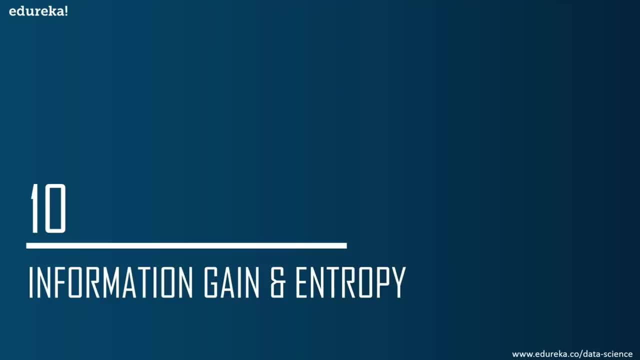 It's very interesting, And this topic is mainly involved in machine learning algorithms like decision trees and random forest. all right, It's very important for you to know how information gain and entropy really work and why they're so essential in building machine learning models. 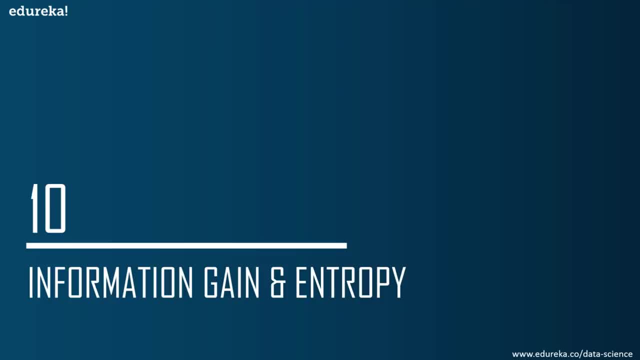 We'll focus on the statistic parts of information gain and entropy, And after that we'll discuss a use case and see how information gain and entropy is used in this. So for those of you who don't know what a decision tree is, it is basically a machine learning algorithm. 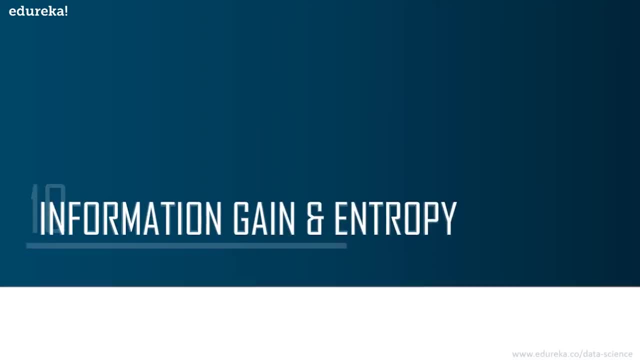 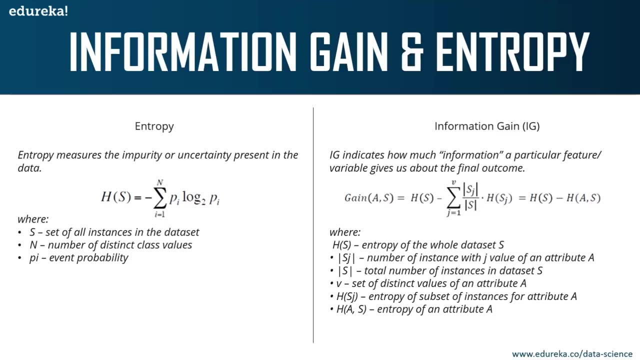 You don't have to know anything about this. I'll explain everything in depth, so don't worry. Now let's look at what exactly entropy and information gain is. Now, guys, entropy is basically the measure of any sort of uncertainty that is present in the data. 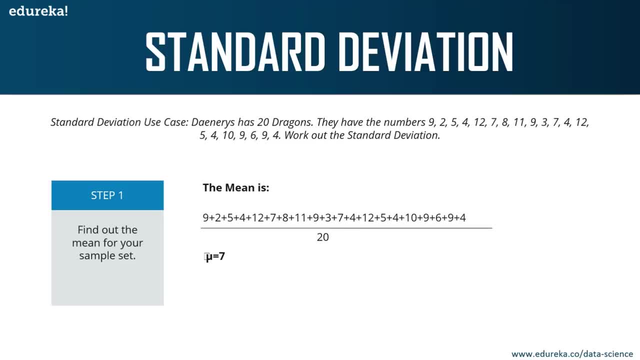 the standard deviation. all right, In order to calculate the standard deviation you need to know the mean, right? So first you're gonna find out the mean of your sample set. So how do you calculate the mean? You add all the numbers in your data set. 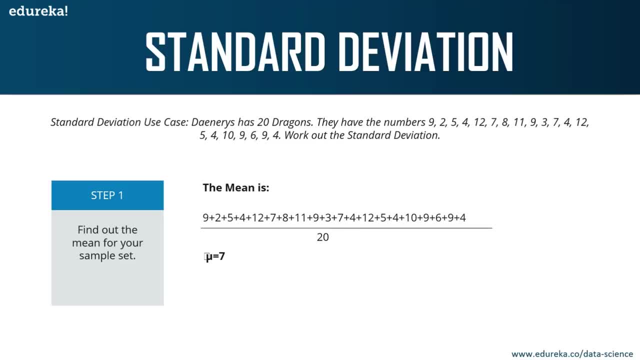 and divide it by the total number of samples in your data set. So you get a value of seven here. Then you calculate the RHS of your standard deviation formula, all right. So from each data point you're going to subtract the mean and you're going to square that, all right. 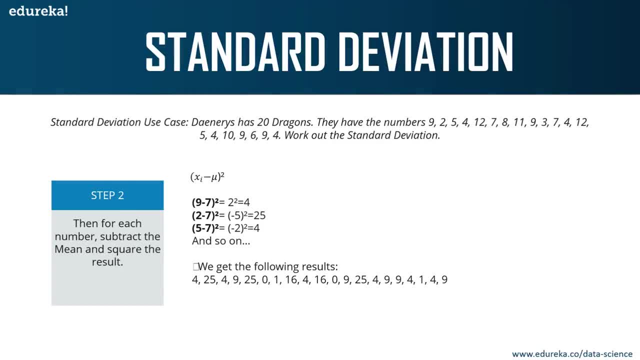 So when you do that, you'll get the following result: You'll basically get this: 425,, 4925, and so on. So finally, you'll just find the mean of these squared differences all right. So your standard deviation will come up to 2.983. 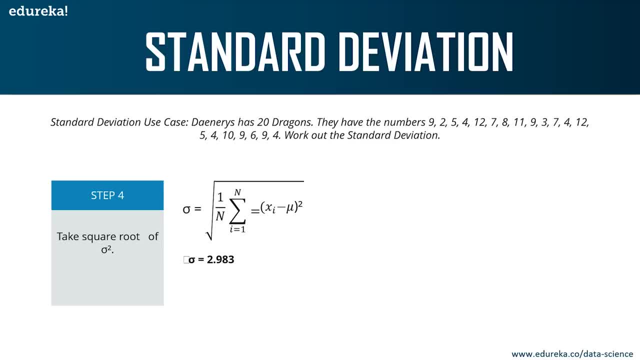 once you take the square root. So, guys, this is pretty simple. It's a simple mathematic technique. All you have to do is you have to substitute the values in the formula. all right, I hope this was clear to all of you. 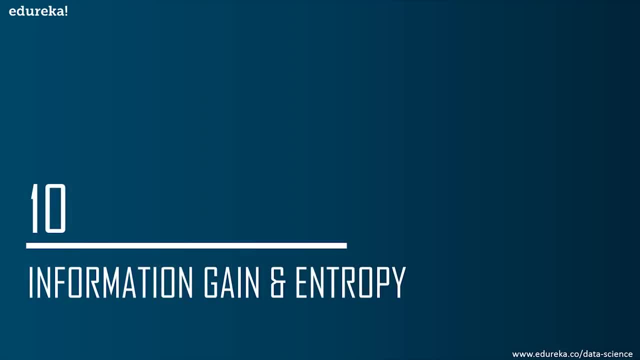 Now let's move on and discuss the next topic, which is information gain and entropy. Now, this is one of my favorite topics in statistics. It's very interesting, And this topic is mainly involved in machine learning algorithms like decision trees and random forest. all right, 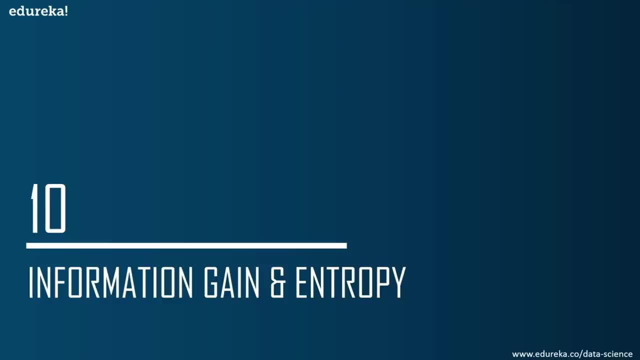 It's very important for you to know how information gain and entropy really work and why they're so essential in building machine learning models. We'll focus on the statistic parts of information gain and entropy And after that we'll discuss a use case and see how information gain and entropy 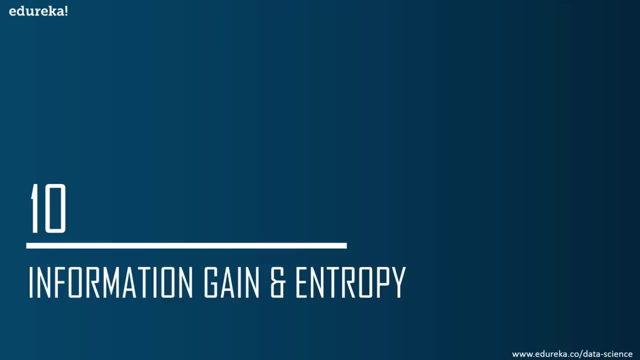 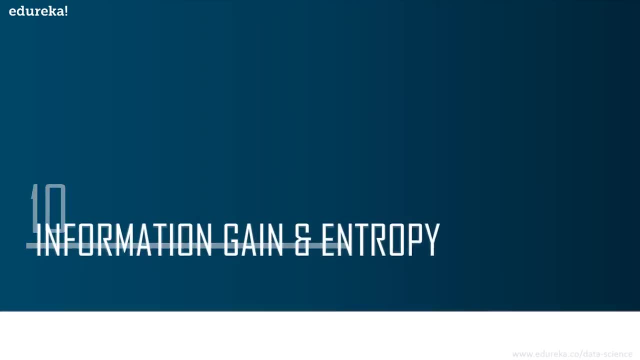 is used in decision trees. So for those of you who don't know what a decision tree is, it is basically a machine learning algorithm. You don't have to know anything about this. I'll explain everything in depth, so don't worry. 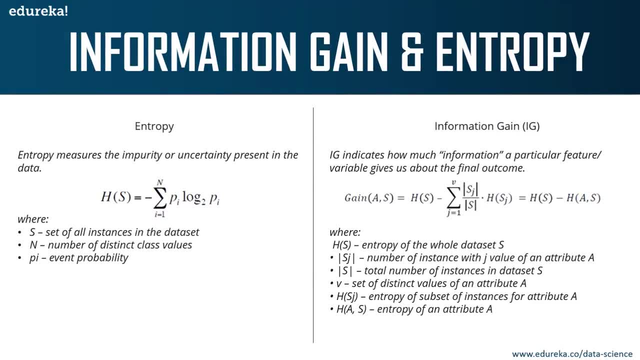 Now let's look at what exactly entropy and information gain is. Now, guys, entropy is basically the measure of any sort of uncertainty that is present in the data. All right, so it can be measured by using this formula. So here, S is the set of all instances in the data set. 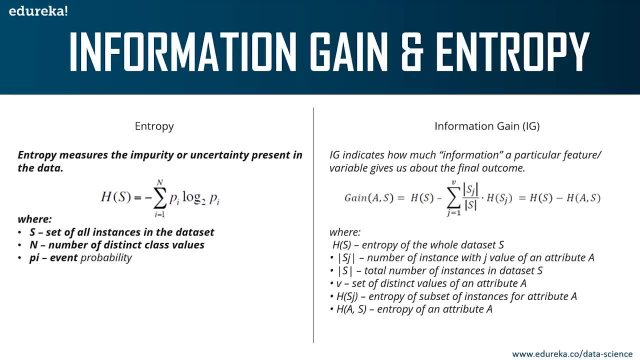 All right, so it can be measured by using this formula. So here: S is the set of all instances in the data set or all the data items in the data set. N is the different type of classes in your data set. Pi is the event probability. 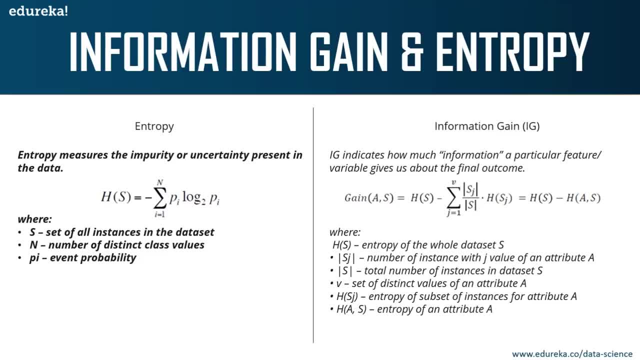 Now, this might seem a little confusing to you all, but when we go through the use case, you'll understand all of these terms even better. all right, Coming to information gain, as the word suggests, information gain indicates how much information a particular feature or a particular variable. 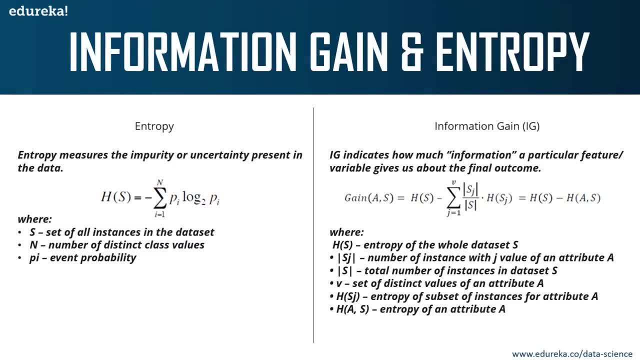 gives us about the final outcome. Okay, it can be measured by using this formula. So again here: H of S is the entropy of the whole data set. S, Sj is the number of instances with the j value of an attribute A. 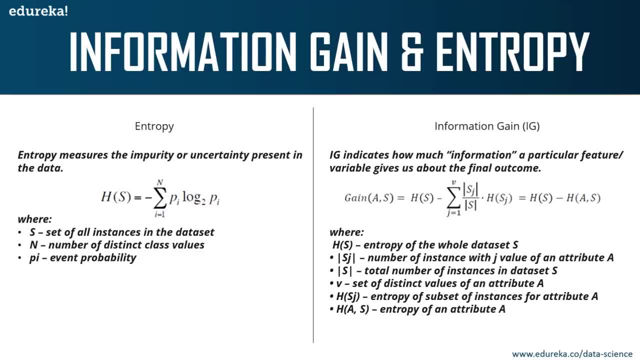 S is the total number of instances in the data set, V is the set of distinct values of an attribute A, H of Sj is the entropy of subset of instances And H of A comma. S is the entropy of an attribute A, Even though this seems confusing. 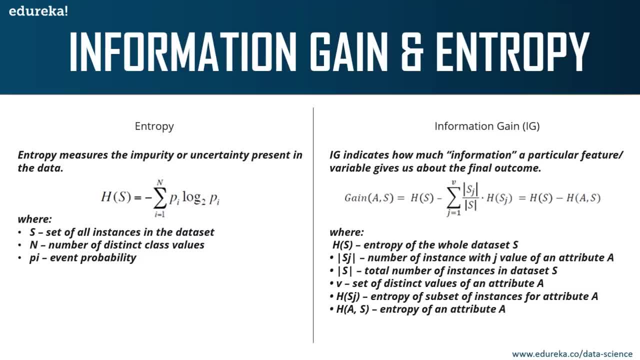 I'll clear out the confusion. All right, let's discuss a small problem statement Where we'll understand how information gain and entropy is used to study the significance of a model. So, like I said, information gain and entropy are very important statistical measures. 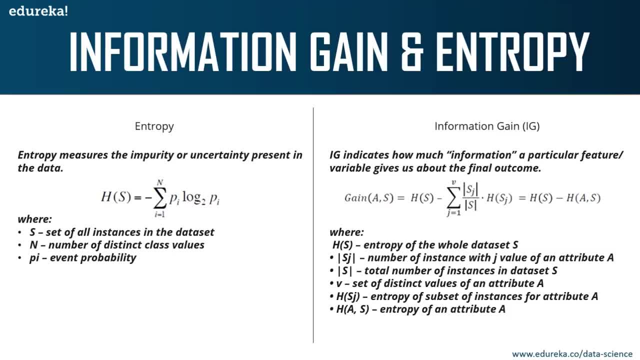 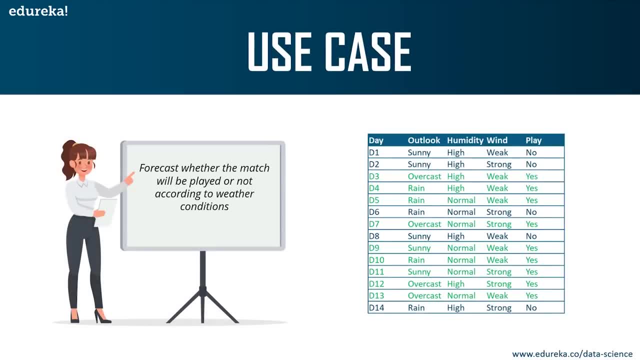 that let us understand the significance of a predictive model. okay, To get a more clear understanding, let's look at a use case. All right, now suppose we're given a problem statement. All right, the statement is that you have to predict. 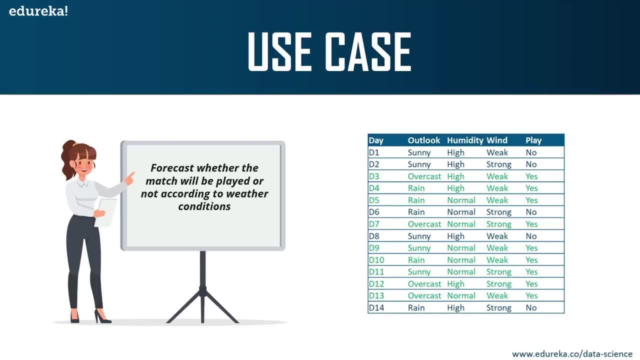 whether a match can be played or not by studying the weather conditions. So the predictor variables here are outlook, humidity, wind Day is also a predictor variable. The target variable is basically play. all right, The target variable is the variable that you're trying to predict. okay, 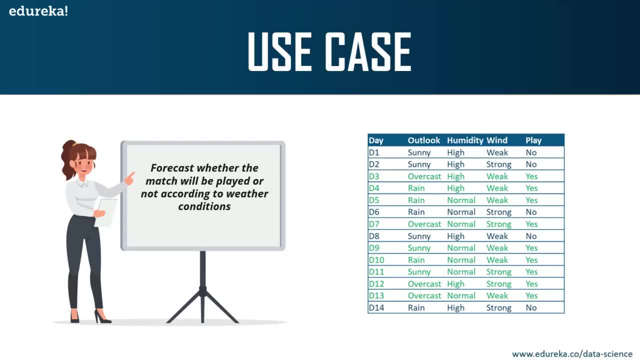 Now the value of the target variable will decide whether or not a game can be played all right. So that's why the play has two values. It has no and yes. No meaning that the weather conditions are not good and therefore you cannot play the game. 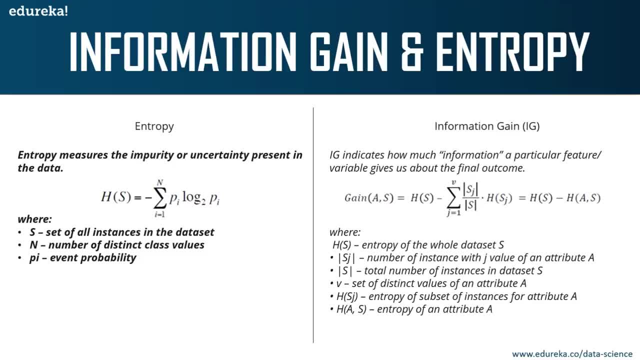 or all the data items. in the data set, N is the different type of classes. in your data set, Pi is the event probability. Now, this might seem a little confusing to y'all, but when we go through the use case you'll understand all of these terms even better. all right, 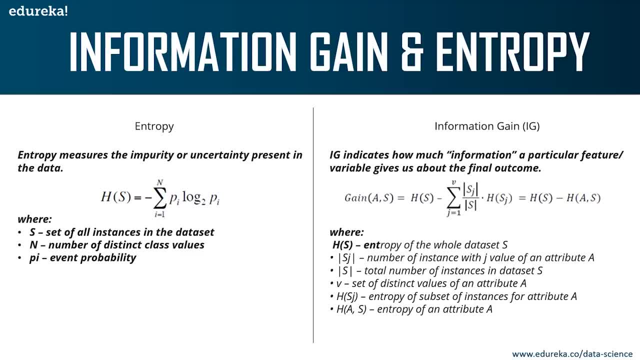 Coming to information gain, as the word suggests, information gain indicates how much information a particular feature or a particular variable can generate. So information gain gives us about the final outcome. Okay, it can be measured by using this formula. So, again here, H is the entropy of the whole data set, S 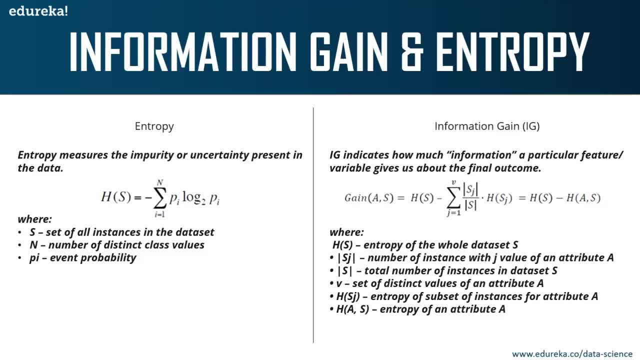 Sj is the number of instances with the j value of an attribute A. S is the total number of instances in the data set. V is the set of distinct values of an attribute A. H is the entropy of subset of instances And H is the entropy of an attribute A. 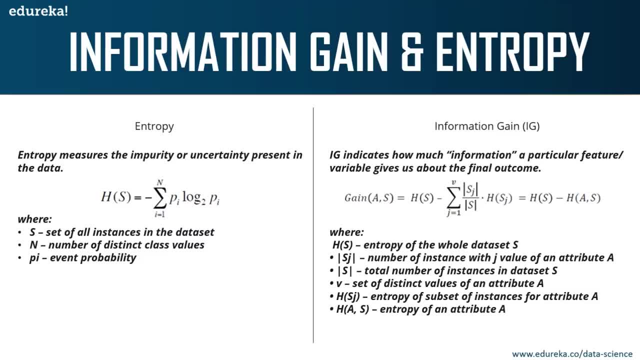 Even though this seems confusing, I'll clear out the confusion. all right, Let's discuss a small problem statement where we'll understand how information gain and entropy is used to study the significance of a model. So, like I said, information gain and entropy. 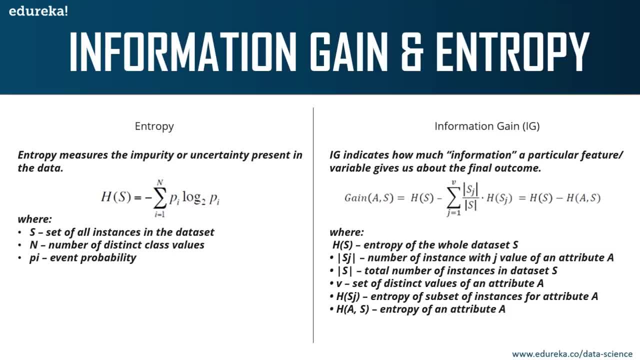 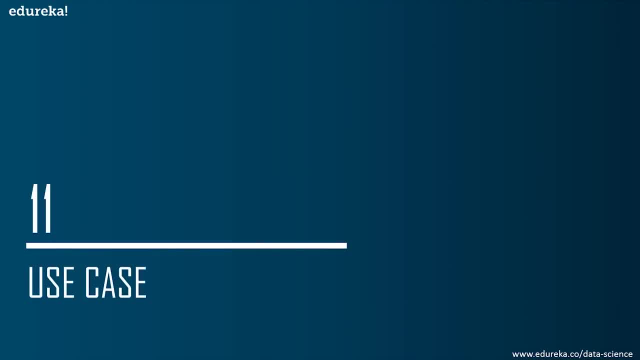 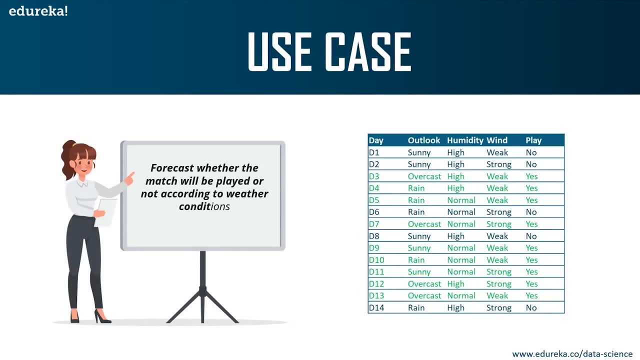 are very important statistical measures that let us understand the significance of a predictive model. okay, To get a more clear understanding, let's look at a use case. All right, now suppose we're given a problem statement. All right, the statement is that you have to predict. 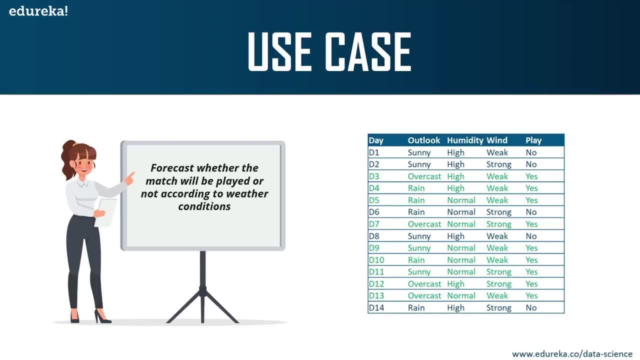 whether a match can be played or not by studying the weather conditions. So the predictor variables here are outlook, humidity, wind Day is also a predictor variable. The target variable is basically play. all right, The target variable is the variable that you're trying to predict. okay, 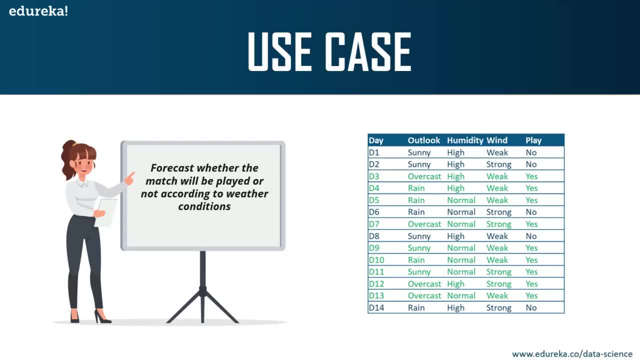 Now the value of the target variable will decide whether or not a game can be played all right. So that's why the play has two values. It has no and yes. No meaning that the weather conditions are not good and therefore you cannot play the game. 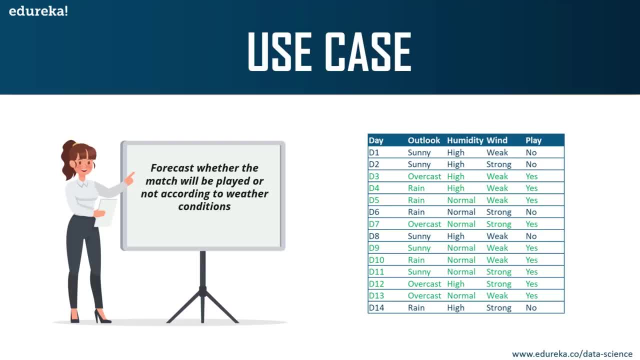 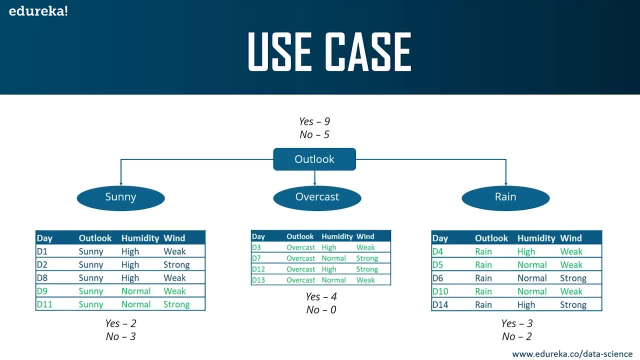 Yes, meaning that the weather conditions are good and suitable for you to play the game. all right. So that was a problem statement. I hope the problem statement is clear to all of you Now. to solve such a problem, we make use of something known as decision trees. 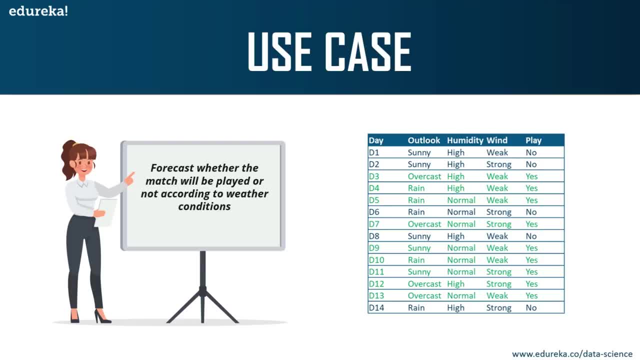 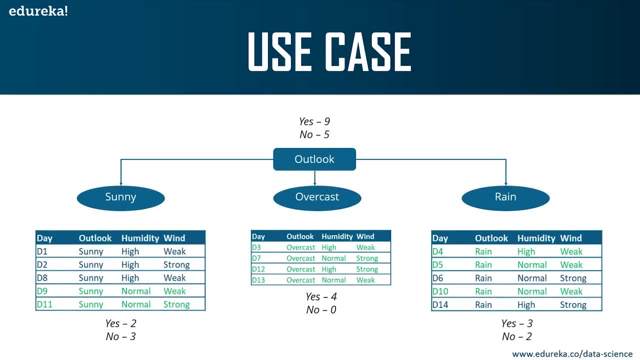 Meaning that the weather conditions are good and suitable for you to play the game. all right, So that was a problem statement. I hope the problem statement is clear to all of you Now. to solve such a problem, we make use of something known as decision trees. 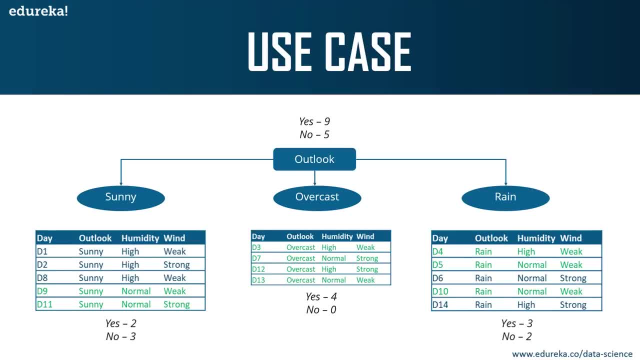 So guys think of an inverted tree, and each branch of the tree denotes some decision. all right, Each branch is known as the branch node and at each branch node you're going to take a decision in such a manner that you'll get an outcome at the end of the branch. 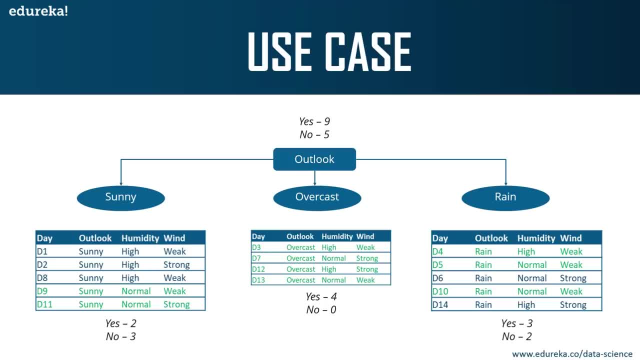 All right Now. this figure here basically shows that out of 14 observations, nine observations result in a yes, Meaning that out of 14 days, the match can be played only on nine days. all right, So here, if you see, on day one, day two, day eight, 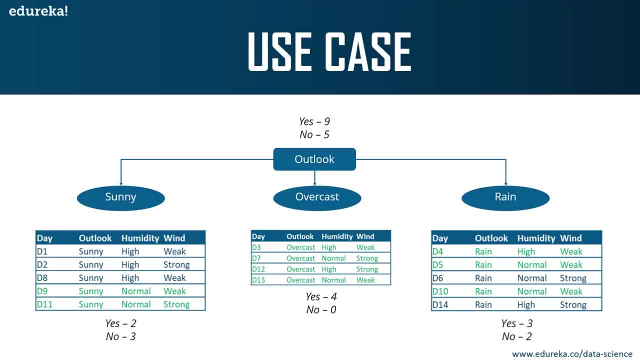 day nine and day 11, the outlook has been sunny, all right. So basically, we're trying to cluster our data set depending on the outlook. So when the outlook is sunny, this is our data set. when the outlook is overcast, this is what we have. 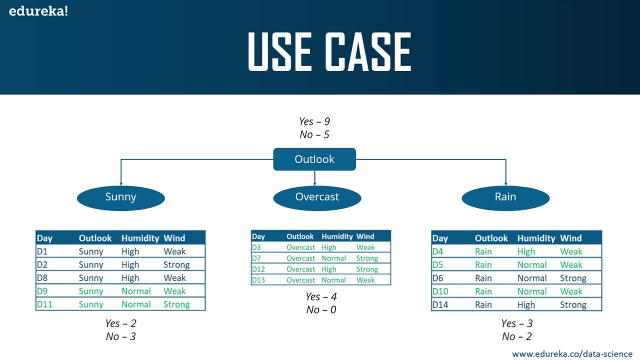 and when the outlook is rain, this is what we have all right. So when it is sunny, we have two yeses and three nos. okay, When the outlook is overcast, we have all four as yeses, meaning that on the four days when the outlook was overcast, 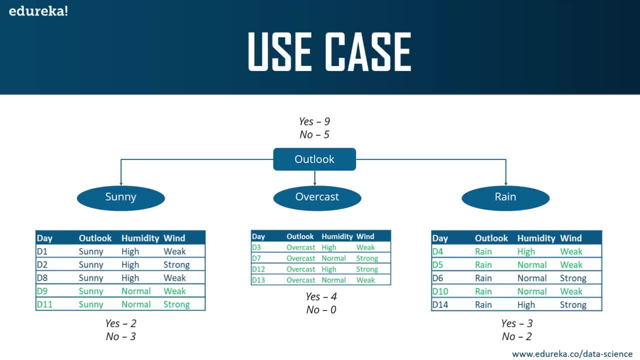 we can play the game all right. Now, when it comes to rain, we have three yeses and two nos, all right. So if you notice, here the decision is being made by choosing the outlook way, by choosing the variable as the root node, okay, 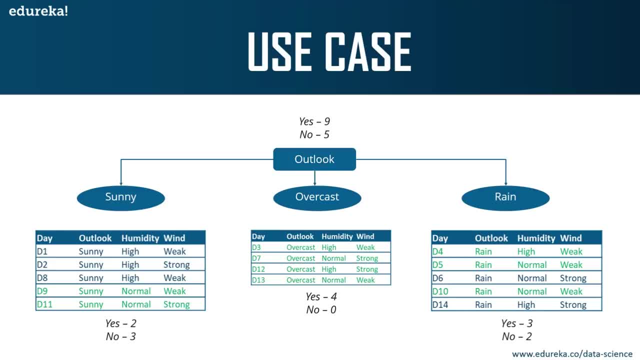 So the root node is basically the topmost node in a decision tree. Now what we've done here is we've created a decision tree that starts with the outlook node, all right. Then you're splitting the decision tree further, depending on other parameters like sunny, overcast and rain, all right. 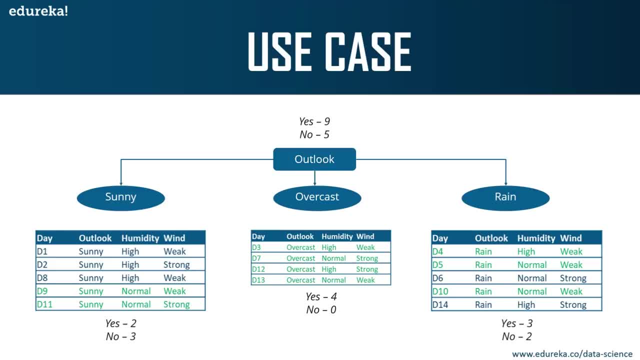 Now, like we know, that outlook has three values- sunny, overcast and rain- So let me explain this in a more in-depth manner. okay, So what you're doing here is you're making the decision tree by choosing the outlook variable at the root node. 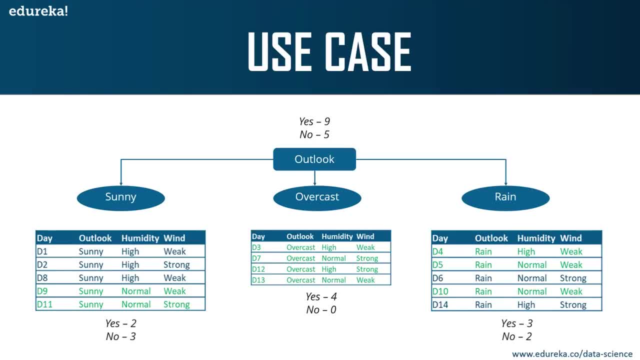 So guys think of an inverted tree, and each branch of the tree denotes some decision. all right, Each branch is known as the branch node and at each branch node, each branch node is a decision. You're going to take a decision in such a manner. 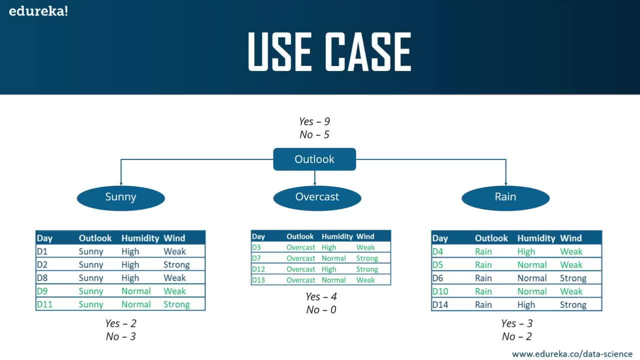 that you'll get an outcome at the end of the branch. all right, Now. this figure here basically shows that, out of 14 observations, nine observations result in a yes, meaning that out of 14 days, the match can be played only on nine days. all right. 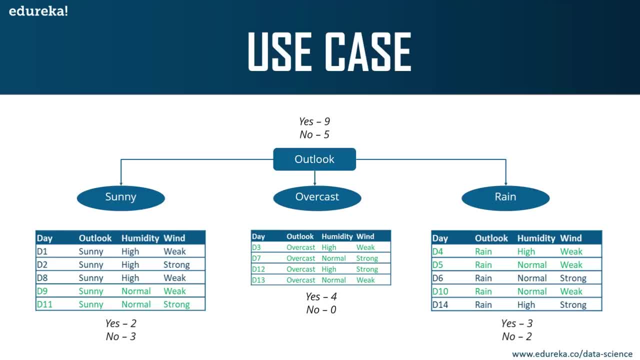 So here, if you see, on day one, day two, day eight, day nine and day 11, the outlook has been sunny, all right. So basically, we're trying to cluster a data set depending on the outlook. So when the outlook is sunny, this is our data set. 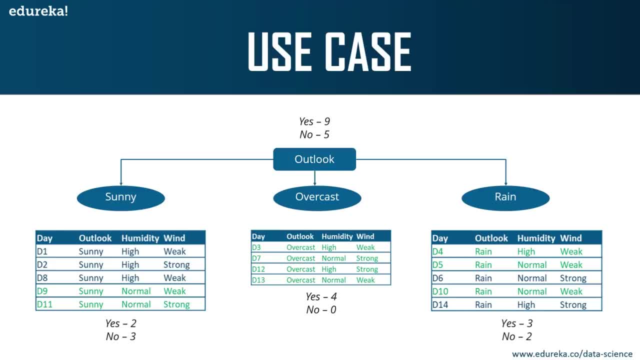 When the outlook is overcast, this is what we have, and when the outlook is rain, this is what we have. all right. So when it is sunny, we have two yeses and three nos. okay, When the outlook is overcast, we have all four as yeses. 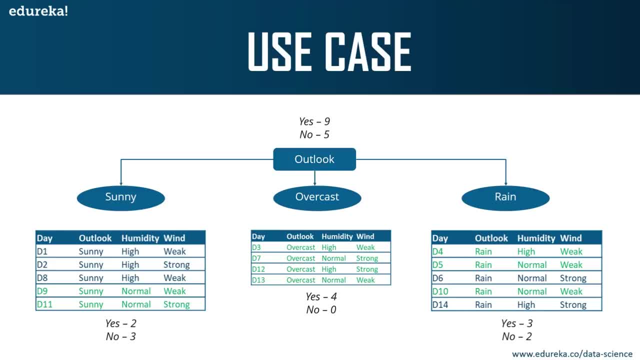 meaning that on the four days when the outlook was overcast, we can play the game all right. Now, when it comes to rain, we have three yeses and two nos, all right. So if you notice, here the decision is being made. 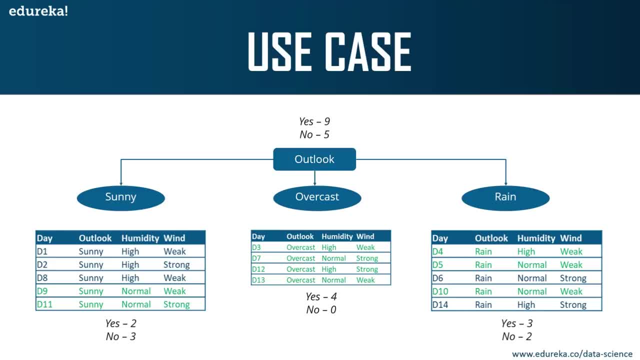 by choosing the outlook variable as the root node. okay, So the root node is basically the topmost node in a decision tree. Now, what we've done here is we've created a decision tree that starts with the outlook node. all right, Then you're splitting the decision tree further. 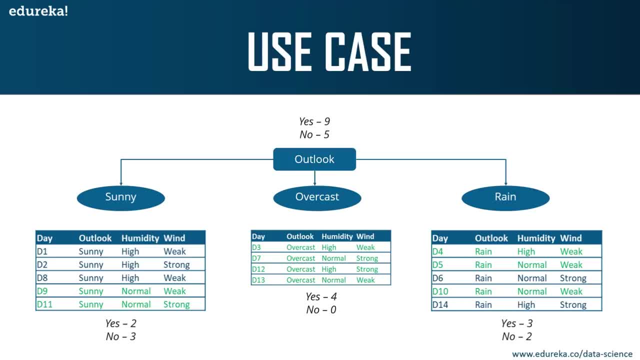 depending on other parameters like sunny, overcast and rain. all right, Now, like we know, that outlook has three values: sunny, overcast and rain. We're gonna explain this in a more in-depth manner. okay, So what you're doing here is you're making the decision tree. 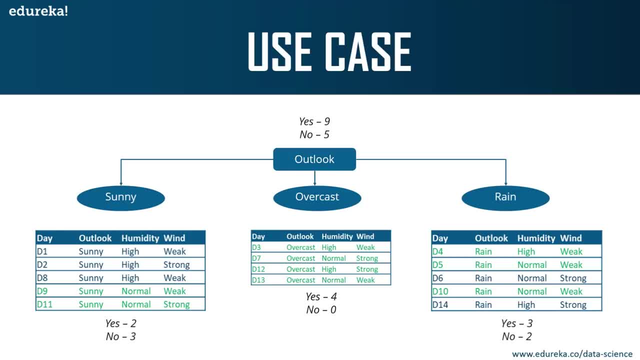 by choosing the outlook variable at the root node. The root node is basically the topmost node in a decision tree. Now the outlook node has three branches coming out from it, which is sunny, overcast and rain. So basically outlook can have three values. 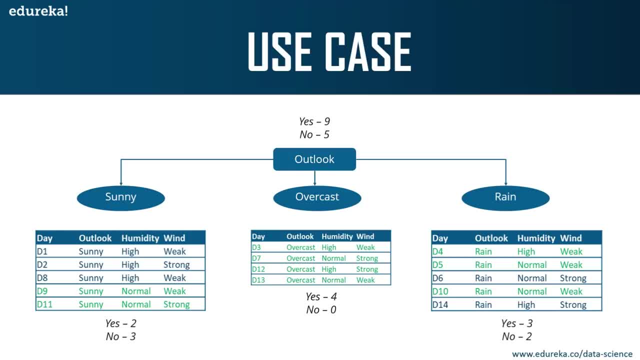 The root node is basically the topmost node in a decision tree. Now the outlook node has three branches coming out from it, which is sunny, overcast and rain. So basically outlook can have three values: Either it can be sunny, it can be overcast. 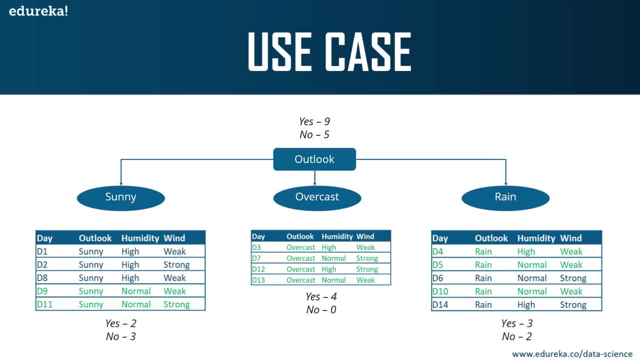 or it can be rainy. Okay now these three values are assigned to the immediate branch nodes and for each of these values, the possibility of play is equal to yes is calculated, So the sunny and the rain branches will give you an impure output. 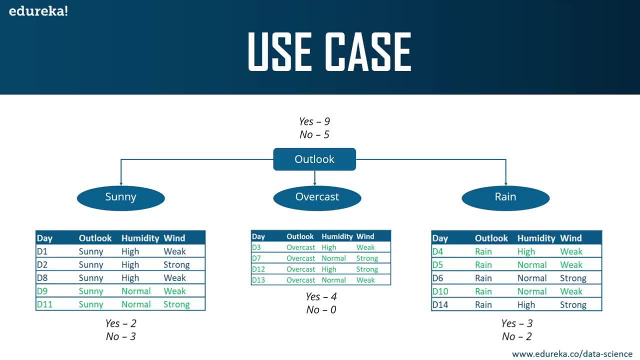 meaning that there is a mix of yes and no. right? There are two yeses here, three nos here. There are three yeses here and two nos over here, But when it comes to the overcast variable, it results in a 100% pure subset. all right, 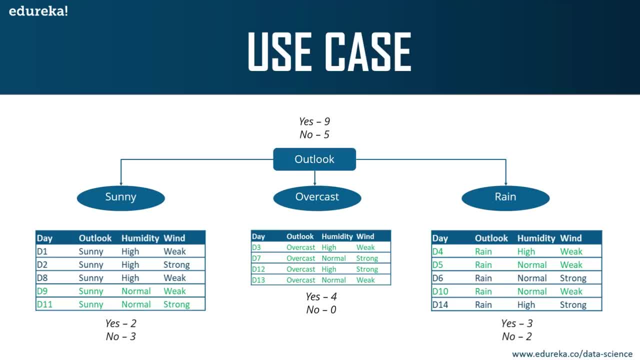 This shows that the overcast variable will result in a definite and certain output. This is exactly what entropy is used to measure. all right, It calculates the impurity or the uncertainty, all right, So the lesser the uncertainty or the entropy of a variable. 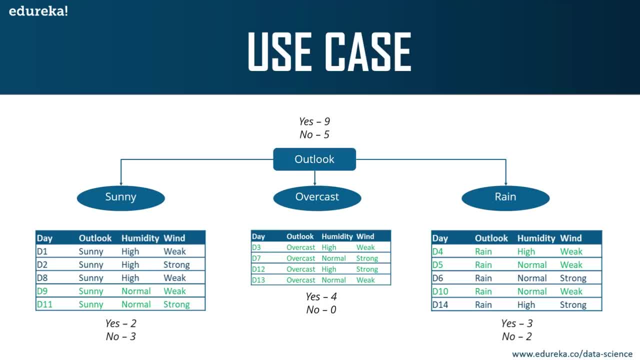 more significant is that variable. So, when it comes to overcast, there's literally no impurity in the data set. It is a 100% pure subset right. So we want variables like these in order to build a model, all right. 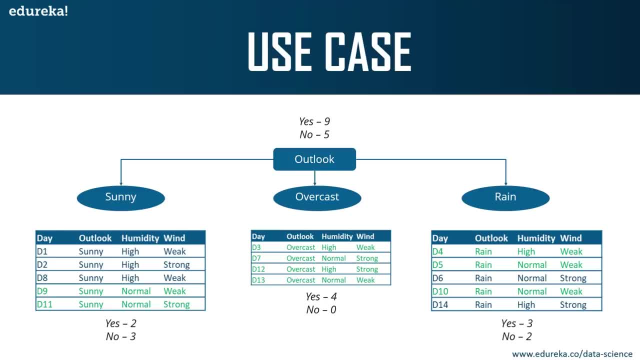 Now we don't always get lucky and we don't always find variables that will result in pure subsets. That's why we have the measure entropy. The more the entropy of a particular variable, the more significant that variable will be, So in a decision tree. 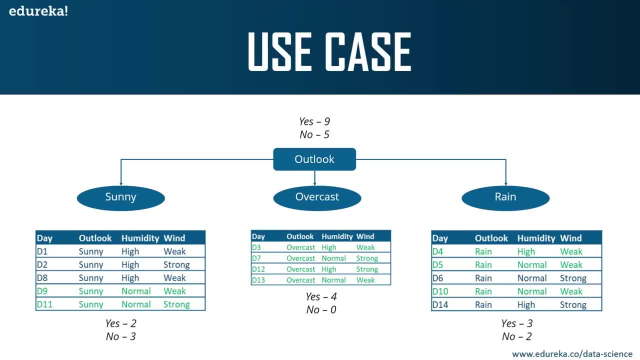 the root node is assigned the best attribute so that the decision tree can predict the most precise outcome, meaning that on the root node, you should have the most significant variable. all right, That's why we've chosen outlook. all right. Now, some of you might ask me: 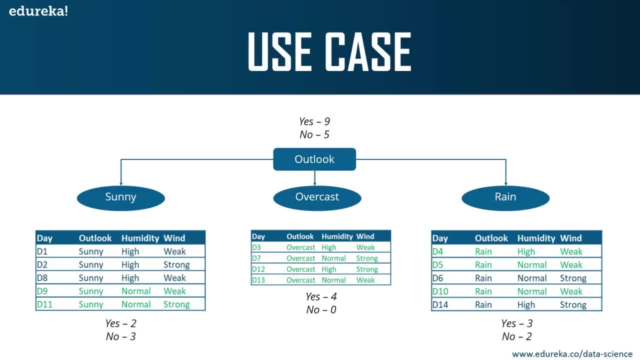 why haven't you chosen overcast? Now, guys, overcast is not a variable. It is a value of the outlook variable. all right. Why have you chosen outlook here? Because it has a 100% pure subset, which is overcast. all right. 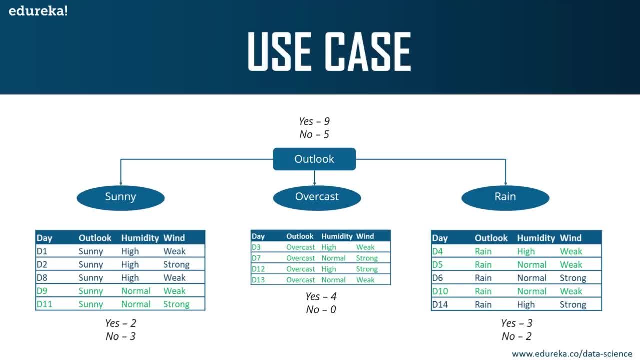 Either it can be sunny, it can be overcast or it can be rainy. Okay, now these three values are assigned to the immediate branch nodes and for each of these values, the possibility of play is equal to yes is calculated. So the sunny and the rain branches. 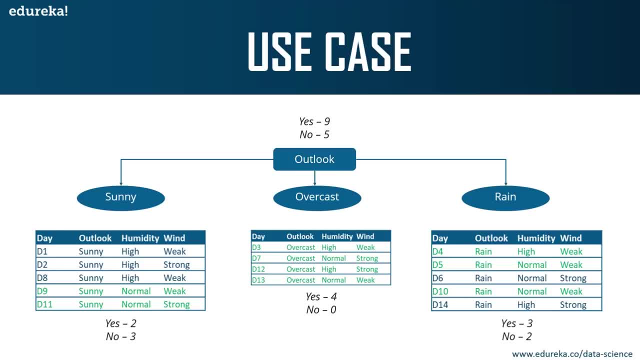 will give you an impure output, meaning that there is a mix of yes and no. right, There are two yeses here, three nos here. There are three yeses here and two nos over here, But when it comes to the overcast variable, 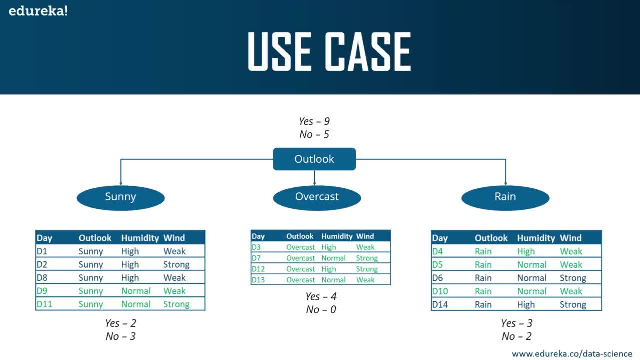 it results in a 100% pure subset. all right. This shows that the overcast variable will result in a definite and certain output. This is exactly what entropy is used to measure. all right, It calculates the impurity or the uncertainty. all right. 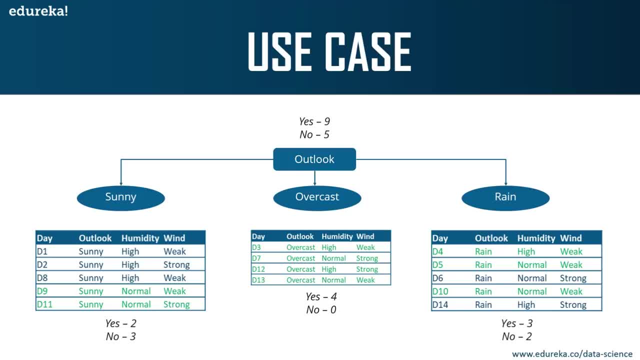 So the lesser the uncertainty or the entropy of a variable, more significant is that variable. So when it comes to overcast, there's literally no impurity in the data set. It is a 100% pure subset right. So we want variables like these. 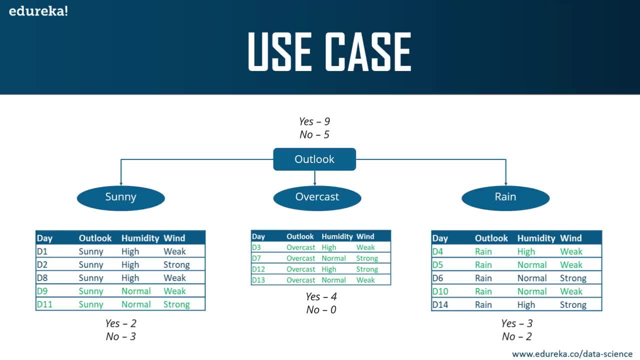 in order to build a model. all right, Now, we don't always get lucky and we don't always find variables that will result in pure subsets. That's why we have the measure entropy, So the lesser the entropy of a particular variable. 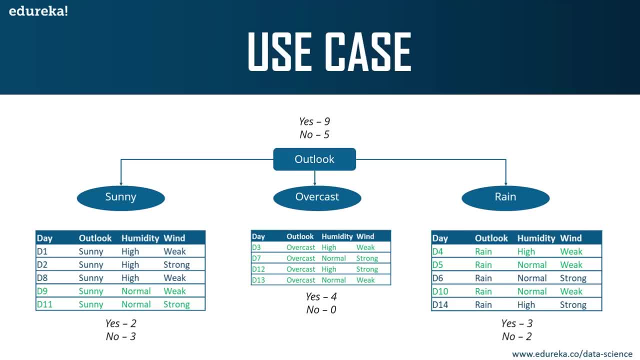 the more significant that variable will be. So in a decision tree, the root node is assigned the best attribute so that the decision tree can predict the most precise outcome, meaning that on the root node you should have the most significant variable. all right, 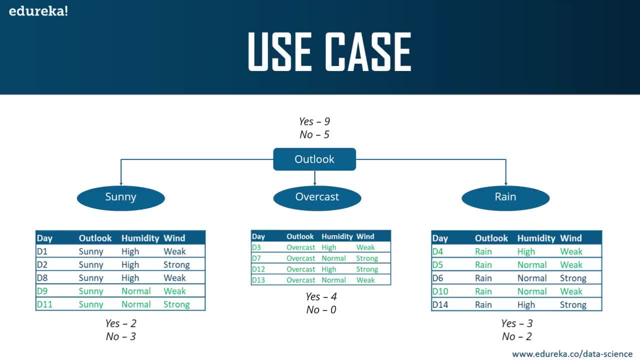 That's why we've chosen outlook. all right. Now some of you might ask me: why haven't you chosen overcast? Now, guys, overcast is not a variable. It is a value of the outlook variable. all right, That's why we've chosen outlook here. 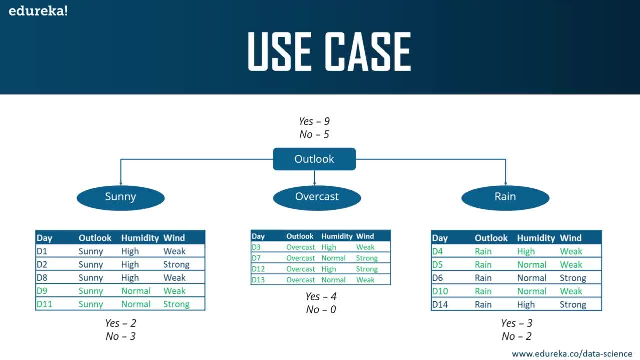 because it has a 100% pure subset which is overcast. all right Now the question in your head is: how do I decide which variable or attribute best splits the data? Now, right now, I know I looked at the data and I told you that you know. 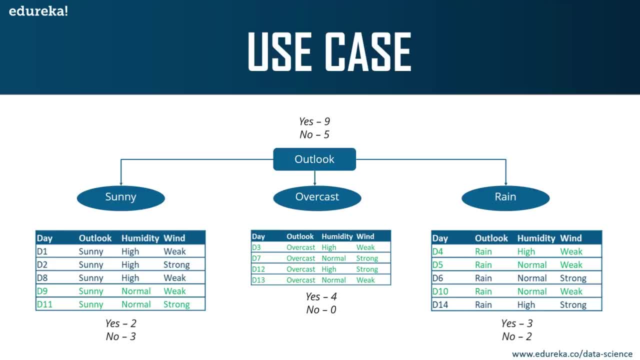 Now the question in your head is: how do I decide which variable or attribute best splits the data? Now, right now, I know I looked at the data and I told you that you know, here we have a 100% pure subset. 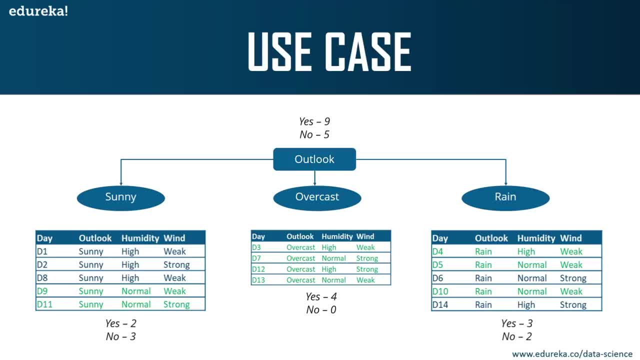 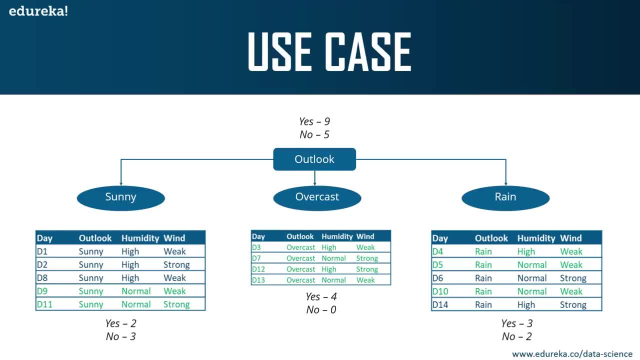 and entropy will help you understand which variable will best split the data set- all right- Or which variable you have to assign to the root node, Because whichever variable is assigned to the root node, it will best split the data set And it has to be the most significant variable, all right. 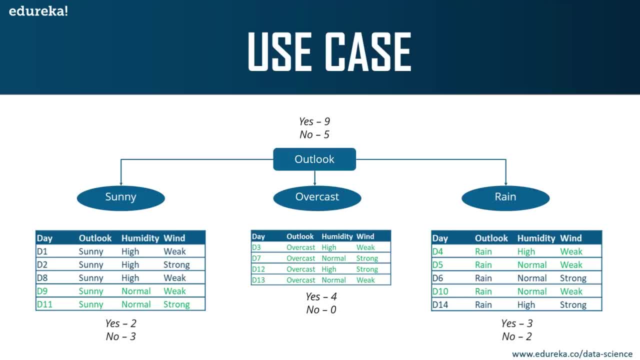 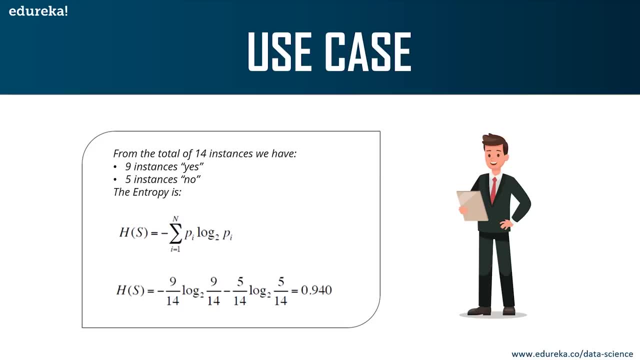 So how we can do this is we need to use information gain and entropy. So from the total of the 14 instances that we saw, nine of them said yes and five of the instances said no, which means that you cannot play on that particular day. 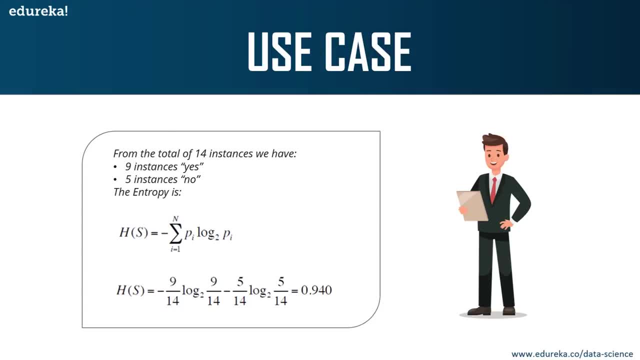 All right. so how do you calculate the entropy? So this is a formula. You just substitute the values in the formula. So when you substitute the values in the formula, you'll get a value of 0.940,. all right, This is the entropy. 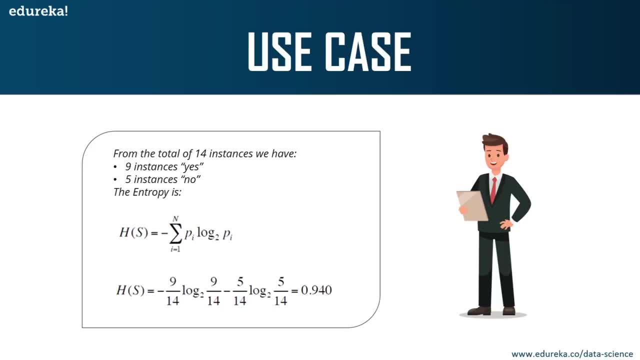 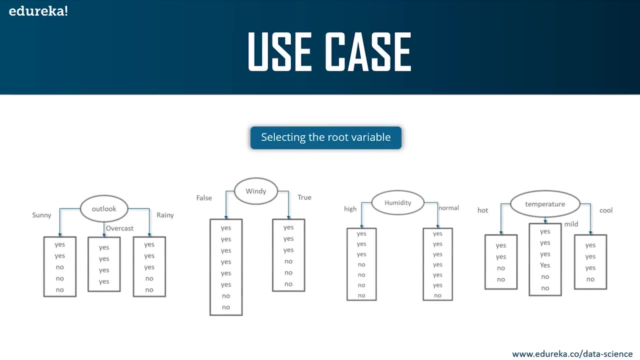 or this is the uncertainty of the data present in our sample. Now, in order to ensure that we choose the best variable for the root node, let us look at all the possible combinations that you can use on the root node. Okay, these are all the possible combinations. You can either have outlook. you can have windy humidity. 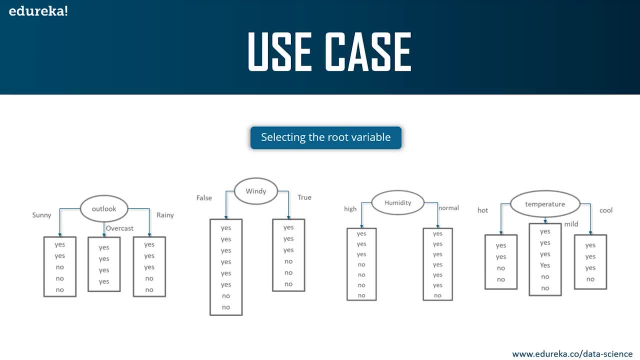 or temperature. Okay, these are our four variables, and you can have any one of these variables as your root node. But how do you select which variable best fits the root node? That's what we are going to see, by using information gain and entropy. So, guys, now the task at hand is to find 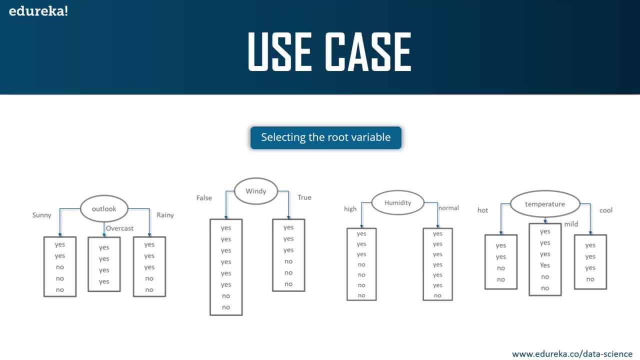 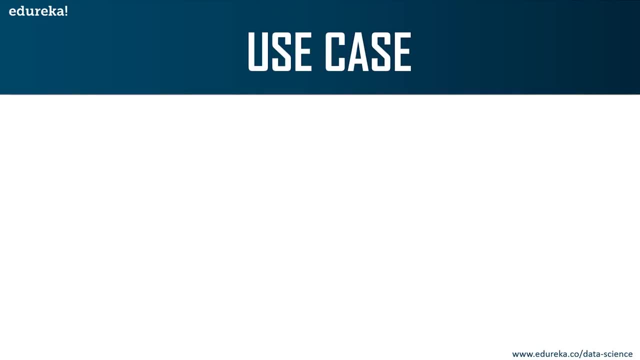 the information gain for each of these attributes. Alright, so for outlook, for windy, for humidity and for temperature, we're going to find out the information gain. Alright, now a point to remember is that the variable that results in the highest information gain must be chosen because it will 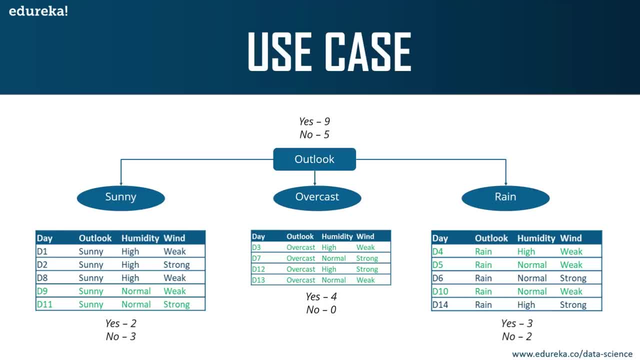 here we have a 100% pure subset, But what if it's a more complex problem and you're not able to understand which variable will best split the data? So, guys, when it comes to decision trees, information gain and entropy will help you understand. 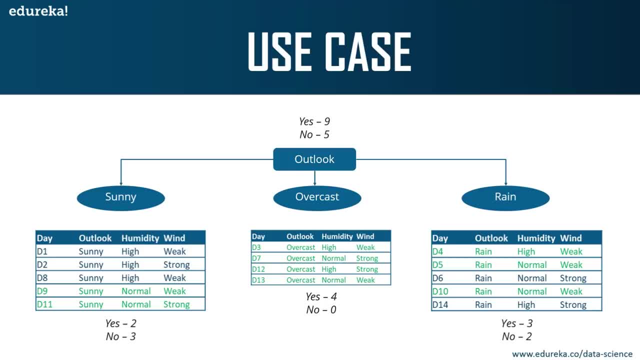 which variable will best split the data set, all right, Or which variable you have to assign to the root node, because whichever variable is assigned to the root node, it will best split the data set and it has to be the most significant variable, all right. 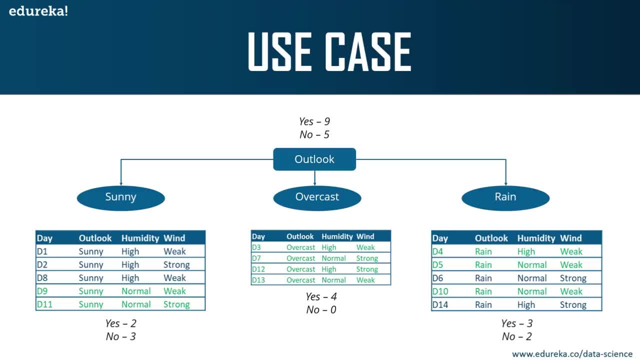 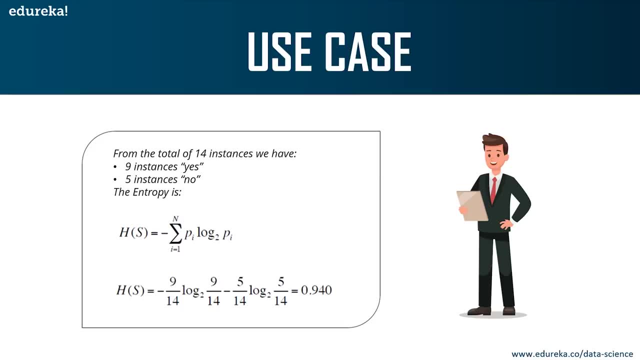 So how we can do this is we need to use information gain and entropy. So from the total of the 14 instances that we saw, nine of them said yes and five of the instances said no, that you cannot play on that particular day. all right. 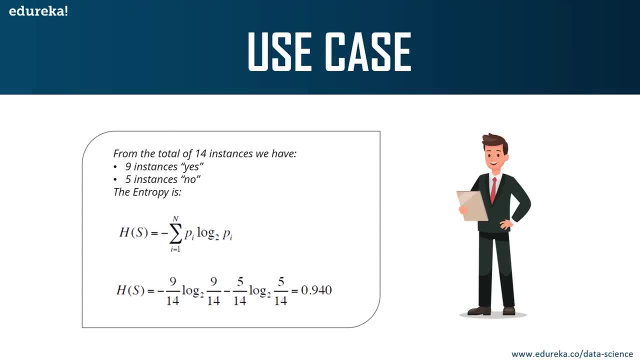 So how do you calculate the entropy? So this is the formula: You just substitute the values in the formula. So when you substitute the values in the formula, you'll get a value of 0.940,. all right, This is the entropy or this is the uncertainty. 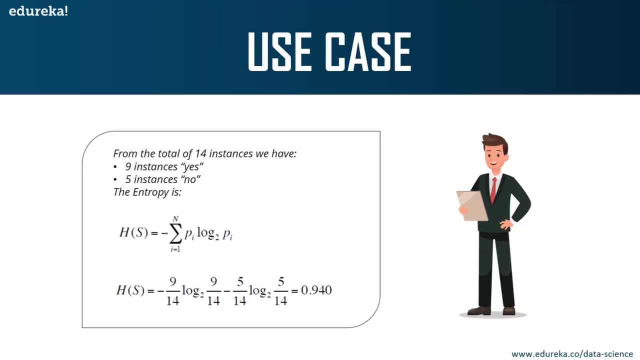 of the data present in our sample. Now, in order to ensure that we choose the best variable for the root node, let us look at all the possibilities that you can use on the root node. okay, So these are all the possible combinations. You can either have outlook. 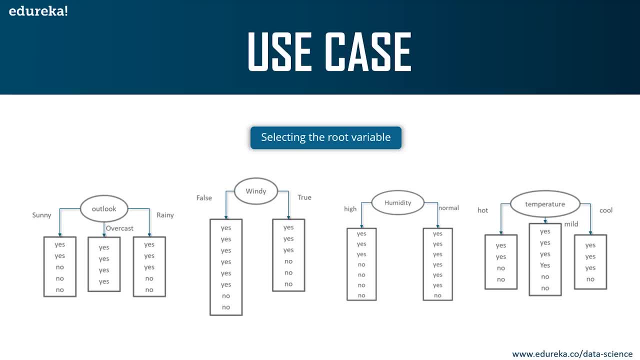 you can have windy humidity or temperature. Okay, these are our four variables, and you can have any one of these variables as your root node. But how do you select which variable best fits the root node? That's what we are going to see. 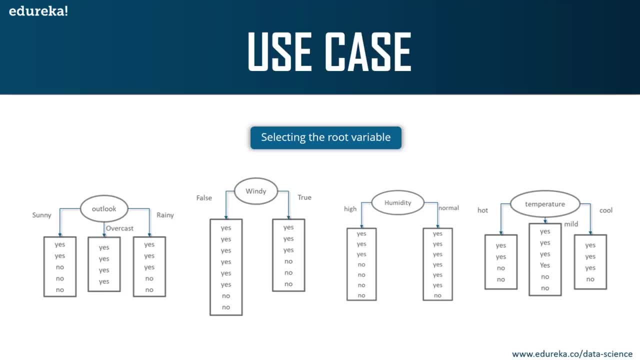 by using information gain and entropy. So, guys, now the task at hand is to find the information gain for each of these attributes. all right, So for outlook, for windy, for humidity and for temperature, we're going to find out the information gain, all right. 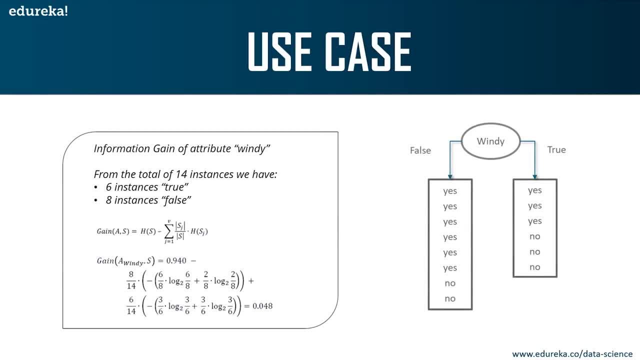 Now a point to remember is that the variable that results in the highest information gain must be chosen because it'll give us the most precise and output information. all right. So the information gain for attribute windy- we'll calculate that first. Here we have six instances of true. 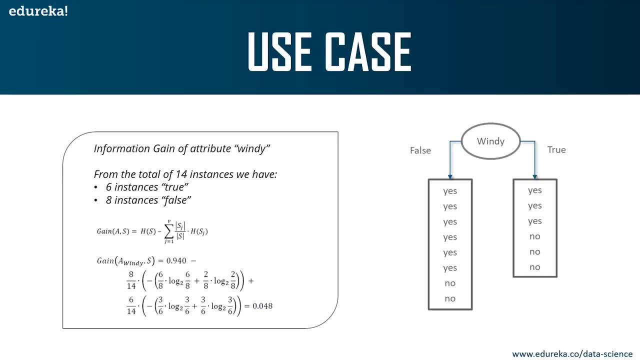 give us the most precise and output information. Alright, so the information gain for attribute windy. we'll calculate that first. Here we have six instances of true and eight instances of false. Okay, so when you substitute all the values in the formula, you'll get a value of 0.0. 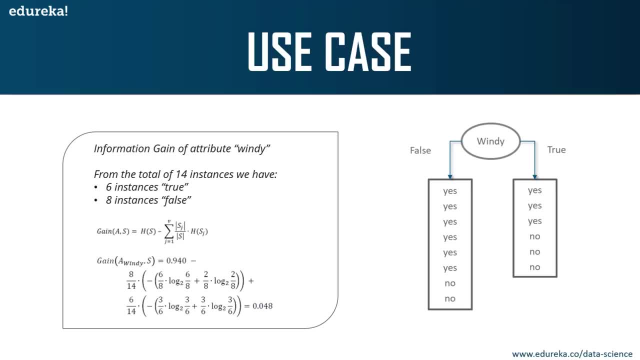 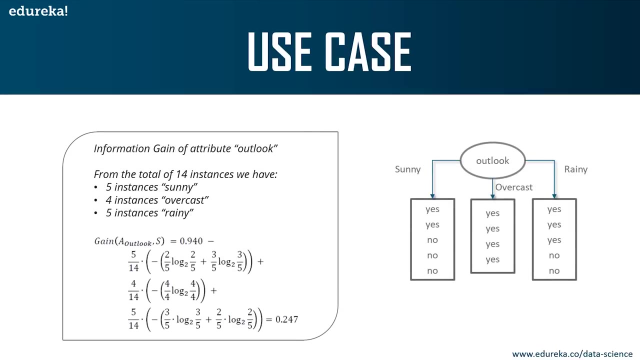 48.. So we get a value of 0.048.. Now, this is a very low value for information gain. Alright, so the information that you're going to get from windy attribute is pretty low. So let's calculate the information gain of attribute outlook. Alright, so from the total of 14 instances, we have five. 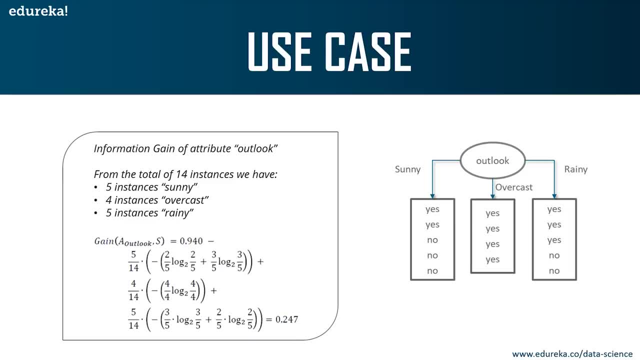 instances which say sunny, four instances which are overcast and five instances which are rainy. Alright, for sunny, we have three yeses and two noes. For overcast, we have all the four as yes. For rainy, we have three yes and two noes. Okay so, 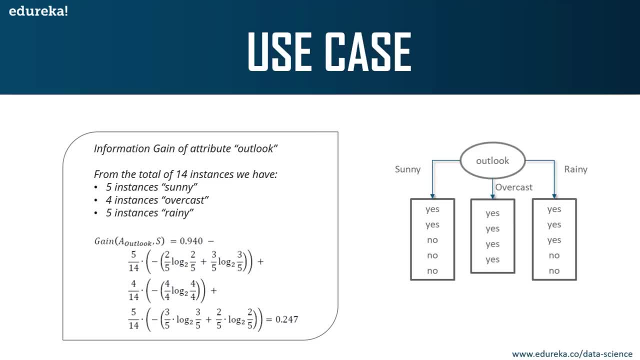 when you calculate the information gain of the outlook variable, we'll get a value of 0.247.. Now compare this to the information gain of the windy attribute. This value is actually pretty good. Right, we have 0.247, which is a pretty good value for information gain. Now let's look at the 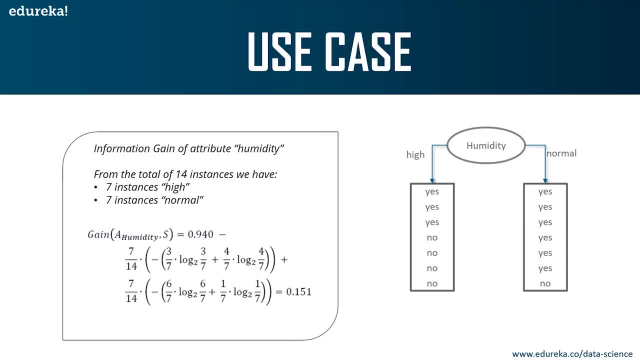 information: gain of attribute humidity. Now over here we have seven instances which say high and seven instances which say normal, Right and under the high branch node we have three instances which say yes and the rest four instances which say no. Similarly, under the normal branch, we 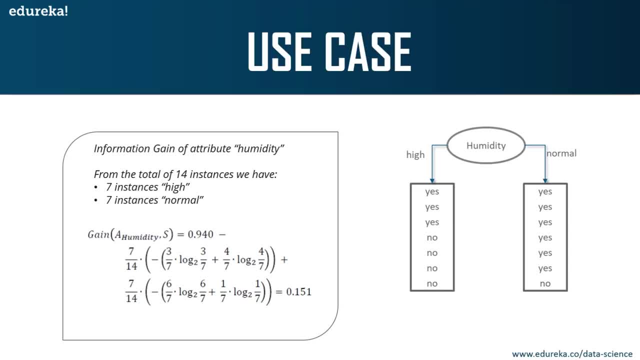 have one, two, three, four, five, six, seven instances which say yes and one instance which says no. Alright, so when you calculate the information gain for the humidity variable, you're going to get a value of 0.151.. Now, this is also a pretty decent value. 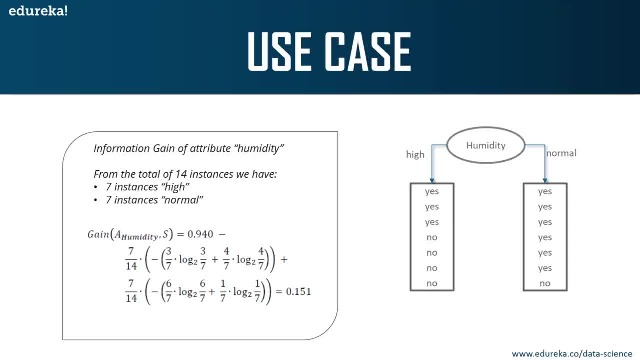 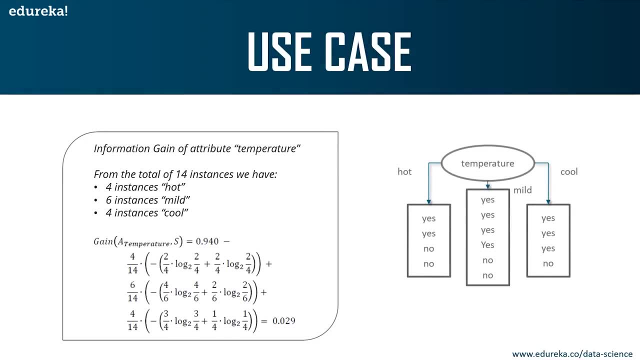 but when you compare it to the information gain of the attribute outlook, it is less. Right now let's look at the information gain of attribute temperature. Alright, so the temperature can hold. repeat. so basically, the temperature attribute can hold hot, mild and cool. Okay, under hot we have. 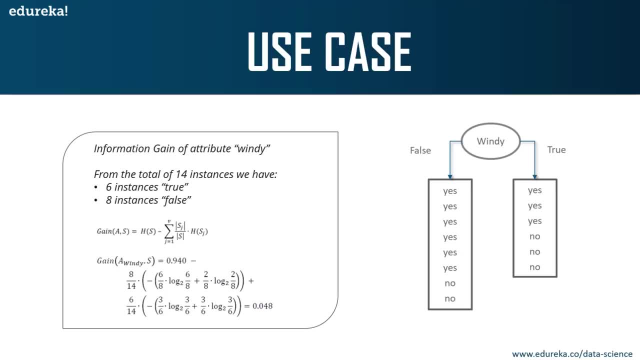 and eight instances of false. okay, So when you substitute all the values in the formula, you'll get a value of 0.048.. So we get a value of 0.048.. Now, this is a very low value for information gain. all right. 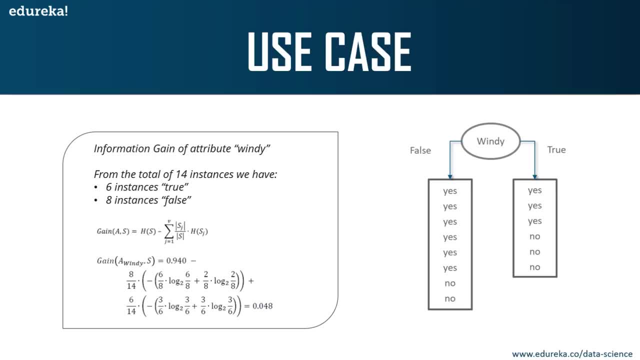 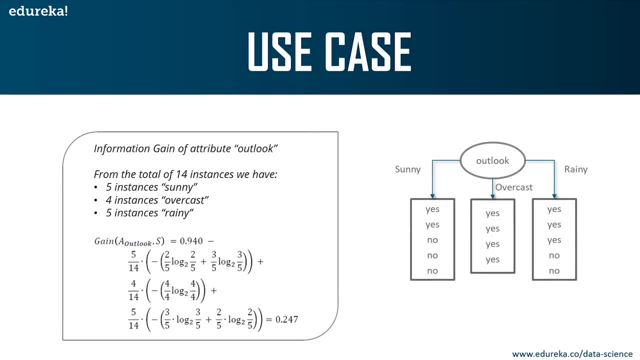 So the information that you're going to get from windy attribute is pretty low. So let's calculate the information gain of attribute outlook all right. So from the total of 14 instances, we have five instances which say sunny, four instances which are overcast. 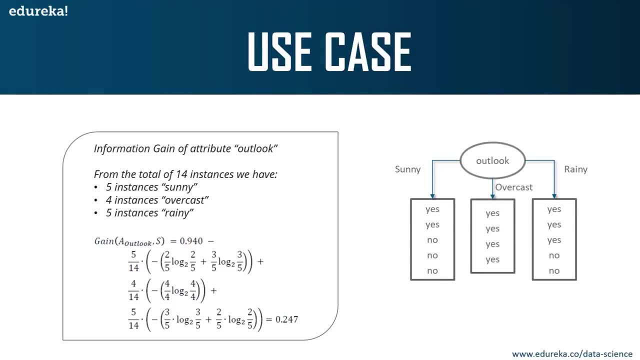 and five instances which are rainy: all right. For sunny, we have three yeses and two noes. For overcast, we have all the four as yes. For rainy, we have three yes and two noes. okay, So when you calculate, the information gain. 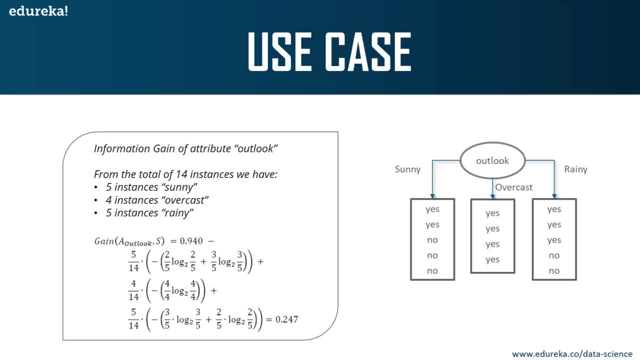 of the outlook variable, we'll get a value of 0.247.. Now compare this to the information gain of the windy attribute. This value is actually pretty good. right, We have 0.247, which is a pretty good value for information gain. 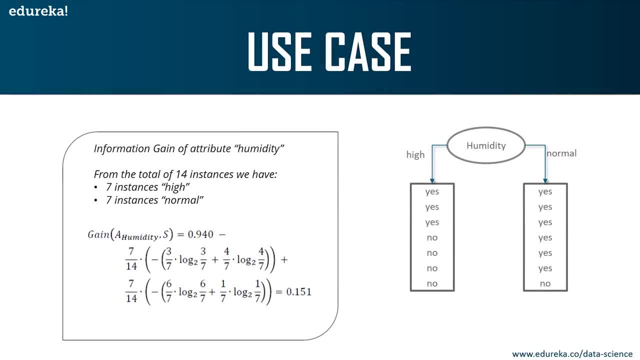 Now let's look at the information gain of attribute humidity. Now over here we have seven instances which say high and seven instances which say normal, right And under the high branch node. we have three instances which say yes and the rest four instances which say no. 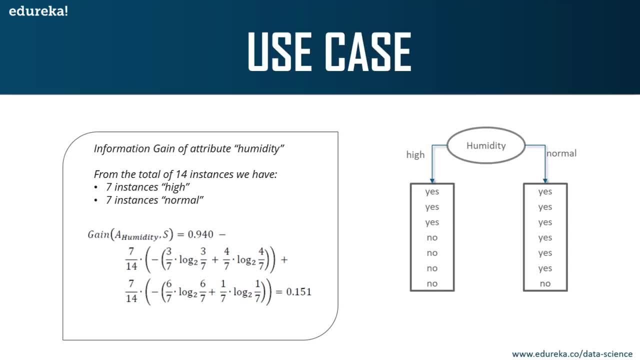 Similarly, under the normal branch, we have one, two, three, four, five, six, seven instances which say yes and one instance which says no. all right, So when you calculate the information gain for the humidity variable, you're going to get a value of 0.151. 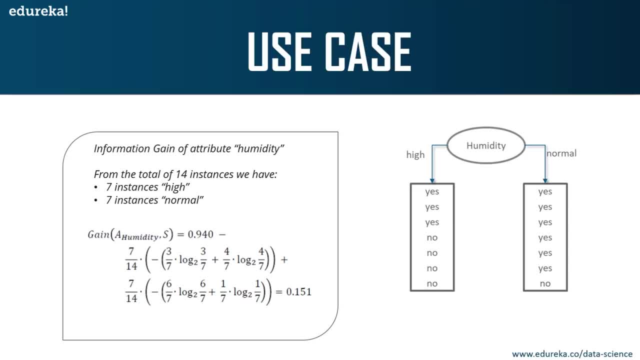 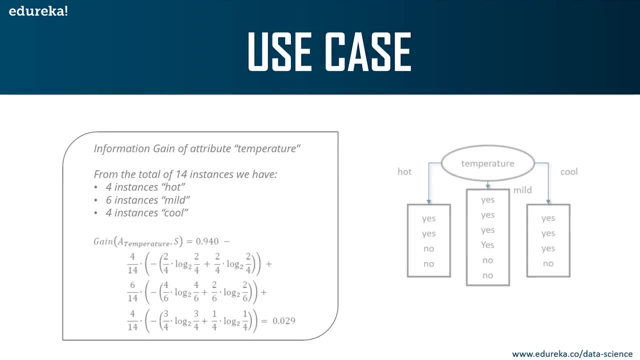 Now, this is also a pretty decent value, but when you compare it to the information gain of the attribute outlook, it is less all right. Now let's look at the information gain of attribute temperature. all right, So the temperature can hold. repeat. 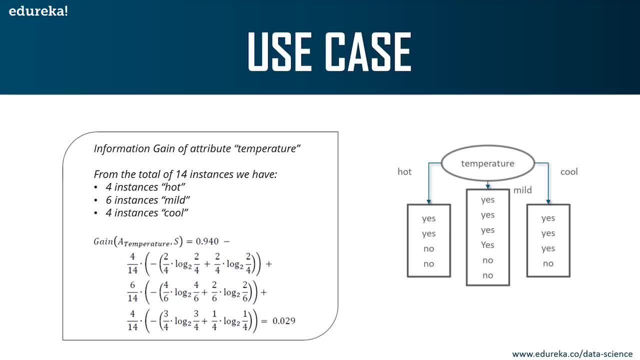 So basically the temperature attribute can hold hot, mild and cool. okay. Under hot, we have two instances which says yes and two instances for no. Under mild, we have four instances of yes and two instances of no. And under cool we have three instances of yes. 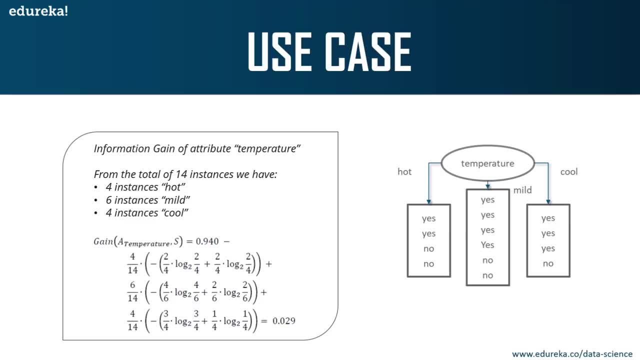 two instances which says yes and two instances for no. Under mild, we have four instances of yes and two instances of no, and under cool, we have three instances of yes and one instance of no. Alright, now, when you calculate the information gain for this attribute, you'll get: 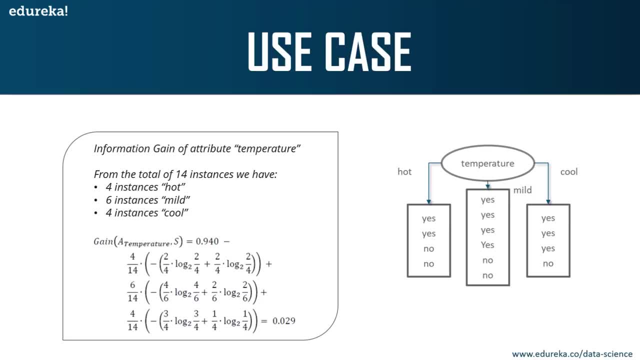 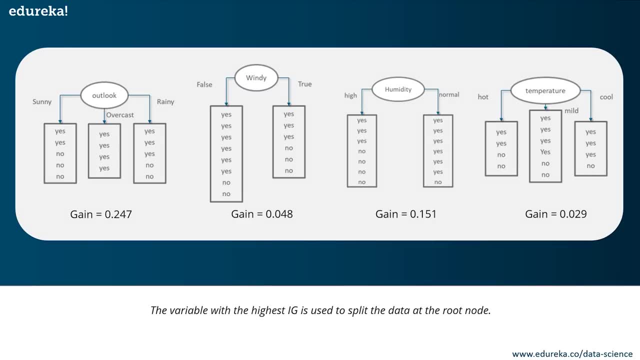 a value of 0.029, which is again very less. So what you can summarize from here is: if we look at the information gain for each of these variable, we'll see that for outlook, we have the maximum gain. Alright, we have 0.247, which is the highest information gain value, and you must always 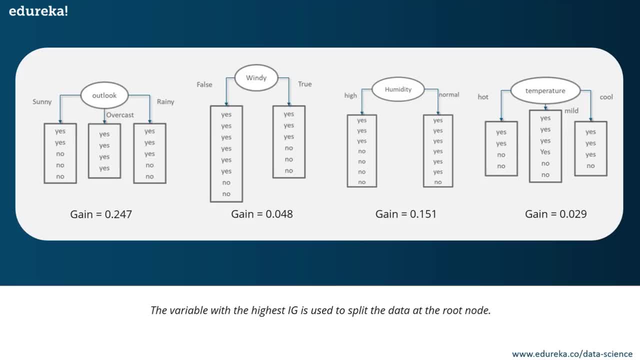 choose a variable with the highest information gain to split the data at the root node. So that's why we assign the outlook variable at the root node. Alright, so, guys, I hope this use case was clear. If any of you have doubts, please keep commenting those doubts. Now let's move on and 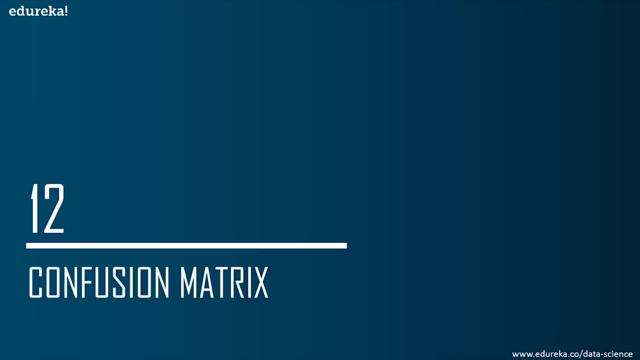 look at what exactly a confusion matrix is. Now, the confusion matrix is the last topic for descriptive statistics. Alright, after this I'll be running a short demo where I'll be showing you how you can calculate mean median mode and standard deviation variance, and all of those values. 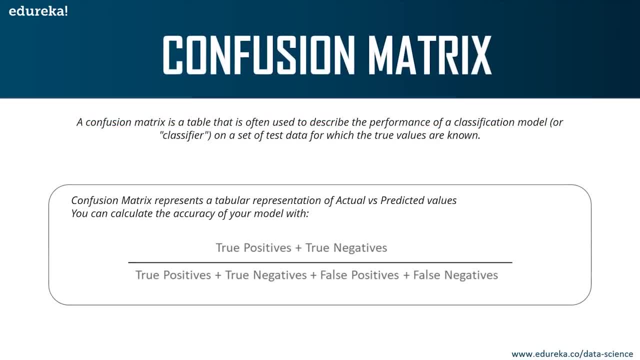 using R. Okay, so let's talk about confusion matrix. Now, guys, what is a confusion matrix? Now, don't get confused. this is not any complex topic Now. a confusion matrix is a matrix that is often used to describe the performance of a model. Alright, and this is specifically used for. 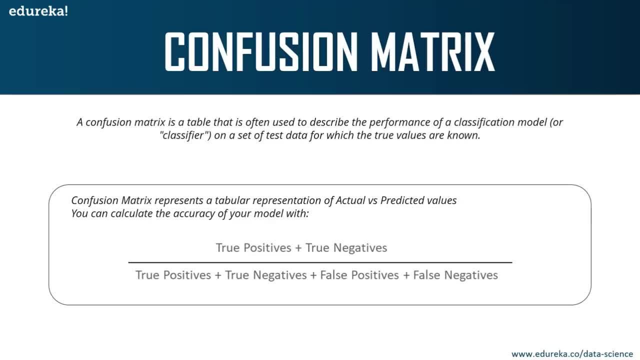 classification models or a classifier, and what it does is it will calculate the accuracy or it will calculate the performance of your classifier By comparing your actual results and your predicted results. Alright, so this is what it looks like: true positive plus true negative and all of that. Now, this is a little confusing. I'll get back to what 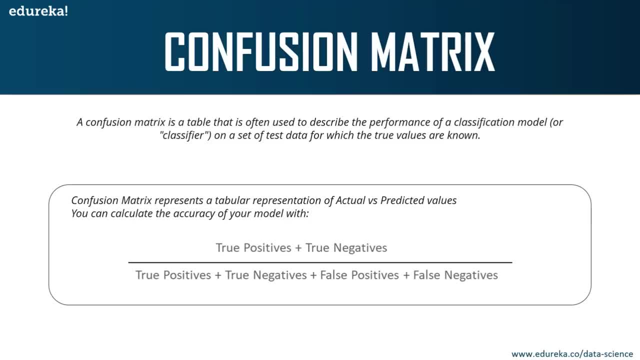 exactly true, positive, true, negative and all of this stands for. For now, let's look at an example and let's try and understand what exactly confusion matrix is. So, guys, I made sure that I put examples after each and every topic, because it's important you understand the practical part of 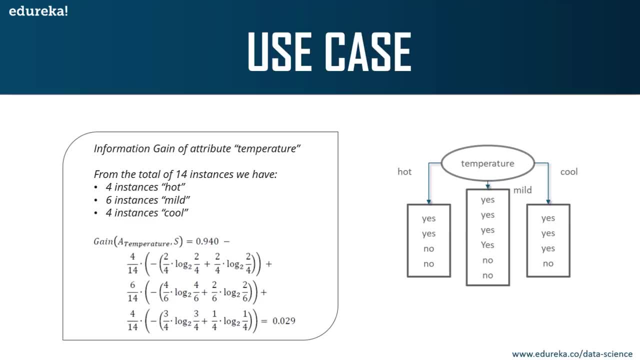 and one instance of no. All right now, when you calculate the information gain for this attribute, you'll get a value of 0.029, which is again very less. So what you can summarize from here is: if you look at the information gain, 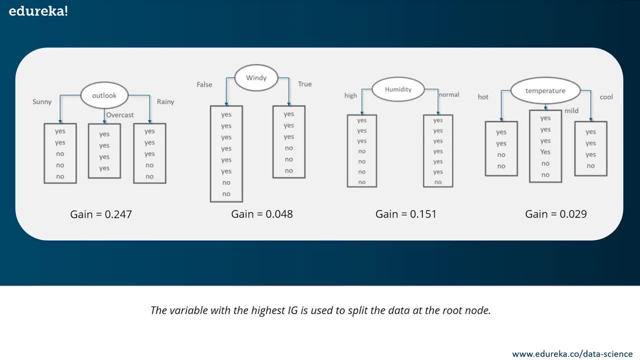 for each of these variables, you'll see that for outlook, we have the maximum gain. all right, we have 0.247, which is the highest information gain value, And you must always choose a variable with the highest values, highest information gain, to split the data at the root node. so that's why we assign the outlook. 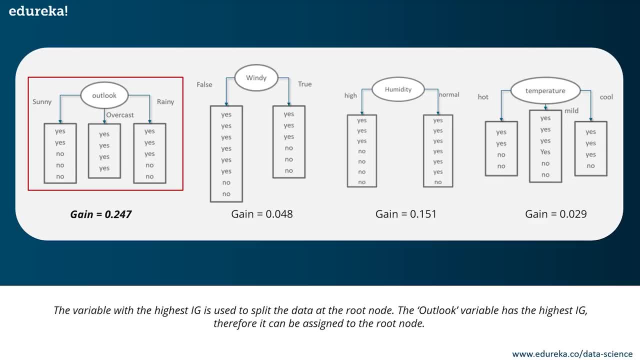 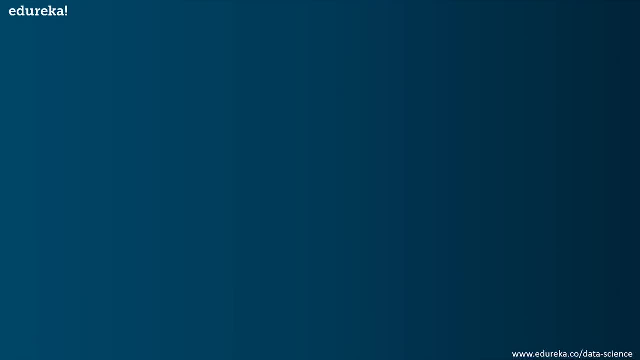 variable at the root node. all right, so, guys, i hope this use case was clear. if any of you have doubts, please keep commenting those doubts. now let's move on and look at what exactly a confusion matrix is. now. the confusion matrix is the last topic for descriptive statistics. all right, after. 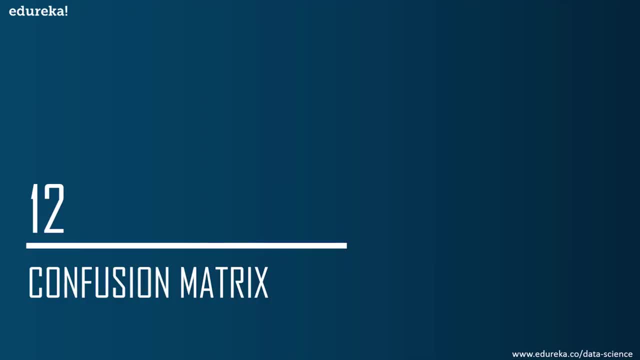 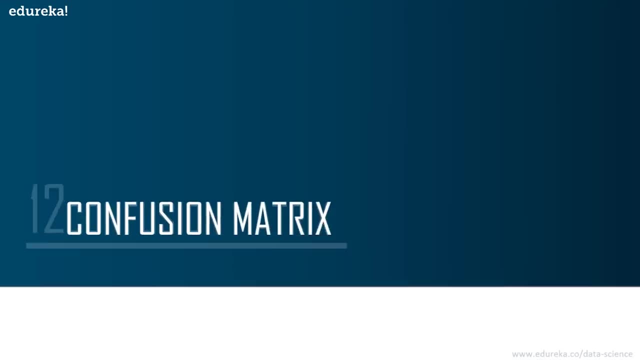 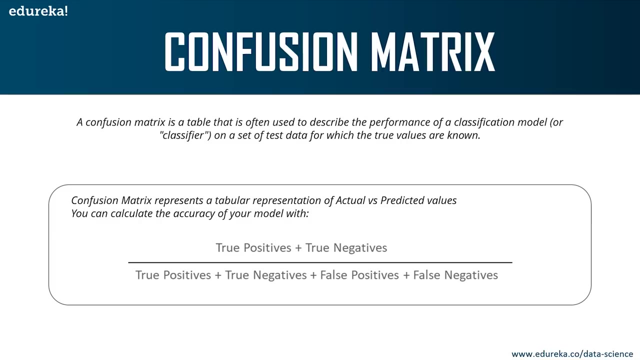 this. i'll be running a short demo where i'll be showing you how you can calculate mean, median mode and standard deviation variance and all of those values by using r. okay, so let's talk about confusion matrix now, guys, what is a confusion matrix? now, don't get confused, this is not any. 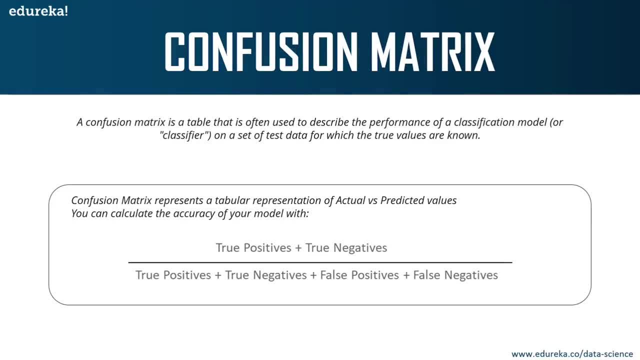 complex topic now confusion. matrix is a matrix that is often used to describe the performance of a model. all right, and this is specifically used for classification models or a classifier, and what it does is it will calculate the accuracy or it will calculate the performance of your classifier by comparing your actual results and 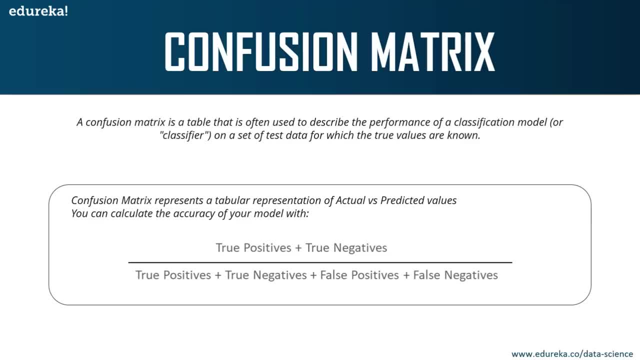 your predicted results. all right, so this is what it looks like: true positive plus true negative and all of that. now, this is a little confusing. i'll get back to what exactly true positive, true negative and all of this stands for. for now, let's look at an example and let's try and understand. 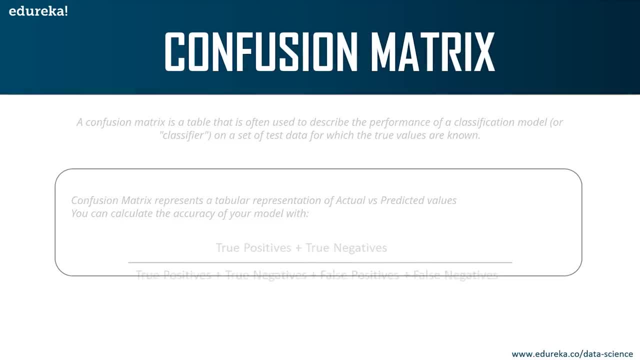 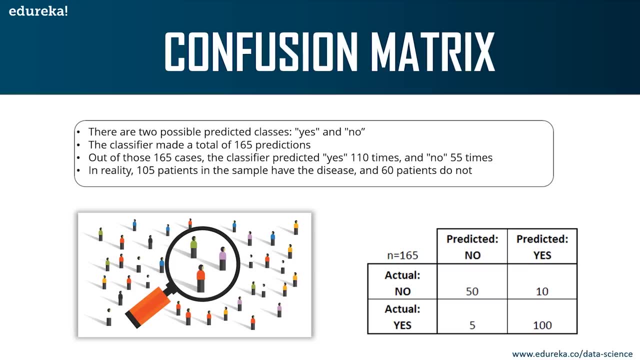 what exactly confusion matrix is. so, guys, i made sure that i put examples after each and every topic because it's important you understand the practical part of statistics. all right, statistics has literally nothing to do with theory. you need to understand how calculations are done in statistics. okay, so here, what i've done is: um, now let's look at a small use case. okay, let's consider. 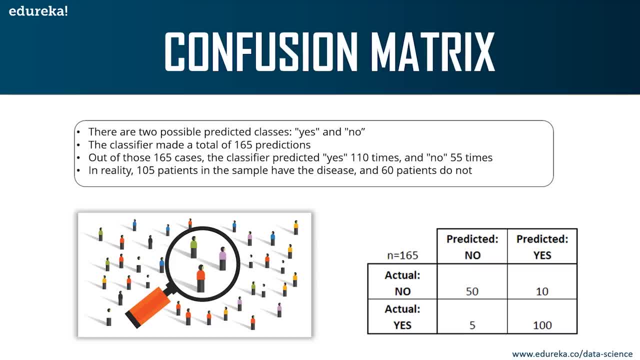 statistics. Alright, statistics has literally nothing to do with theory. You need to understand how calculations are done in statistics. Okay, so here, what I've done is now let's look at a small use case. Okay, let's consider that you're given data about 165 patients, out of which 105 patients have a disease and the remaining 50. 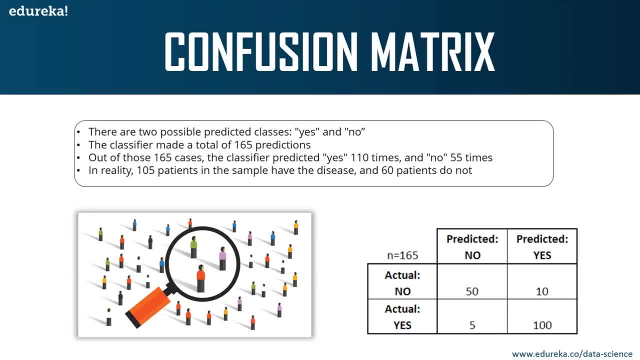 patients don't have a disease. Okay, so what you're going to do is you'll build a classifier that predicts by using these 165 observations. You'll feed all of these 165 patients and you're going to give 165 observations to your classifier and it will predict the output every time a new patient's. 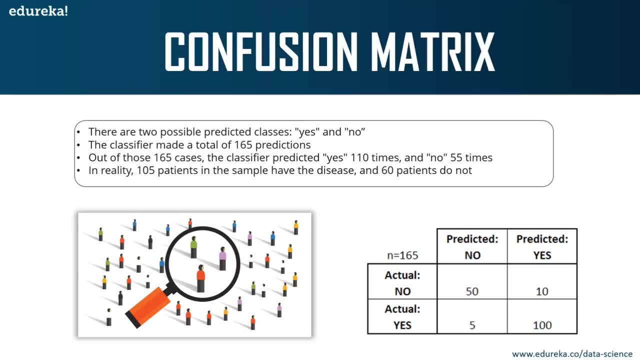 detail is fed to the classifier. Alright. now, out of these 165 cases, let's say that the classifier predicted yes 110 times and no 55 times. Alright, so yes basically stands for yes- the person has a disease, and no stands for no- the person does not have a disease. Alright, that's pretty self-explanatory. 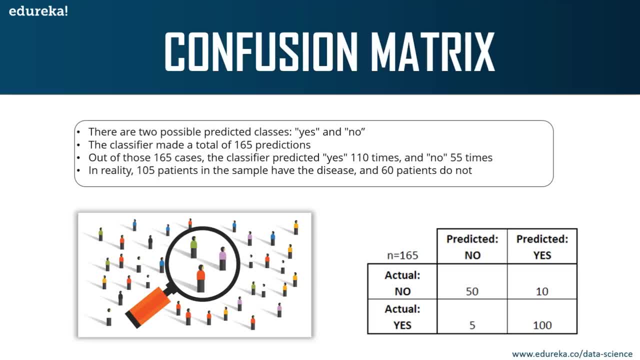 and it predicts that 110 times the patient has a disease and 55 times that, no, the patient doesn't have a disease. However, in reality, only 105 patients in the sample have the disease and 60 patients do not have the disease, Right? so how do you calculate the accuracy of your model? You? 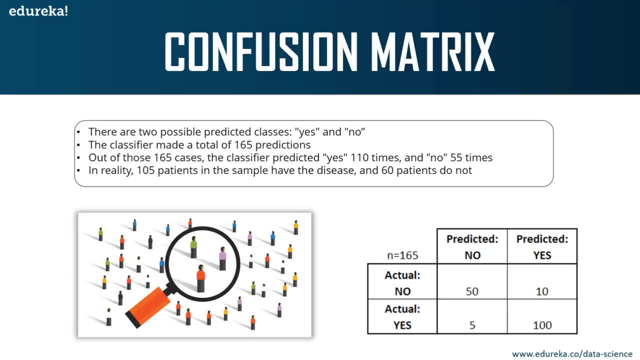 basically build the confusion matrix. Alright, this is how the matrix looks like and basically denotes the total number of observations that you have, which is 165 in our case. Actual denotes the actual values in the data set and predicted denotes the predicted values by the classifier. So the actual value is no here and the predicted value is no here. So your classifier was. 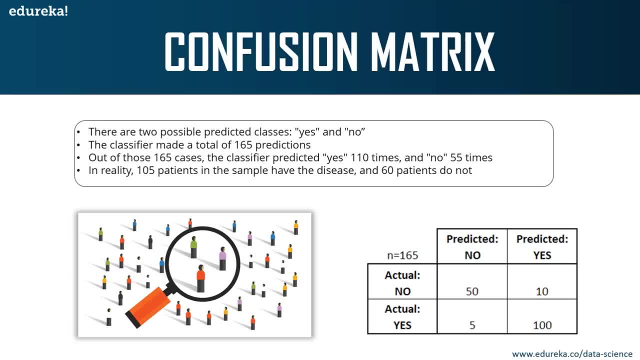 correctly able to classify 50 cases as no Alright, since both of these are no. so 50 it was correctly able to classify, but 10 of these cases it incorrectly classified, Meaning that your actual value here is no, but your classifier predicts that it is no Alright. so you can see that the 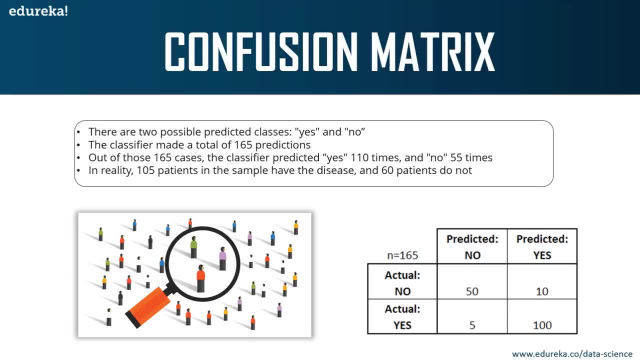 value here is no, but your classifier predicted it as yes. Alright, that's why this 10 over here. Similarly, it wrongly predicted that five patients do not have diseases, whereas they actually did have diseases, and it correctly predicted 100 patients which had the disease. Alright, I know. 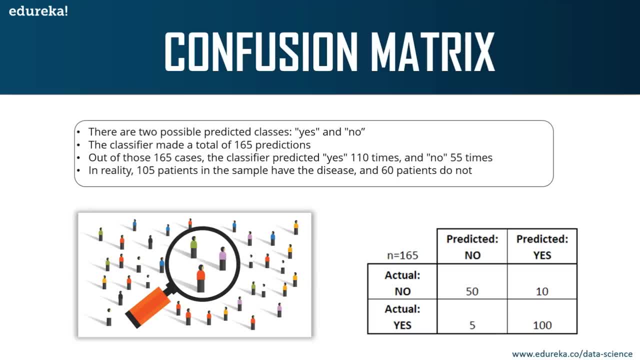 that you're given data about 165 patients, out of which 105 patients have a disease and the remaining 50 patients don't have a disease. okay, so what you're going to do is you'll build a classifier that predicts by using these 165 observations. you'll feed all of these 165 observations to 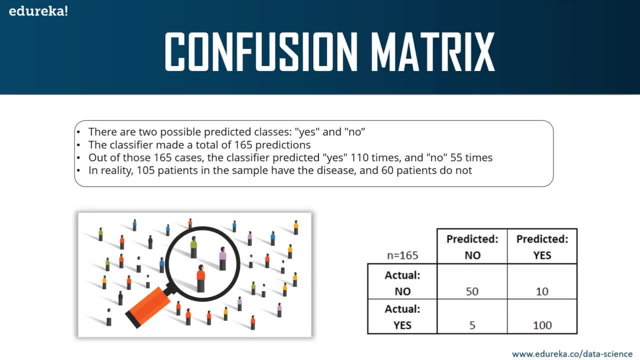 your classifier and it will predict the output every time a new patient's detail is fed to the classifier. right now, out of these 165 cases, let's say that the classifier predicted yes 110 times and no 55 times. all right, so yes basically stands for yes- the person has a disease, and no stands for. 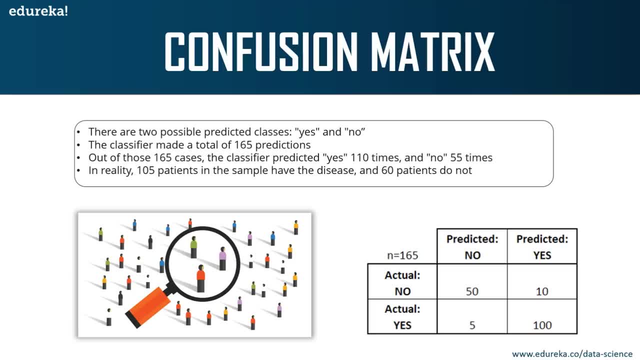 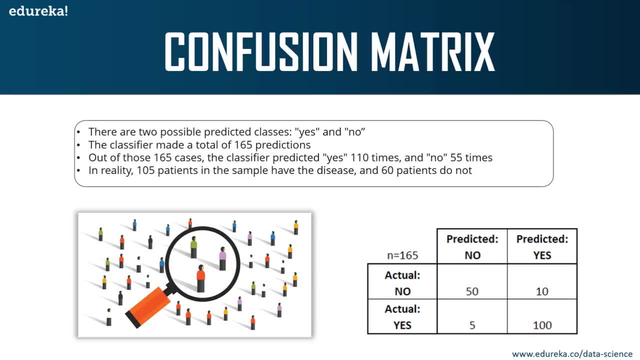 disease. however, in reality, only 105 patients in the sample have the disease and 60 patients do not have the disease, right? so how do you calculate the accuracy of your model? you basically build the confusion matrix, all right. this is how the matrix looks like and basically denotes the total number. 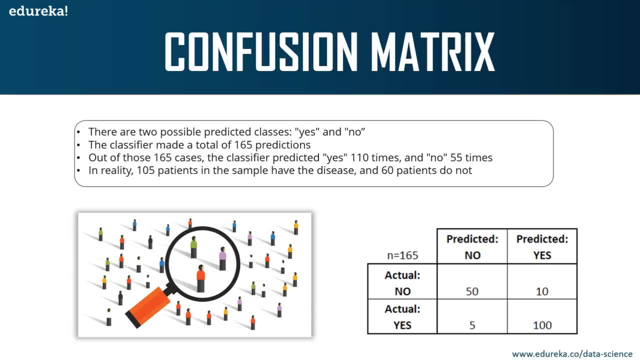 of observations that you have, which is 165 in our case. actual denotes the actual values in the data set and predicted denotes the predicted values by the classifier. so the actual value is no here and the predicted value is no here. so your classifier was correctly able to classify 50 cases as no. 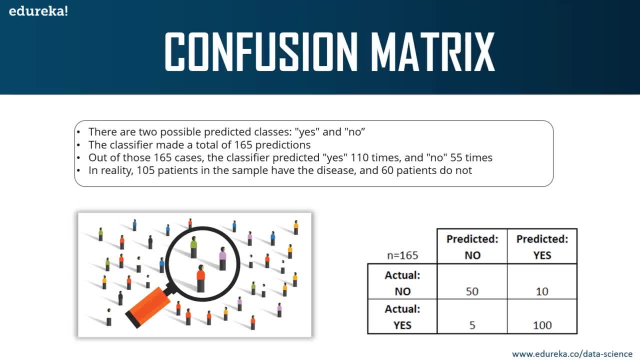 all right, since both of these are no, so 50, it was- is correctly able to classify but 10 of these cases. it incorrectly classified, meaning that your actual value here is no, but your classifier predicted it as yes. all right, that's why there's 10 over here. similarly, it wrongly predicted that five patients do not have diseases. 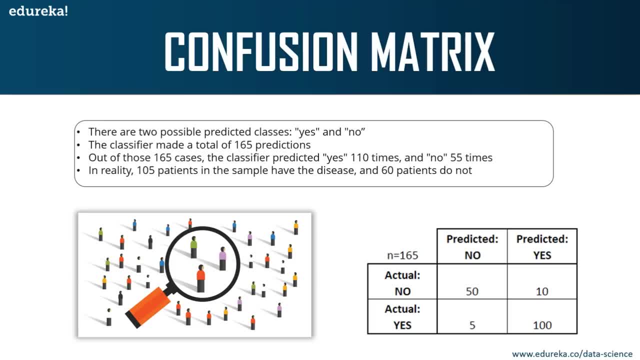 whereas they actually did have diseases, and it correctly predicted 100 patients which had the disease. all right, i know this is a little bit confusing, but if you look at these values, no, no, 50, meaning that it correctly predicted 50 values. no, yes, means that it wrongly predicted yes for. 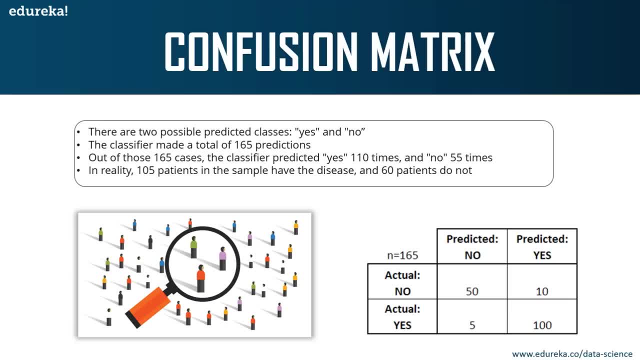 this is a little bit confusing, but if you look at these values, no, no, 50, meaning that it correctly predicted 50 values. No, yes, means that it wrongly predicted yes for the values that it was supposed to. Alright, now, what exactly is this? true, positive, true, negative, and all of that. I'll tell you what. 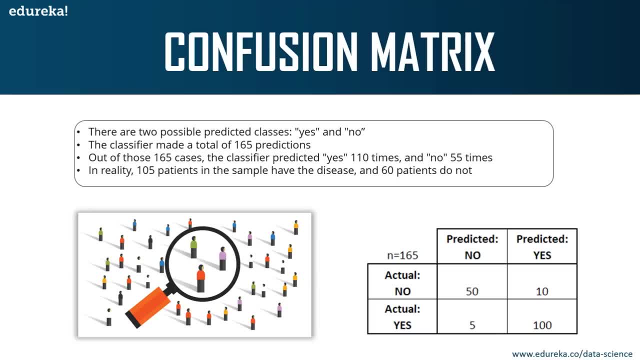 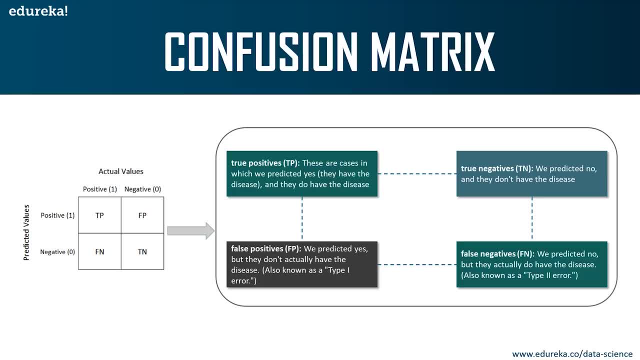 Meaning that this is correct. False positive is we predicted yes, but they do not actually have the disease. Alright, this is also known as type 1 error. False negative is we predicted no, but they actually do not have the disease. So, guys, basically false negative and true negatives are basically: 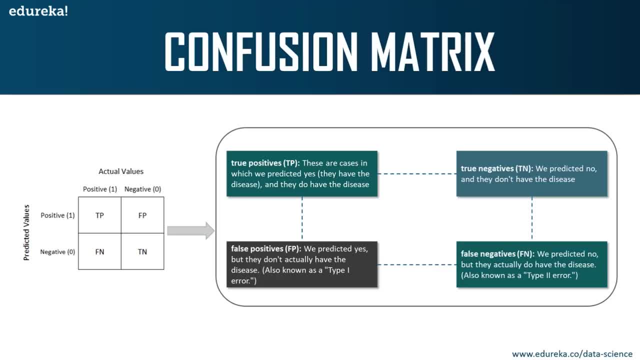 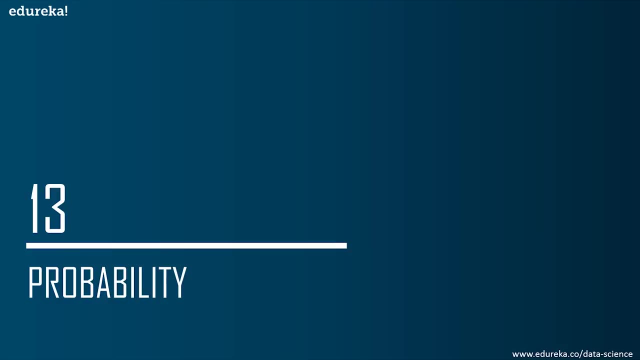 correct classifications. Alright, so this was confusion matrix and I hope this concept is clear. Again, guys, if you have doubts, please comment your doubts in the comment section. So, guys, that was descriptive statistics. Now, before we go to probability, I promised you all that we'll run a small demo in R. Alright, we'll try and understand how mean median mode works. 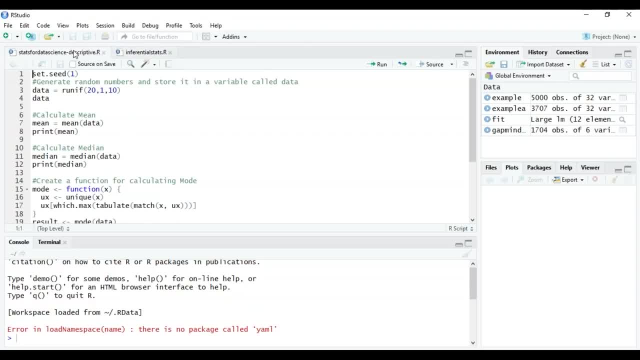 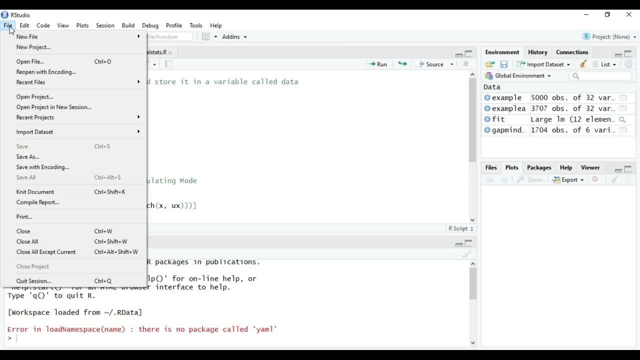 in R. Okay, so let's do that first. So, guys, again, what we just discussed so far was descriptive statistics. Alright, next we're going to discuss probability and then we'll move on to inferential statistics. Okay, inferential statistics is basically the second type of statistics. 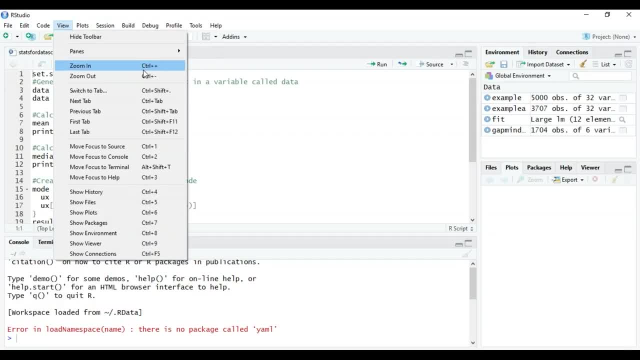 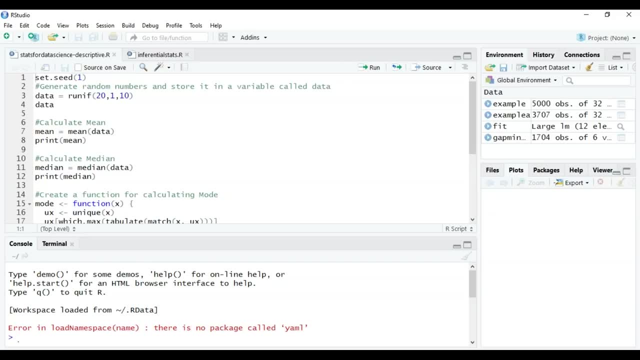 Okay, now, to make things more clearer for you, let me just zoom in. So, guys, it's always best to perform practical implementations in order to understand the concepts in a better way. Okay, so here we'll be executing a small demo that will show you how to. 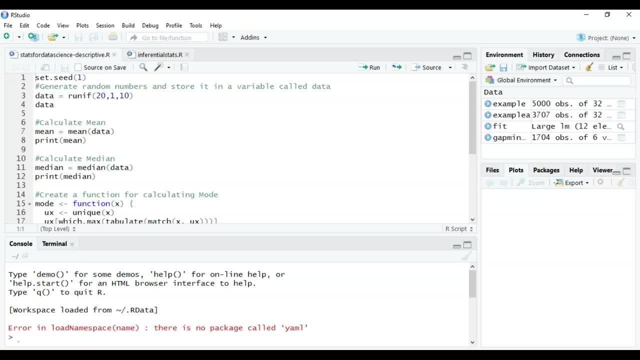 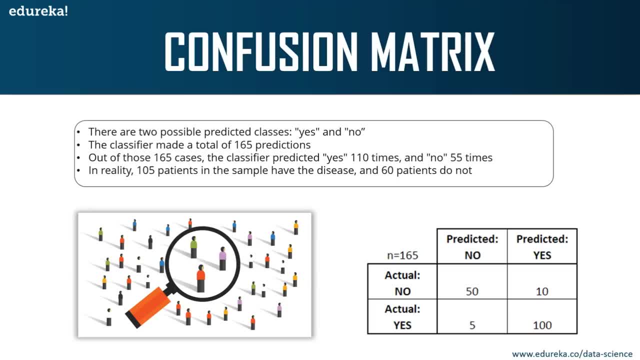 the values that it was supposed to predict? no, all right. now, what exactly is this? true positive, true, negative? and all of that. i'll tell you what exactly it is so true? positive are the cases in which we predicted a yes and they do not actually have the disease. all right, so it is. 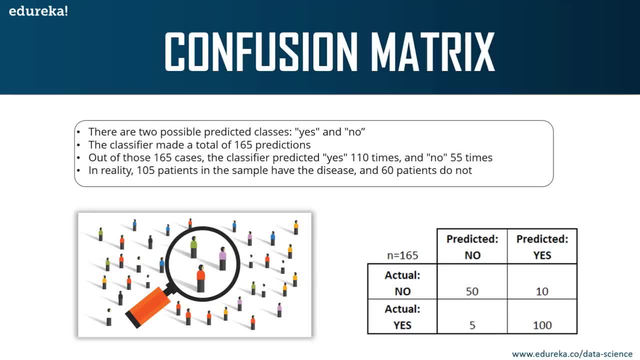 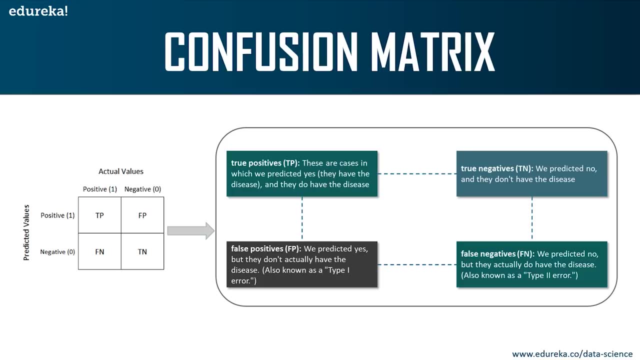 basically this value. all right, we predicted a yes here, even though they did not have the disease. so we have 10 true positives, right. similarly true negative: is we predicted no and they don't have the disease, meaning that this is correct. false positive is we predicted yes, but they do not actually have the disease. all right, this is. 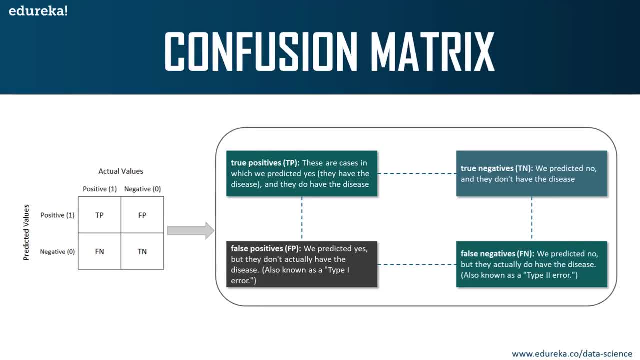 also known as type 1 error. false negative is we predicted? no, but they actually do not have the disease. so, guys, basically false negative and true negatives are basically correct classifications, all right. so this was confusion matrix and i hope this concept is clear again, guys, if you have, 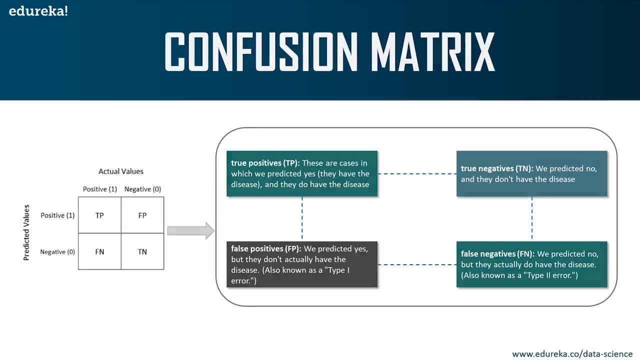 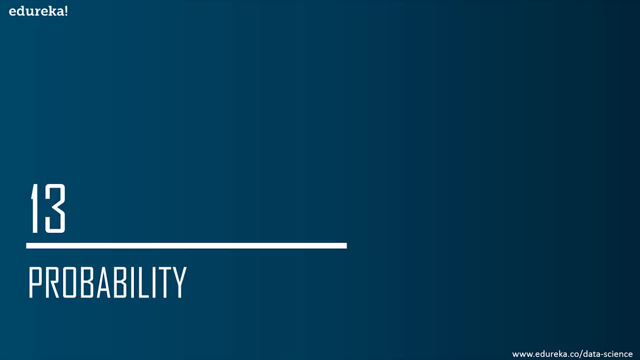 doubts. please comment your doubts in the comment section. so, guys, that was descriptive statistics. now, before we go to probability, i promised you all that we'll run a small demo in r. all right, we'll try and understand how mean median mode works in r okay, so let's do that first. 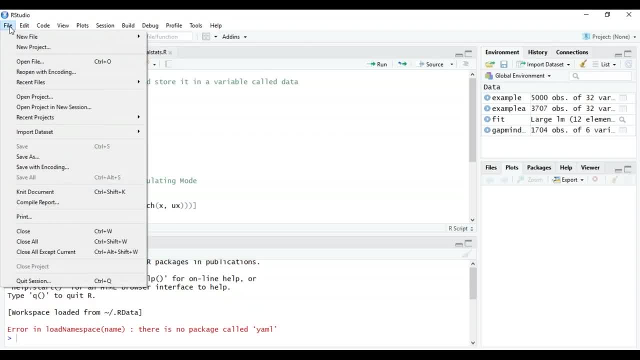 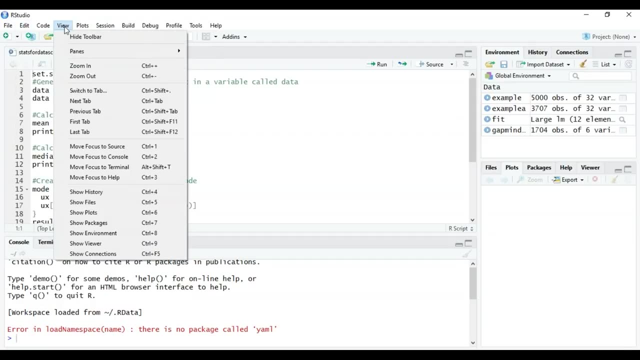 so, guys, again, uh, what we just discussed so far was descriptive statistics. all right, next we're going to discuss probability and then we'll move on to inferential statistics. okay, inferential statistics is basically the second type of statistics. okay, now, to make things more clearer for you, let me just zoom in. 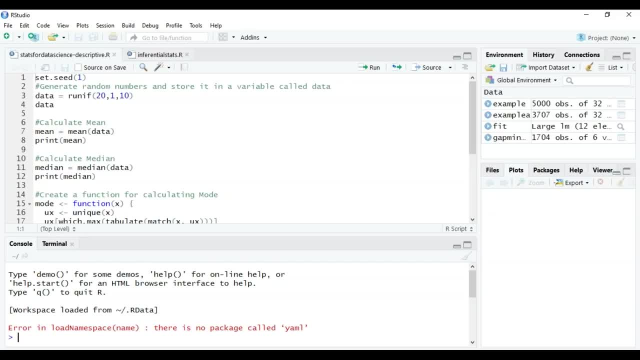 so, guys, it's always best to perform practical implementations in order to understand the concepts in a better way. okay, so here we'll be executing a small demo that will show you how to calculate the mean median mode of the simulation mode- variance, standard deviation- and how to study the variables by plotting a histogram. 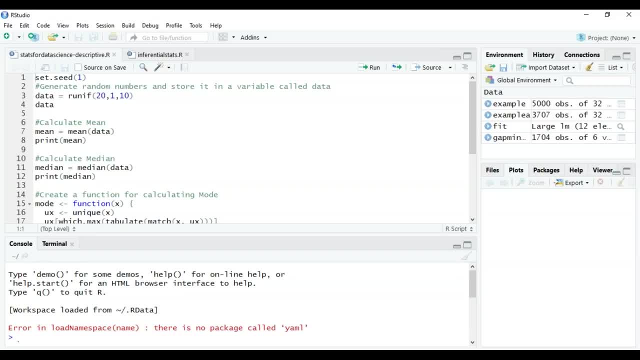 okay, don't worry if you don't know what a histogram is. it's basically a frequency plot. there's no big science behind it. all right, this is a very simple demo, but it also forms a foundation that every machine learning algorithm is built upon. okay, you can say that most of the machine 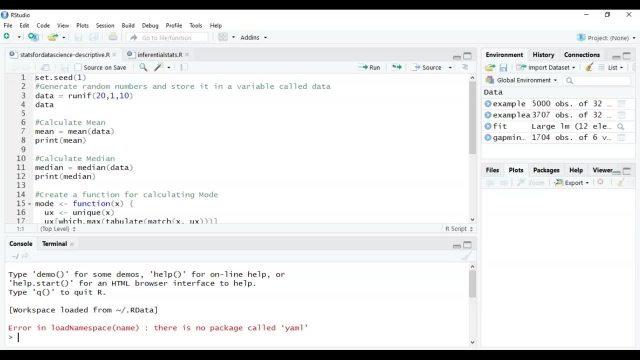 Let's do that. So let's go ahead and bring over a frequency plot. There's no big science behind it. Alright, this is a very simple demo, but it also forms the foundation that every machine learning algorithm is built upon. Okay, you can say that most of the machine learning algorithms out. 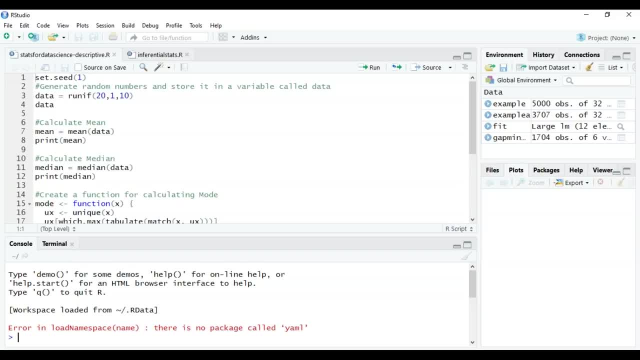 of all the machine learning algorithms and deep learning algorithms have this basic concept behind them. Okay, you need to know how mean, median mode and all of that is calculated. So, guys, I'm using the R language to perform this and I'm running this on R studio, for those of you who don't. 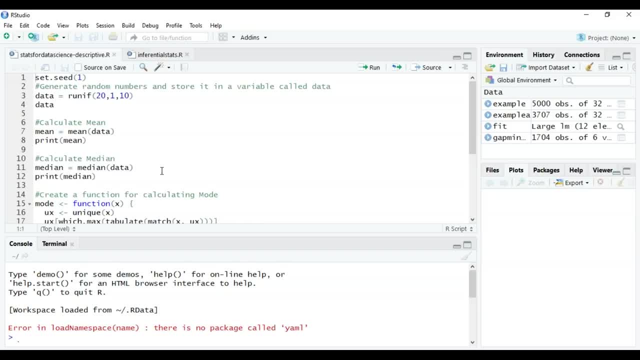 our language. I will leave a couple of links in the description box. you can go through those videos. so what we're doing is we're randomly generating numbers and we're storing it in a variable called data, right. so if you want to see the generated numbers, just run the line data, all right, this variable basically stores: 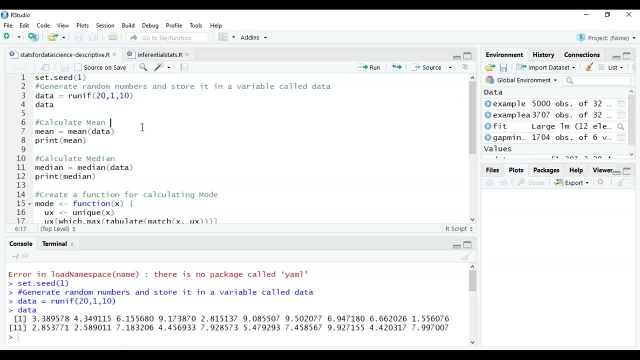 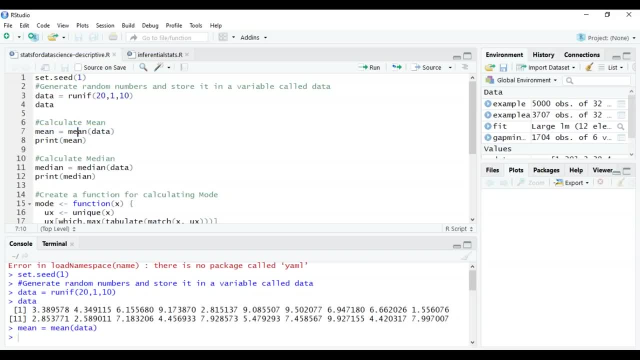 all our numbers. all right. now what we're going to do is we're going to calculate the mean. now, all you have to do in R is specify the word mean along with the data that you're calculating the mean of, and I was signed this whole thing into a. 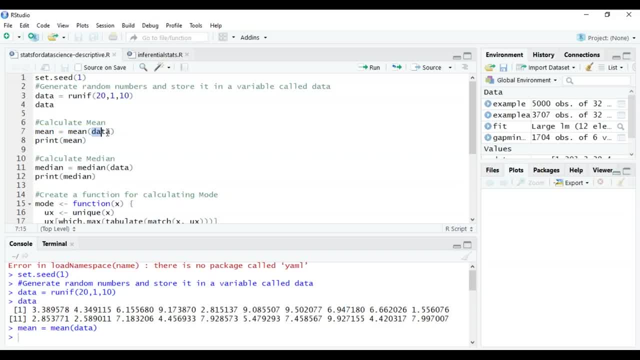 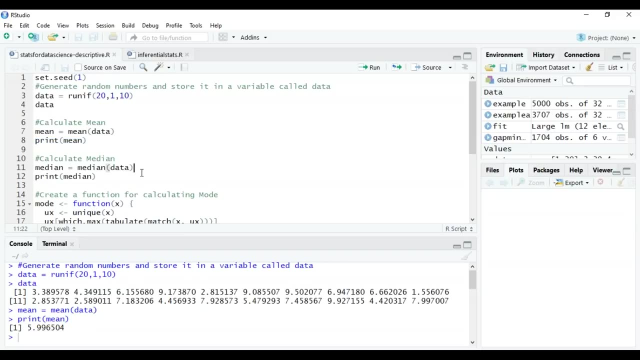 variable called mean, which will hold the mean value of this data. so now let's look at the mean. for that I've used a function called print and mean. all right, so our mean is around five point nine nine. okay, next is calculating the median. it's very simple, guys. all you have to do is use a function: median- all. 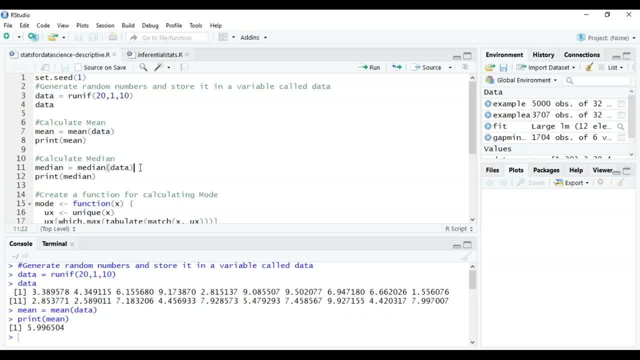 right and pass the data as a parameter to this function. that's all you have to do. so R provides functions for each and everything. all right, statistics is very easy when it comes to R, because R is basically a statistical language. okay, so all you have to do is just name the function, and that function is already in. 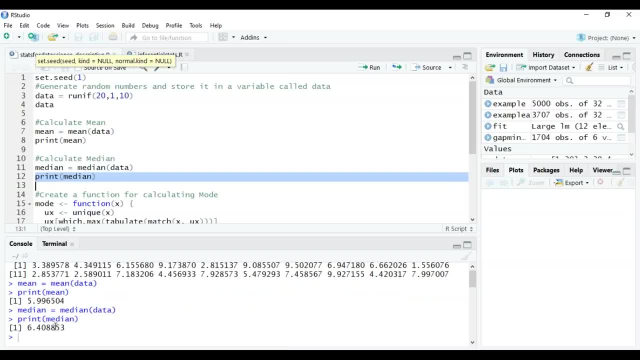 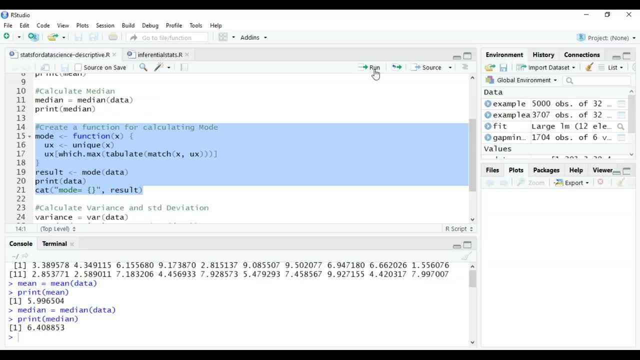 built in your R. okay, so your median is around six point four. so now let's go ahead and create a function called print, and we're going to. similarly, we'll calculate the mode. all right, let's run this function. I basically created a small function for calculating the mode. so, guys, this is our. 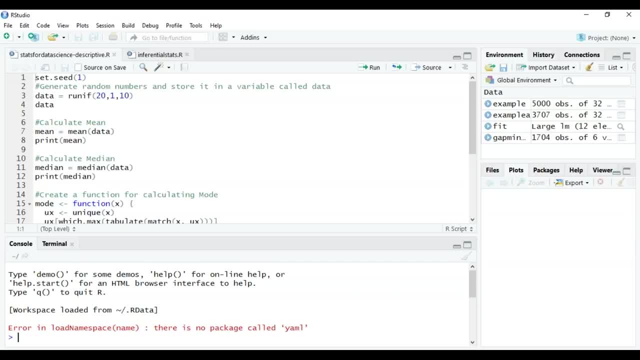 learning algorithms- actually all the machine learning algorithms and deep learning algorithms- have this basic concept behind them. okay, you need to know how mean median mode and all of that is calculated. so, guys, i'm using the r language to perform this and i'm running this on our studio. 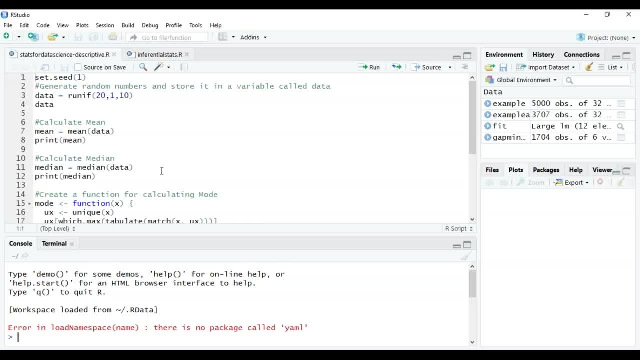 for those of you who don't know our language, i will leave a couple of links in the description box. you can go through those videos. so what we're doing is we're randomly generating numbers and we're storing it in a variable called data, right? so if you want to see the generated numbers, just 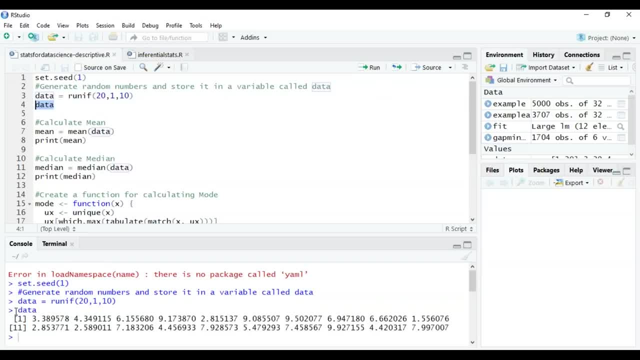 run the line data right. this variable basically stores all our numbers, all, right. now what we're going to do is we're going to calculate the mean. now all you have to do in r is specify the word mean along with the data that you're calculating the mean of, and i've assigned this whole thing into a variable called. 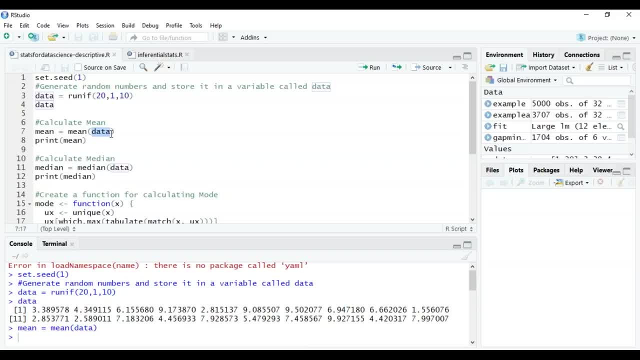 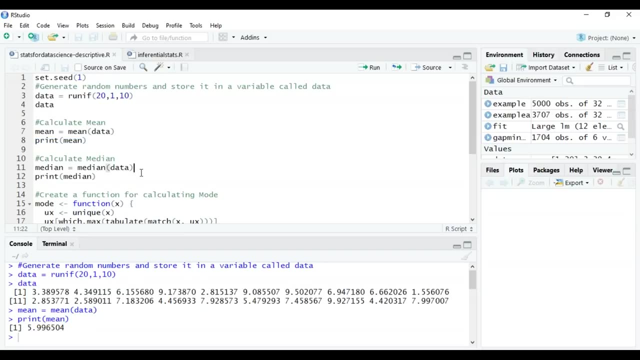 mean, which will hold the mean value of this data. so now let's look at the mean. for that, i've used a function called print and mean. now i've assigned this product to the term meant, the mean for my function. all right, so our main is around 5.99. okay, next is calculating the median. it's very simple, guys. 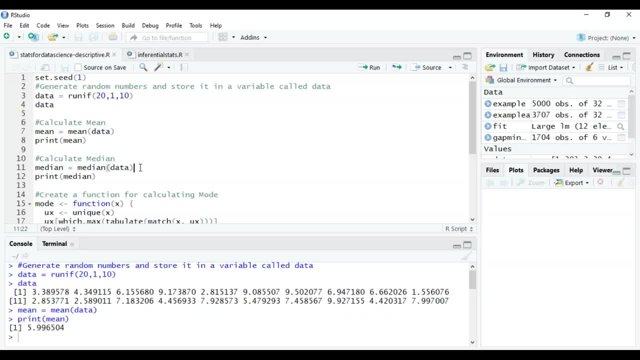 all you have to do is use a function- median- all right- and pass the data as a parameter to this function. that's all you have to do. so r provides functions for each and everything. all right, statistics is very easy when it comes to r, because r is basically a statistical language. 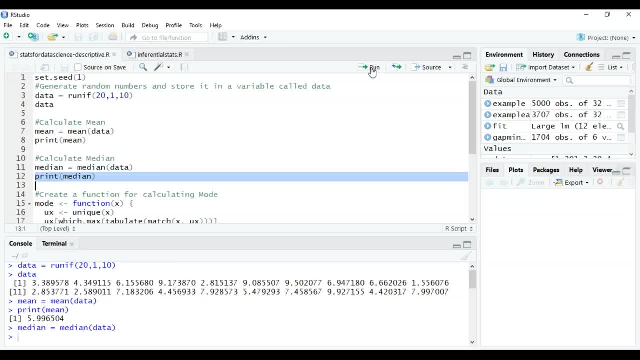 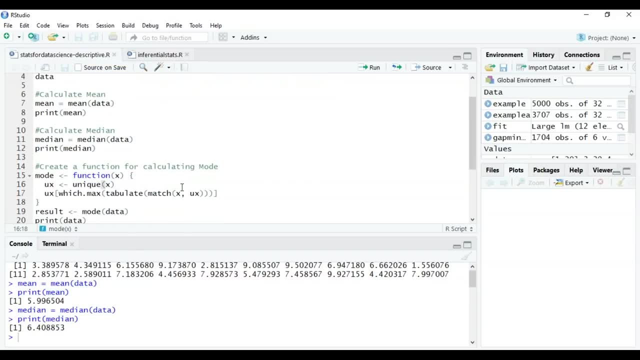 okay is just name the function, and that function is already inbuilt in your R. Okay, so your median is around 6.4.. Similarly, we'll calculate the mode. all right, Let's run this function. I basically created a small function. 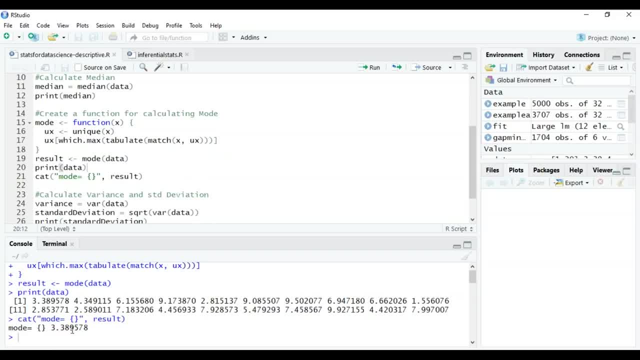 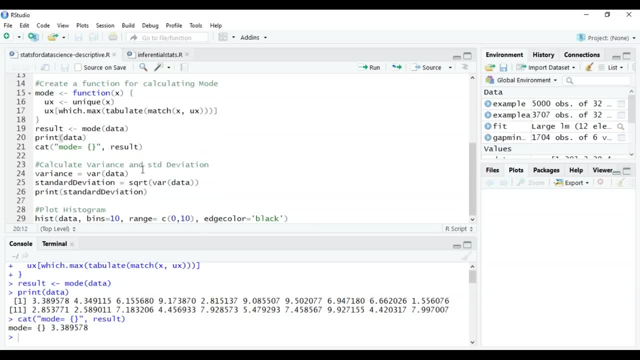 for calculating the mode. So, guys, this is our mode, meaning that this is the most recurrent value right Now. we're gonna calculate the variance and the standard deviation. For that, again, we have a function in R called as var. all right, 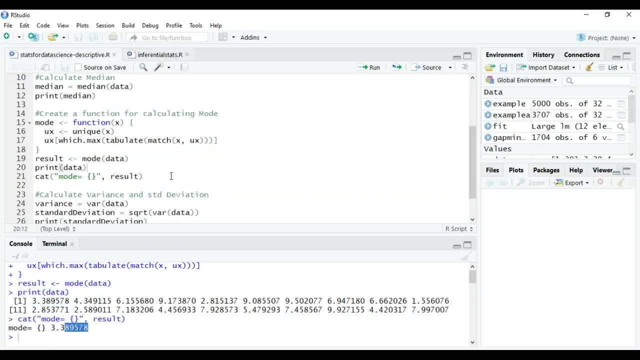 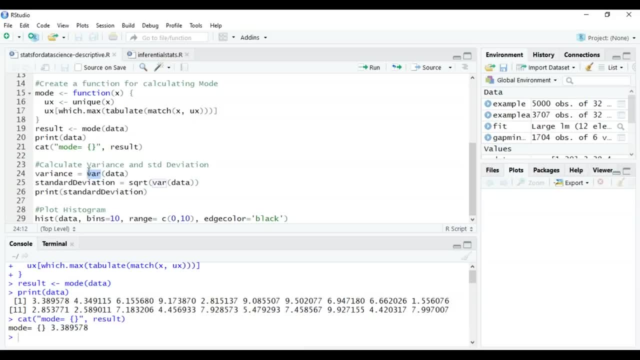 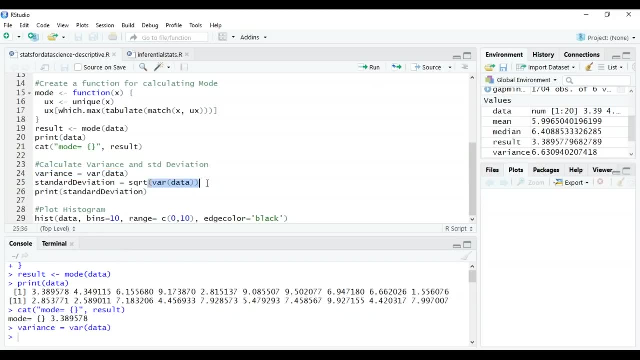 mode, meaning that this is the most recurrent value right now. we're going to calculate the variance and the standard deviation. for that, again, we have a function in R called as, where. all right, all you have to do is pass the data to that function. okay, similarly, we'll calculate the standard deviation. 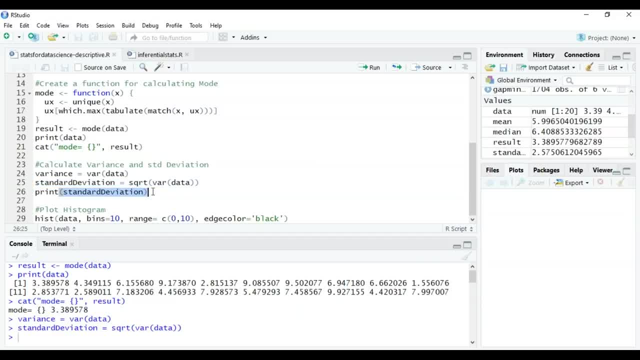 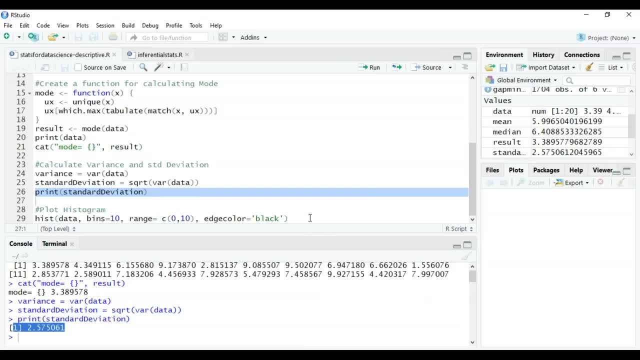 which is basically the square root of your warians. right now, we'll print the standard deviation, right? this is our standard deviation value. now, finally, we'll just plot a small histogram- histogram is nothing, but it's a frequency plot, all right- and show you how frequently your data point is. 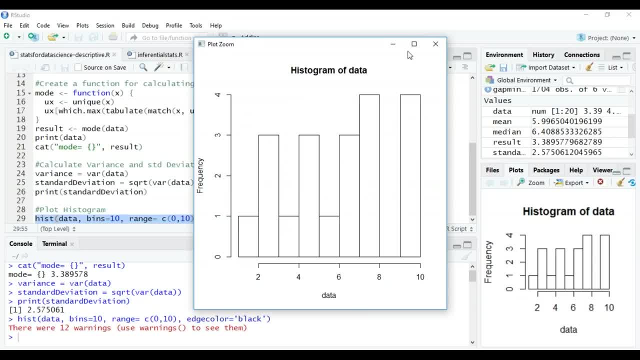 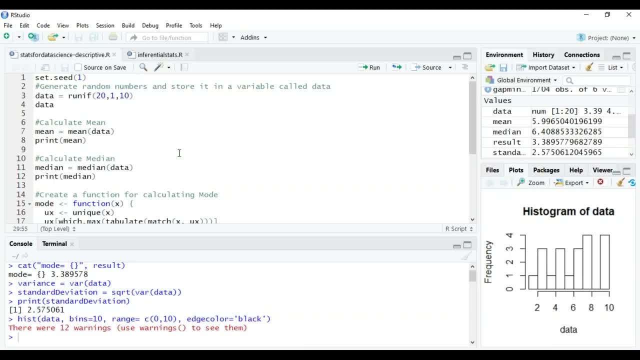 occurring. so this is the histogram that we've just created. it's quite simple in R, because R has a lot of packages and a lot of inbuilt functions that support statistics. all right, it is a statistic doubt, butlin R basically requires the match in combination with the relation of�. 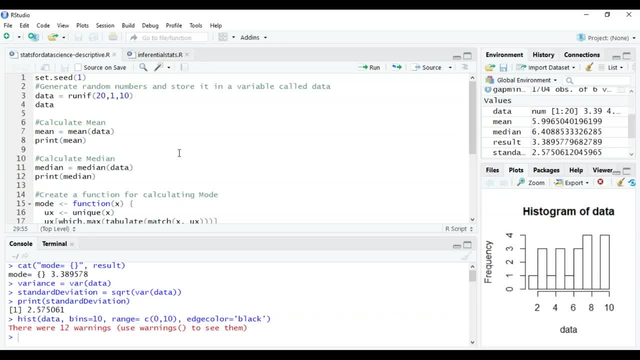 language that is mainly used by data scientists or by data analysts and machine learning engineers, because they don't have to sit and code these functions. All they have to do is they have to mention the name of the function and pass the corresponding parameters. So, guys, that was the. 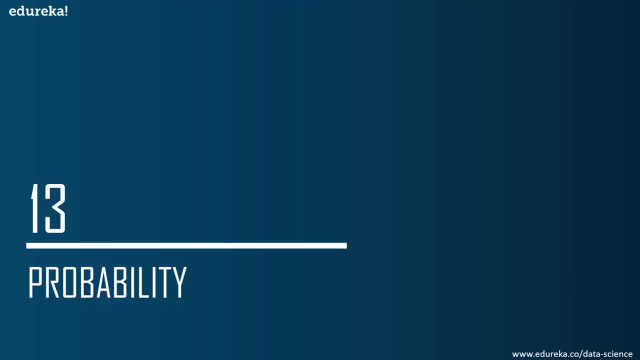 entire descriptive statistics module, and now we'll discuss about probability. Okay, so before we understand what exactly probability is, let me clear out a very common misconception. People often tend to ask me this question: what is the relationship between statistics and probability? So probability and statistics are related fields, All right, so probability is a mathematical method. 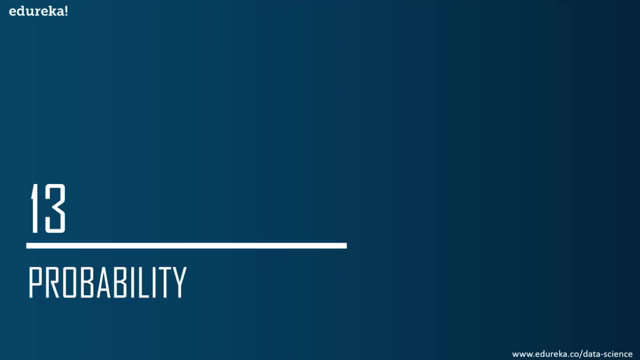 used for statistical analysis. Therefore, we can say that a probability and statistics are interconnected branches of mathematics that deal with analyzing the relative frequency of events. So they're very interconnected fields. and probability makes use of statistics and statistics makes use of probability. all right, they're very interconnected fields. so 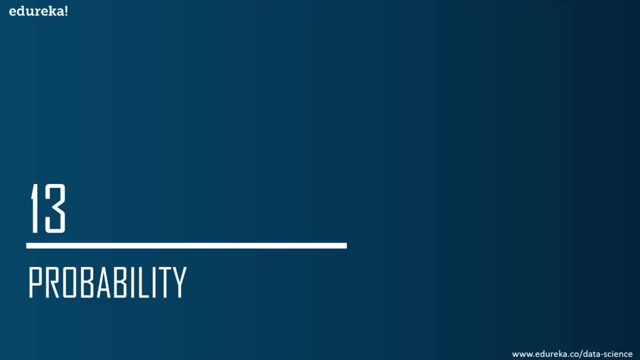 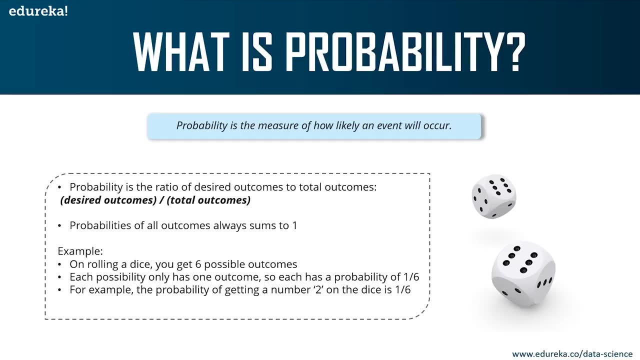 that is the relationship between statistics and probability. now let's understand what exactly is probability. so probability is the measure of how likely an event will occur. to be more precise, it is the ratio of desired outcome to the total outcomes. now, the probability of all outcomes always sum. 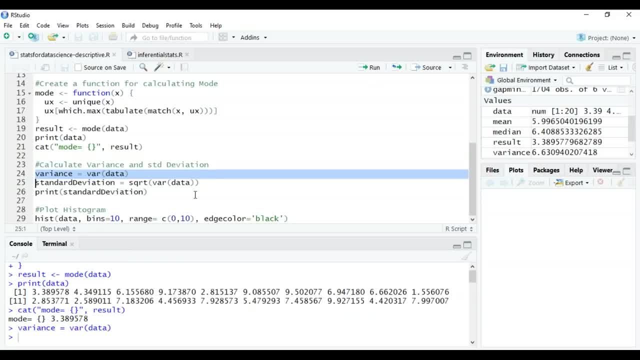 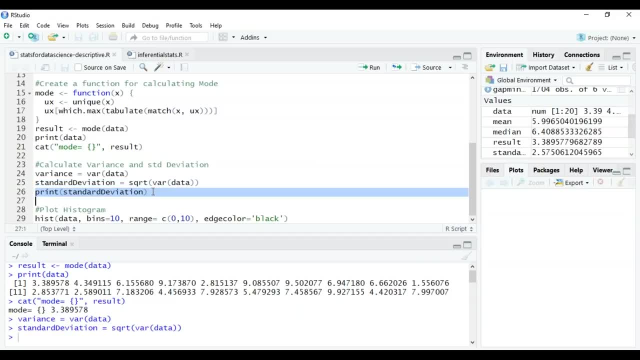 All you have to do is pass the data to that function. Okay. similarly, we'll calculate the standard deviation, which is basically the square root of your variance. right Now, we'll print the standard deviation. right, This is our standard deviation value. 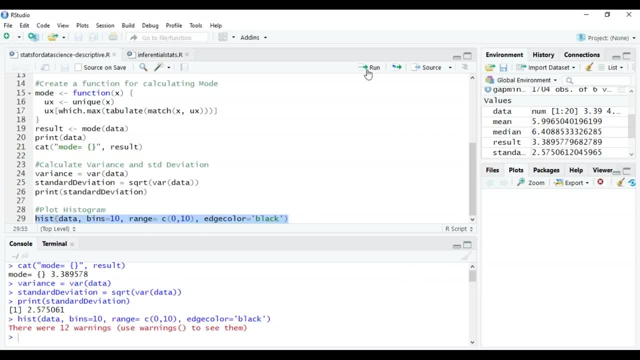 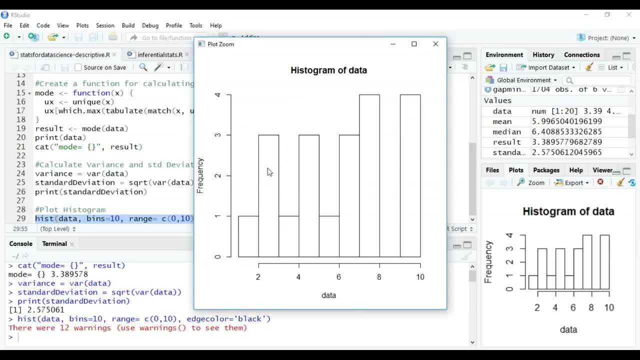 Now, finally, we'll just plot a small histogram. Histogram is nothing, but it's a frequency plot. all right, It'll show you how frequently a data point is occurring. So this is the histogram that we've just created. It's quite simple in R, because R has a lot of packages. 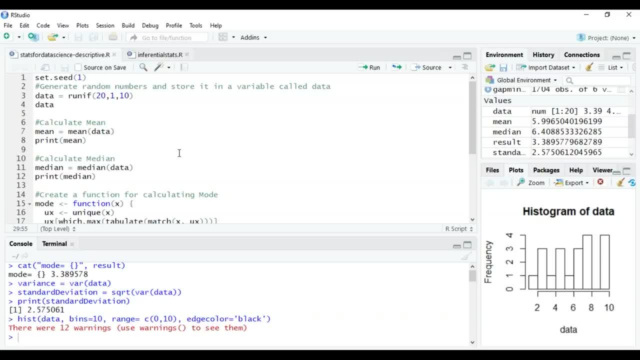 and a lot of inbuilt functions that support statistics. All right, it is a statistical language that is mainly used by data scientists or by data analysts and machine learning engineers, because they don't have to sit and code these functions. All they have to do is they have to mention. 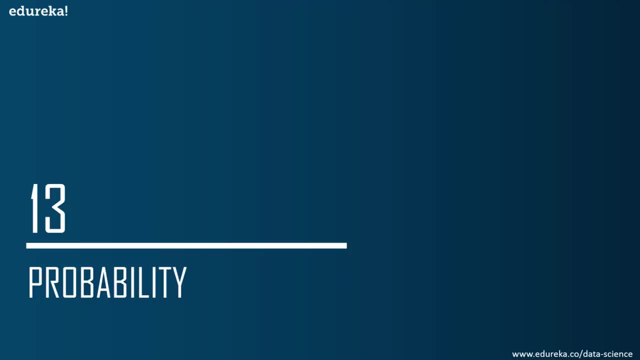 the name of the function and pass the corresponding parameters. So, guys, that was the entire descriptive statistics module, And now we'll discuss about probability. Okay, so before we end, before we understand what exactly probability is, let me clear out a very common misconception. 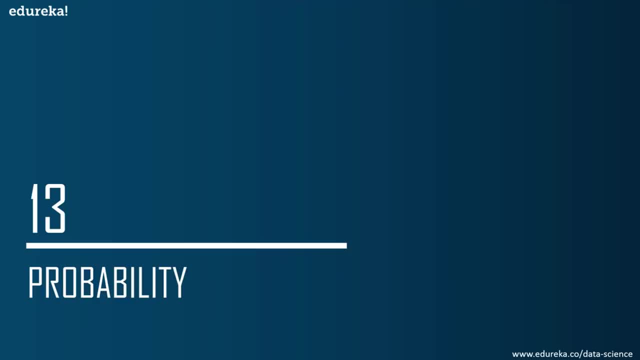 People often tend to ask me this question: what is the relationship between statistics and probability? So probability and statistics are related fields. all right, So probability is a mathematical method used for statistical analysis. Therefore, we can say that probability and statistics are interconnected branches of mathematics. 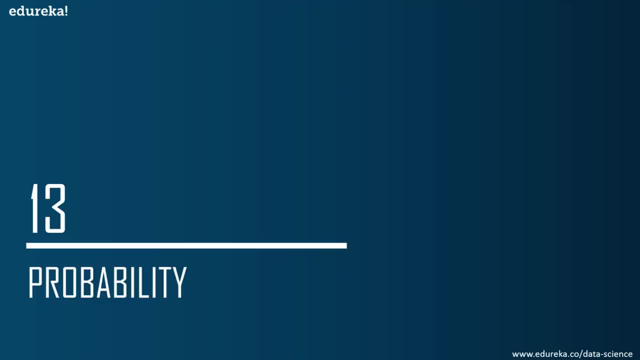 that deal with analyzing the relative frequency of events. So they're very interconnected fields. and probability makes use of statistics and statistics makes use of probability. All right, they're very interconnected fields. So that is the relationship between statistics and probability. Now let's understand what exactly is probability. 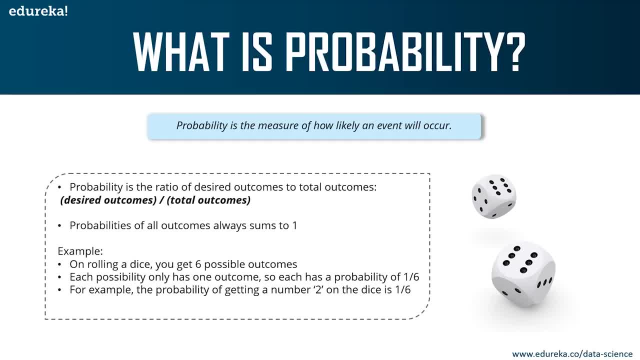 So probability is the measure of how likely an event will occur. To be more precise, it is the ratio of desired outcome to the total outcomes. Now, the probability of all outcomes always sum up to one. Now, the probability will always sum up to one. 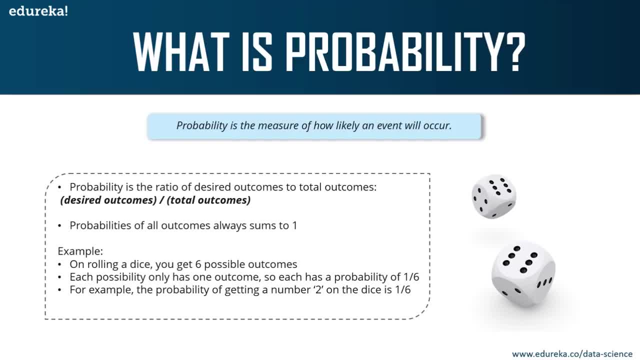 Probability cannot go beyond one. Okay, so either your probability can be zero, or it can be one, or it can be in the form of decimals, like 0.52 or 0.55, or it can be in the form of 0.5, 0.7, 0.9. 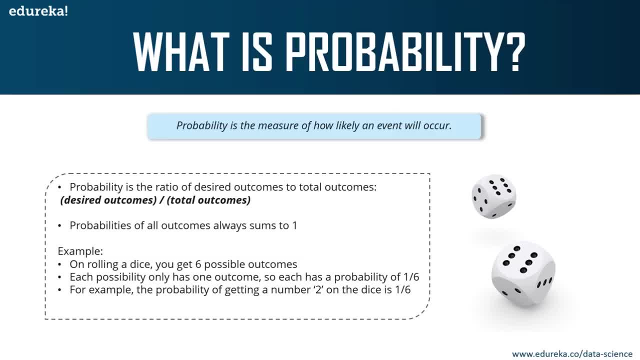 up to 1. now the probability will always sum up to 1. probability cannot go beyond 1. ok, so either your probability can be 0 or it can be 1, or it can be in the form of decimals like 0.52 or 0.55, or it can be in the form of 0.5, 0.7, 0.9, but its 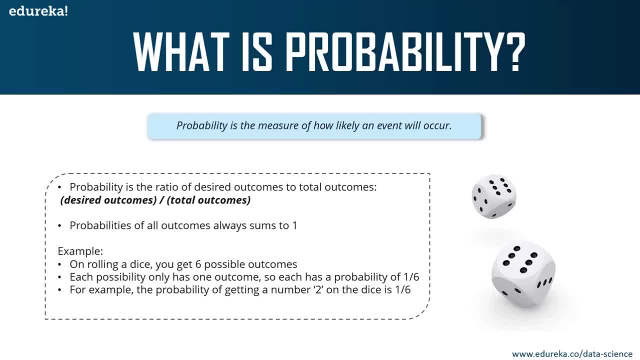 value will always stay between the range 0 and 1. ok, now the famous example of probability is rolling a dice example. so when you roll a dice, you get six points, and if you roll a dice, you get six points. and if you roll a dice, you get. 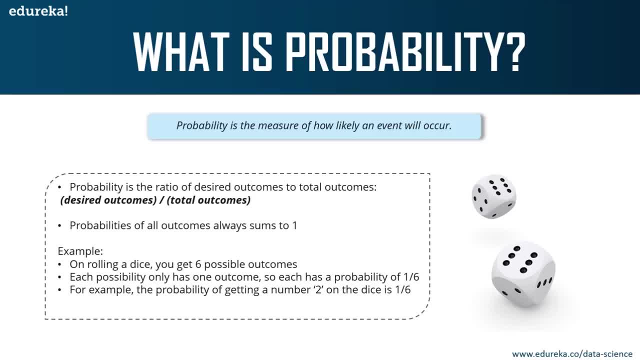 six possible outcomes. right, you get 1, 2, 3, 4 and 5- 6 phases of a dice. now, each possibility only has one outcome. so what is the probability that, on rolling a dice, you'll get 3? the probability is 1 by 6. right, because there's only one phase. 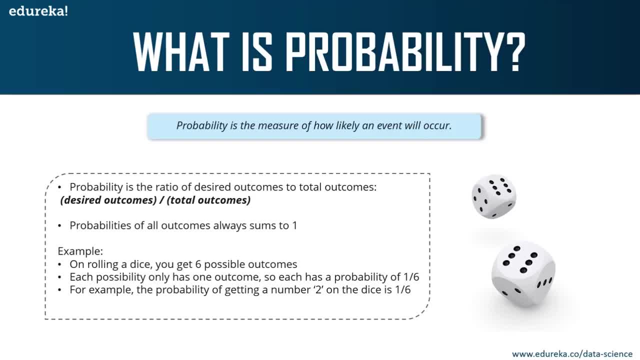 which has the number 3 on it. out of 6 phases, there's only one phase which has the number 3. so the probability of getting 3 when you roll a dice is 1 by 6. similarly, if you want to find the probability of getting 3, then you have to find the probability of getting 3. 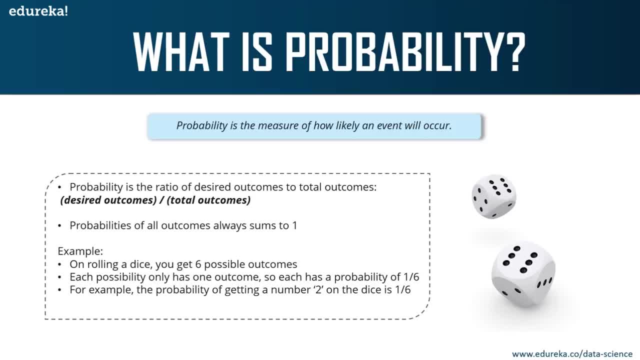 then you have to find the probability of getting 3. then you have to find the probability of getting a number 5. again, the probability is going to be 1 by 6, all right, so all of this will sum up to 1, all right. so, guys, this is exactly what probability is. it's a very simple. 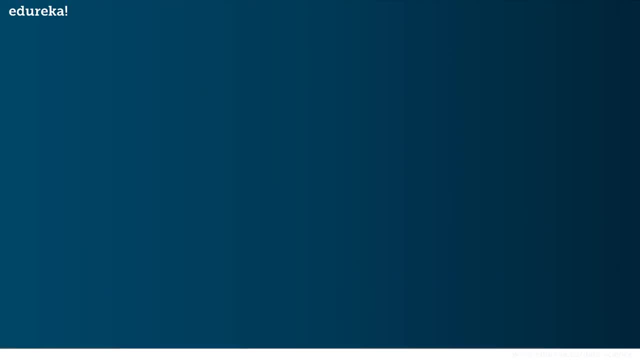 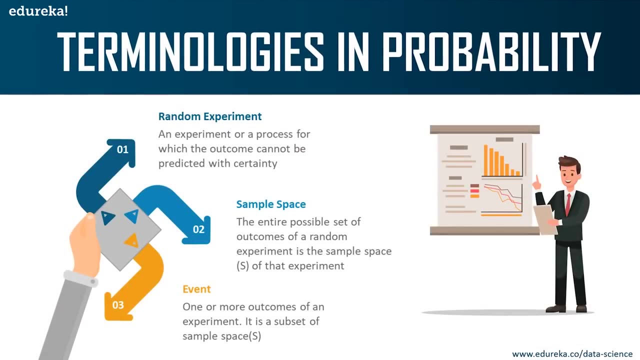 concept. we all learnt it in 8th standard onwards. right now, let's understand the different terminologies that are related to probability. now there are three terminologies that you often come across when we talk about probability. we have something known as the random experiment. okay, it's basically an 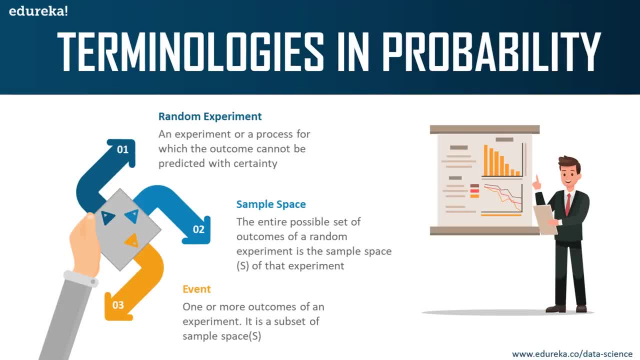 experiment or a process for which the outcomes cannot be predicted with certainty. all right, that's why you use probability. you're going to use probability in order to predict the outcome with some sort of certainty. sample space is the entire possible set of outcomes of a random experiment. an 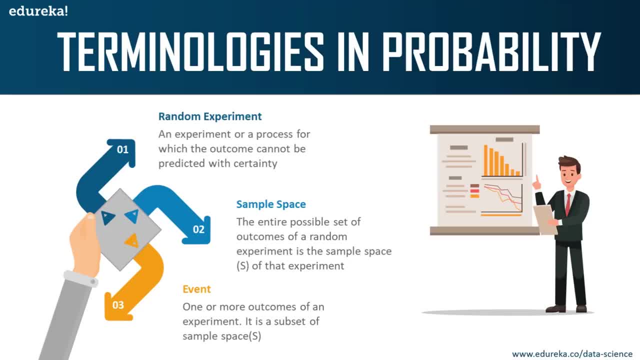 event is one or more outcomes of an experiment. so if you consider the example of rolling a dice- now let's say that you want to find out the probability of getting a 3- then you have to find the probability of getting 3 or 2 when you roll a dice. okay, so finding this probability is the random. 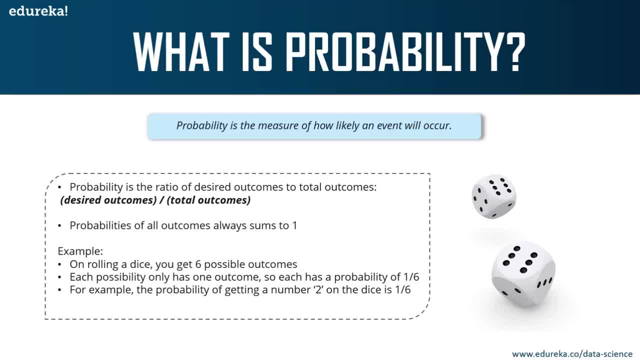 but its value will always stay between the range zero and one. Okay, now the famous example of probability is rolling a dice example. So when you roll a dice, you get six possible outcomes. Right, you get one, two, three, four and five. 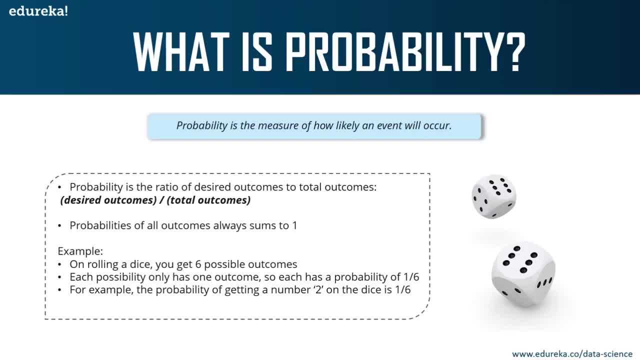 six phases of a dice. Now each possibility only has one outcome. So what is the probability that on rolling a dice, you'll get three? The probability is one by six, right, Because there's only one phase which has the number three on it. 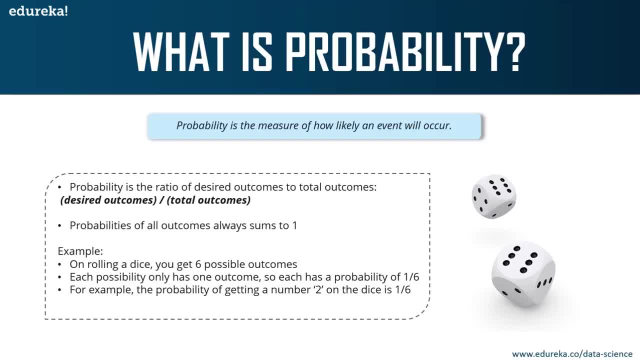 Out of six phases, there's only one phase which has the number three. So the probability of getting three when you roll a dice is one by six. Similarly, if you want to find the probability of getting a number five, again, the probability is going to be one by six. all right. 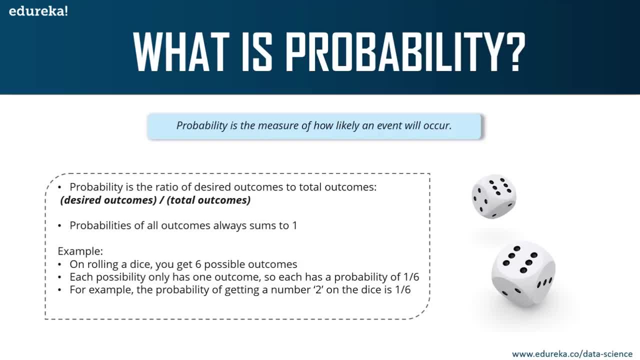 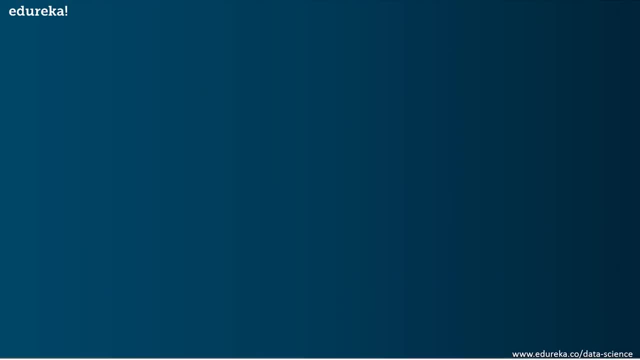 So all of this will sum up to one, all right. So, guys, this is exactly what probability is. It's a very simple concept. We all learned it in eight standard onwards. right Now, let's understand the different terminologies that are related to probability. 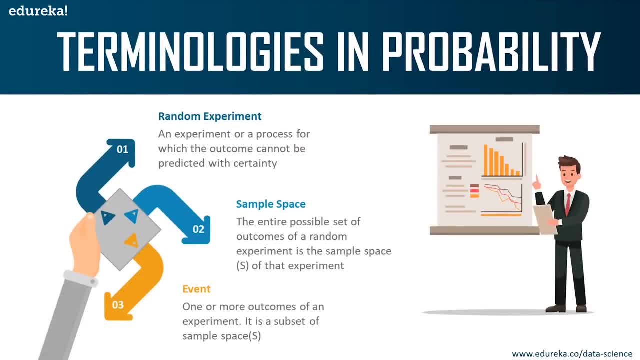 Now, there are three terminologies that you often come across when we talk about probability. We have something known as zero. It's a random experiment. okay, It's basically an experiment or a process for which the outcomes cannot be predicted with certainty. All right, that's why you use probability. 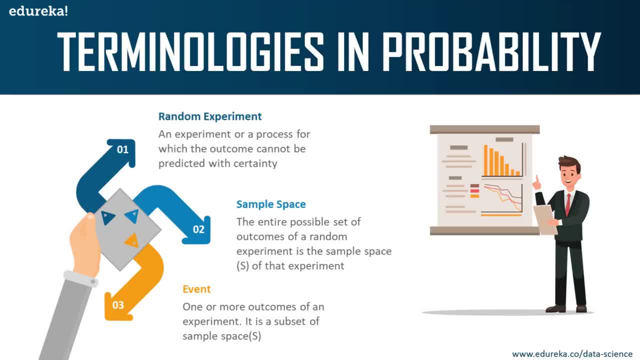 You're going to use probability in order to predict the outcome with some sort of certainty. Sample space is the entire possible set of outcomes of a random experiment. An event is one or more outcomes of an experiment. So if you consider the example of rolling a dice, 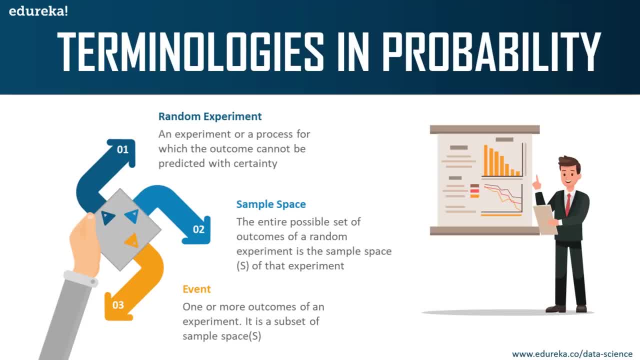 now let's say that you want to find out the probability of getting a two when you roll a dice. okay, So finding this probability is the random experiment. The sample space is basically your entire possibility. okay, So one, two, three, four, five, six phases are there. 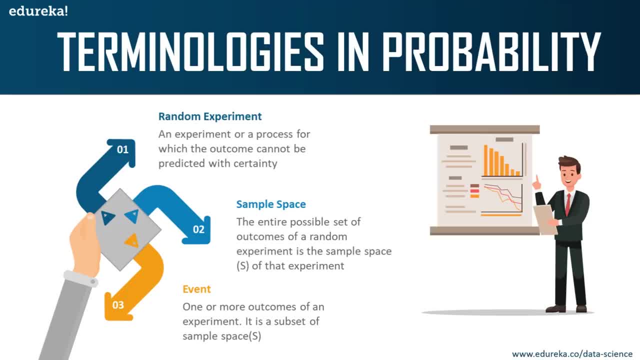 and out of that you need to find the probability of getting a two right. So all the possible outcomes will basically represent your sample space. okay, So one to six are all your possible outcomes. This represents your sample space. Now, event is one or more outcomes. 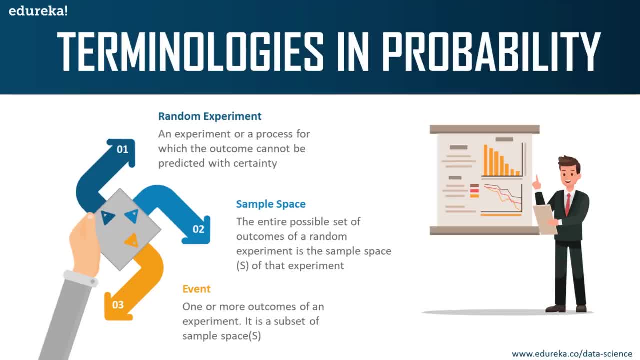 experiment. the sample space is basically your entire possibility. okay, so 1, 2, 3, 4, 5, 6 phases are there, and out of that you need to find the probability of getting a 2 right. so all the possible outcomes will basically represent your sample. 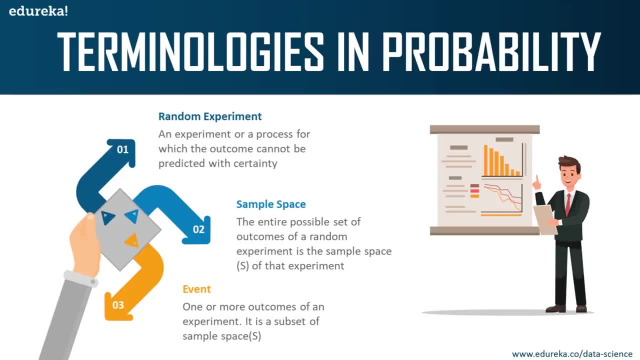 space. okay, so 1 to 6 are all your possible outcomes. this represents your sample space. now, event is one or more outcome of an experiment. so in this case, my event is to get a 2 when I roll a dice, right, so my event is the. 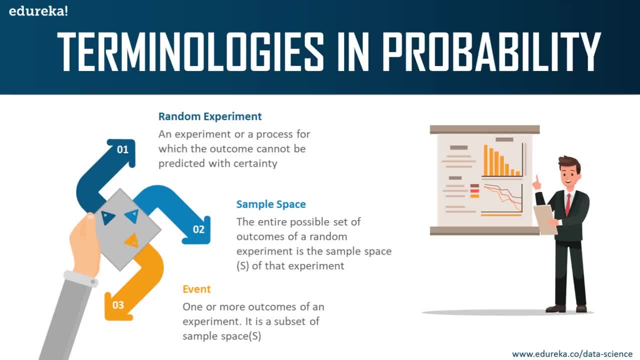 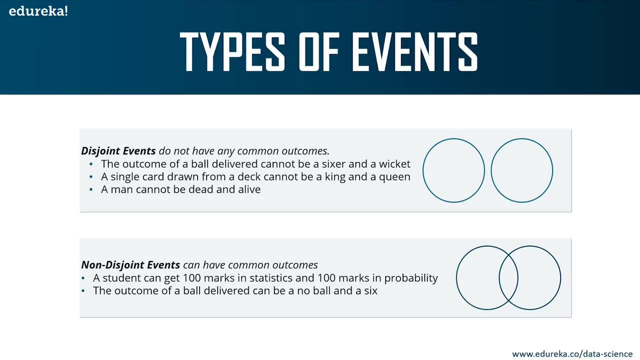 probability of getting a 2 when I roll a dice. so, guys, this is basically what random experiment, sample space, an event, really means. all right now let's discuss the different types of events. there are two types of events that you should know about. there is disjoined and non disjoined events. disjoined events are: 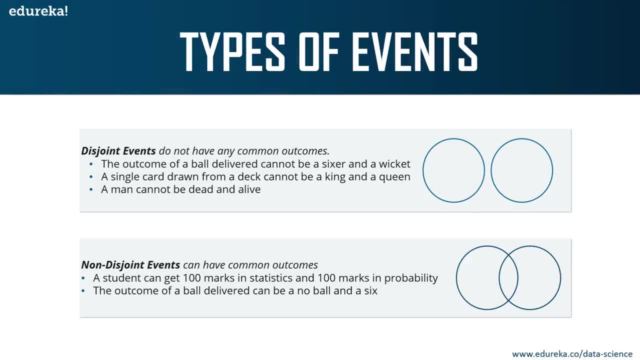 events that do not have any common outcome. for example, if you draw the, a single card from a deck of cards, it cannot be a king and a queen, correct? it can either be king or it can be queen. now, non-disjoint events are events that have common outcomes, for example, a: 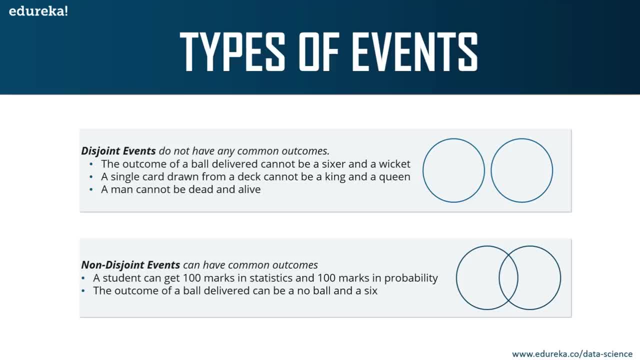 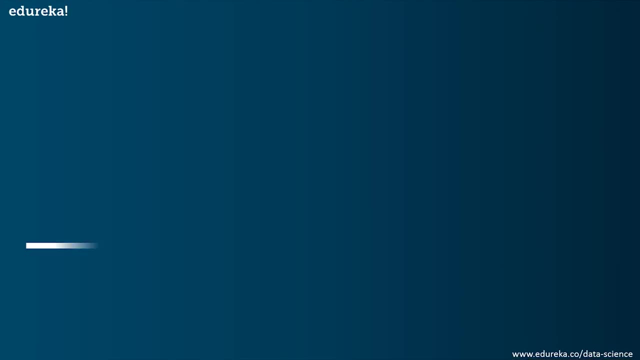 student can get 100 marks in statistics and 100 marks in probability, all right. and also, the outcome of a ball delivered can be a no ball and it can be a six, right. so this is what non-disjoint events are. all right, these are very simple to understand right now. let's move on and look at the different. 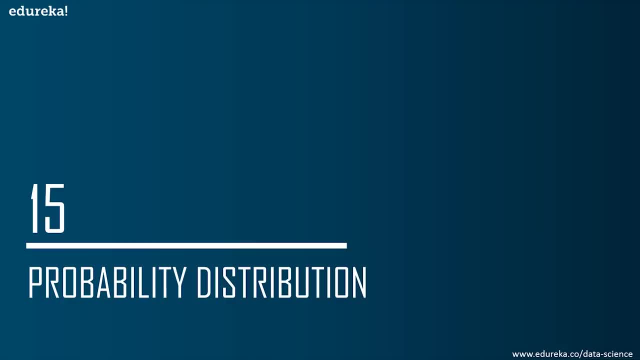 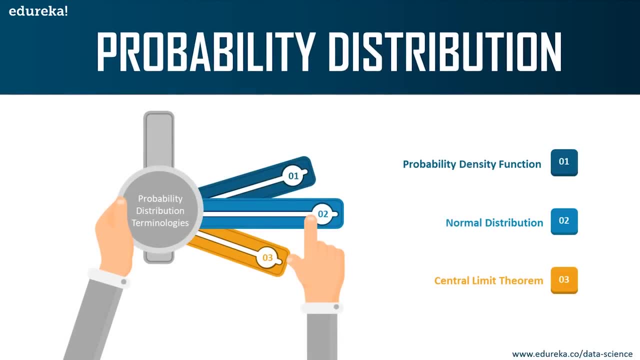 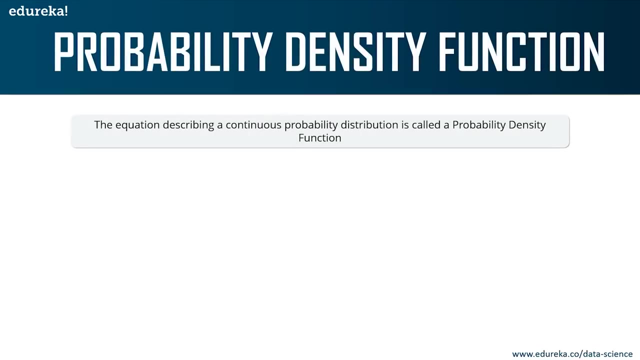 types of probability distribution. all right, i'll be discussing the three main probability distribution functions. i'll be talking about probability density function, normal distribution and central limit theorem. okay, probability density function, also known as pdf, is concerned with the relative likelihood for a continuous random variable to take on a given value. 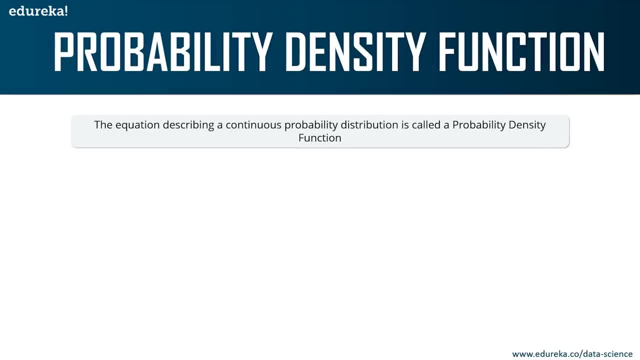 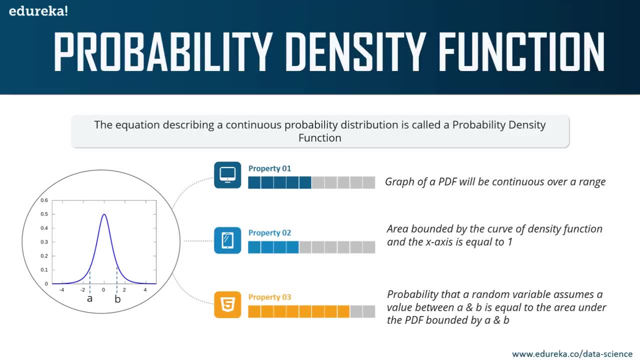 all right, so the pdf gives the probability of a variable that lies between the range a and b. so basically, what you're trying to do is you're going to try and find the probability of a continuous random variable over a specified range. okay, now this graph denotes the pdf of a continuous variable. 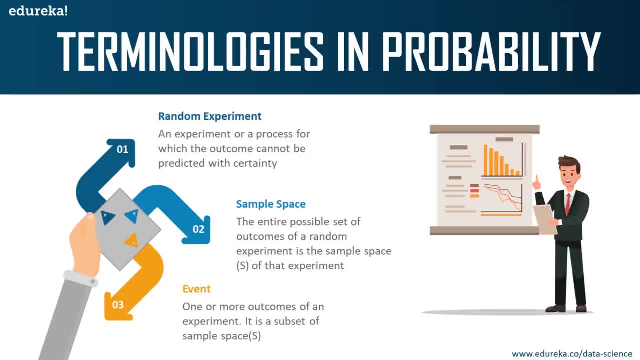 This represents the outcome of an experiment. So, in this case, my event is to get a two when I roll a dice, right? So my event is the probability of getting a two when I roll a dice. So, guys, this is basically what random experiment. 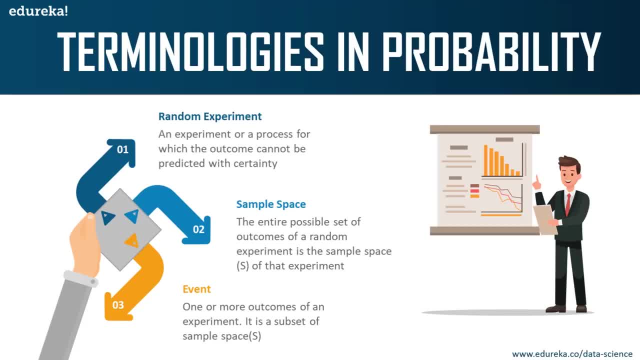 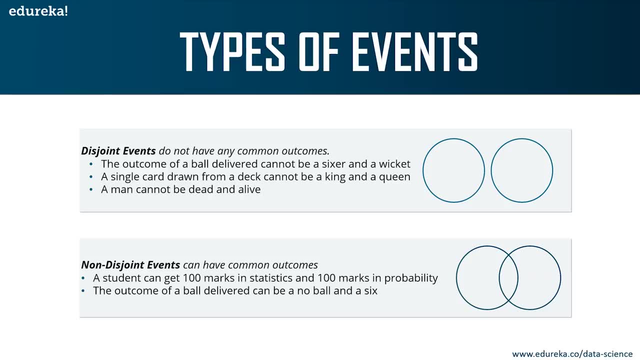 sample space and event really means all right. Now let's discuss the different types of events. There are two types of events that you should know about. There is disjoint and non-disjoint events. Disjoint events are events that do not have any common outcome. 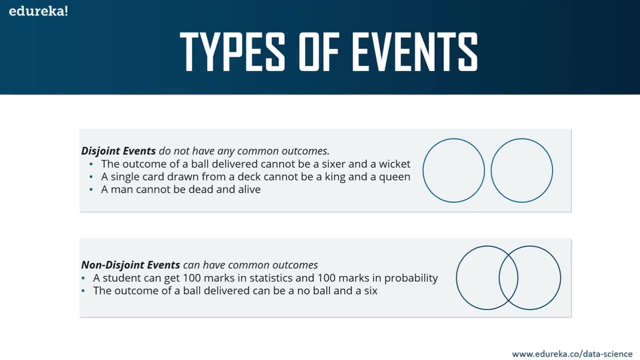 For example, if you draw a single card from a deck of cards, it cannot be a king and a queen, correct? It can either be king or it can be queen. Now, non-disjoint events are events that have common outcomes. For example, a student can get 100 marks in statistics. 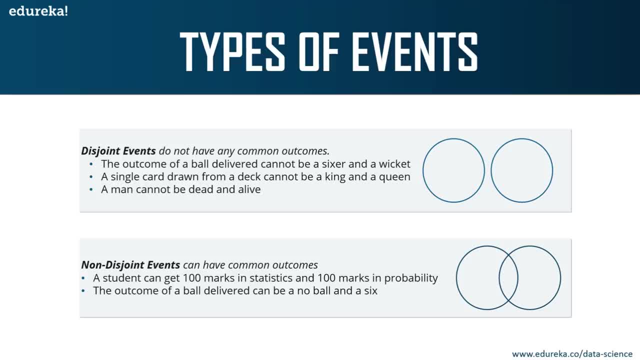 and 100 marks in probability, all right. And also the outcome of a ball delivered can be a no ball and it can be a six right. So this is what non-disjoint events are all right, Very simple to understand, right. 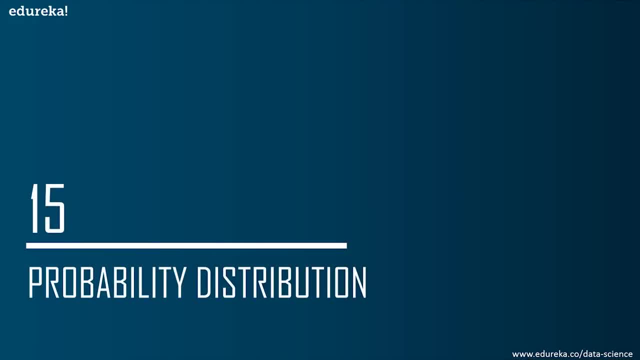 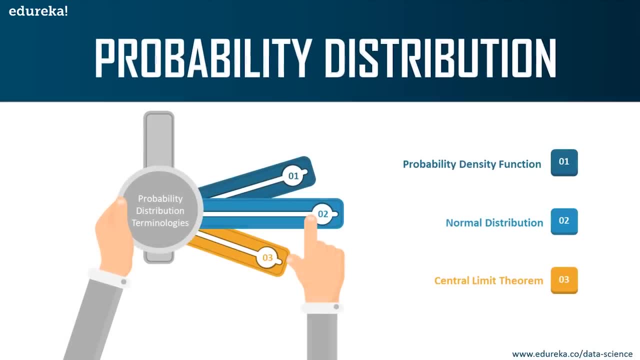 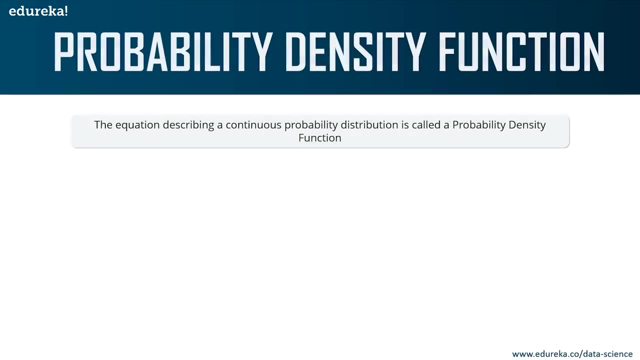 Now let's move on and look at the different types of probability distribution. all right, I'll be discussing the three main probability distribution functions. I'll be talking about probability density function, normal distribution and central limit theorem. okay, Probability density function, also known as PDF, 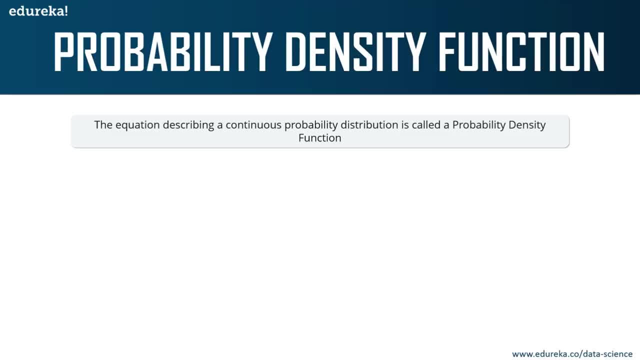 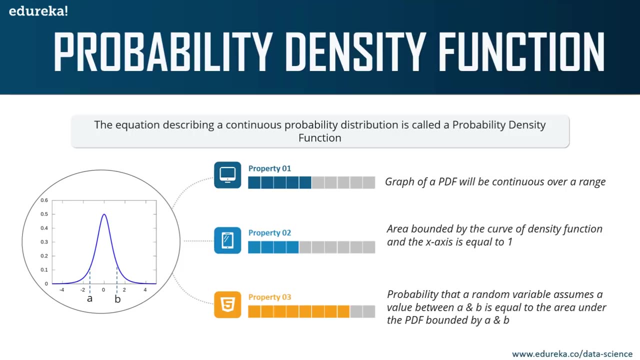 is concerned with the relative likelihood for a continuous random variable to take on a given value. All right, So the PDF gives the probability of a variable that lies between the range A and B. So, basically, what you're trying to do is you're going to try and find the probability. 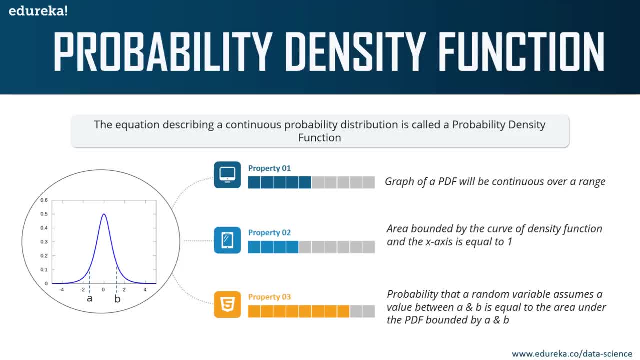 of a continuous random variable over a specified range. okay, Now this graph denotes the PDF of a continuous variable. Now, this graph is also known as the bell curve. all right, It's famously called the bell curve because of its shape, And there are three important properties. 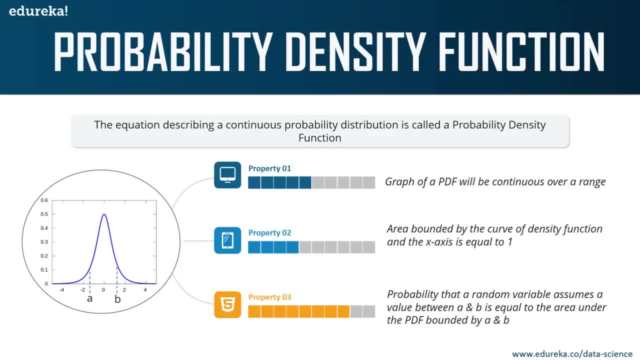 that you need to know about a probability density function. Now, the graph of a PDF will be continuous over a range. This is because you're finding the probability that a continuous variable lies between the ranges A and B, all right. The second property is that the area bounded by the curve 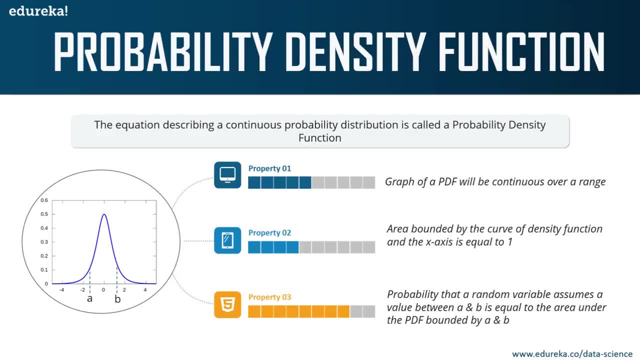 now, this graph is also known as the bell curve. all right, it's famously called the bell curve because of its shape, and there are three important properties that you need to know about: a probability distribution, probability density, function. now the graph of a pdf will be continuous over a range. 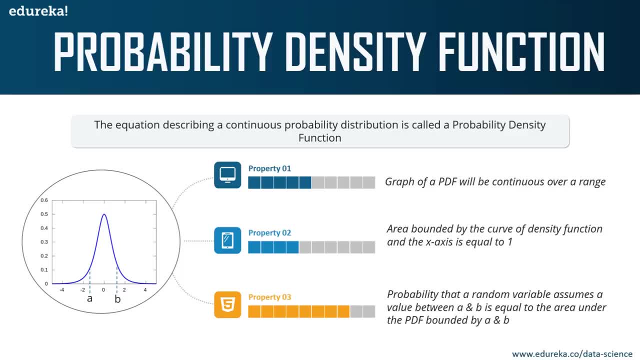 this is because you're finding the probability that a continuous variable lies between the ranges a and b right. the second property is that the area bounded by the curve of a density function and the x-axis is equal to one. basically, the area below the curve is equal to one. all right. 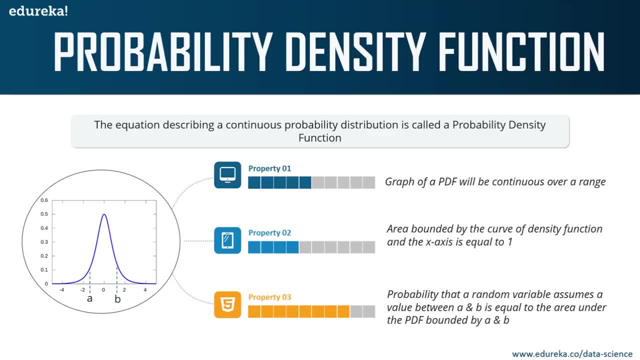 because it denotes probability. again, the probability cannot arrange more than one. it has to be between zero and one property. number three is that the probability that a random variable assumes a value between a and b is equal to the area under the pdf bounded by a and b. okay, 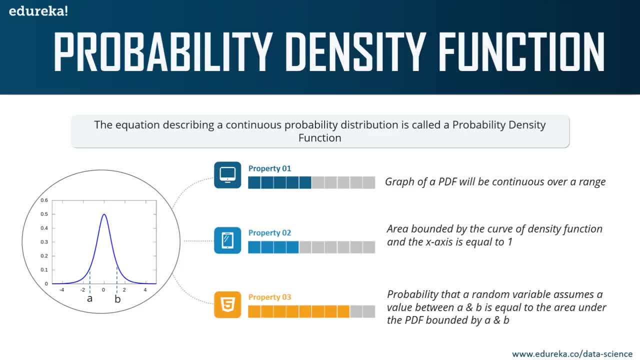 now, what this means is that the probability value is denoted by the area of the graph. all right, so whatever value that you get here, which is basically one, is the probability that a random variable will lie between the range a and b. all right, so i hope all of you have. 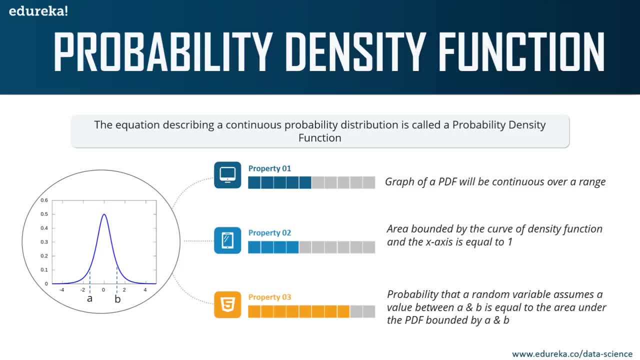 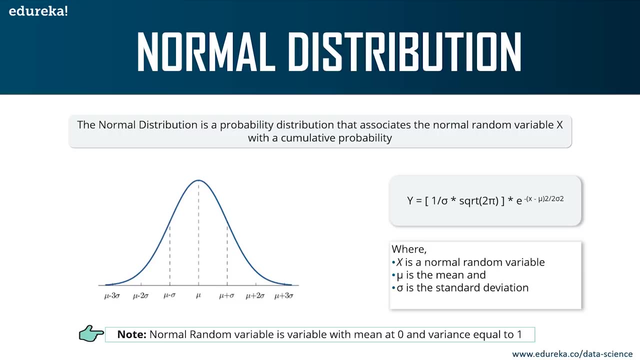 understood the probability density function. it's basically the probability of finding the value of a continuous random variable between the range a and b. all right, now let's look at our next distribution, which is normal distribution. now, normal distribution, which is also known as the gaussian distribution, is a probability distribution that denotes the symmetric 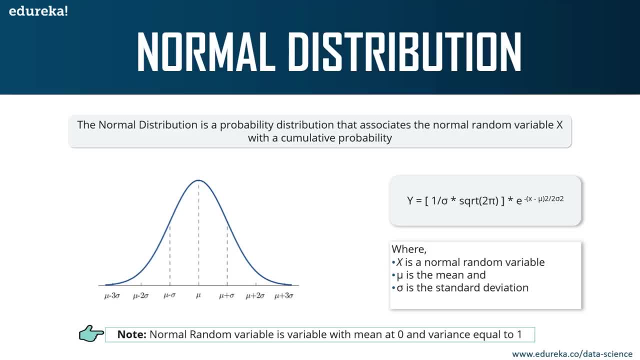 property of the mean right, meaning that the idea behind this function is that the data near the mean occurs more frequently than the data away from the mean. so what it means to say is that the data around the mean represents the entire data set. okay, so if you just take a sample, 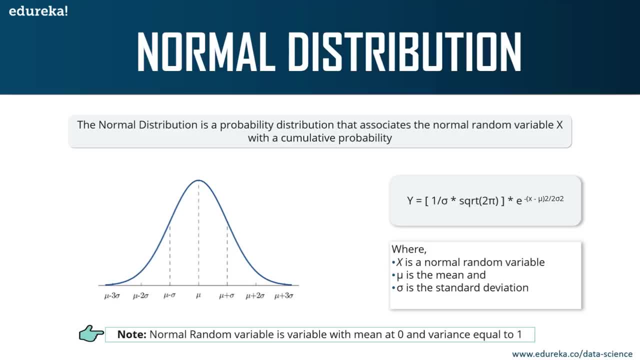 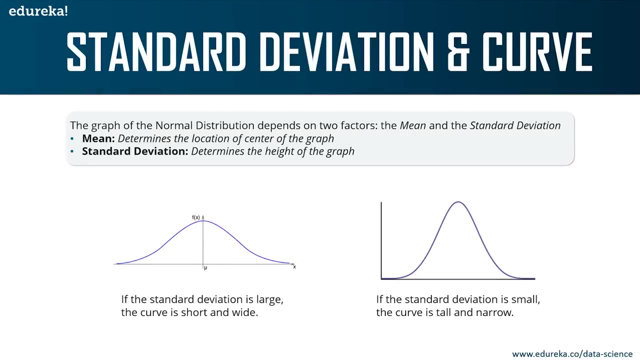 of data around the mean, it can represent the entire data set. now, similar to the probability density function, the normal distribution appears as a bell curve. all right now, when it comes to normal distribution, there are two important factors. all right, we have the mean of the population and 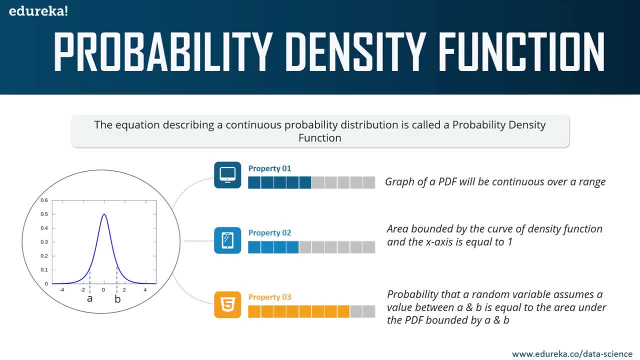 of a density function and the x-axis is equal to one. Basically, the area below the curve is equal to one. all right, Because it denotes probability. Again, the probability cannot range more than one. It has to be between zero and one. 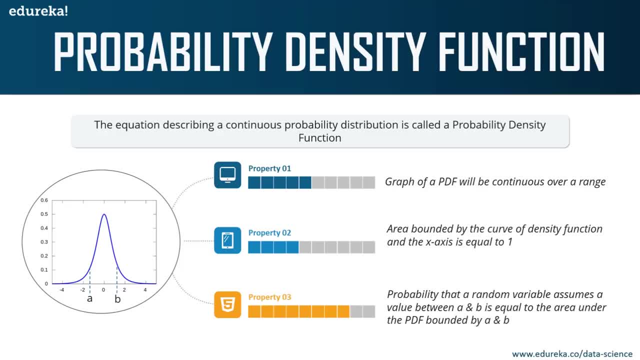 Property number three is that the probability that a random variable assumes a value between A and B is equal to the area under the PDF bounded by A and B. Okay now, what this means is that the probability value is denoted by the area of the graph. all right, 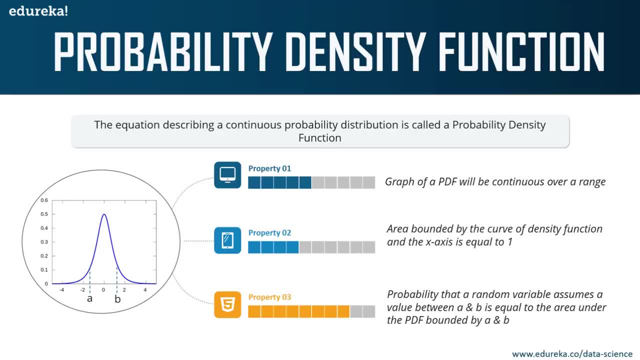 So whatever value that you get here, which is basically one, is the probability that a random variable will lie between the range A and B. all right, So I hope all of you have understood the probability density function. It's basically the probability of finding the value. 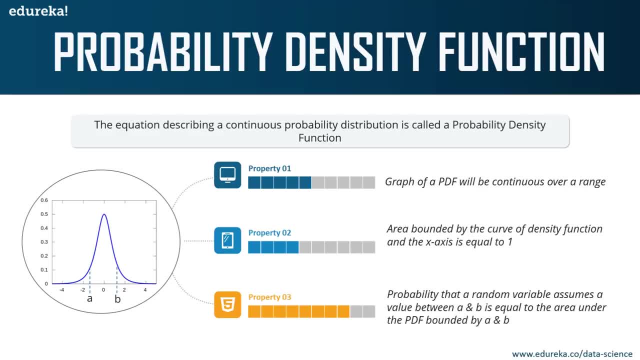 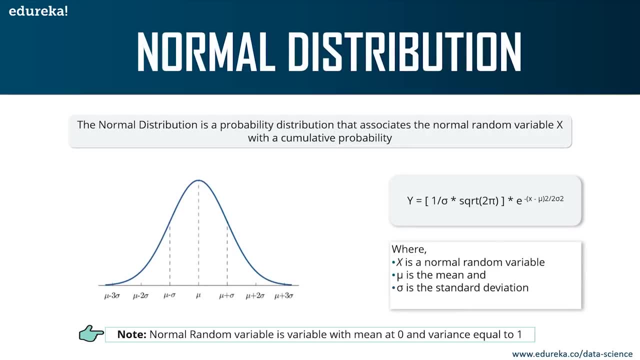 of a continuous random variable between the range A and B. all right, Now let's look at our next distribution, which is normal distribution. Now, normal distribution, which is also known as the Gaussian distribution, is a probability distribution that denotes the symmetric property of the mean. all right, 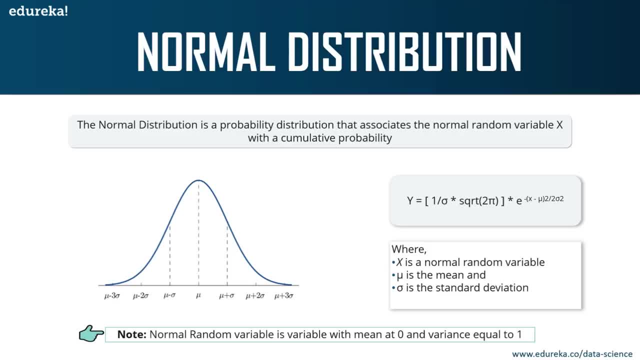 Meaning that the idea behind this function is that the data near the mean occurs more frequently than the data away from the mean. So what it means to say is that the data around the mean represents the entire data set. okay, So if you just take a sample of data around the mean, 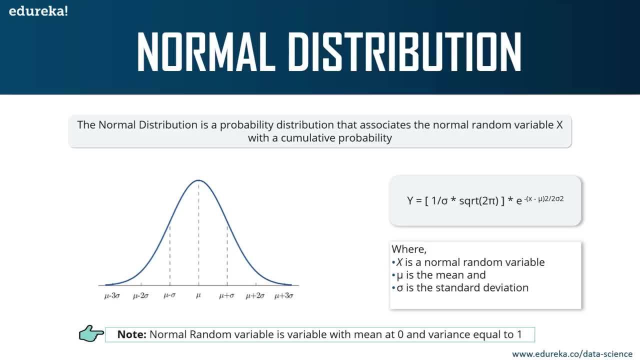 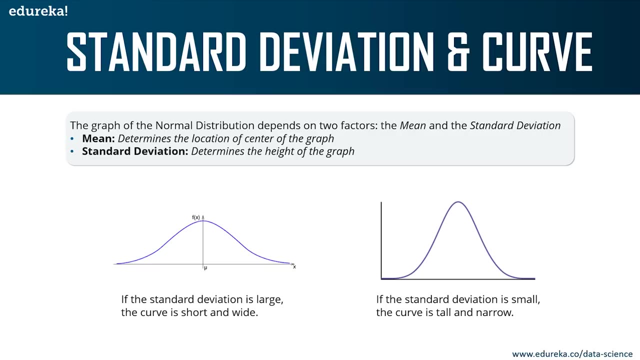 it can represent the entire data set. Now, similar to the probability density function, the normal distribution appears as a bell curve. all right. Now, when it comes to normal distribution, there are two important factors. all right, We have the mean of the population and the standard deviation. 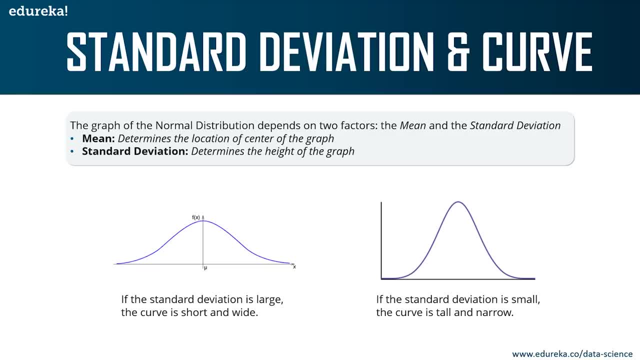 Okay, so the mean and the graph determines the location of the center of the graph, all right. And the standard deviation determines the height of the graph. okay, So if the standard deviation is large, the curve is going to look something like this, all right? 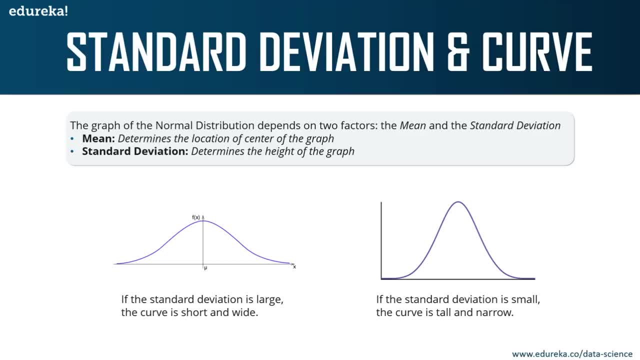 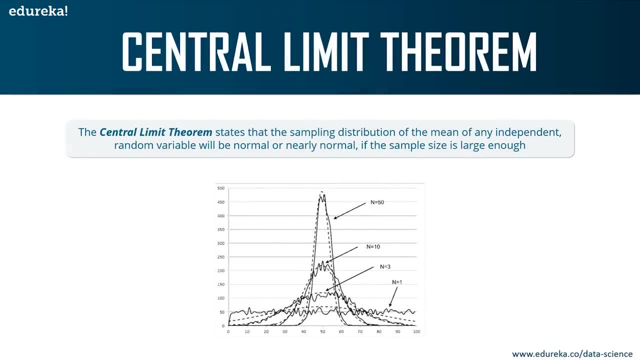 It'll be short and wide, And if the standard deviation is small, the curve is tall and narrow. all right, So this was it about normal distribution. Now let's look at the central limit theory. Now, the central limit theory states that the sampling distribution of the mean 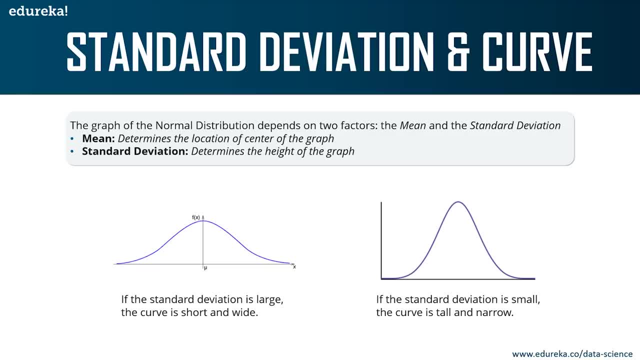 the standard deviation. okay, so the mean and the graph determines the location of the center of the graph right, and the standard deviation determines the height of the graph. okay, so if the standard deviation is large, the curve is going to look something like this: all right, it will be short. 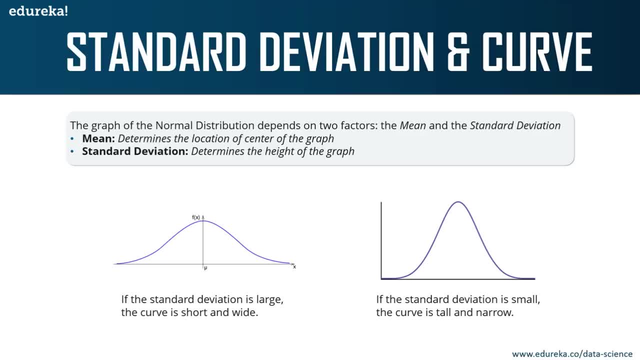 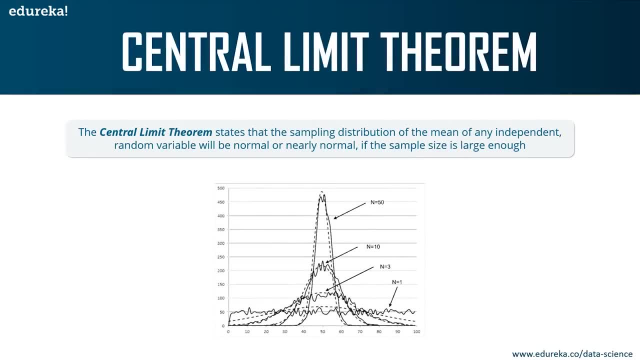 and wide, and if the standard deviation is small, the curve is tall and narrow. all right, so this was it about normal distribution. now let's look at the central limit theory. now, the central limit theory states that the sampling distribution of a random variable between the range a and b- all right, 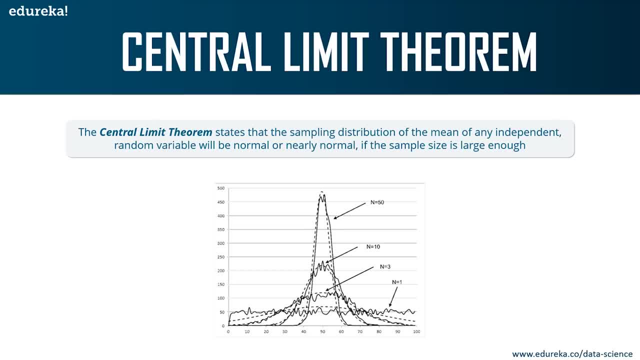 distribution of the mean of any independent random variable will be normal or nearly normal if the sample size is large enough. now that's a little confusing. okay, let me break it down for you now in simple terms. if we had a large population and we divided it into many samples, then the mean 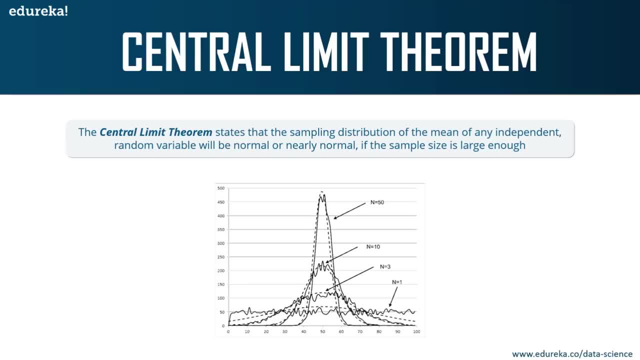 of all the samples from the population will be almost equal to the mean of the entire population. all right, meaning that each of the sample is normally distributed, right. so if you compare the mean of each of the sample, it will almost be equal to the mean of the. 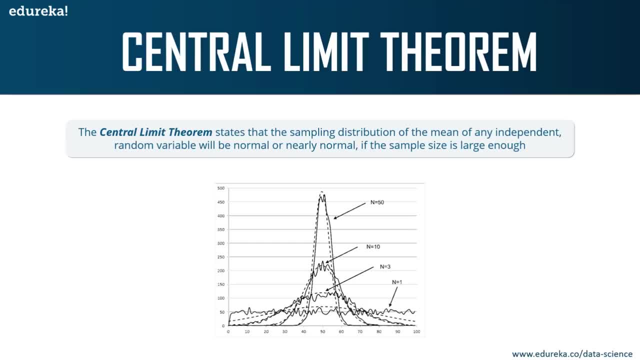 population, right? so this graph basically shows a more clear understanding of the central limit theorem. right? you can see each sample here and the mean of each sample is almost along the same line, right? okay, so this is exactly what the central limit theorem states. now, the accuracy or the 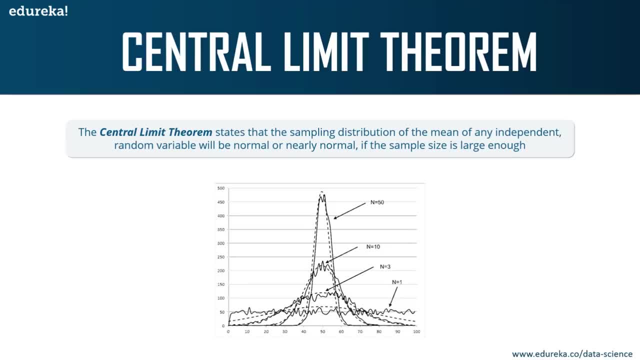 resemblance to the normal distribution depends on two main factors, right? so the first is the number of sample points, that you consider all right, and the second is the shape of the underlying population. now, the shape obviously depends on the standard deviation and the mean of a sample, correct? so, guys, central limit theorem basically states that each sample will be normally. 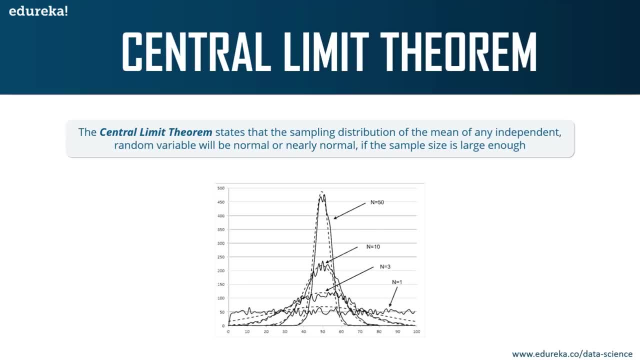 distributed in such a way that the mean of each sample will coincide with the mean of the actual population. all right, in short terms, that's what central limit theorem states. all right, and this holds true only for a large data set, mostly for a small data set. there are more deviations when compared to a large data set. 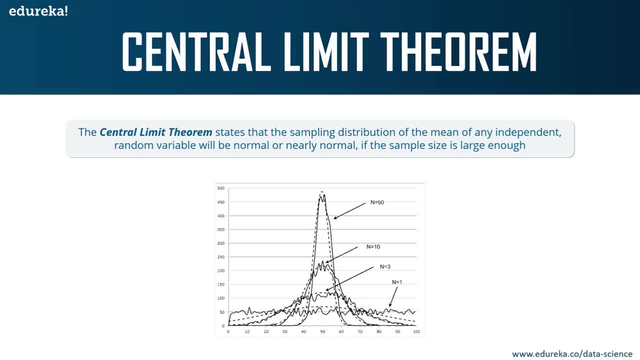 of any independent, random variable will be normal or nearly normal if the sample size is large enough. Now that's a little confusing. Okay, let me break it down for you Now in simple terms. if we had a large population and we divided it into many samples, 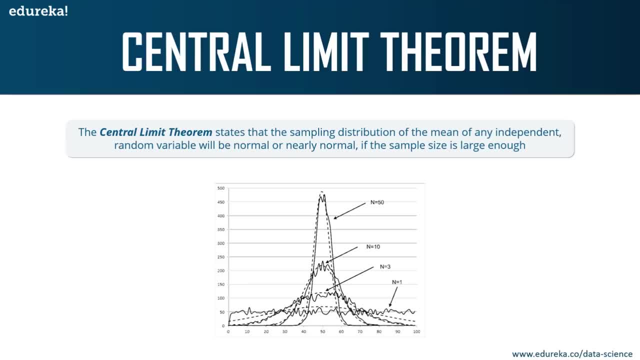 then the mean of all the samples from the population will be almost equal to the mean of the entire population. all right, meaning that each of the sample is normally distributed, right? So if you compare the mean of each of the sample, it'll almost be equal. 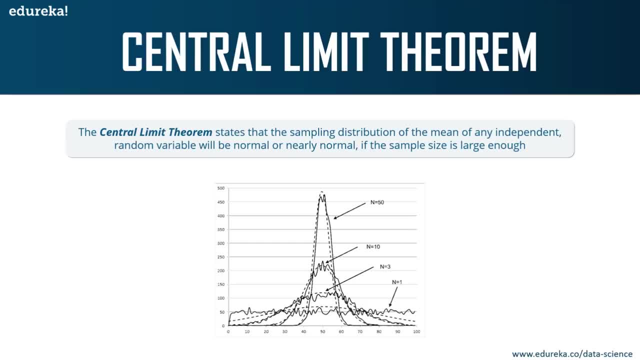 to the mean of the population, right? So this graph basically shows a more clear understanding of the central limit theorem, right? You can see each sample here and the mean of each sample is almost along the same line, right? Okay, so this is exactly. 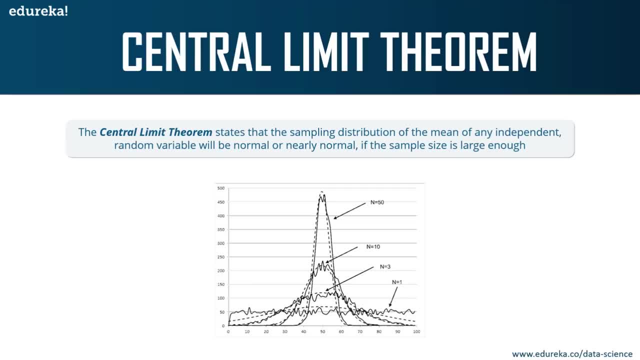 what the central limit theorem states. Now, the accuracy or the resemblance to the normal distribution depends on two main factors, right. One is the sample points that you consider all right, And the second is the shape of the underlying population. Now, the shape obviously depends on the standard deviation. 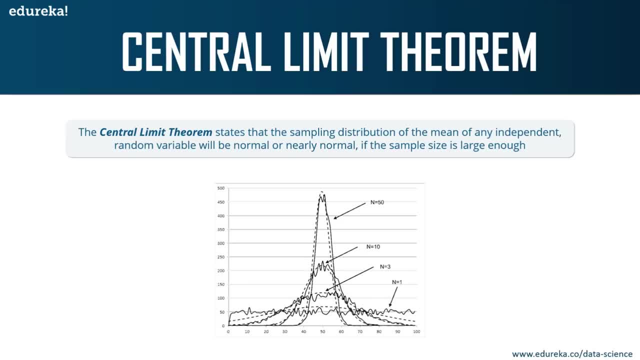 and the mean of a sample, correct? So, guys, central limit theorem basically states that each sample will be normally distributed in such a way that the mean of each sample will coincide with the mean of the actual population. all right, in short terms. 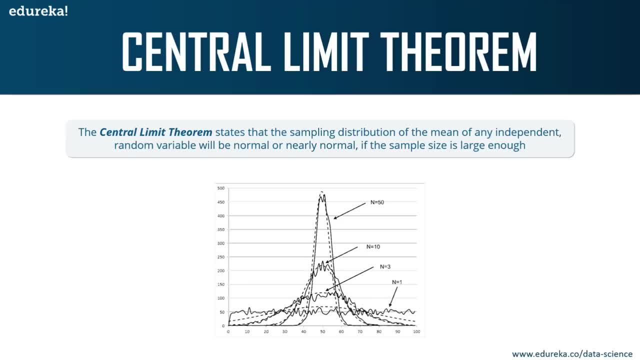 that's what central limit theorem states. all right, And this holds true only for a large data set. Mostly for a small data set there are more deviations when compared to a large data set. It's because of the scaling factor, right. 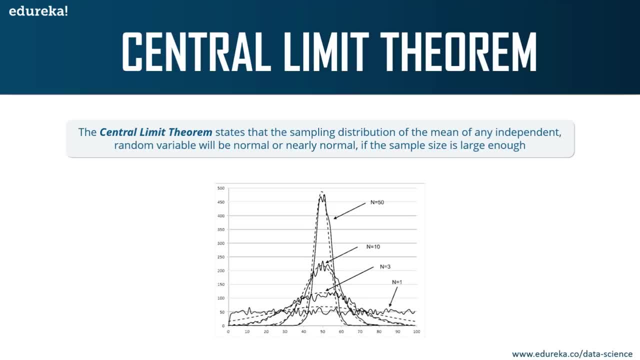 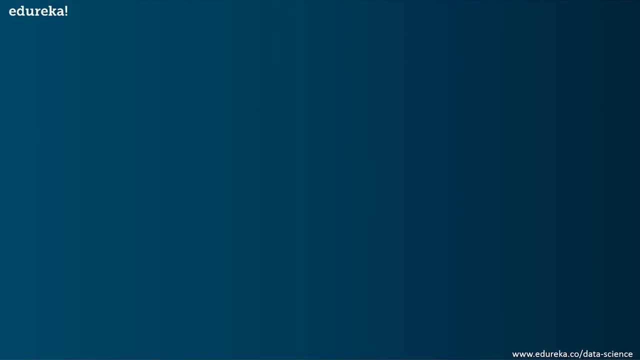 The smallest deviation in a small data set will change the value very drastically, But in a large data set, a small deviation will not matter at all. Now let's move on and look at our next topic, which is the different types of probability. 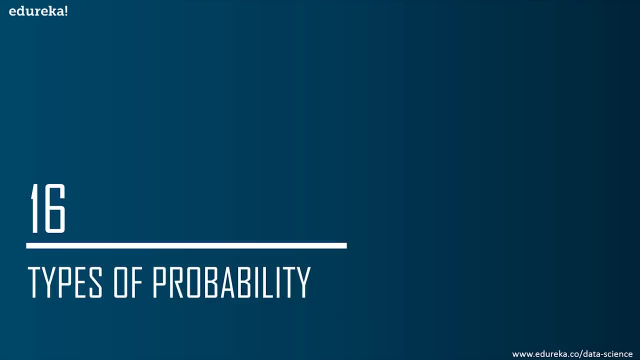 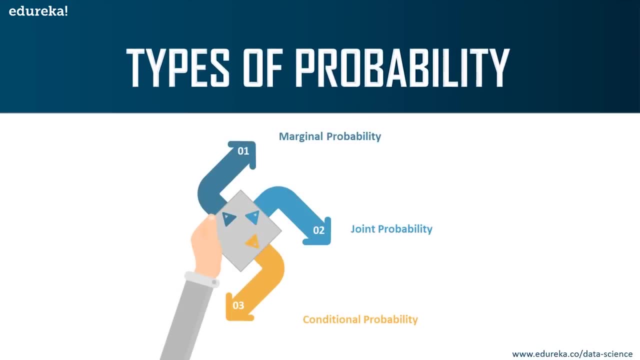 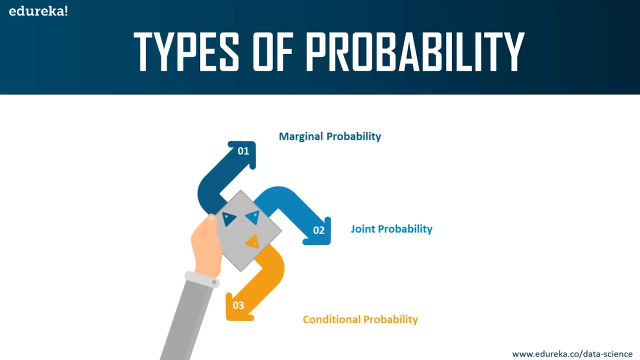 Now, this is a important topic because most of your problems can be solved by understanding which type of probability should I use to solve this problem, right? So we have three important types of probability. We have marginal, joint and conditional probability. So let's discuss each of these. 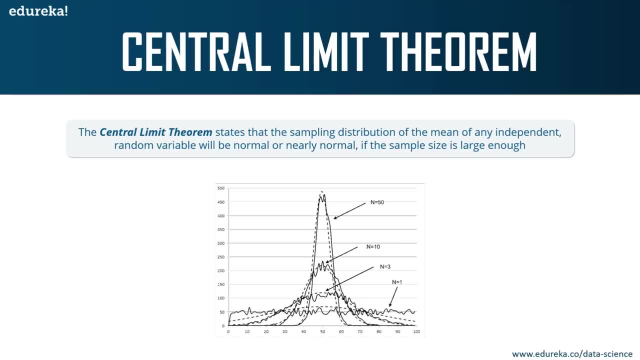 it's because of the scaling factor right. the smallest deviation in a small data set will change the value very drastically, but in a large data set, a small deviation will not matter at all. now let's move on and look at our next topic, which is the different types of probability. 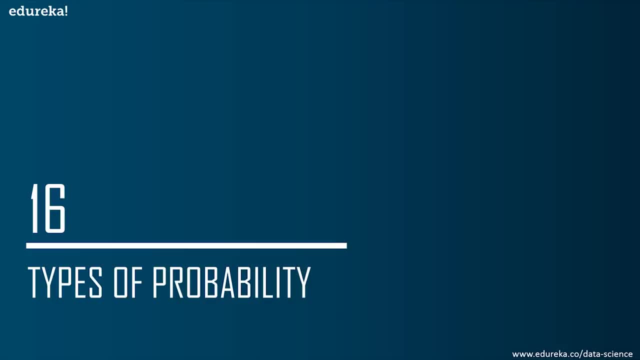 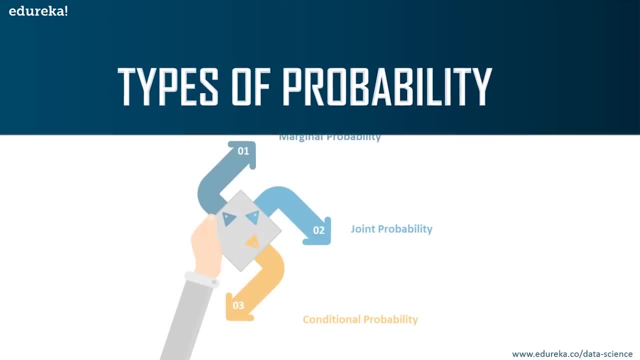 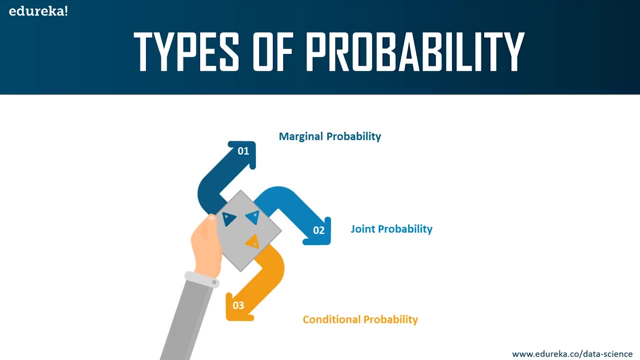 now. this is a important topic because most of your problems can be solved by understanding which type of probability should i use to solve this problem right? so we have three important types of probability. we have marginal, joint and conditional probability. so let's discuss each of these now. the probability of an event occurring: 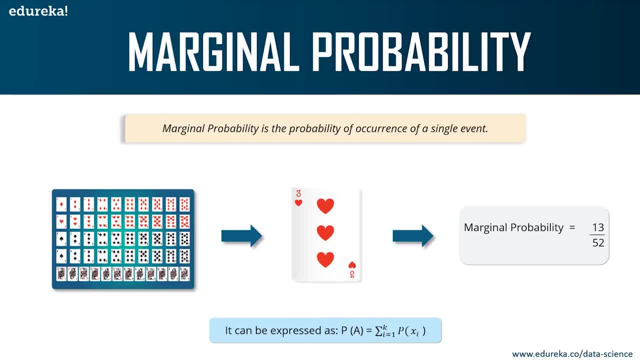 unconditioned on any other event is known as marginal probability or unconditional probability. so let's say that you want to find the probability that a car drawn is a heart, all right. so if you want to find the probability that a car drawn is a heart, the probability will be 30. 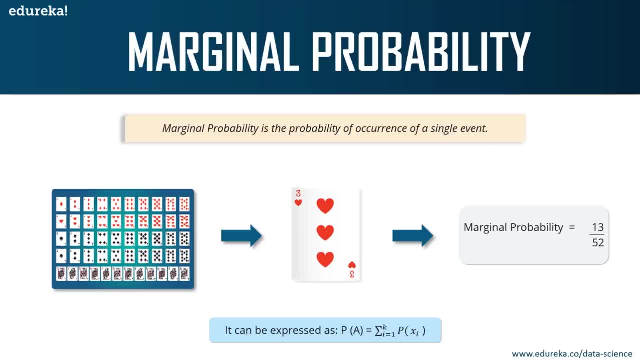 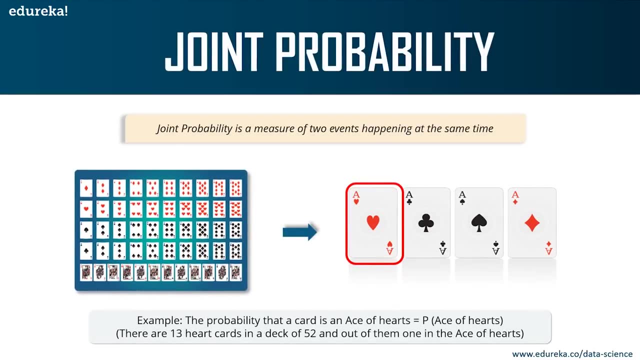 by 52, since there are 52 cards in a deck and there are 13 hearts in a deck of cards right, and there are 52 cards in a total deck. so your marginal probability will be 13 by 52.. that's about marginal probability. now let's understand what is joint probability. now, joint probability. 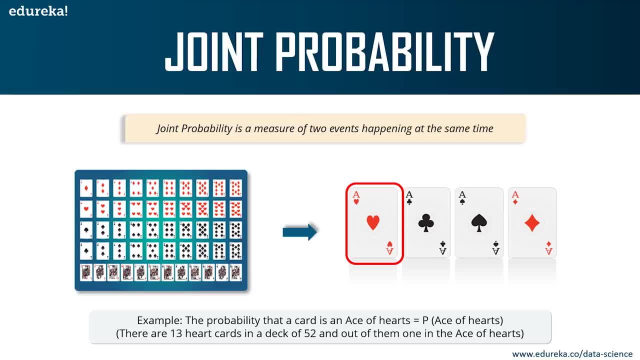 is a measure of two events happening at the same time. okay, let's say that the two events are a and b. so the probability of event a and b occurring is the intersection of a and b. so, for example, if you want to find the probability that a card is a 4 and a red, 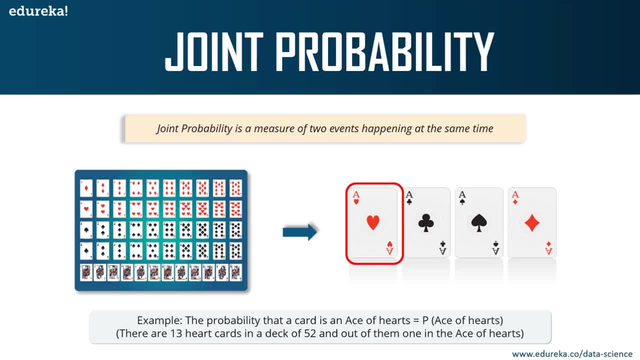 that would be joint probability. all right, because you're finding a card that is 4 and the card has to be red in color. so for the answer, this will be 2 by 52, because we have 1, 2 in hearts and we have 1, 2 in diamonds, correct? so both of these are red in color. 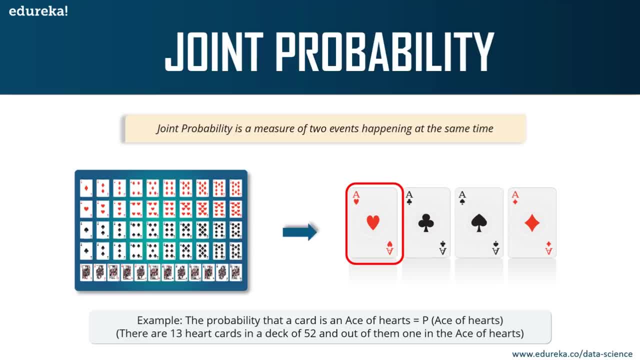 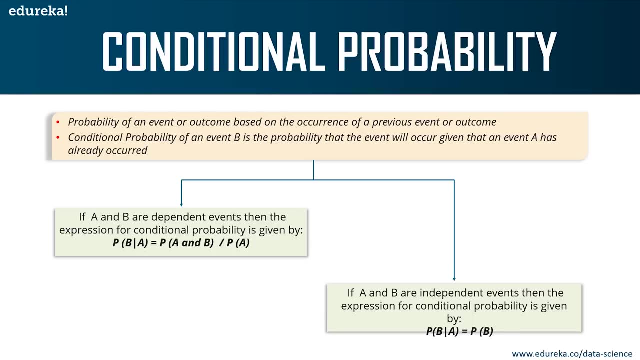 therefore, our probability is 2 by 52, and if you further down it, it is 1 by 52, 26, right? so this is what joint probability is all about. moving on, let's look at what exactly conditional probability is. so if the probability of an event or an outcome is based on the 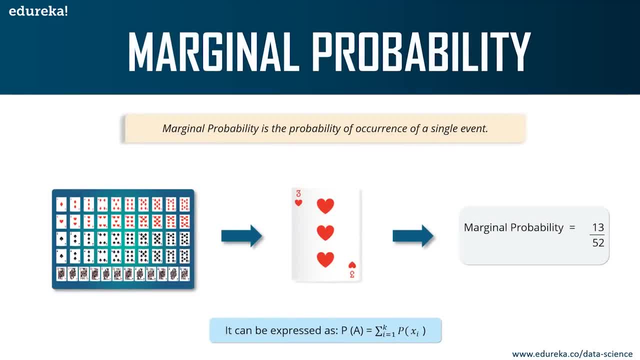 Now, the probability of an event occurring unconditioned on any other event is known as marginal probability or unconditional probability. So let's say that you want to find the probability that a card drawn is a heart, all right, So if you want to find the probability, 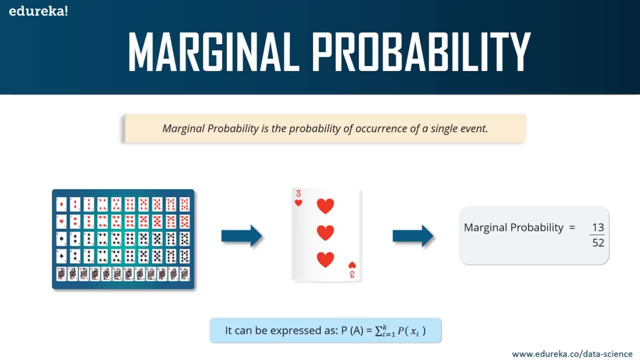 that a card drawn is a heart, the probability will be 13 by 52.. Since there are 52 cards in a deck and there are 13 hearts in a deck of cards, right, And there are 52 cards in a total deck. 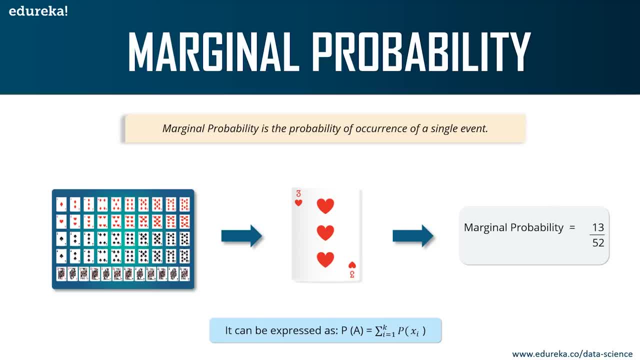 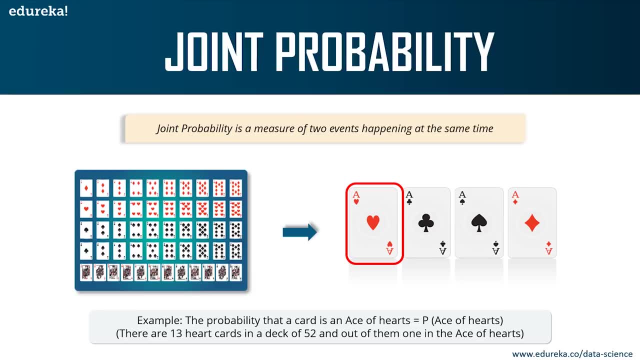 So your marginal probability will be 13 by 52.. That's about marginal probability. Now let's understand what is joint probability. Now, joint probability is a measure of two events happening at the same time. Okay, let's say that the two events are A and B. 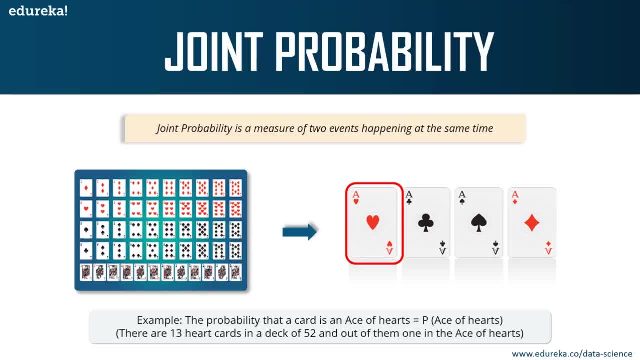 So the probability of event A and B occurring is the intersection of A and B. So, for example, if you want to find the probability that a card is a four and a red, that would be joint probability. all right, Because you're finding a card that is four. 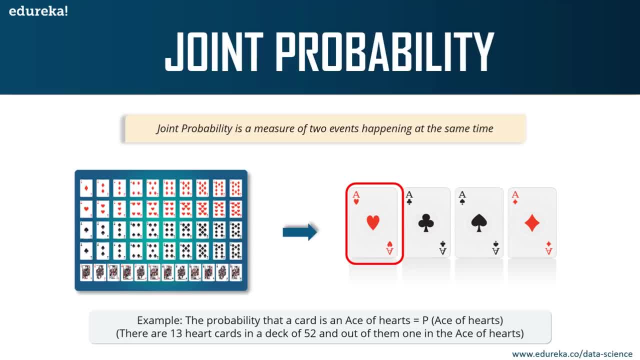 and the card has to be red in color. So, for the answer, this will be two by 52, because we have one two in hearts and we have one two in diamonds, correct? So both of these are red in color. therefore, our probability is two by 52.. 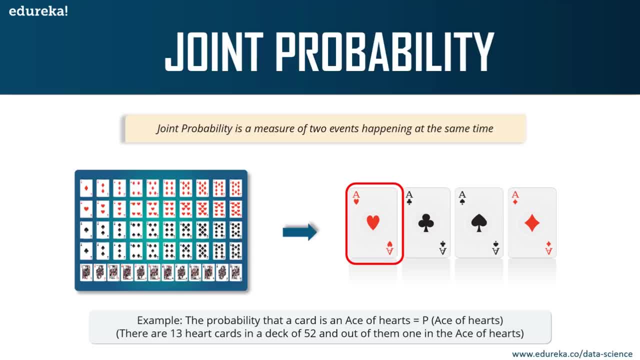 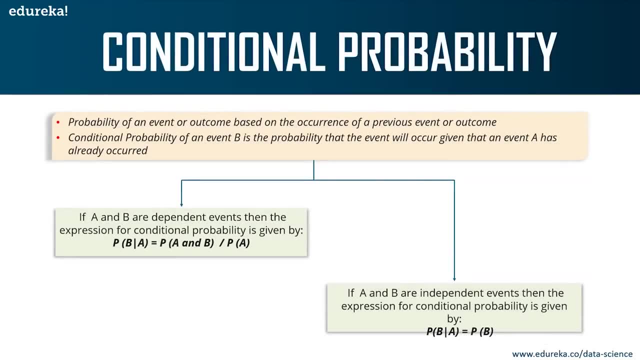 And if you further down it, it is one by 26.. All right, So this is what joint probability is all about. Moving on, let's look at what exactly conditional probability is. So if the probability of an event or an outcome is based on the occurrence of a previous event, 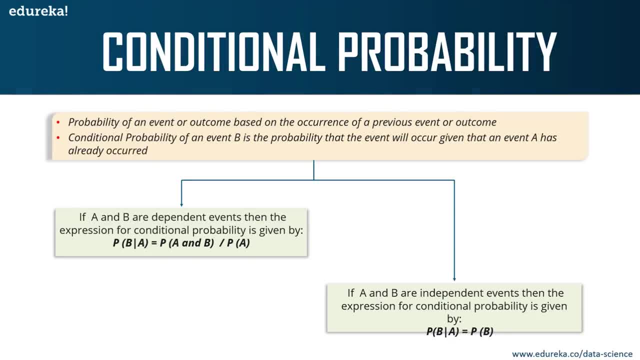 or an outcome, then you call it as a conditional probability. okay, So the conditional probability of an event B is the probability that the event will occur, given that an event A has already occurred. right? So if A and B are dependent on each other, 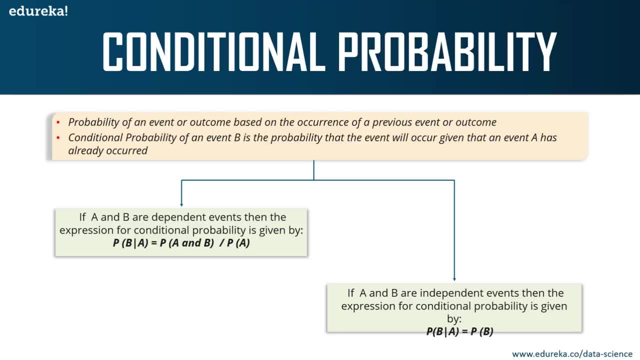 dependent events, then the expression for conditional probability is given by this. Now, this first term on the left-hand side, which is P, B of A, is basically the probability of event B occurring, given that event A has already occurred. all right. 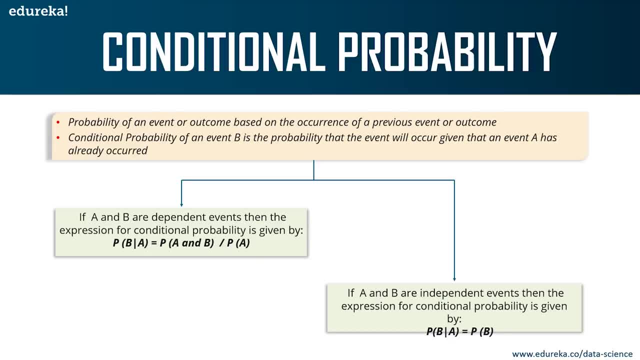 occurrence of a previous event or an outcome. then you called it as a conditional probability. okay, so the conditional probability of an event b is the probability that the event will occur, given that an event a has already occurred. right? so if a and b are dependent events, then the expression 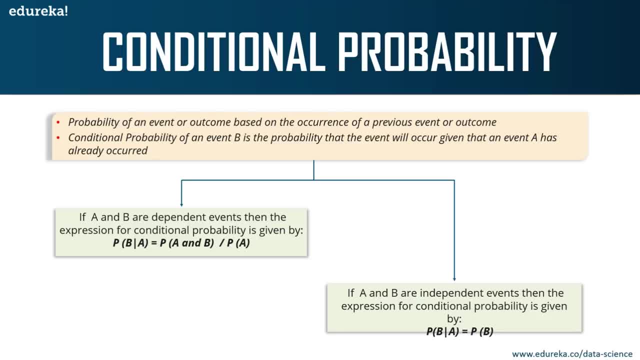 for conditional probability is given by this. now, this first term on the left hand side, which is p b of a, is basically the probability of event b occurring, given that event a has already occurred. all right, so, like i said, if a and b are dependent events, then this is the expression. 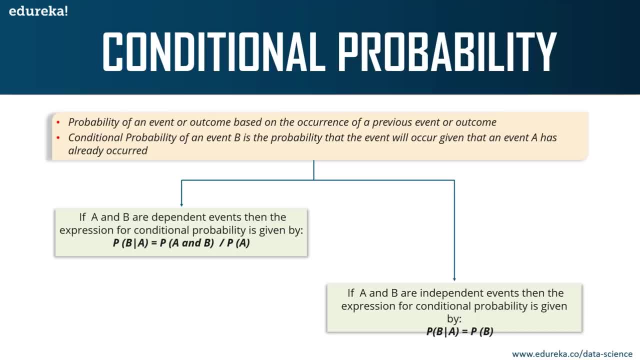 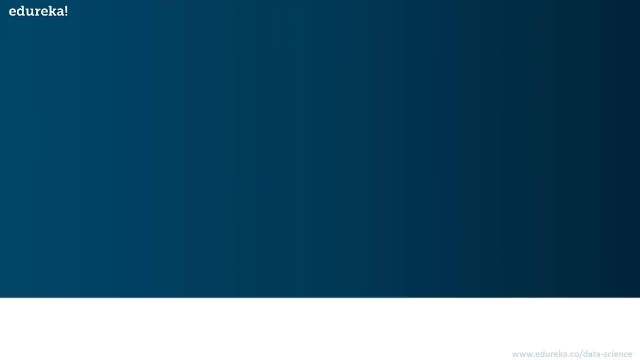 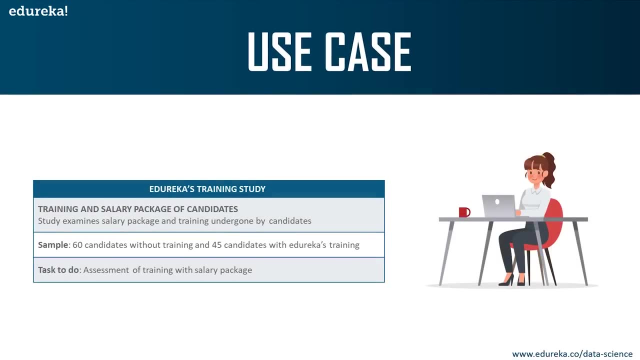 but if a and b are independent events, then the expression for conditional probability is like this: right, so, guys, p of a and p of b is obviously the probability of a and probability of b. right now. let's move on now in order to understand, uh, conditional probability, joint probability and. 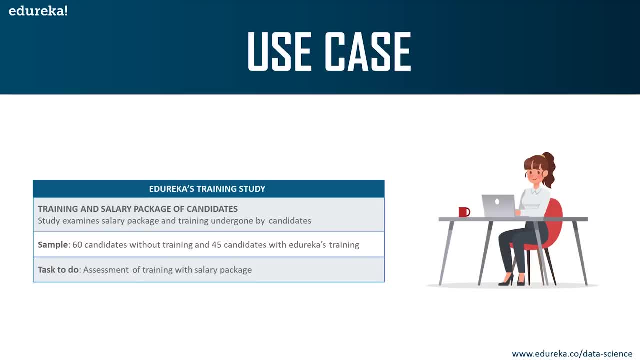 marginal probability. let's look at a small uh use case. okay now, basically, we're going to take a data set which examines the salary package and training undergone by candidates. okay, now, in this there are 60 candidates without training and 45 candidates which have enrolled for edureka's training right now. the task here is you. 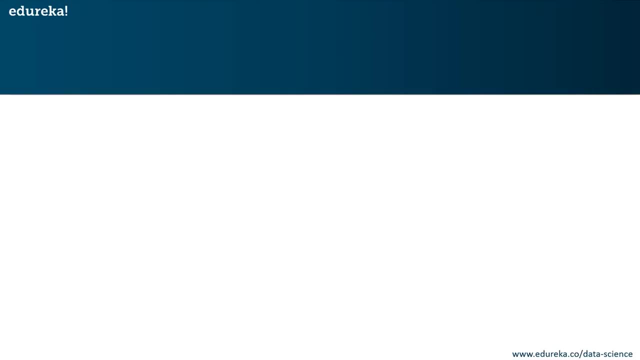 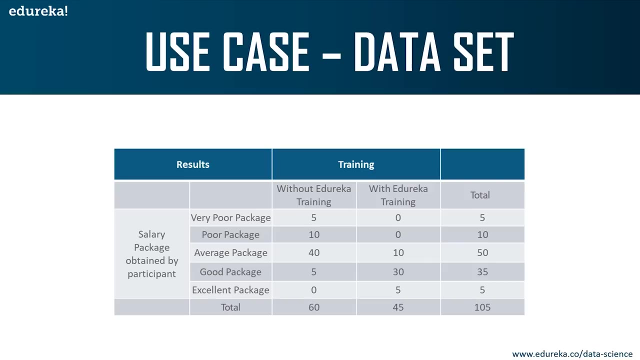 have to assess the training with a salary package. okay, let's look at this in a little more depth. so in total, we have 105 candidates, out of which 60 of them have not enrolled for edureka's training and 45 of them have enrolled for edureka's training. all right, this is a small survey. 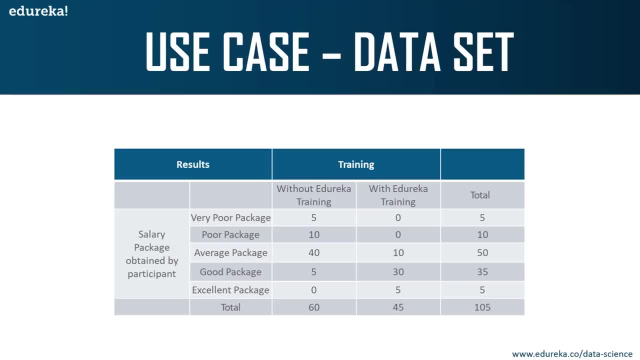 that was conducted and, um, this is the rating of the package or the salary that they got right. so if you read through the data, you can understand. there were five candidates without edureka training who got a very poor salary package- okay. similarly, there are 30 candidates with edureka training who 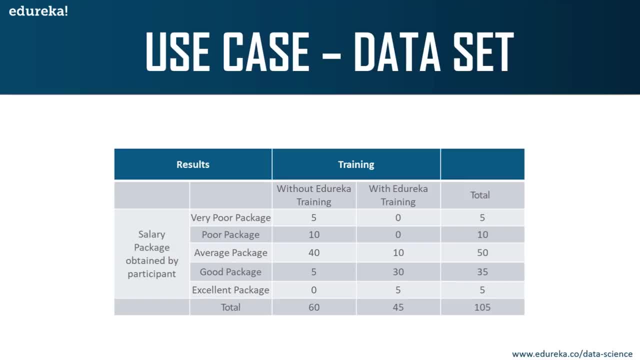 got a good package right. so, guys, basically you're comparing the salary package of a person depending on whether or not they've enrolled for edureka training, right? this is our data set. now let's look at our problem statement. find the probability that a candidate has undergone. 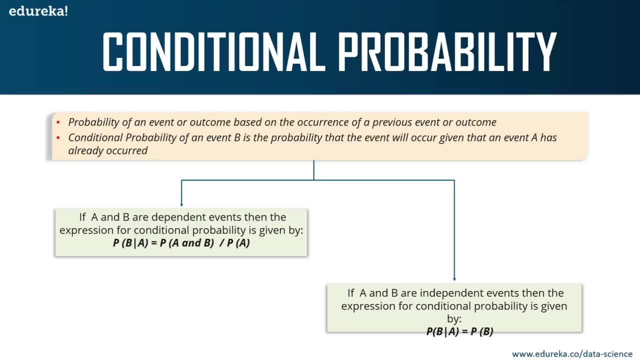 So, like I said, if A and B are dependent events, then this is the expression, But if A and B are independent events, then the expression for conditional probability is like this: right? So, guys, P of A and P of B is obviously. 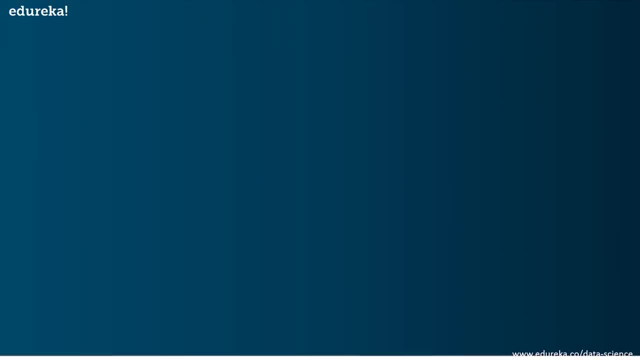 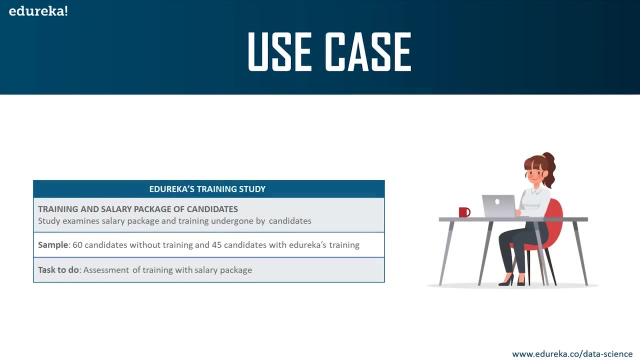 the probability of A and probability of B. right Now, let's move on. Now, in order to understand conditional probability, joint probability and marginal probability, let's look at a small use case. okay, Now, basically, we're gonna take a data set. 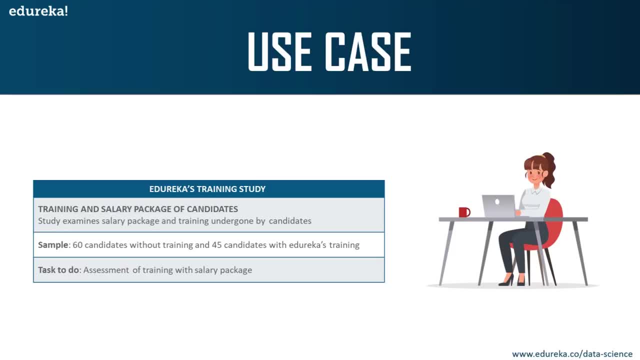 which examines the salary package and training undergone by candidates. okay, Now in this there are 60 candidates without training and 45 candidates which have enrolled for Edureka's training right Now. the task here is you have to assess the training with the salary package. 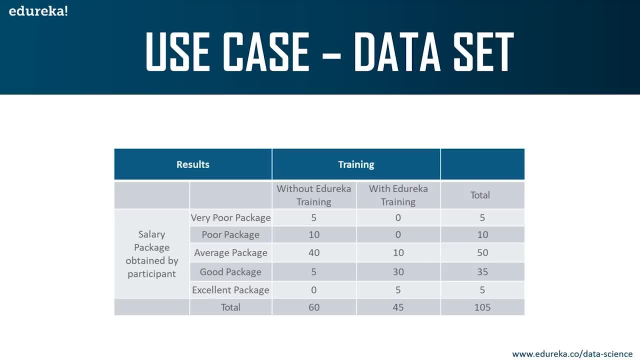 Okay, let's look at this in a little more depth. So in total, we have 105 candidates, out of which 60 of them have not enrolled for Edureka's training and 45 of them have enrolled for Edureka's training. 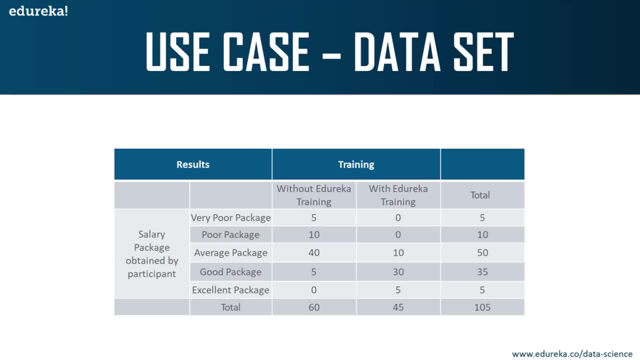 All right, this is a small survey that was conducted and this is the rating of the package or the salary that they got right. So if you read through the data, you can understand. There were five candidates without Edureka training. There were five candidates without Edureka training. 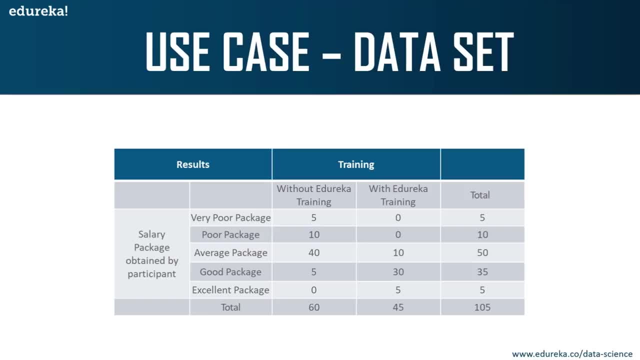 who got a very poor salary package- Okay. similarly, there are 30 candidates with Edureka training who got a good package, right. So, guys, basically you're comparing the salary package of a person depending on whether or not they've enrolled for Edureka training, right? 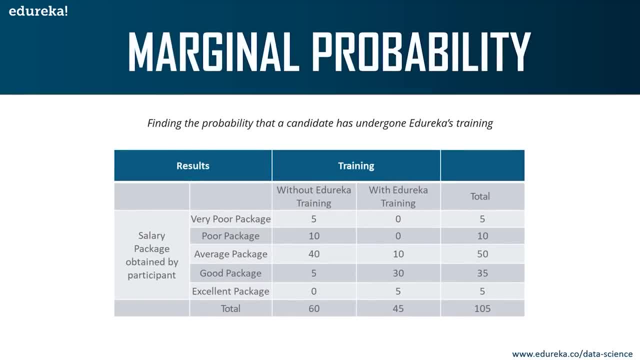 This is our data set. Now let's look at our problem statement. Find the probability that a candidate has undergone Edureka's training Quite simple. Which type of probability is this? This is marginal probability. This is marginal probability, right? So the probability that a candidate 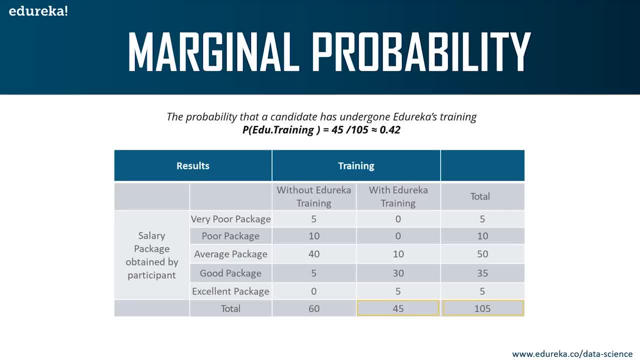 has undergone Edureka's training is obviously 45 divided by 105, since 45 is the number of candidates with Edureka training and 105 is the total number of candidates. So you get a value of approximately 0.42.. All right, that's the probability of a candidate. 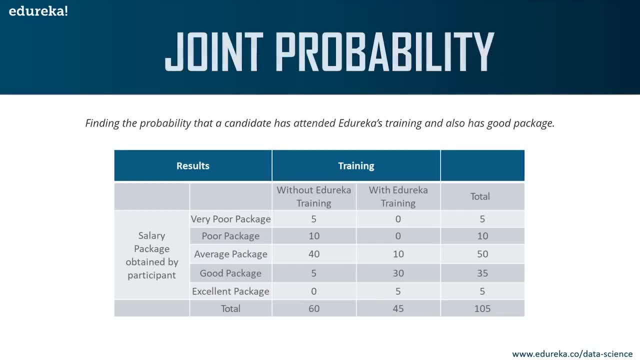 that has undergone Edureka's training. Next question: Find the probability that a candidate has attended Edureka's training and also has good training. Find the probability that a candidate has attended Edureka's training and also has good training. Find the probability that a candidate has attended Edureka's training and also has good training. 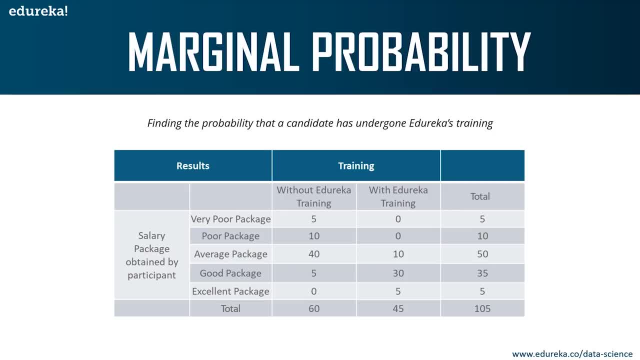 edureka's training. quite simple: which type of probability is this? this is marginal probability, right? so the probability that a candidate has undergone edureka's training is obviously 45 divided by 105, since 45 is the number of candidates with edureka training and 105 is. 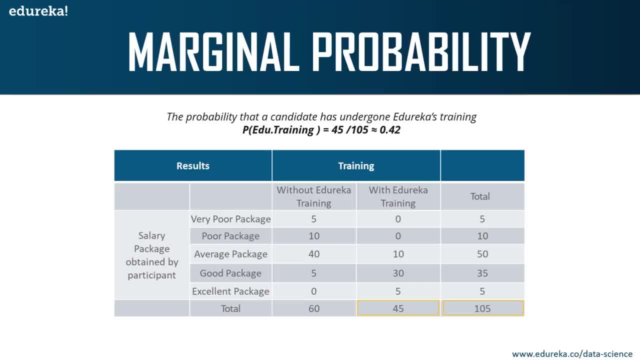 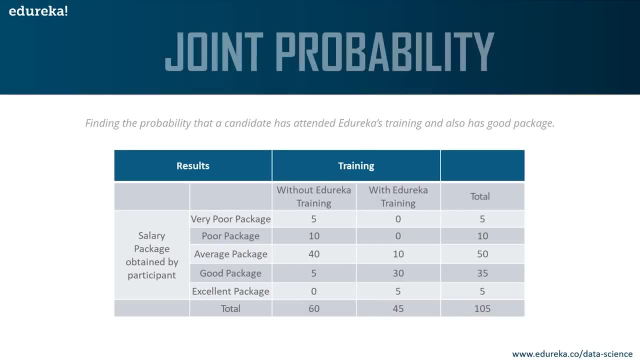 the total number of candidates. so you get a value of approximately 0.42. all right, that's the probability of a candidate that has undergone edureka's training. next question: find the probability that a candidate has attended edureka's training and also has good package. 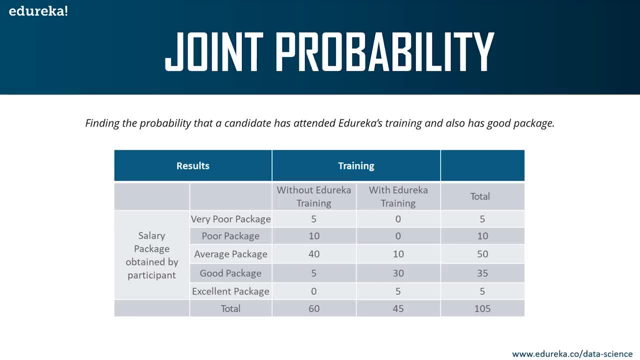 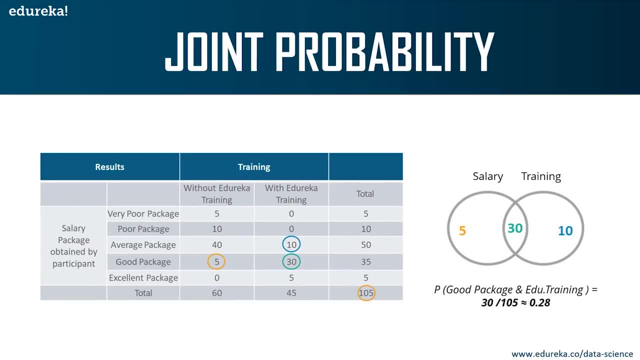 now, this is obviously a joint probability problem, right? so how do you calculate this? now, since our table is quite formatted, we can directly find that people who have gotten a good package along with edureka training are 30, right? so out of 105 people, 30 people have a edureka training. 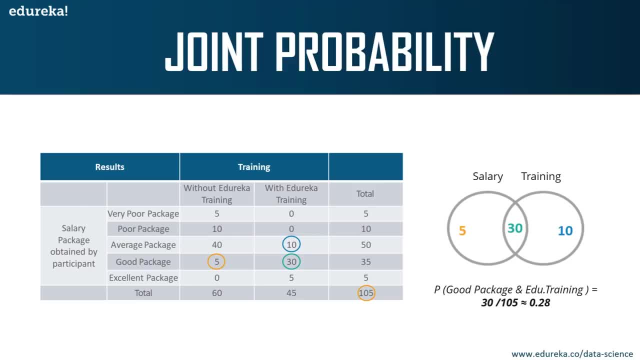 and a good package, right, they're specifically asking for people with training. remember that right. the question is: find the probability that a candidate has attended edureka's training and also has a good package alright, so we need to consider two factors. that is, a candidate who's 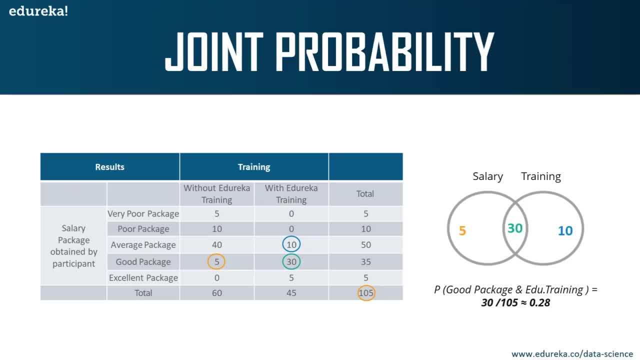 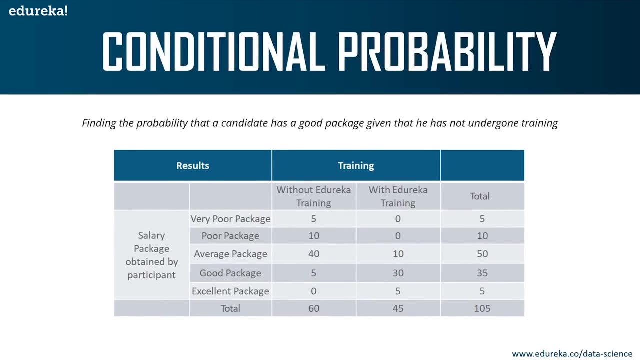 attended edureka's training and who has a good package. so clearly, that number is 30, 30 divided by total number of candidates, which is 105, right? so here you get the answer clearly. next, we have find the probability that a candidate has a good package given that he has not undergone training. okay, now this is. 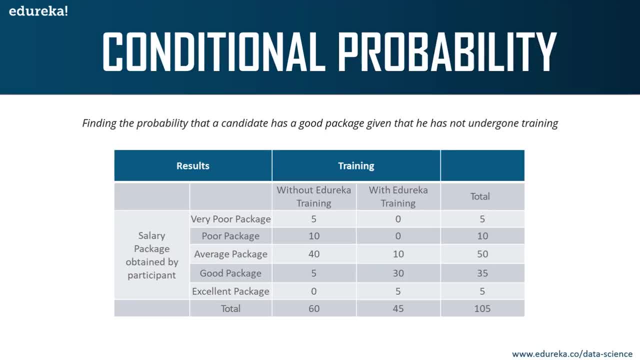 clearly conditional probability, because here you're defining a condition. you're saying that you want to find the probability of a candidate who has a good package, given that he's not undergone any training. right, the condition is that he's not undergone any training, alright, so the number of people 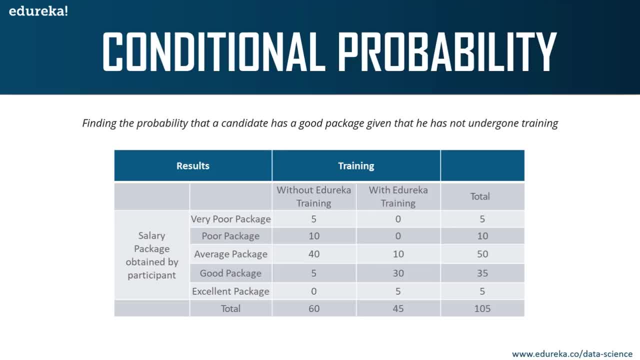 who have not undergone training are 60, and out of that, five of them have got a good package right. so that's why this is 5 by 60 and not 5 by 105, because here they've clearly mentioned has a good package, given that he has not undergone training. so you have to only consider: 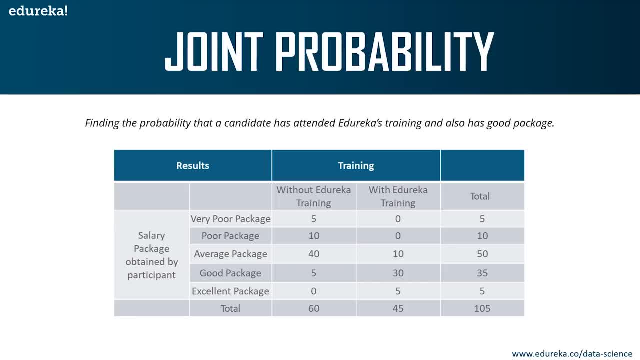 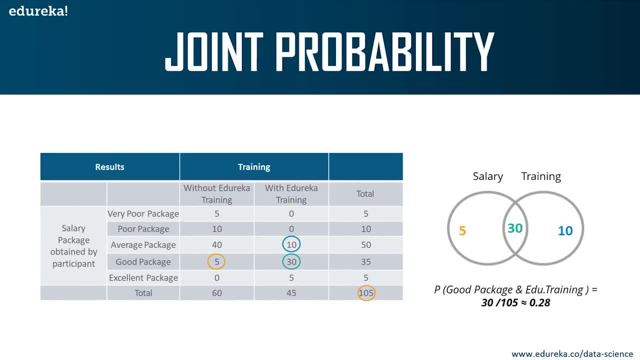 Now, this is obviously a joint probability problem, right? So how do you calculate this? Now, since our table is quite formatted, we can directly find that people who have gotten a good package along with Edureka training are 30, right? So, out of 105 people, 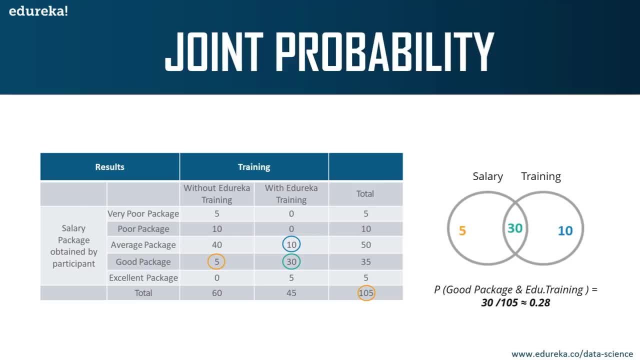 30 people have Edureka training and a good package. right, They're specifically asking for people with Edureka training. remember that, right? The question is: find the probability that a candidate has attended Edureka's training, that a candidate has attended Edureka's training. 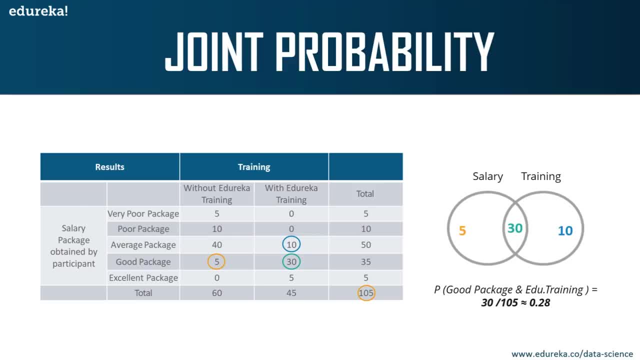 and also has a good package, all right. So you need to consider two factors, that is, a candidate who's attended Edureka's training and who has a good package. So clearly, that number is 30, 30 divided by total number of candidates, which is 105, right. 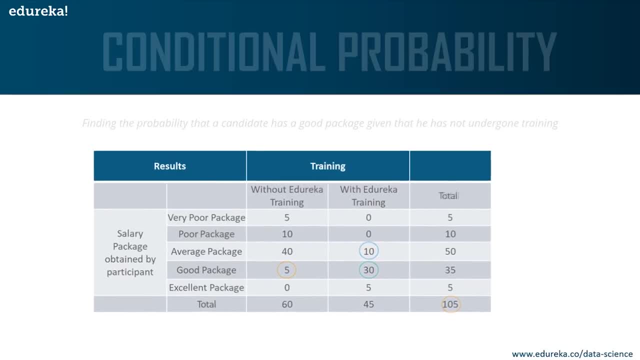 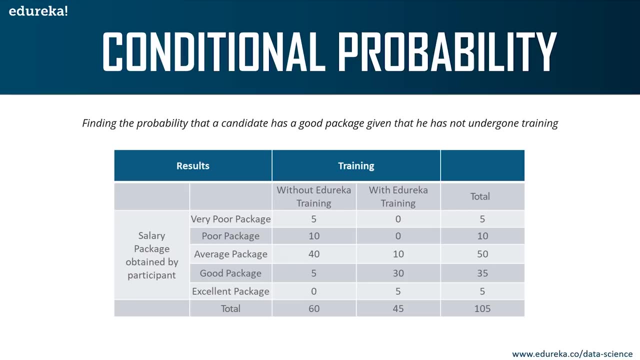 So here you get the answer clearly. Next, we have find the probability that a candidate has a good package, given that he has not undergone training. Okay now, this is clearly conditional probability. Okay now, this is clearly conditional probability because here you're defining a condition. 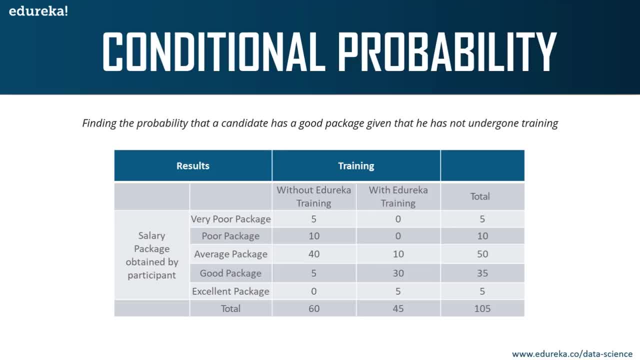 You're saying that you want to find the probability of a candidate who has a good package, given that he's not undergone any training. right, The condition is that he's not undergone any training. All right, so the number of people who have not undergone training are 60. 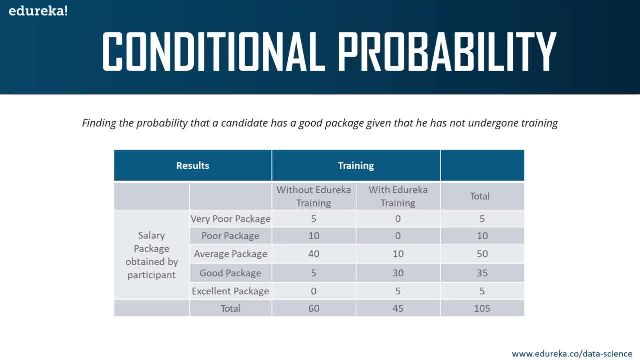 and out of that, five of them have got a good package right. So that's why this is five by 60 and not five by 105, because here they've clearly mentioned has a good package, given that he has not undergone training. So you have to only consider people. 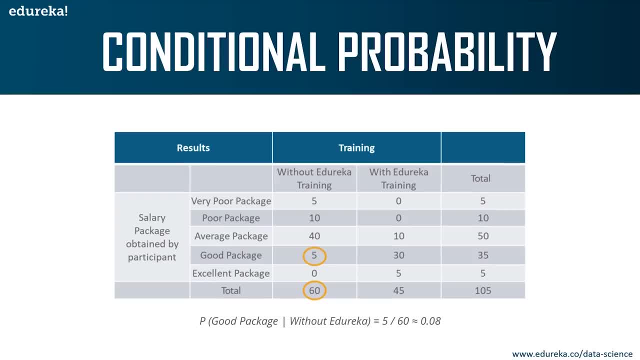 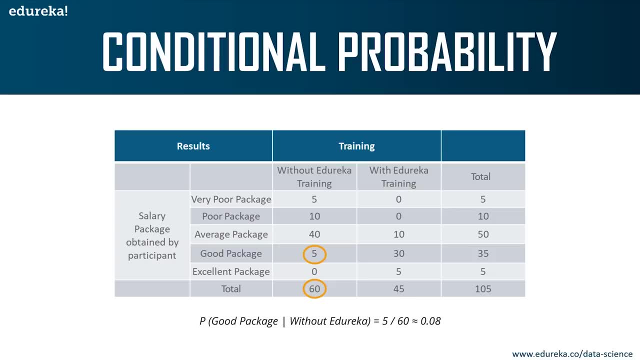 who have not undergone training, right? So only five people who have not undergone training have gotten a good package, right? So five divided by 60, you get a probability of around 0.08, which is pretty low, right? Okay, so this was all about. 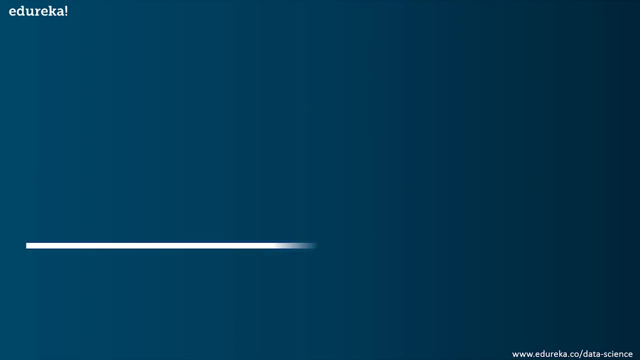 the different types of probability. Now let's move on and look at our last topic in probability, which is Bayes' theorem. Now, guys, Bayes' theorem is a very important concept when it comes to statistics and probability. It is majorly used in naive bias algorithm. 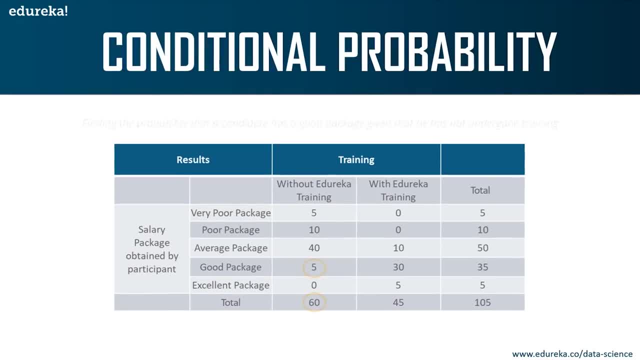 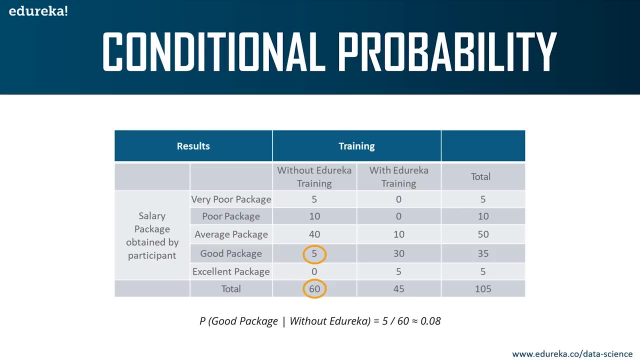 people who have not undergone training, right. so only five people who have not undergone training have gotten a good package, right. so 5 divided by 60, you get a probability of around 0.08, which is pretty low, right. okay, so this was all about the different types of probability. 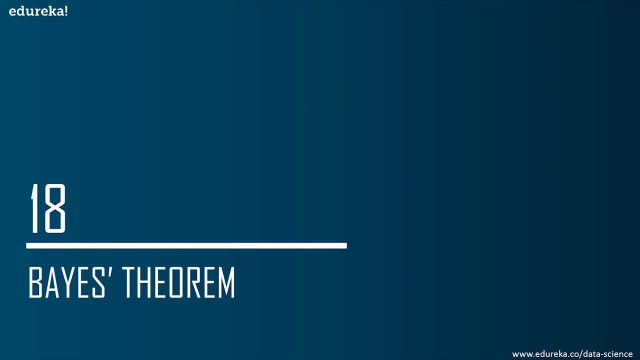 now let's move on and look at our last topic in probability, which is Bayes theorem. now, guys, Bayes theorem is a very important concept when it comes to statistics and probability. it is majorly used in knife bias algorithm. those of you who aren't aware, knife bias is a supervised learning. 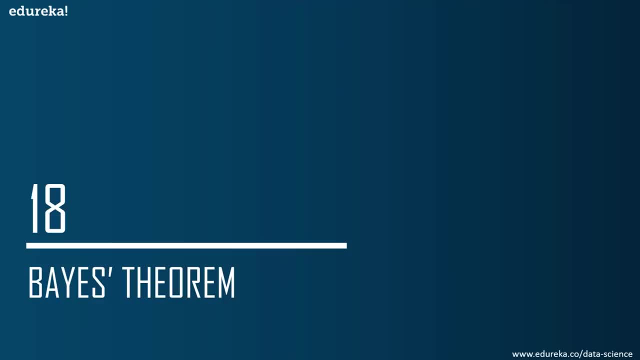 classification algorithm, and it is mainly used in Gmail spam filtering right. a lot of you might have noticed that if you open up Gmail, you'll see that you have a folder called spam right. all of that is carried out through machine learning, and the algorithm used there is naive bias right. so now let's discuss what exactly the bias theorem. 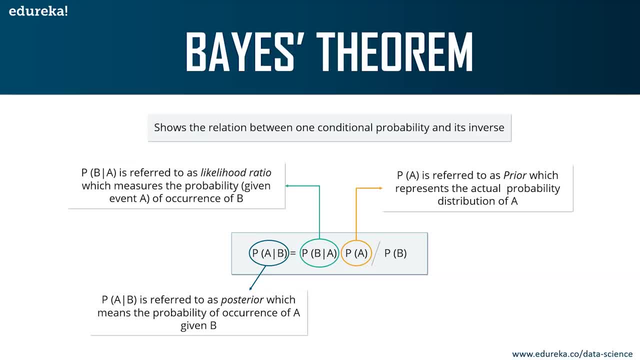 is and what it denotes. the bias theorem is used to show the relation between one conditional probability and its inverse. all right, basically, it's nothing but the probability of an event occurring, based on prior knowledge of conditions that might be related to the same event. okay, so mathematically the bell theorem is represented like this right, like shown in. 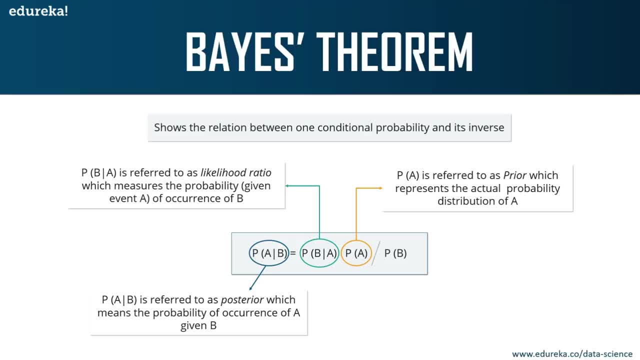 this equation, the left hand term is referred to as the likelihood ratio, which measures the probability of occurrence of event b, given an event a, okay, on the left hand side is what is known as the posterior. right is referred to as posterior, which means that the probability of occurrence of hacen is not given during bias. 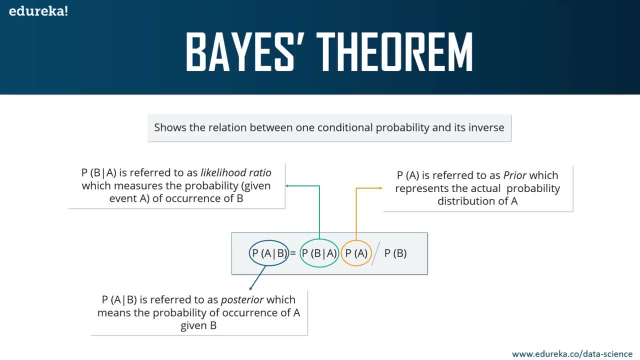 of A given an event B right. The second term is referred to as the likelihood ratio. All right. this measures the probability of occurrence of B given an event A. Now, P of A is also known as the prior, which refers to the actual probability distribution of A. 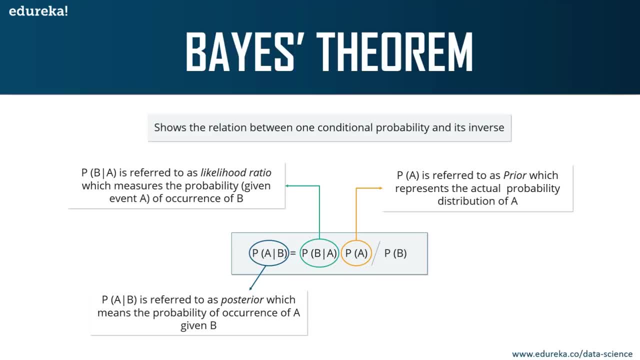 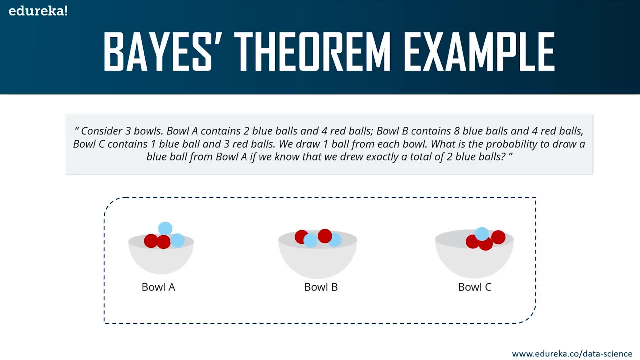 and P of B is again the probability of B, right. This is the Bayes theorem. Now, in order to better understand the Bayes theorem, let's look at a small example. Let's say that we have three bowels. We have bowl A, bowl B and bowl C. 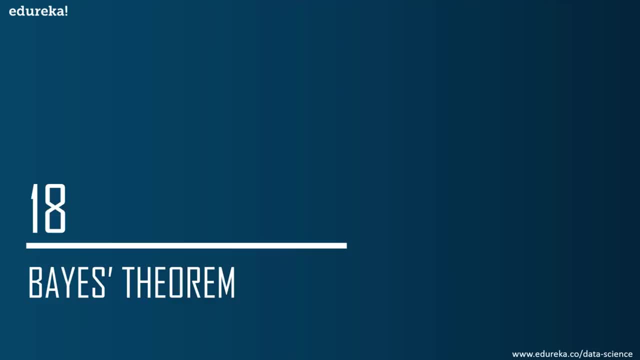 Those of you who aren't aware, naive bias is a supervised learning classification algorithm and it is mainly used in Gmail spam filtering right. A lot of you might have noticed that if you open up Gmail, you'll see that you have a folder called spam right. 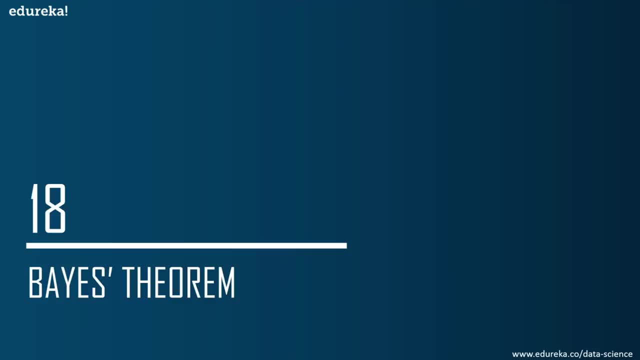 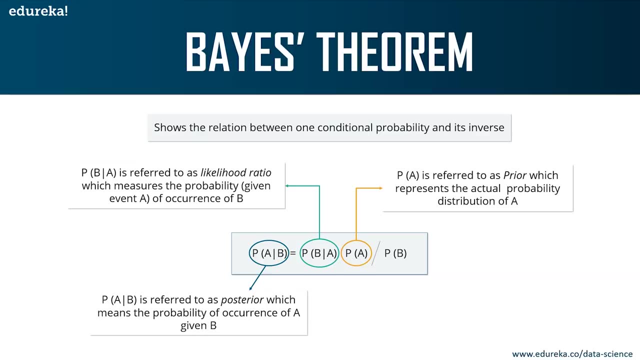 All of that is carried out through machine learning and the algorithm used. there is naive bias right. So now let's discuss what exactly the Bayes' theorem is and what it denotes. The Bayes' theorem is used to show the relation between one conditional probability and its inverse right. 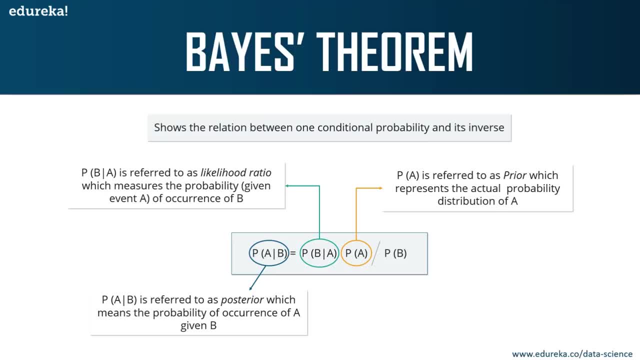 Basically, it's nothing but the probability of an event occurring, based on prior knowledge of conditions that might be related to the same event. Okay, so mathematically, the Bayes' theorem is represented like this: All right, like shown in this equation. 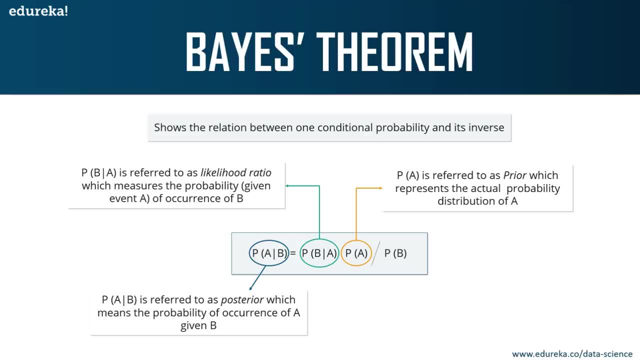 The left-hand term is referred to as the likelihood ratio, which measures the probability of occurrence of event B given an event A. okay, On the left-hand side is what is known as the posterior. All right, it is referred to as posterior, which means that the probability of occurrence of A. 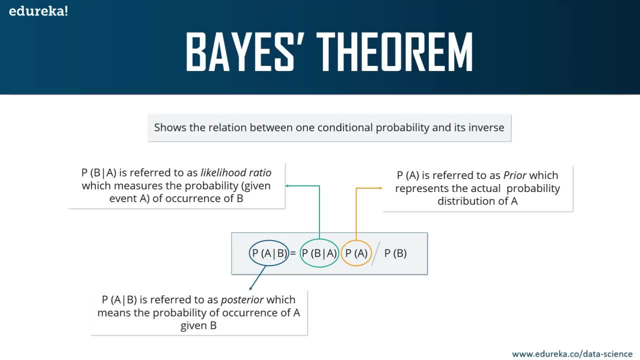 given an event B right. The second term is referred to as the likelihood ratio. All right, this measures the probability of occurrence of B given an event A. Now, P of A is also known as the prior, which refers to the actual probability distribution of A. 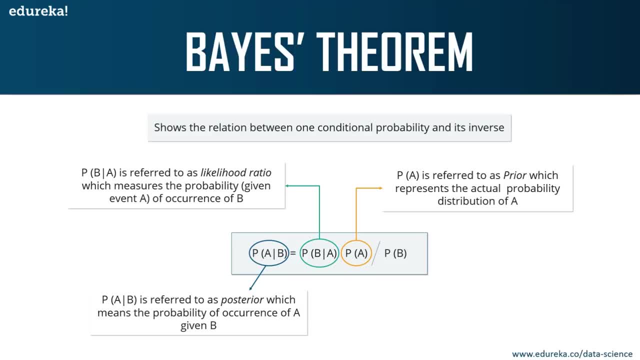 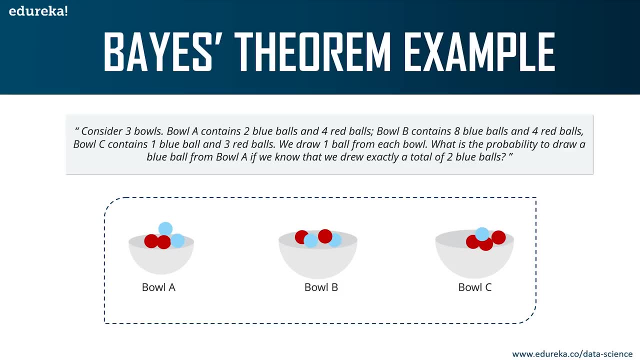 and P of B is again the probability of B right. This is the Bayes' theorem. Now, in order to better understand the Bayes' theorem, let's look at a small example. Let's say that we have three bowels. 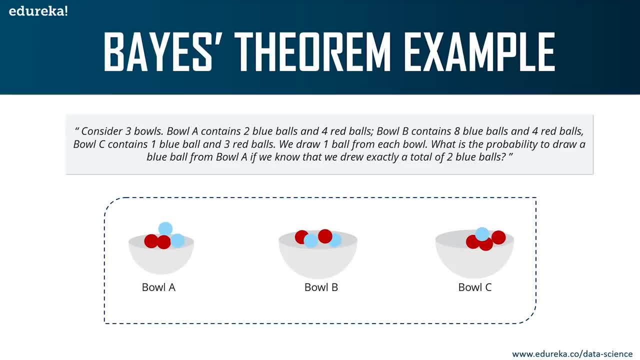 We have bowl A, bowl B and bowl C. Okay, bowl A contains two blue balls and four red balls. Bowl B contains eight blue balls and four red balls. Bowl C contains one blue ball and three red balls. Now, if we draw one ball from each bowl, 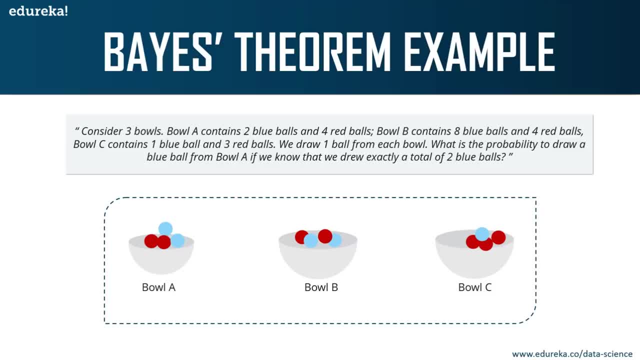 what is the probability to draw a blue ball from a bowl A if we know that we drew exactly a total of two blue balls, Right? if you didn't understand the question, please reread it. I shall pause for a second or two. 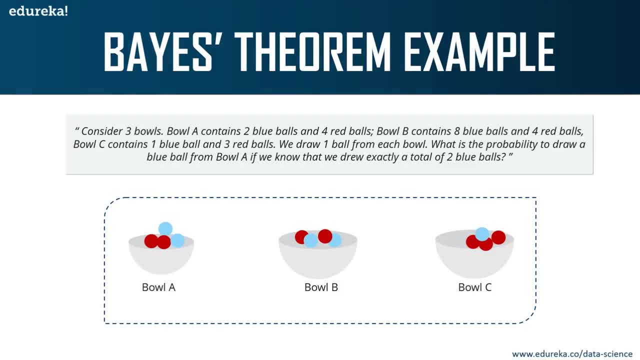 Okay, bowl A contains two blue balls and four red balls. Bowl B contains eight blue balls and four red balls. Bowl C contains one blue ball and three red balls. Now, if we draw one ball from each bowl, what is the probability to draw a blue ball from a bowl A? 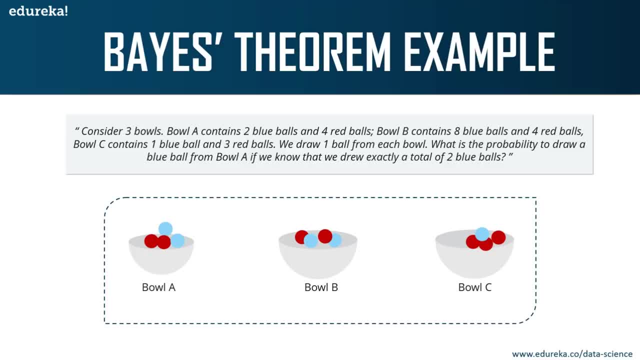 if we know that we drew exactly a total of two blue balls, Right? if you didn't understand the question, please re-read it. I shall pause for a second or two, Right? so I hope all of you have understood the question. 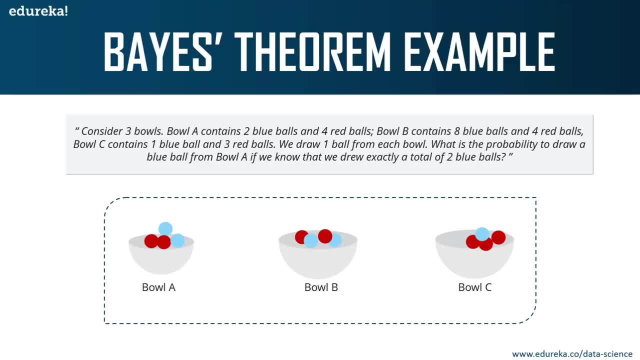 Okay, now what I'm gonna do is I'm gonna draw a blueprint for you and tell you how exactly to solve the problem. but I want you all to give me the solution to this problem. right? I'll draw a blueprint, I'll tell you what exactly the steps are. 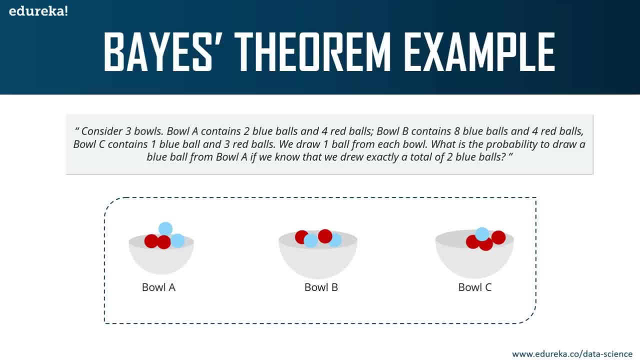 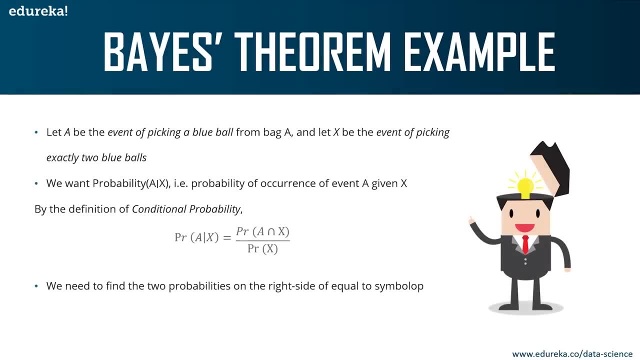 but I want you to come up with a solution on your own right. The formula is also given to you. Everything is given to you. All you have to do is come up with a final answer. All right, let's look at how you can solve this problem. 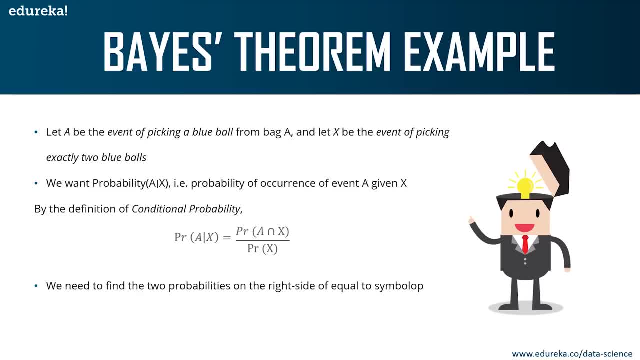 So, first of all, what we'll do is: let's consider A. All right, let A be the event of picking a blue ball from bag A and let X be the event of picking exactly two blue balls. right, Because these are the two events. 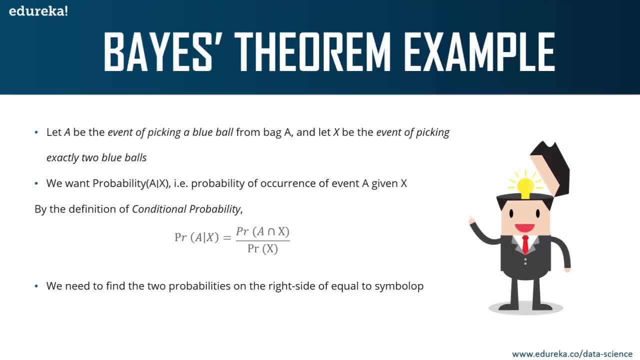 that we need to calculate the probability of Now. there are two probabilities that you need to consider here. One is the event of picking a blue ball from bag A, and the other is the event of picking exactly two blue balls. Okay, So these two are represented by A and X respectively. 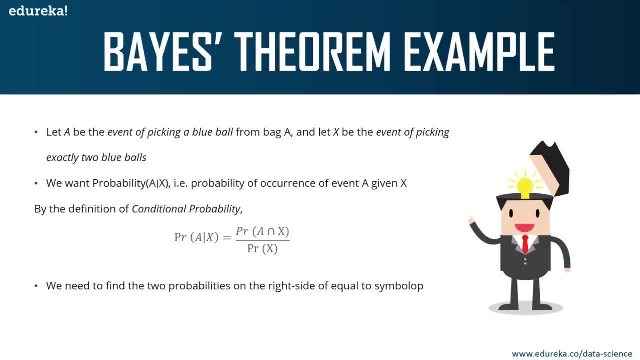 So what we want is the probability of occurrence of event A given X, which means that, given that we're picking exactly two blue balls, what is the probability that we are picking a blue ball from bag A? So, by the definition of conditional probability, 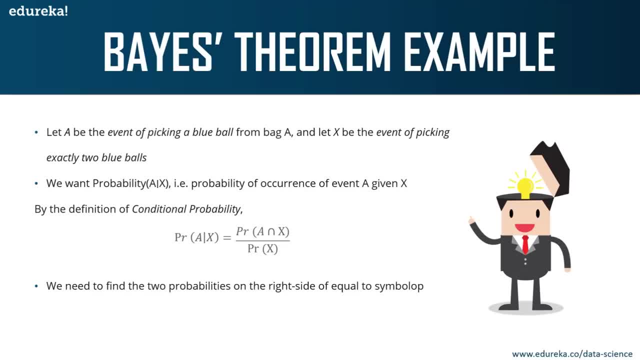 this is exactly what our equation will look like, correct? This is basically occurrence of event A given an event X, and this is the probability of A and X, and this is the probability of X alone, correct? Now what we need to do is we need to find: 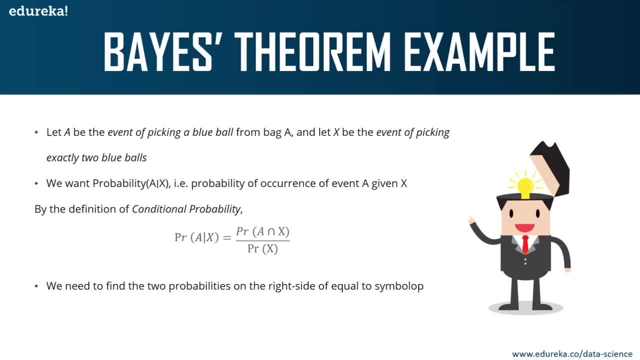 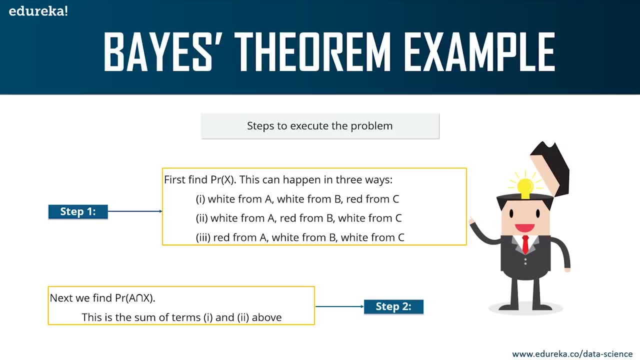 these two probabilities, which is probability of A and X occurring together and probability of X. okay, This is the entire solution. So how do you find the probability of X? This you can do in three ways. So first is white ball from A. 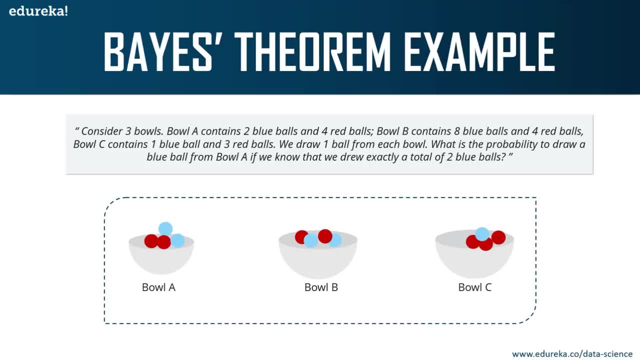 Right, so I hope all of you have understood the question. Okay, now what I'm gonna do is I'm gonna do draw a blueprint for you and tell you how exactly to solve the problem, but I want you all to give me the solution to this problem. 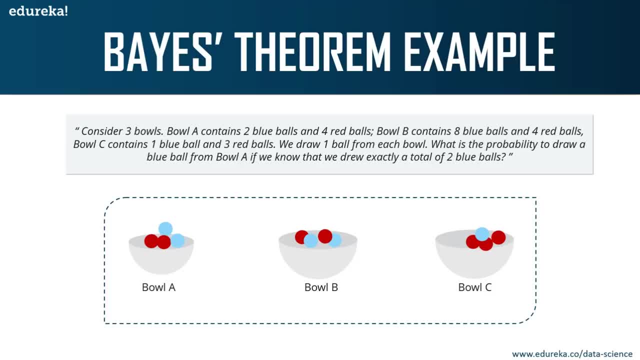 Right, I'll draw a blueprint, I'll tell you what exactly the steps are, but I want you to come up with a solution on your own Right. the formula is also given to you. Everything is given to you. All you have to do is come up with a final answer. 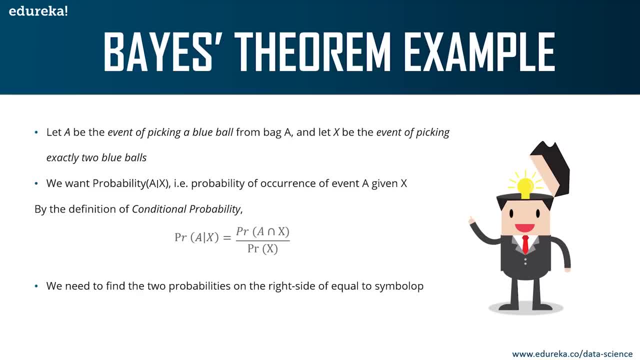 Right, let's look at how you can solve this problem. So, first of all, what we'll do is: let's consider A. All right, let A be the event of picking a blue ball from bag A. Let X be the event of picking exactly two blue balls. 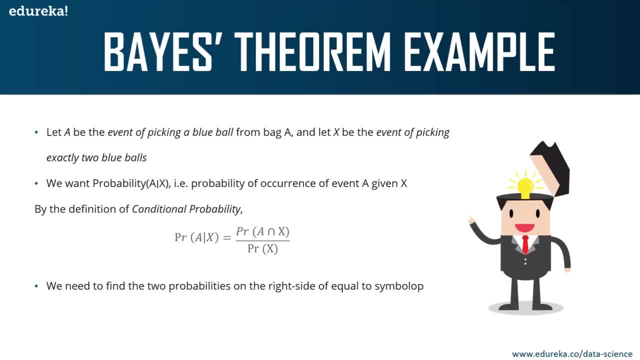 Right, because these are the two events that we need to calculate the probability of. Now. there are two probabilities that you need to consider here. One is the event of picking a blue ball from bag A and the other is the event of picking 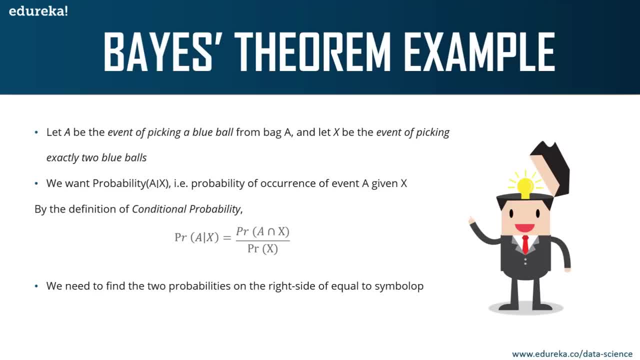 exactly two blue balls. okay, So these two are represented by A and X respectively. So what we want is the probability of occurrence of event A given X, which means that, given that we're picking exactly two blue balls, what is the probability that we are picking? 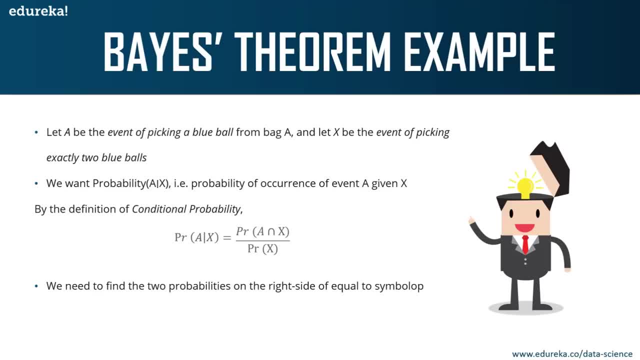 a blue ball from bag A. So, by the definition of conditional probability, this is exactly what our equation will look like, correct? This is basically occurrence of event A given an event X, and this is the probability of A and X, and this is the probability of X alone, correct? 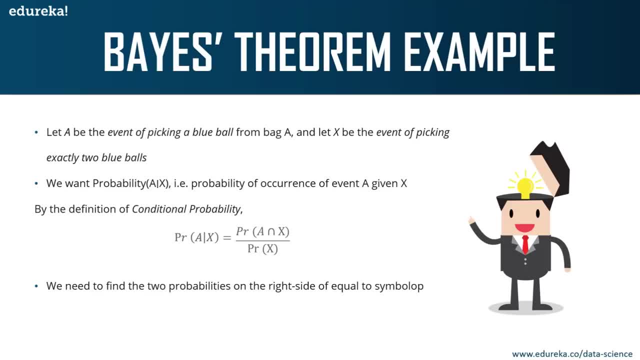 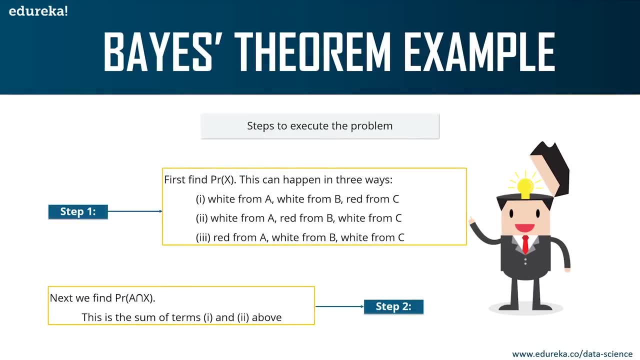 Now what we need to do is we need to find these two probabilities, which is probability of A and X occurring together And probability of X. okay, This is the entire solution. So how do you find the probability of X? This you can do in three ways. 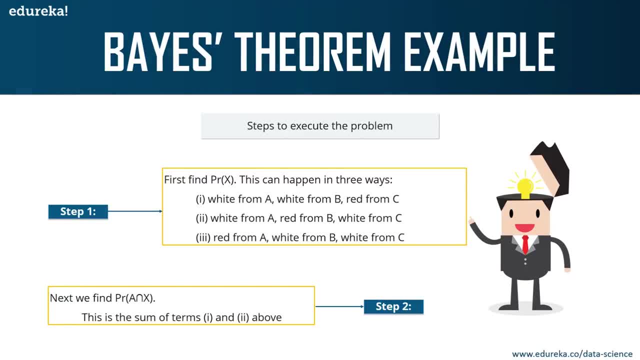 So first is white ball from A, either white from B or red from C. Now, first is to find the probability of X. X basically represents the event of picking exactly two blue balls, right? So these are the three ways in which it is possible. 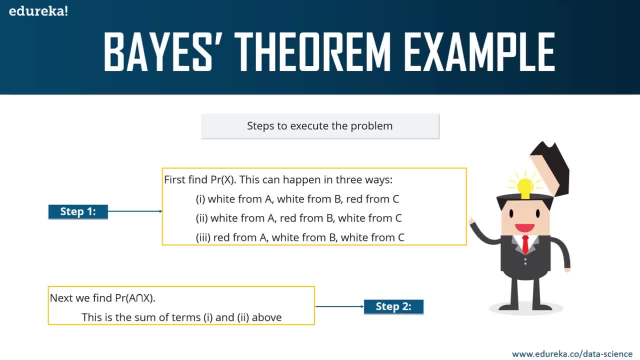 So you'll pick one blue ball from bowl A and one from bowl B. In the second case, you can pick one from A and another blue ball from C. In the third case, you can pick a blue ball from bag B. 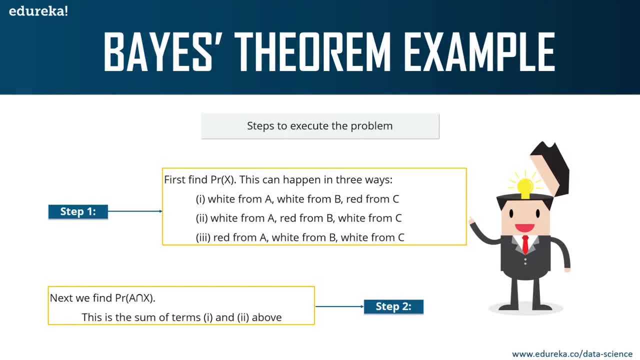 either white from B or red from C. Now, first is to find the probability of X. Now, first is to find the probability of X. Now, first is to find the probability of X. X basically represents the event of picking exactly two blue balls right. 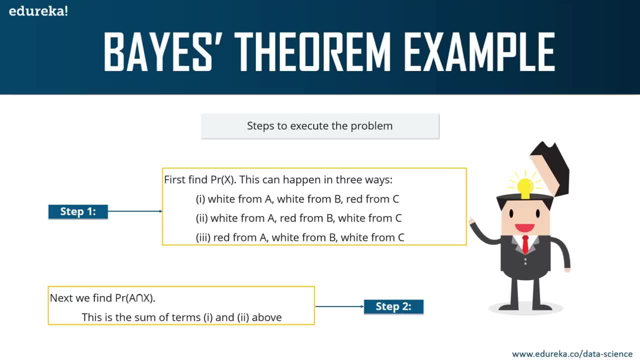 So these are the three ways in which it is possible. So you'll pick one blue ball from bowl A and one from bowl B. In the second case, you can pick one from A and another blue ball from C. In the third case, you can pick a blue ball from bag B. 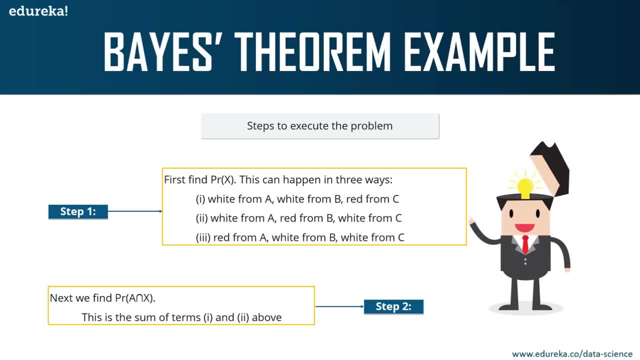 and a blue ball from bag C right. These are the three ways in which it is possible, so you need to find the probability of each of this. Step two is that you need to find the probability of A and X occurring together. This is the sum of terms one and two. 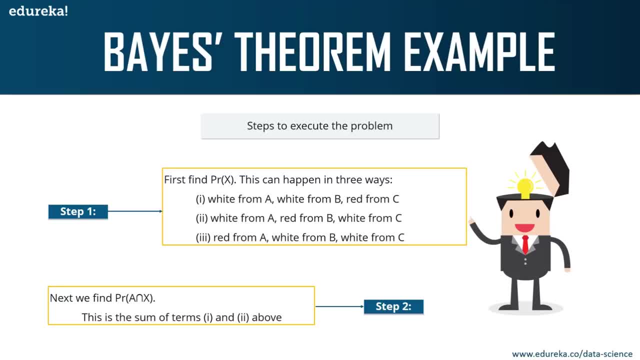 Okay, this is because in both of these events you're picking a ball from bag A, correct? So, guys, find out this probability and let me know your answer in the comment section. All right, we'll see if you get the answer right. 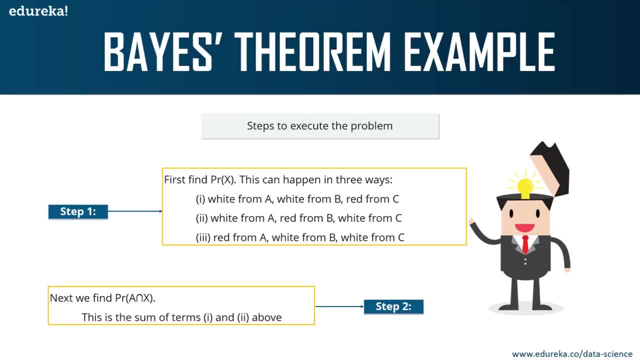 I gave you the entire solution to this. All you have to do is substitute the value, right? If you want a second or two, I'm gonna pause on the screen so that you can go through this in a more clearer way, all right? 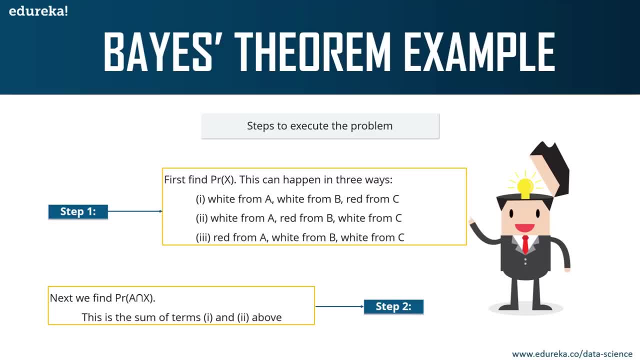 Remember that you need to calculate two probabilities. The first probability that you need to calculate is the event of picking a blue ball from bag A, given that you're picking exactly two blue balls, okay. The second probability you need to calculate is the event of picking exactly two blue balls, all right. 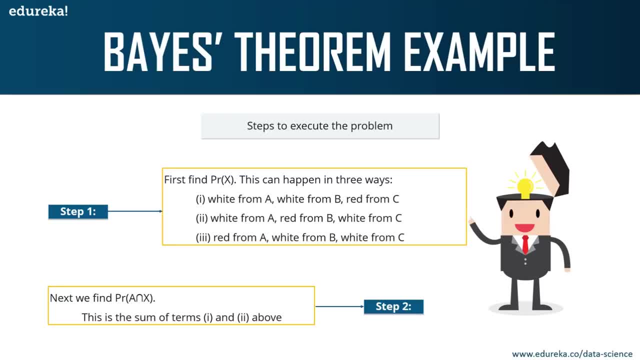 These are the two probabilities you need to calculate. so remember that and this is the solution. All right, so, guys, make sure you mention your answers in the comment section. For now, let's move on and look at our next topic. 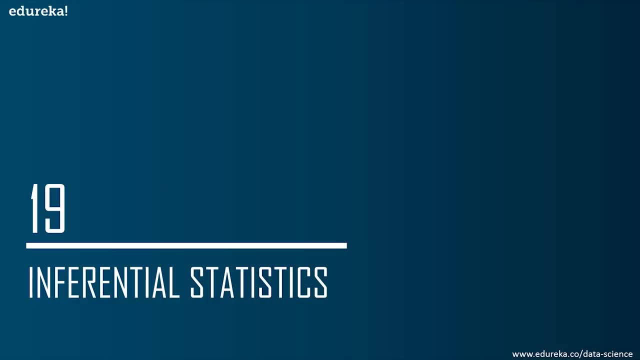 which is the inferential statistics. So, guys, we just completed the probability module. right Now we'll discuss inferential statistics, which is the second type of statistics. We discussed descriptive statistics earlier. all right, So, like I mentioned earlier, inferential statistics. 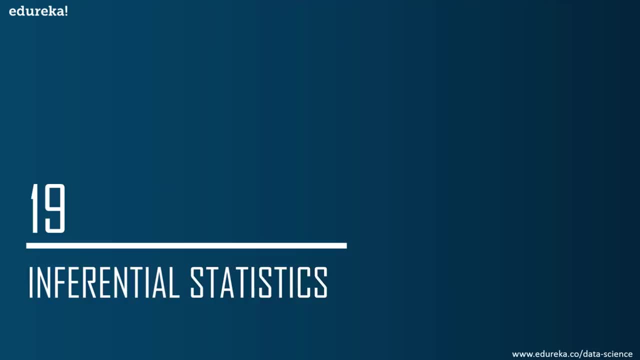 also known as statistical inference, is a branch of statistics that deals with forming inferences and predictions about a population based on a sample of data taken from the population. all right, Now the question you should ask is: how does one form inferences or predictions on a sample? 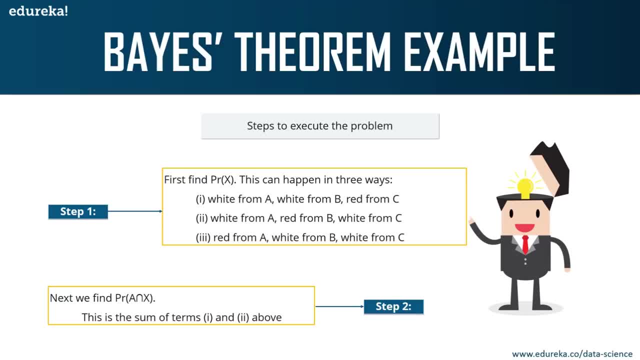 and a blue ball from bag C right. These are the three ways in which it is possible, so you need to find the probability of each of this. Step two is that you need to find the probability of A and X occurring together. This is the sum of terms one and two. okay, 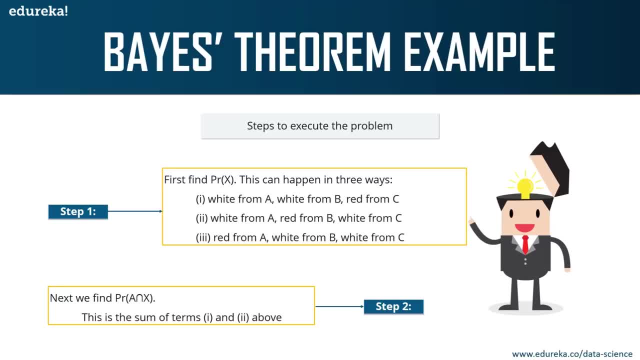 This is because in both of these events, you're picking a ball from bag A, correct? So, guys, find out this probability and let me know your answer in the comment section. all right, We'll see if you get the answer right. 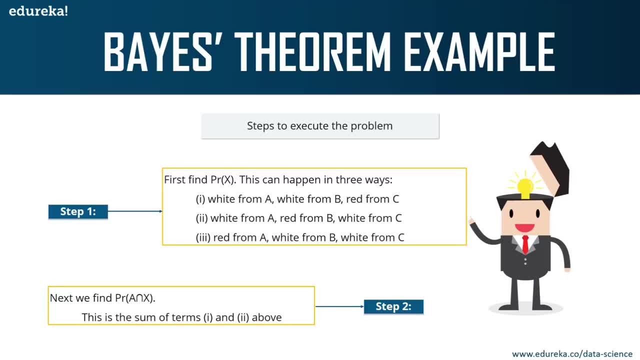 I gave you the entire solution to this. All you have to do is substitute the value, right? If you want a second or two, I'm gonna pause on the screen so that you can go through this in a more clearer way, All right? 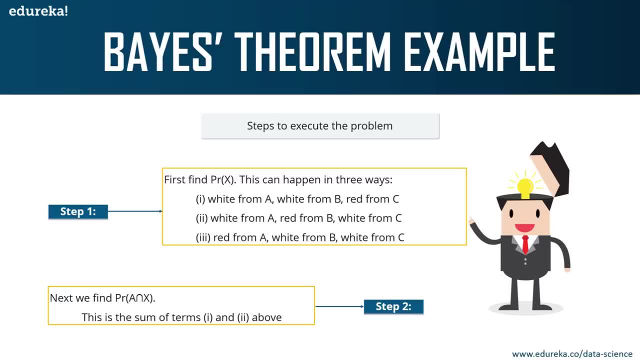 Remember that you need to calculate two probabilities. The first probability that you need to calculate is the event of picking a blue ball from bag A, given that you're picking exactly two blue balls, okay. The second probability you need to calculate is the event of picking exactly two blue balls, all right. 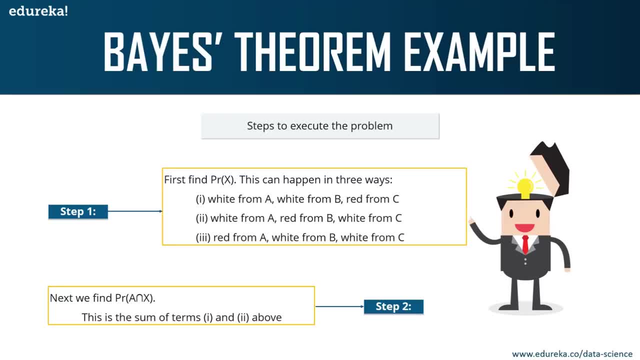 These are the two probabilities you need to calculate. so remember that and this is the solution. All right, so, guys, make sure you mention your answers in the comment section. For now, let's move on and look at our next topic. 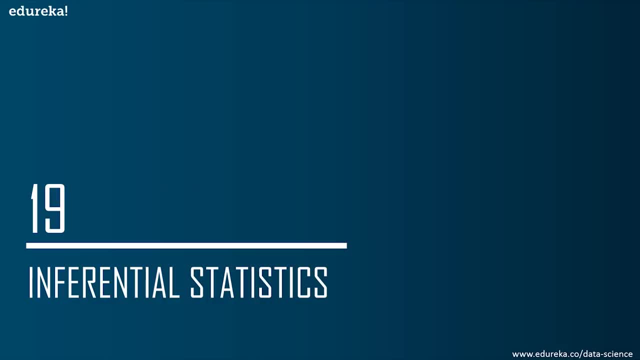 which is the inferential statistics. So, guys, we just completed the probability module. right Now we'll discuss inferential statistics, which is the second type of statistics. We discussed descriptive statistics earlier. all right, So, like I mentioned earlier, inferential statistics. 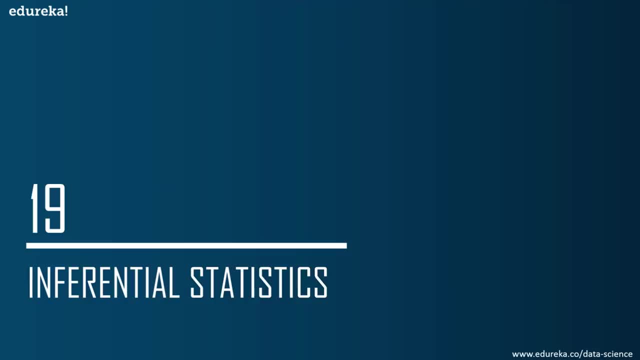 also known as statistical inference, is a branch of statistics that deals with forming inferences and predictions about a population based on a sample of data taken from the population. all right, And the question you should ask is: how does one form inferences or predictions on a sample? 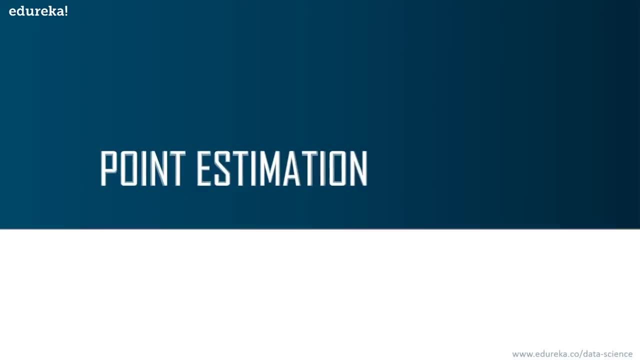 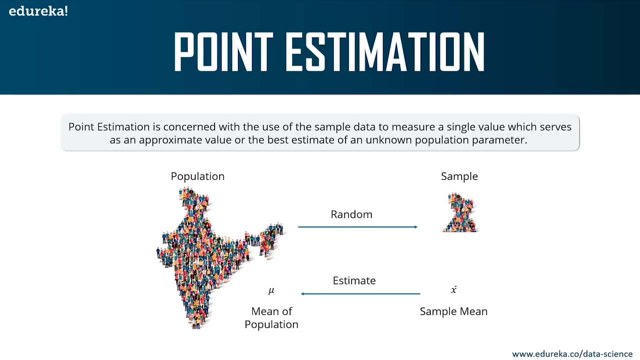 The answer is you use point estimation. okay, Now you must be wondering: what is point estimation? Point estimation is concerned with the use of the sample data to measure a single value which serves as an approximate value or the best estimate of an unknown population parameter. 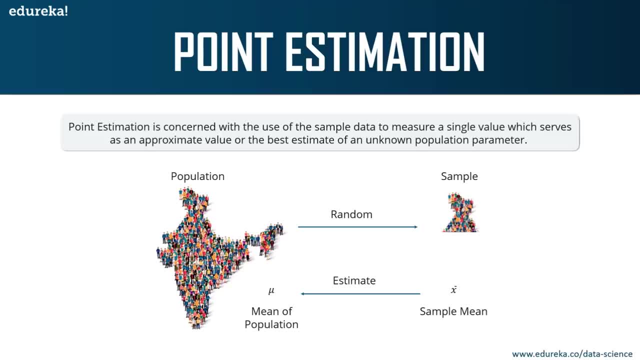 That's a little confusing. let me break it down to you. For example, in order to calculate the mean of a huge population, what we do is we first draw out the sample of the population and then we find the sample mean right. 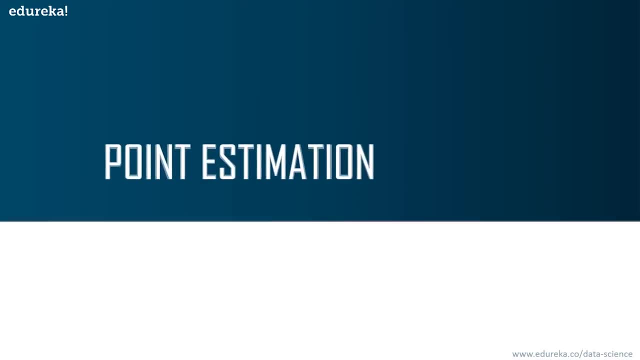 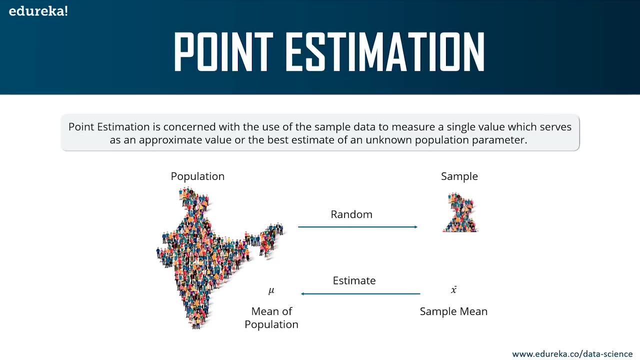 The answer is you use point estimation. okay, Now you must be wondering: what is point estimation? Point estimation is concerned with the use of the sample data to measure a single value which serves as an approximate value or the best estimate of an unknown population parameter. 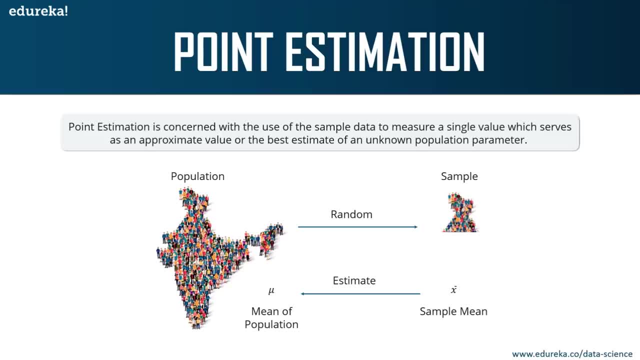 That's a little confusing. let me break it down to you. For example, in order to calculate the mean of a huge population, what we do is we first draw out the sample of the population and then we find the sample mean right. 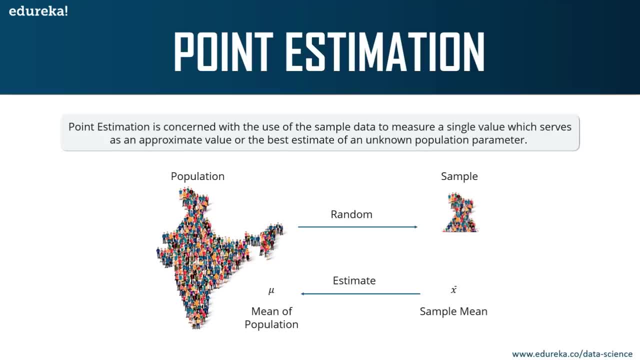 The sample mean is then used to estimate the population mean. This is basically point estimate. You're estimating the value of one of the parameters of the population, right, Basically the mean. you're trying to estimate the value of the mean. This is what point estimation is. 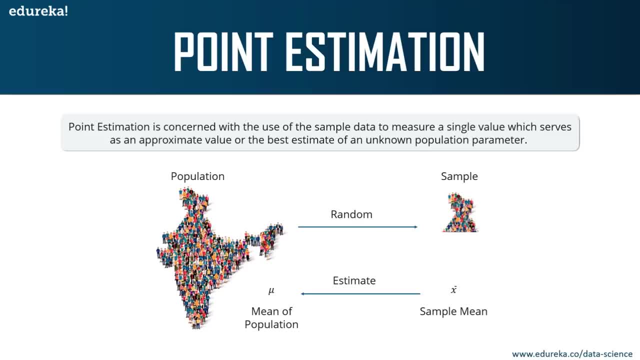 The two main terms in point: estimation. there's something known as the estimator and there's something known as the estimate. Estimator is a function of the sample that is used to find out the estimate. all right, In this example it's basically the sample mean, right. 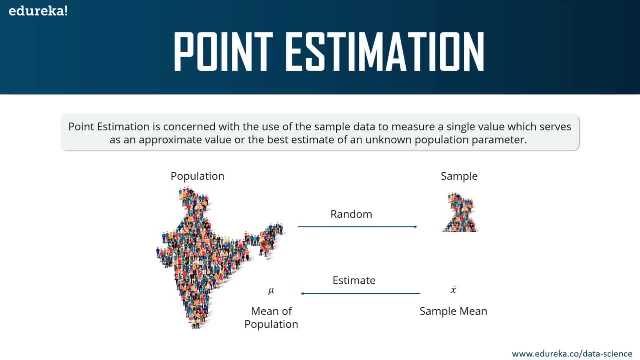 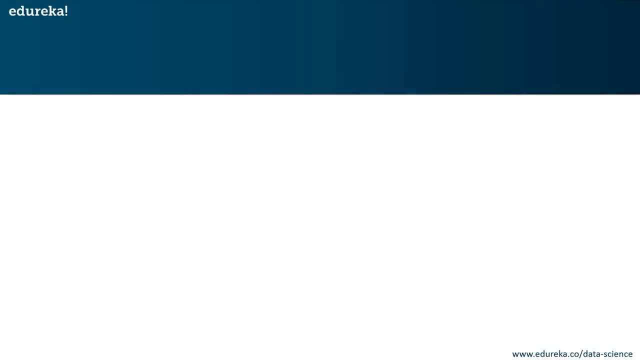 So a function that calculates the sample mean is known as the estimator, and the realized value of the estimator is the estimate right? So I hope point estimation is clear. Now how do you find the estimates? There are four common ways in which you can do this. 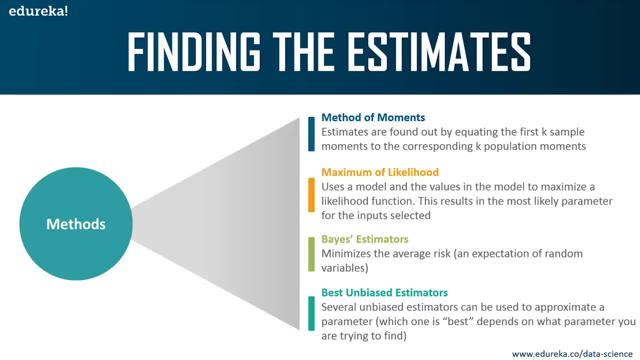 The first one is method of moments. Here, what you do is you form an equation in the sample data set and then you analyze a similar equation in the population data set as well, like the population, mean, population variance and so on. So, in simple terms, what you're doing is: 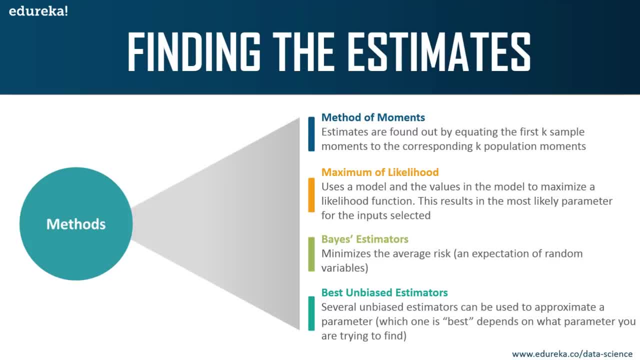 you're taking down some known facts about the population and you're extending those ideas to the sample. all right, Once you do that, you can analyze the sample and estimate more essential or more complex values right. Next we have maximum of likelihood. 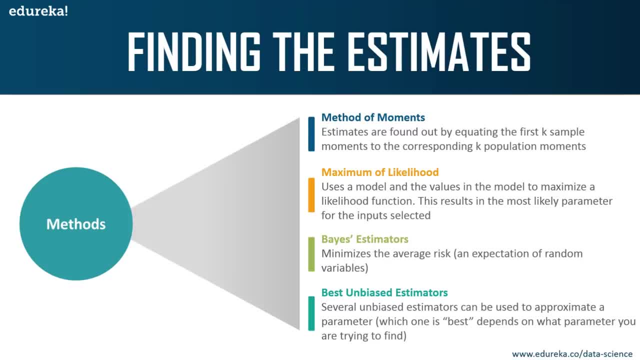 Now, this method basically uses a model to estimate a value. all right, Now, maximum of likelihood is majorly based on probability, so there's a lot of probability involved in this method. Next we have the Bayes estimator. This works by minimizing the errors or the average risk. okay, 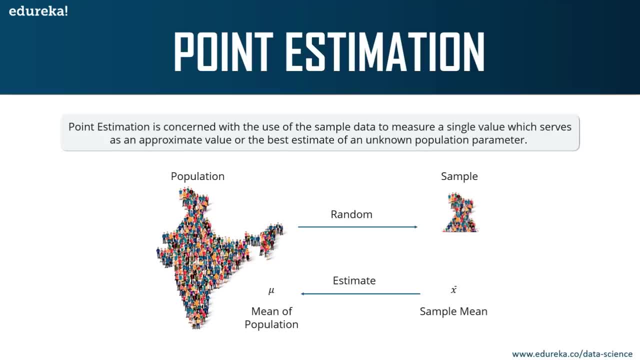 The sample mean is then used to estimate the population mean. This is basically point estimate. You're estimating the value of one of the parameters of the population, right, Basically the mean. you're trying to estimate the value of the mean. This is what point estimation is. 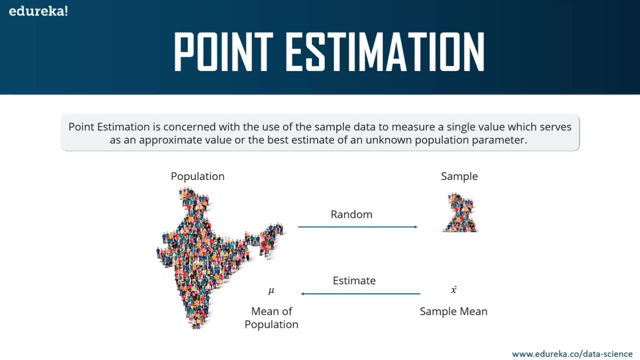 The two main terms in point: estimation. there's something known as the estimator and there's something known as the estimate. Estimator is a functional parameter function of the sample that is used to find out the estimate. all right, in this example it's basically the sample mean, right? so a function that calculates the sample mean is known as the. 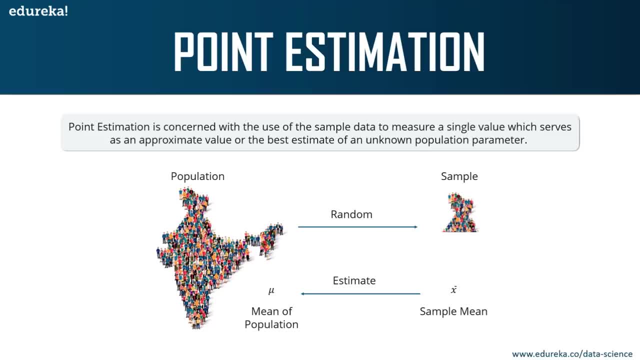 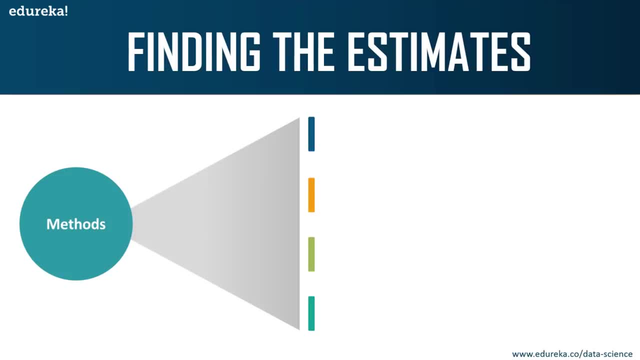 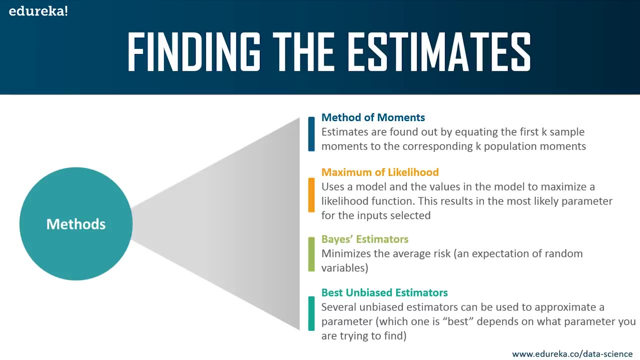 estimator and the realized value of the estimator. is the estimate right? so i hope point estimation is clear. now how do you find the estimates? there are four common ways in which you can do this. the first one is method of moments. here what you do is you form an equation in the sample data set. 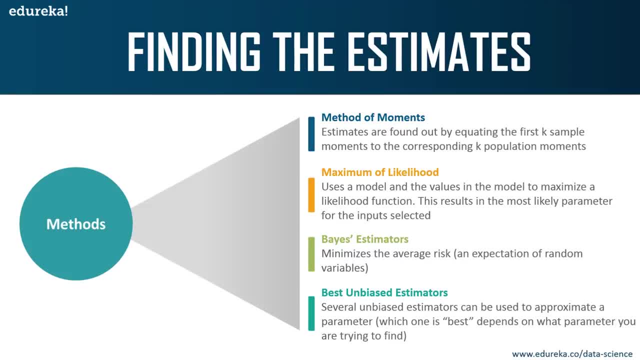 and then you analyze a similar equation in the population data set as well, like the population mean, population variance and so on. so, in simple terms, what you're doing is you're taking down some known facts about the population and you're extending those ideas to the sample. 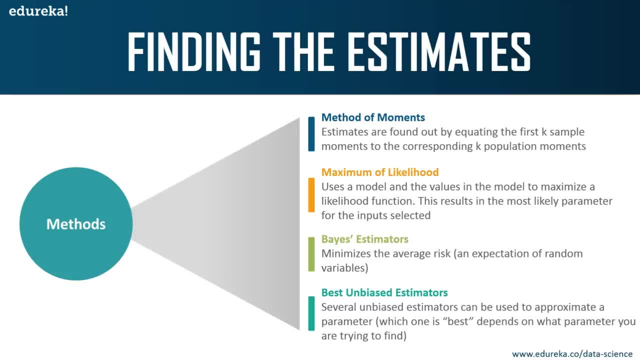 all right. once you do that, you can analyze the sample and estimate more essential or more complex values. right next. we have maximum of likelihood. now, this method basically uses a model to estimate a value. all right now. maximum likelihood is majorly based on probability, so there's a lot of probability. 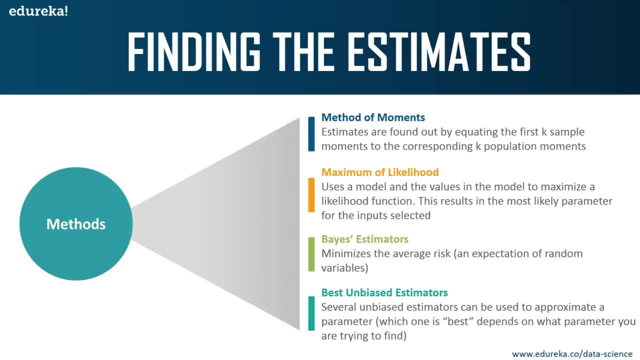 involved in this method. next, we have the base estimator. this works by minimizing the errors or the average risk. okay, the base estimator has a lot to do with the bias theorem. all right, let's not get into the depth of these estimation methods. finally, we have the best unbiased estimators. 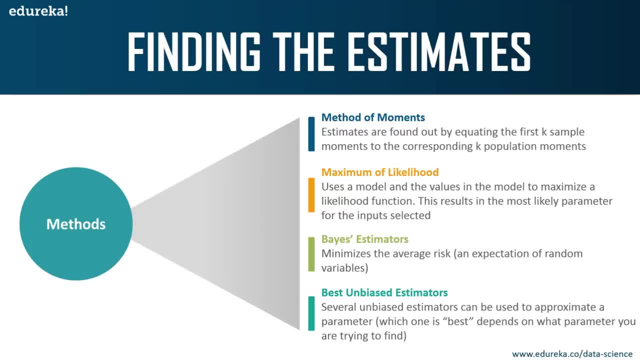 in this method, there are several unbiased estimators that can be used to approximate a pattern. okay, so, guys, these were a couple of methods that are used to find the estimate, but the most well known method to find the estimate is known as the interval estimation. okay, this is one of the most 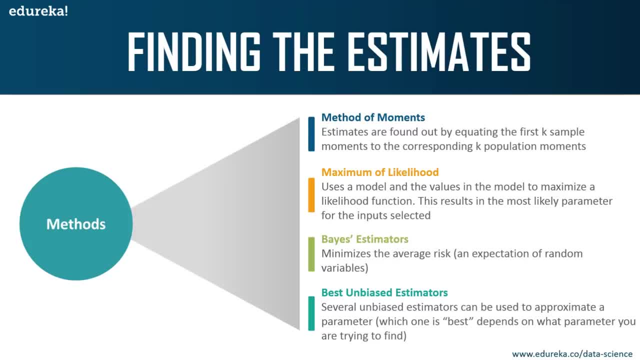 The Bayes estimator has a lot to do with the Bayes theorem. All right, We want to get into the depth of these estimation methods. Finally, we have the best unbiased estimators In this method. there are several unbiased estimators that can be used to approximate a parameter. okay, 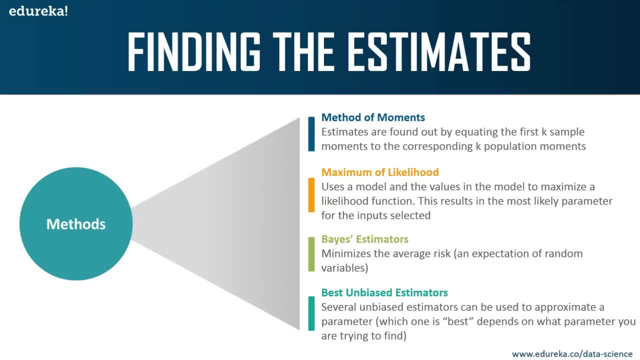 So, guys, these were a couple of methods that are used to find the estimate, but the most well-known method to find the estimate is known as the interval estimation. okay, This is one of the most important estimation methods. All right, this is where confidence interval. 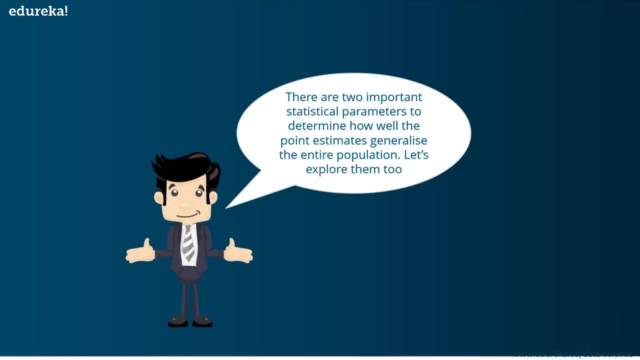 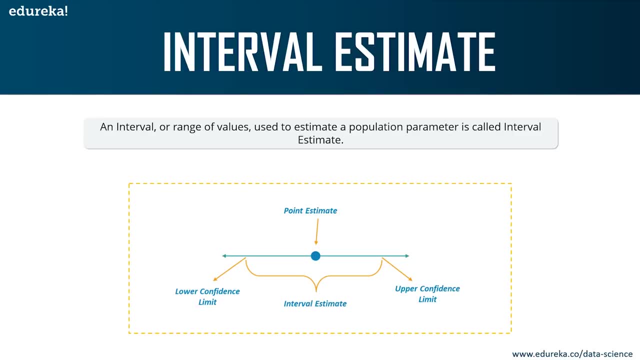 also comes into the picture. Right Apart from interval estimation, we also have something known as margin of error. So I'll be discussing all of this in the upcoming slides. So first let's understand what is interval estimate? okay, An interval or range of values which are used. 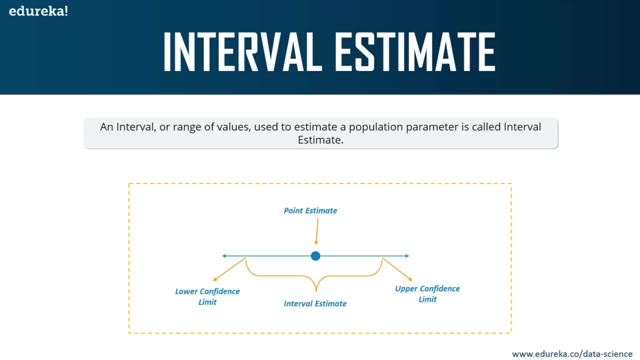 to estimate a population parameter is known as an interval estimation. Right, that's very understandable. Basically, what they're trying to say is: you're going to estimate the value of a parameter. Let's say you're trying to find the mean of a population. 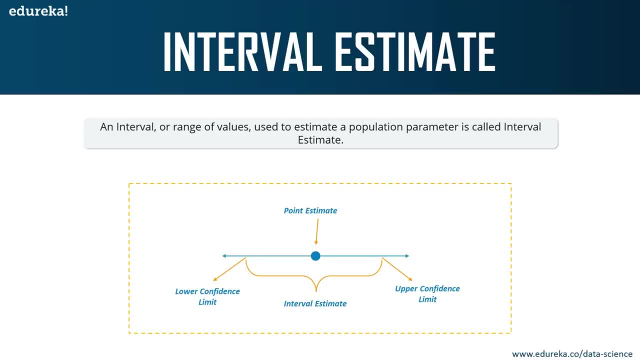 What you're going to do is you're going to build a range and your value will lie in that range or in that interval. All right, so this way your output is gonna be more accurate, because you've not predicted a point estimation. Instead, you have estimated an interval. 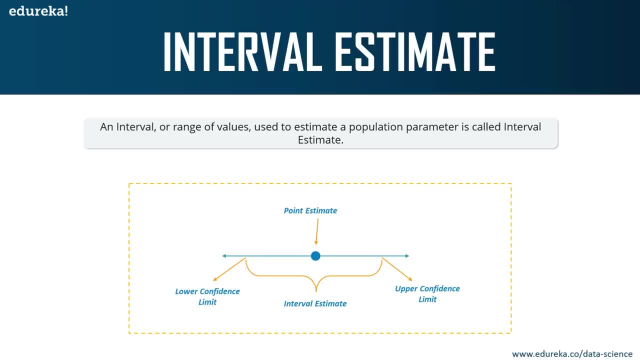 within which your value might occur. right, Okay, now this image clearly shows how point estimate and interval estimate are different. So, as interval estimate is obviously more accurate because you're not just focusing on a particular value or a particular point in order to predict the probability, 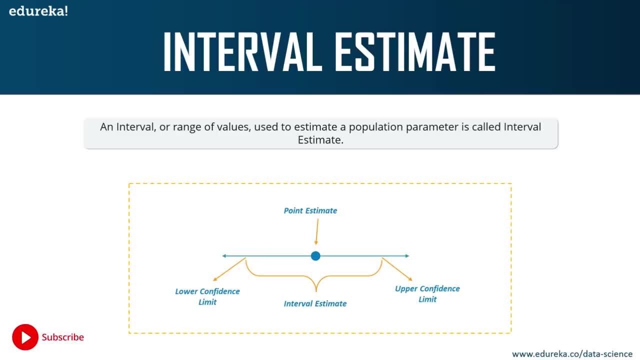 Instead, you're saying that the value might be within this range between the lower confidence limit and the upper confidence limit. all right, This just denotes the range or the interval. Okay, if you're still confused about interval estimation, let me give you a small example. 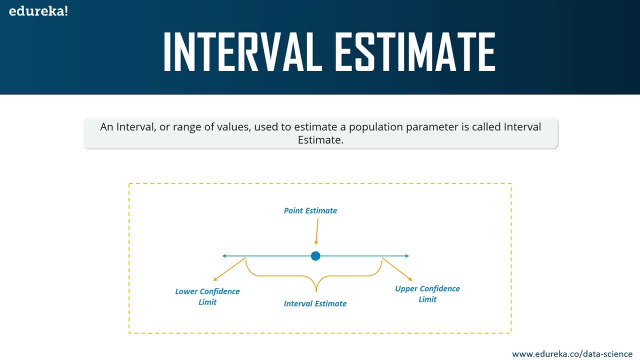 If I stated that I will take 30 minutes to reach the theater- this is known as point estimation- Okay, But if I stated that I will take between 45 minutes to an hour to reach the theater, this is an example of interval estimation. 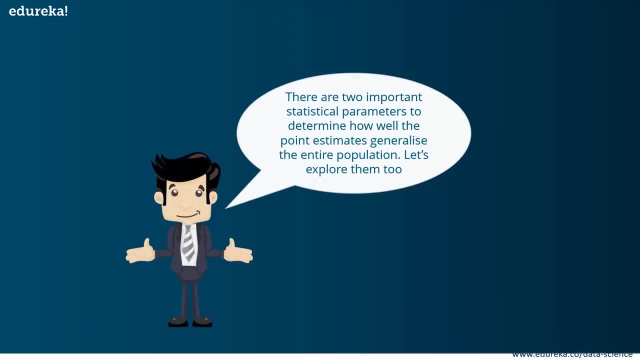 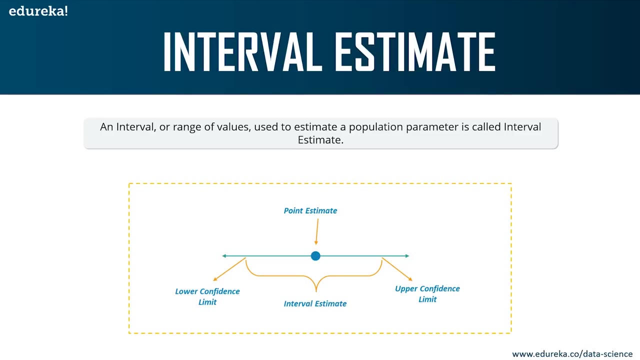 important estimation methods. all right, this is where confidence interval also comes into the picture. right apart from interval estimation, we also have something known as margin of error. so i'll be discussing all of this in the upcoming slides. so first let's understand what is interval estimation? okay, an interval or range of values which are used to estimate a population parameter is known. 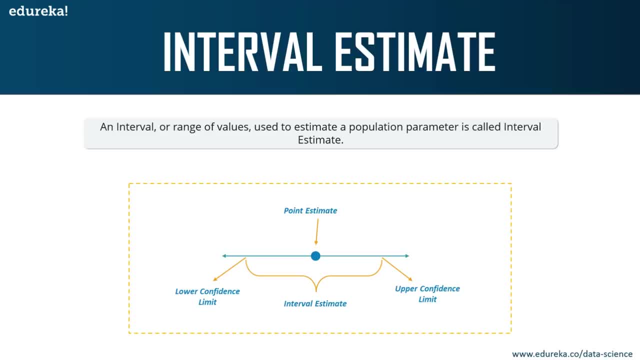 as an interval estimation. right, that's very understandable. basically, what they're trying to say is you're going to estimate the value of a parameter. let's say you're trying to find the mean of a population. what you're going to do is you're going to build a range and your value will. 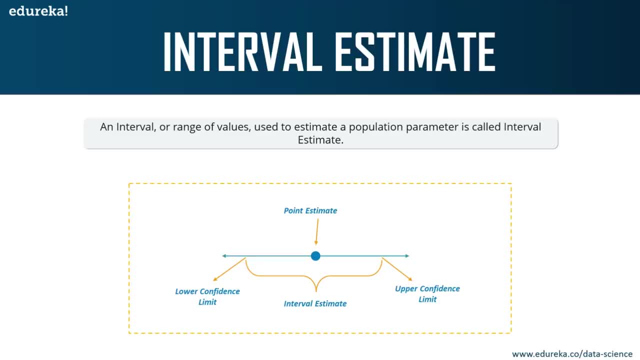 lie in that range or in that interval. all right, so this way your output is going to be more accurate, because you've not predicted a point estimation. instead, you have estimated an interval within which your value might occur. right, okay, now this image clearly shows how point estimate and interval estimate 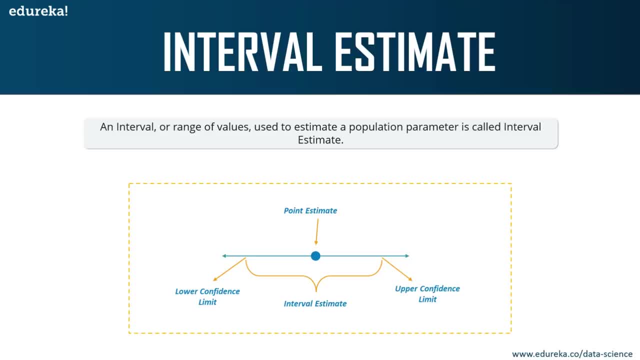 are different. so, guys interval estimate is obviously more accurate, because you're not just focusing on a particular value or a particular point in order to predict the probability. instead, you're saying that the value might be within this range between the lower confidence limit and the upper confidence limit. all right, this just denotes the 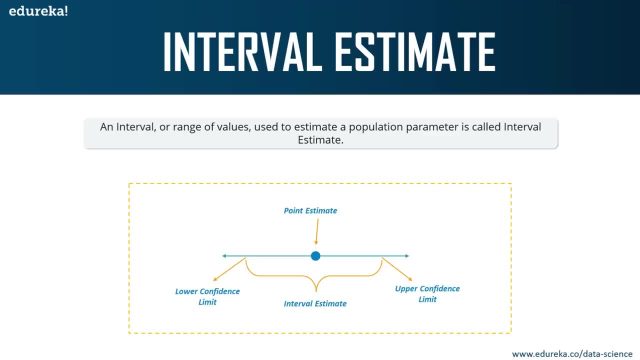 range or the interval, okay. if you're still confused about interval estimation, let me give you a small example. if i stated that i will take 30 minutes to reach the theater, this is known as point estimation- okay. but if i stated that i will take between 45 minutes to an hour to reach the theater, this 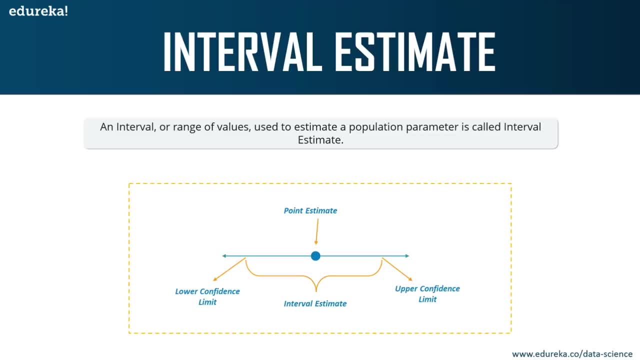 is an example of interval estimation. all right, i hope it's clear now. now, interval estimation, you're seeing, gives rise to two important statistical terminologies. one is known as confidence interval and the other is known as margin of error. all right, so, guys, it's important that you pay attention to. 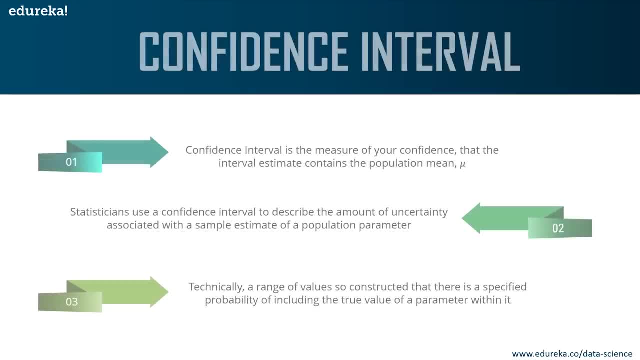 both of these terminologies. confidence interval is one of the most significant measures that are used to check how essential a machine learning model is. all right, so what is confidence interval? confidence interval is the measure of your confidence that the interval estimated contains the population parameter or the population mean or any of those parameters. right now, statisticians, 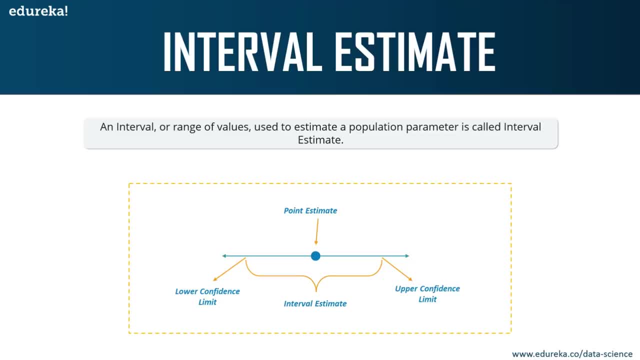 All right, I hope it's clear now. Now, interval estimation gives rise to two important statistical terminologies. One is known as confidence interval and the other is known as margin of error. all right, So, guys, it's important that you pay attention. 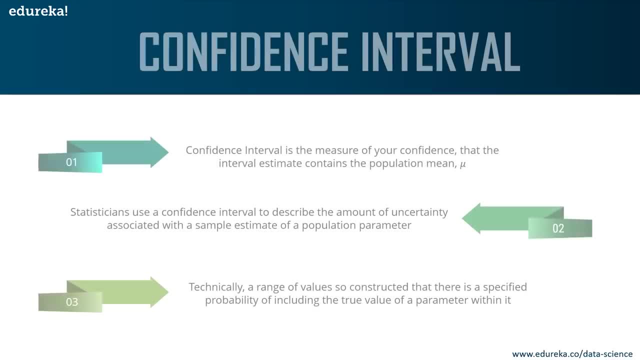 to both of these terminologies. Confidence interval is one of the most significant measures that are used to check how essential a machine learning model is. all right. So what is confidence interval? Confidence interval is the measure of your confidence that the interval estimated contains the population parameter. 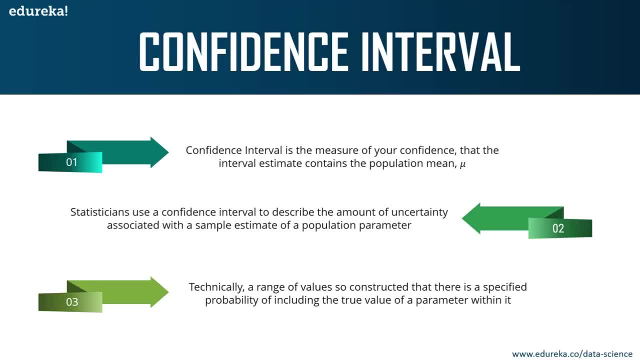 or the population mean or any of those parameters. right Now, statisticians use confidence interval to describe the amount of uncertainty associated with a sample estimate of a population parameter. Now, guys, this is a lot of definition. Let me just make you understand confidence interval. 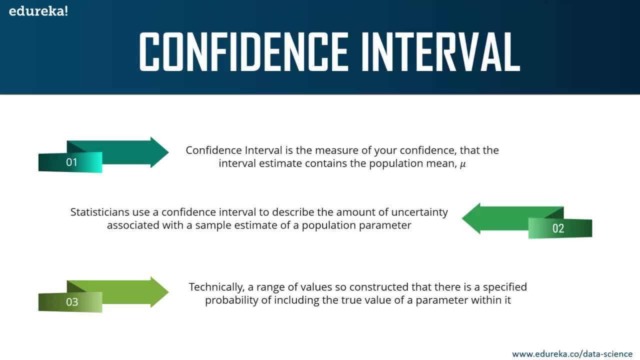 Let me just give you an example of confidence interval with a small example. Okay, let's say that you perform a survey and you survey a group of cat owners to see how many cans of cat food they purchase in one year. Okay, you test your statistics at the 99% confidence level. 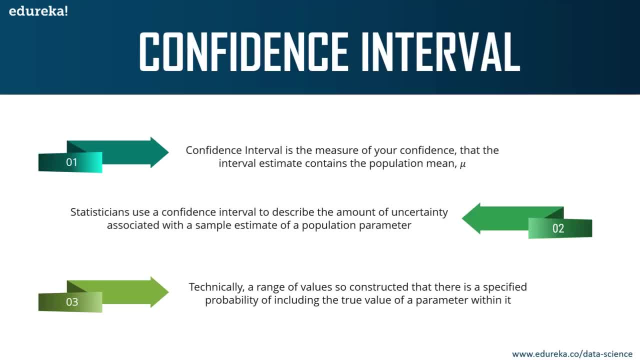 and you get a confidence interval of 100, 200.. This means that you think that the cat owners buy between 100 to 200 cans in a year And also, since the confidence level is 99%, it shows that you're very confident. 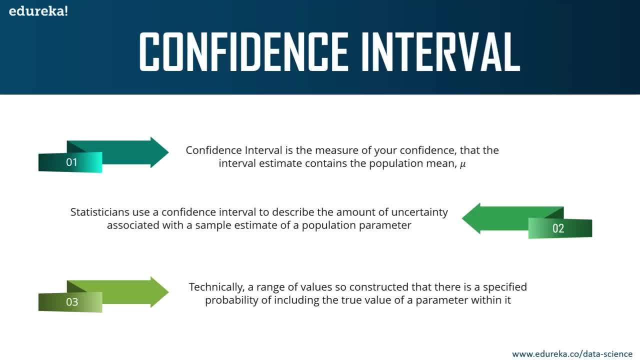 that the results are correct. okay, I hope all of you are clear with that. All right, so your confidence interval here will be 100 and 200 and your confidence level will be 99%. right, That's the difference between confidence interval. 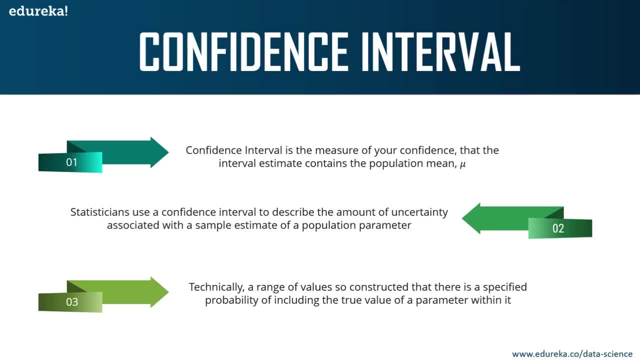 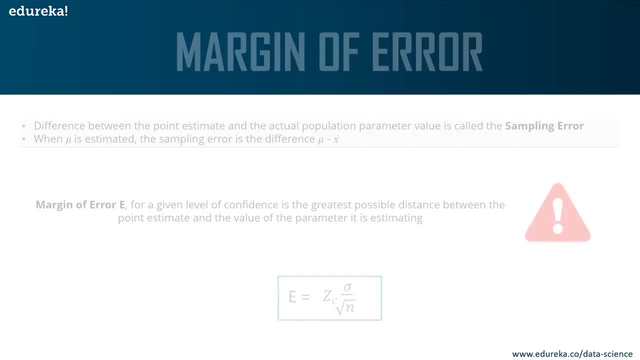 and confidence level. So within your confidence interval your value is going to lie and your confidence level will show how confident you are about your estimation right? I hope that was clear. Let's look at margin of error Now. margin of error for a given level of confidence. 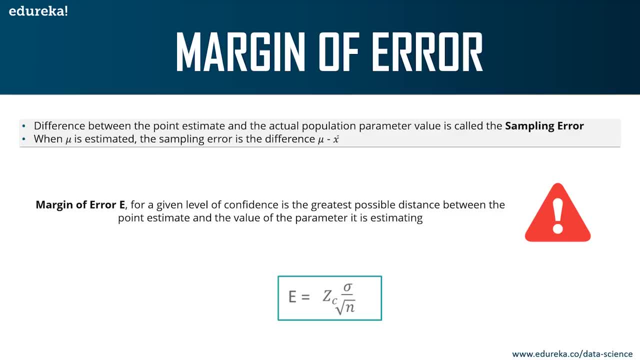 is the greatest possible distance between the point estimate and the value of the parameter that it is estimating. You can say that it is a deviation from the actual point estimate. right Now. the margin of error can be calculated using this formula Now: ZC here denotes the critical value. 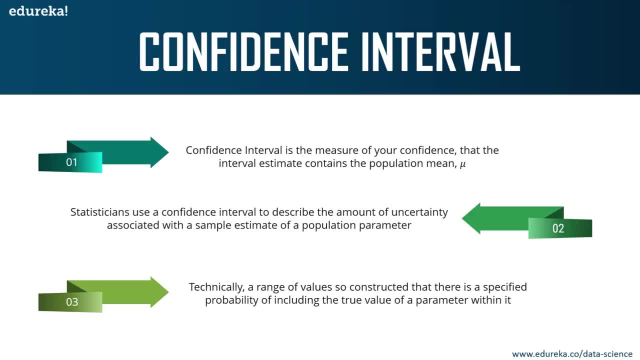 use a confidence interval to describe the amount of uncertainty associated with a sample estimate of a population parameter. now, guys, this is a lot of definition. let me just make you understand confidence interval with a small example. okay, let's say that you perform a survey and you survey. 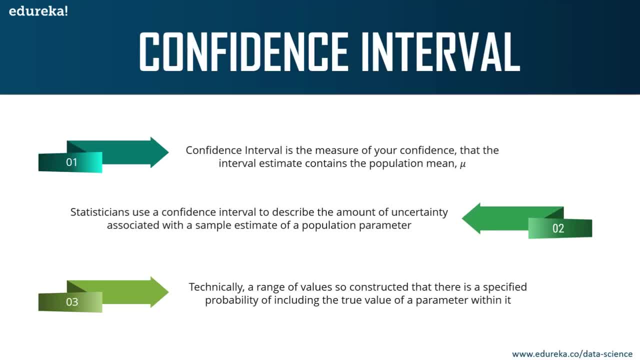 a group of cat owners to see how many cans of cat food they purchase in one year. okay, you test your statistics at the 99 confidence level and you get a confidence interval of 100,200. this means that you think that the cat owners buy between 100 to 200 cans in a year. and also since 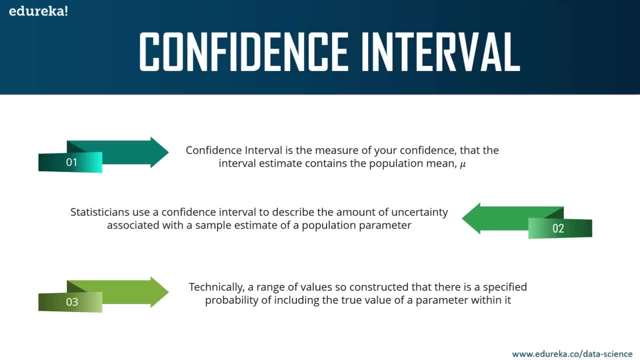 the confidence level is 99, it shows that you're very confident that the results are correct. okay, i hope all of you are clear with that, right? so your confidence interval here will be 100 and 200 confidence level will be 99. right, that's the difference between confidence interval and. 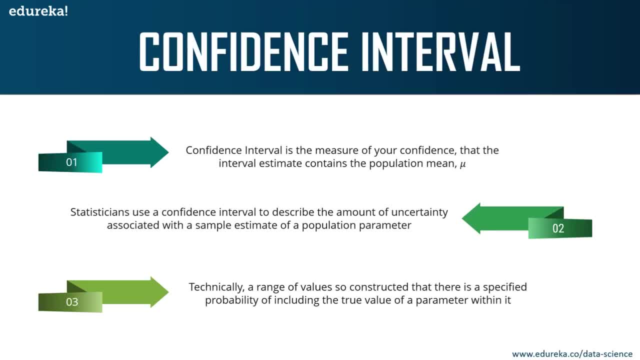 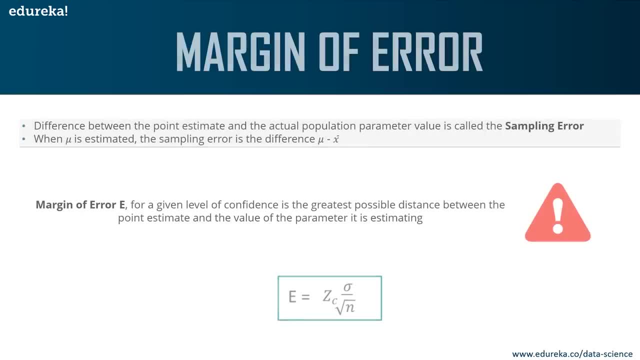 confidence level. so within your confidence interval your value is going to lie and your confidence level will show how confident you are about your estimation right? i hope that was clear. let's look at margin of error now. margin of error for a given level of confidence is the greatest. 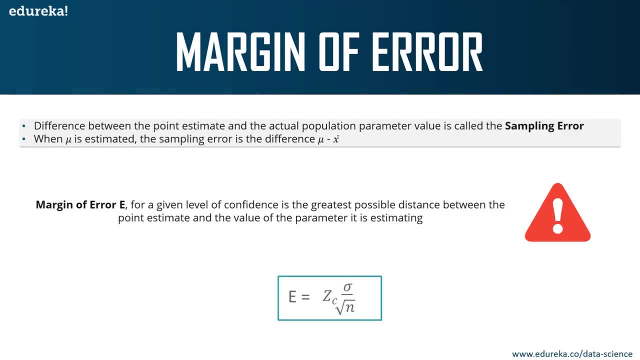 possible distance between the point estimate and the value of the parameter that it is estimating. it is a deviation from the actual point estimate. right now, the margin of error can be calculated using this formula. now, zc here denotes the critical value or the confidence interval, and this is multiplied by standard deviation, divided by root of the sample size. all right, 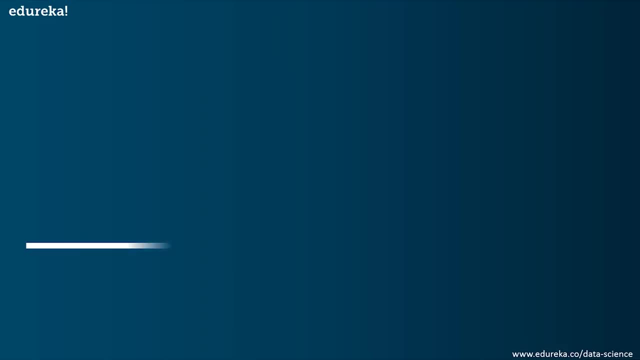 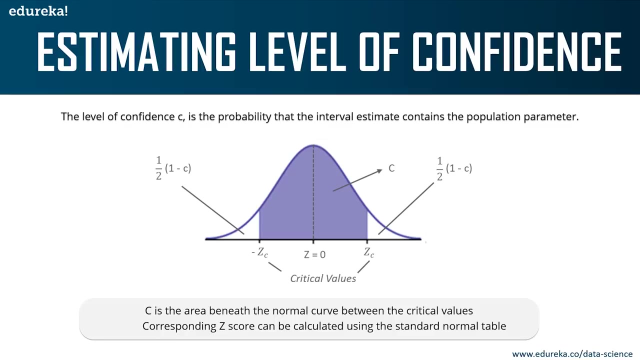 n is basically the sample size. now let's understand how you can estimate the confidence intervals. so, guys, the level of confidence, which is denoted by c, is the probability that the interval estimate contains the population parameter. let's say that you're trying to estimate the mean, all right. so the level of confidence is the probability that the interval estimate 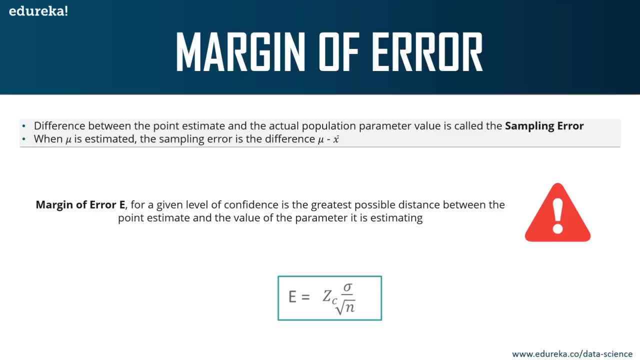 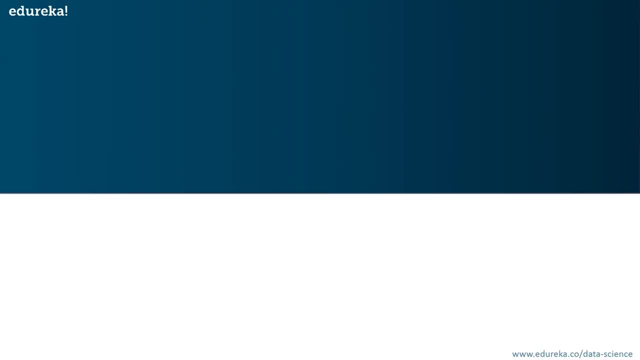 or the confidence interval, and this is multiplied by standard deviation, divided by root of the sample size. All right, N is basically the sample size. Now let's understand how you can estimate the confidence intervals. So, guys, the level of confidence. 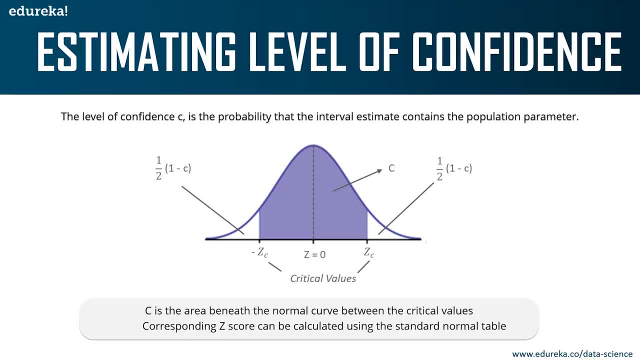 which is denoted by C, is the probability that the interval estimate contains the population parameter. Let's say that you're trying to estimate the mean, all right. So the level of confidence is the probability that the interval estimate contains the population parameter. 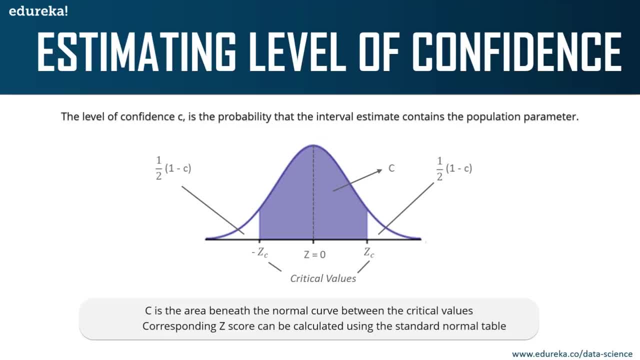 So this interval between minus ZC and ZC, the area beneath this curve, is nothing but the probability that the interval estimate contains the population parameter. all right, It should basically contain the value that you are predicting right Now. these are known as critical values. 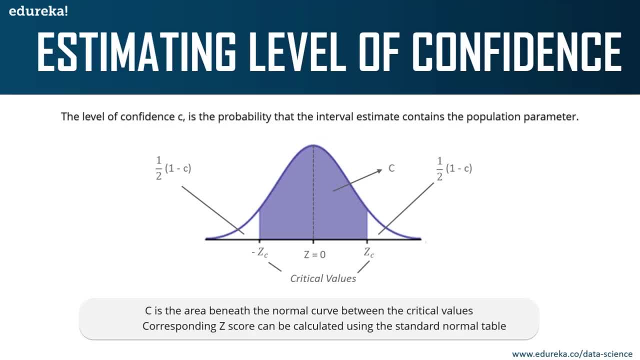 This is basically your lower limit and your higher limit confidence level. Also, there's something known as the Z-score. Now, this score can be calculated by using the standard normal table. all right, If you look it up anywhere on Google, you'll find the Z-score table. 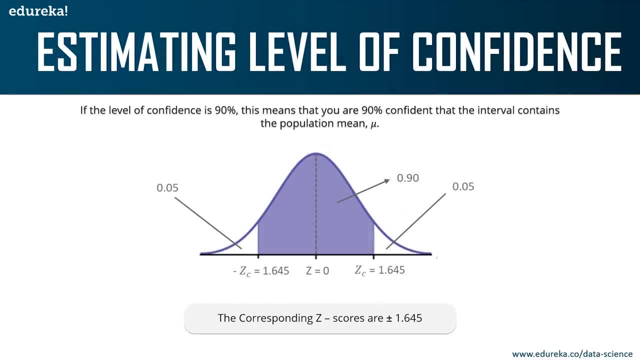 or the standard normal table. All right, To understand how this is done, let's look at a small example. Okay, let's say that the level of confidence is 90%. This means that you are 90% confident that the interval contains the population mean okay. 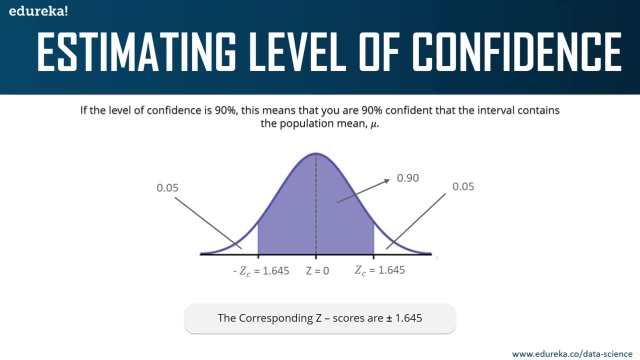 So the remaining 10%, which is out of 100%, the remaining 10% is equally distributed on these tail regions. okay, So you have 0.05 here and 0.05 over here, right? So on either side of C. 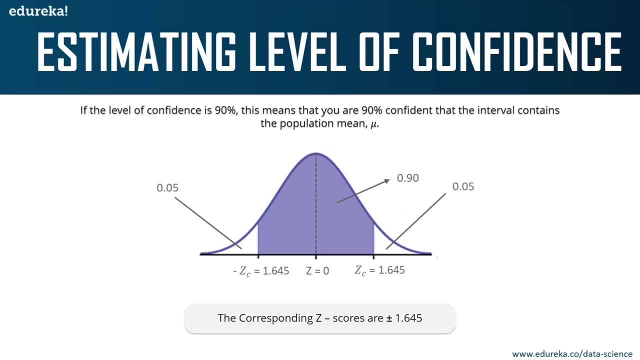 you'll distribute the other left over percentage. Now, these Z-scores are calculated from the table, as I mentioned before. all right, 1.645 is calculated from the standard normal table. okay, So guys, this is how you estimate the level of confidence. 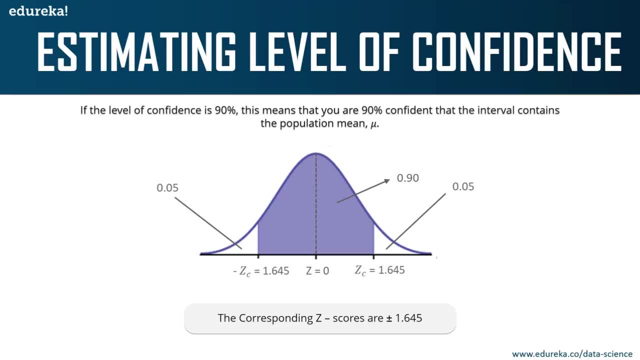 So, to sum it up, let me tell you the steps that are involved in constructing a confidence interval. First, you'll start by identifying a sample statistic. okay, This is the statistic that you will use to estimate a population parameter. This can be anything like the mean of the sample. 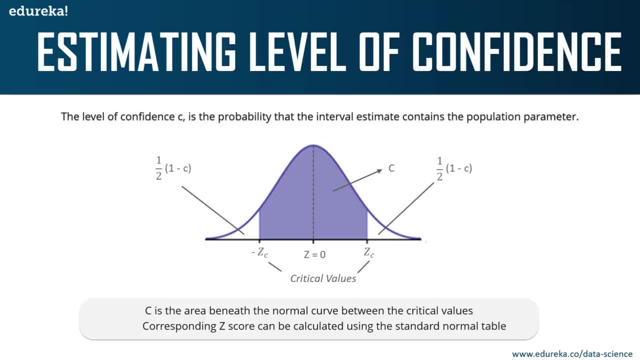 contains the population parameter. so this interval between minus zc and zc, or the area beneath this curve, is nothing but the probability that the interval estimate contains the population parameter. all right, it should basically contain the value that you are predicting. now these are known as critical values. this is basically your lower limit and your higher limit. 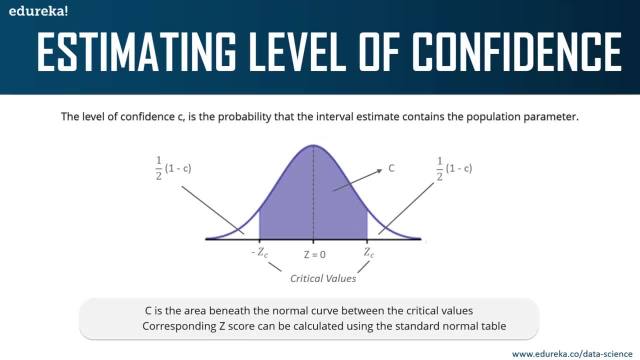 confidence level. also, there's something known as the z score. now, this code can be calculated by using the standard normal table. all right, if you look it up anywhere on google, you'll find the z score table or the standard normal table. okay to understand, uh, how this is done, let's look at a 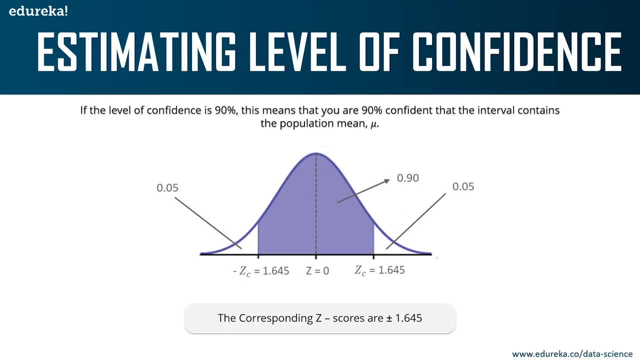 small example. okay, let's say that the level of confidence is 90 percent. this means that you are 90 percent confident, that the interval estimate is 90 percent and the level of confidence is 90 percent interval contains the population mean: okay, so, uh, the remaining 10 percent, which is out of 100. 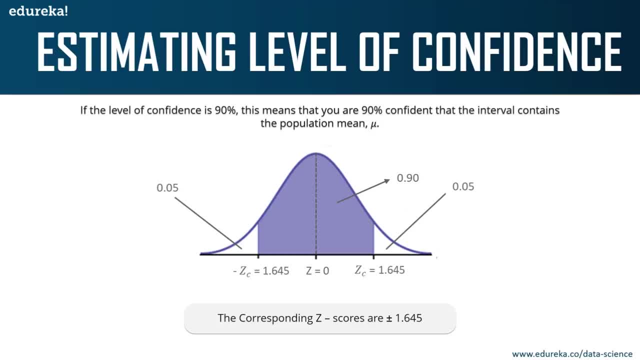 the remaining 10 percent is equally distributed on these tail regions. okay, so you have 0.05 here and 0.05 over here, right? so on either side of c you'll distribute the other left over percentage. now, these these codes are calculated from the table as i mentioned before. all right, 1.645. 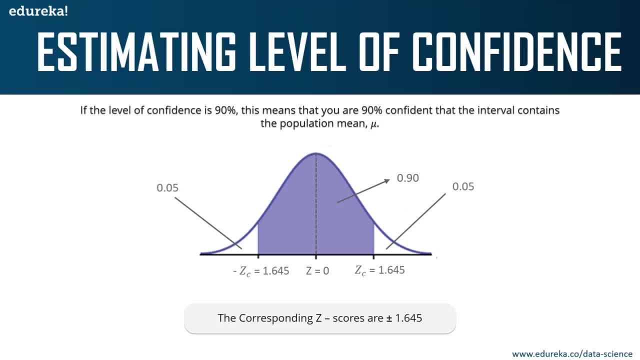 is calculated from the standard normal table. okay, so, guys, this is how you estimate the level of confidence. so, to sum it up, let me tell you the steps that are involved in constructing a confidence interval. first, you'll start by identifying a sample statistic. okay, this is the statistic that you will use to estimate a population parameter. this can be: 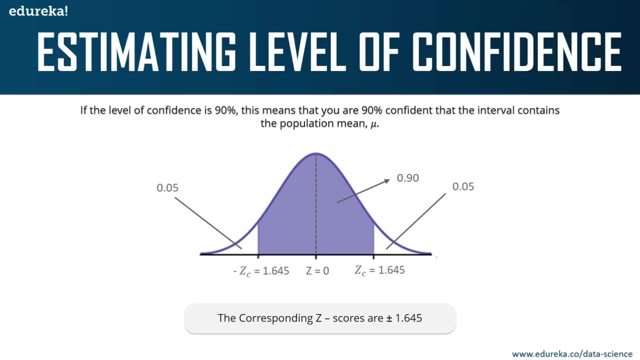 anything like the mean of the sample. next, you will select a confidence level. now, the confidence level describes the uncertainty of a sampling method. right after that, you'll find something known as the margin of error. right, we discussed margin of error earlier, so you find this based on the equation that i explained. 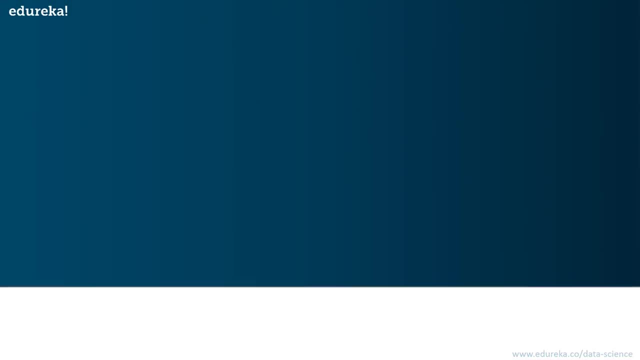 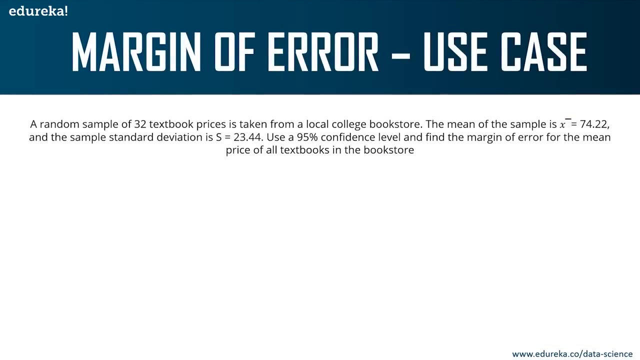 in the previous slide. then you'll finally specify the confidence interval. all right, now let's look at a problem statement to better understand this concept. a random sample of 32 textbook prices is taken from a local college bookstore. the mean of the sample is so, so and so, and the sample? 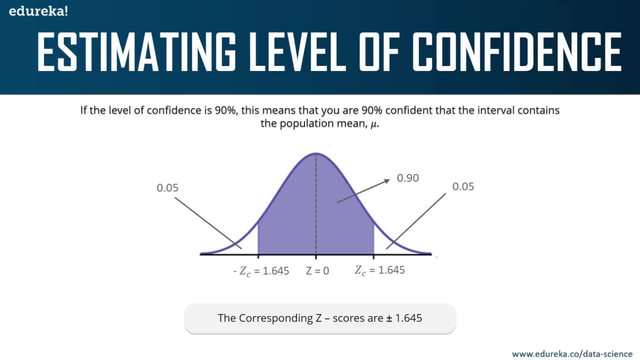 Next, you will select a confidence level. Now, the confidence level describes the uncertainty of a sampling method. right After that, you'll find something known as the margin of error. right, We discussed margin of error earlier, So you find this based on the equation. 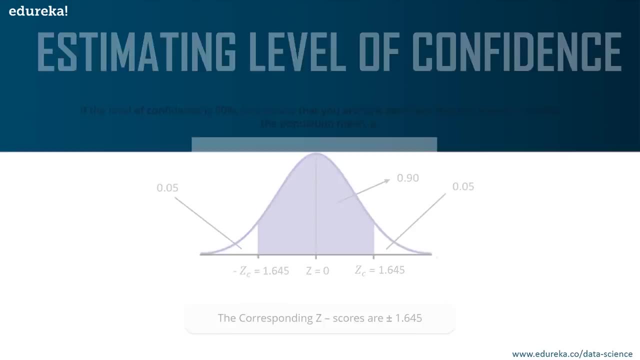 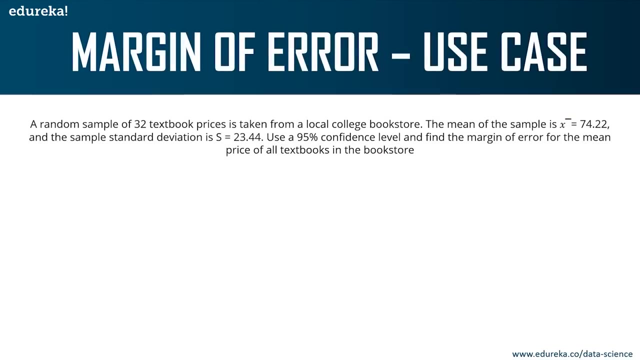 that I explained in the previous slide. Then you'll finally specify the confidence interval. all right, Now let's look at a problem statement. to better understand this concept, A random sample of 32 textbook prizes is taken, say, from a local college bookstore. 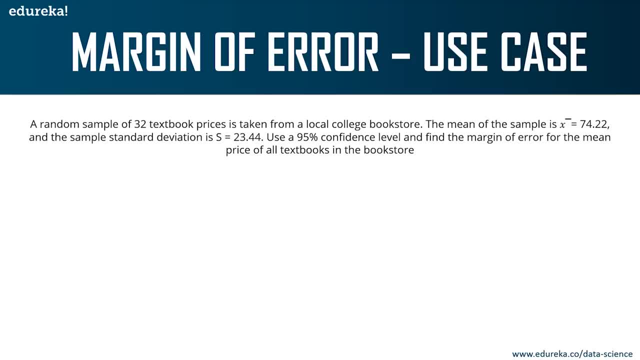 The mean of the sample is so, so and so, and the sample standard deviation is this: Use a 95% confidence level and find the margin of error for the mean prize of all textbooks in the bookstore. okay, Now, this is a very straightforward question. 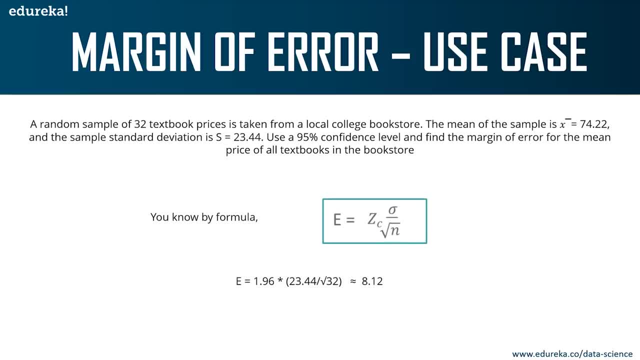 If you want, you can read the question again. All you have to do is you have to just substitute the values into the equation, all right, So, guys, we know the formula for margin of error. You take the z-score from the table. 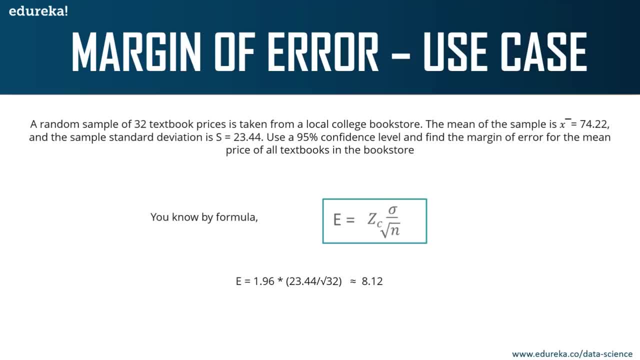 After that we have deviation which is 23.44,. right, That's standard deviation. and n stands for the number of samples. Now the number of samples is 32, basically 32 textbooks. So approximately your margin of error. 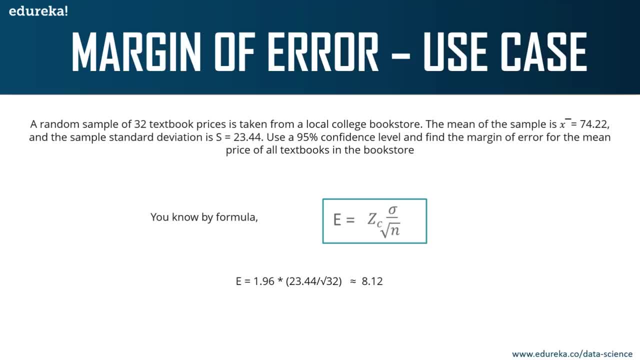 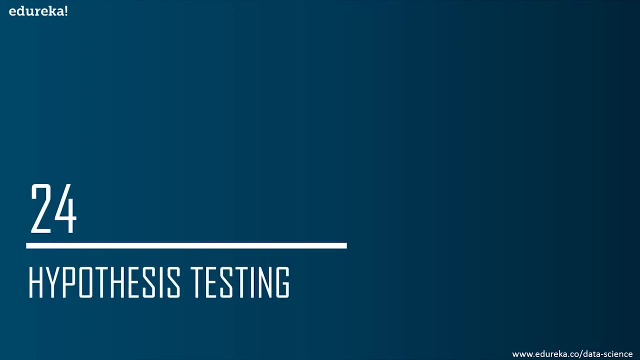 is going to be around 8.12.. This is a pretty simple question, all right, I hope all of you understood this. Now that you know the idea behind confidence interval, let's move ahead to one of the most important topics in statistical inference, which is hypothesis testing right. 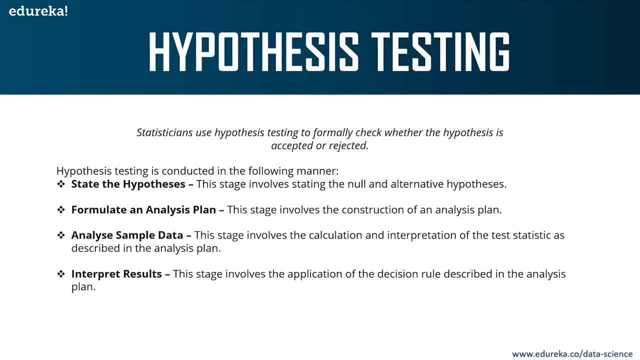 So, basically, statisticians use hypothesis testing to formally check whether the hypothesis is accepted or rejected. okay, Hypothesis testing is an inferential statistical technique used to determine whether there is enough evidence in a data sample to infer that a certain condition holds true for an entire population. 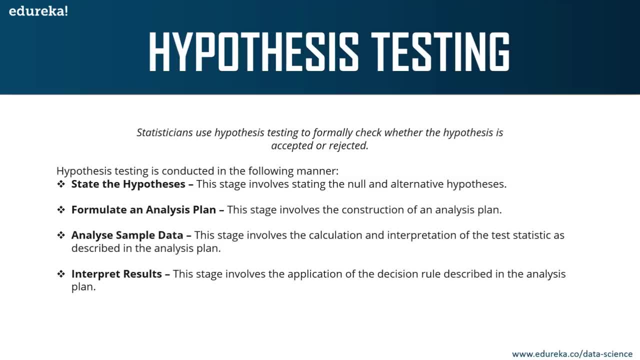 So, to understand the characteristics of a general population, we take a random sample and we analyze the properties of the sample right, We test whether or not the identified conclusion represents the population accurately and finally we interpret their results. Now, whether or not to accept the hypothesis. 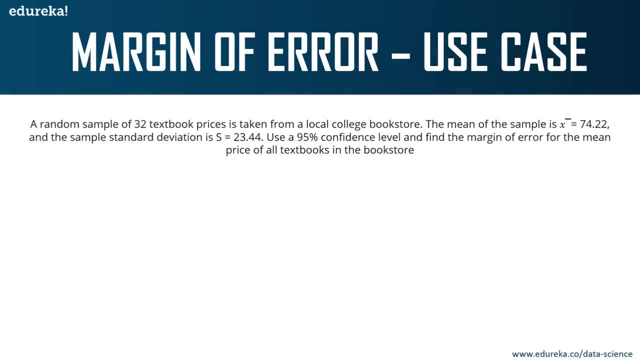 standard deviation is this: use a 95 percent confident level and find the margin of error for the mean price of all textbooks in the bookstore. okay now, this is a very straightforward question. if you want, you can read the question again. all you have to do is you have to just. 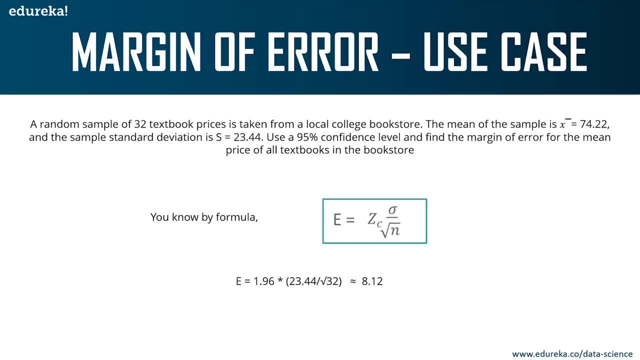 substitute the values into the equation, all right, so, guys, we know the formula for margin of error. you take the z score from the table. after that we have deviation, which is 23.44. right, and that's standard deviation. and n stands for the number of samples. here are the number of: 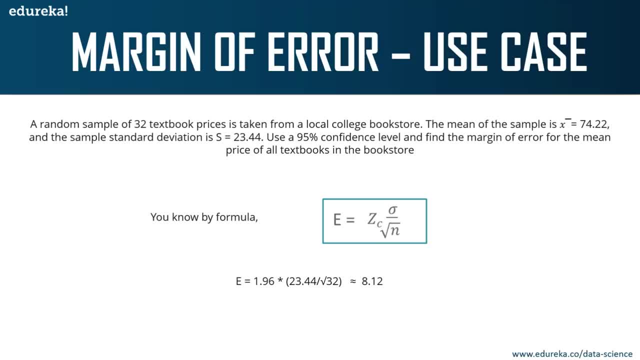 samples is 32, basically 32 textbooks. so approximately your margin of error is going to be around 8.12. this is a pretty simple uh question. all right, i hope all of you understood this. now that you know the idea behind confidence interval, let's move ahead to one of the most important. 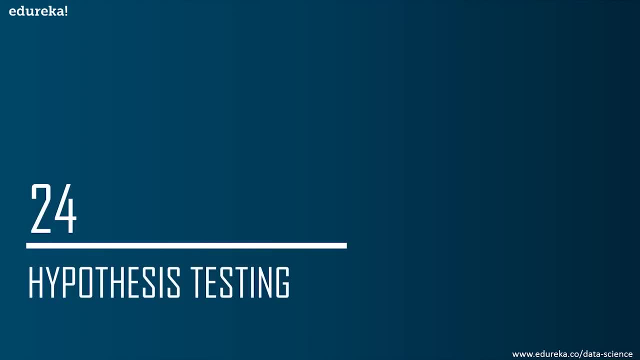 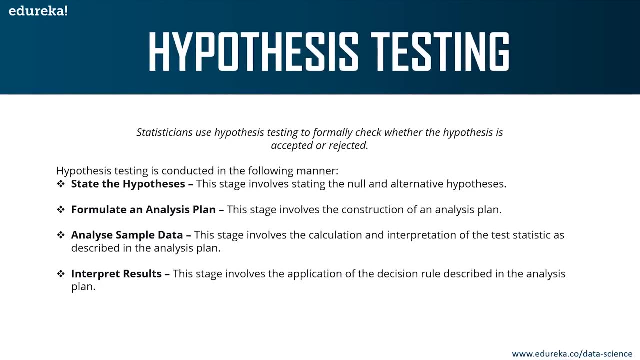 topics in statistical inference, which is hypothesis testing, right? so basically, statisticians use hypothesis testing to formally check whether the hypothesis is correct or not, and then you can use this to determine whether the hypothesis is accepted or rejected. okay, hypothesis testing is an inferential statistical technique used to determine whether there is enough evidence in 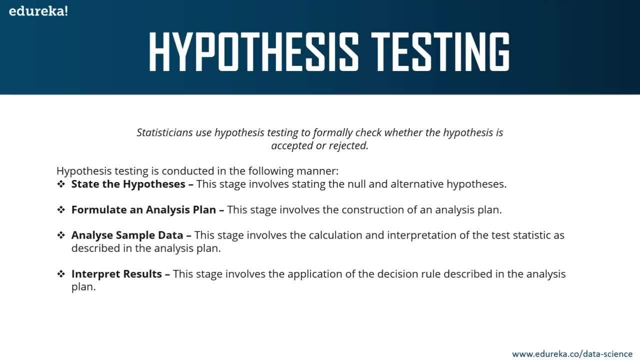 a data sample to infer that a certain condition holds true for an entire population. so to understand the characteristics of a general population, we take a random sample and we analyze the properties of the sample right, we test whether or not the identified conclusion is correct or not and finally we interpret their results. now, whether or not to accept the hypothesis. 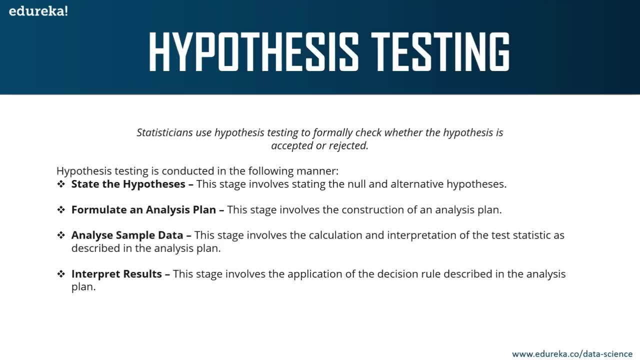 depends upon the percentage value that we get from the hypothesis. okay, so to better understand this, let's look at a small example. before that, there are few steps that are followed in hypothesis testing. you begin by stating the null and the alternative hypothesis. all right, i'll tell you what. 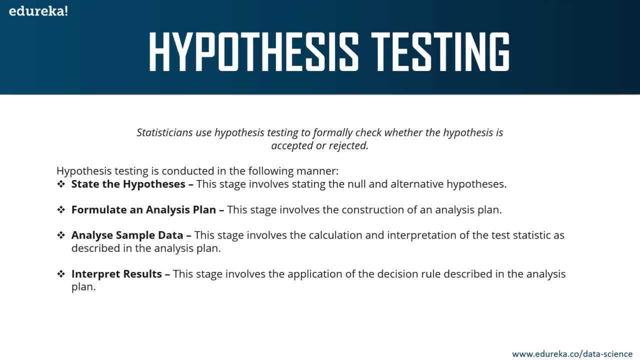 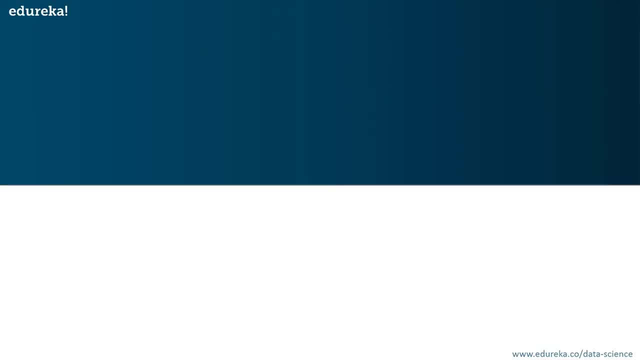 exactly these terms are, and then you formulate an analysis plan, all right. after that you analyze the sample data, and then you formulate an analysis plan, all right. after that you analyze the sample data and finally, you can interpret the results right now to understand the entire hypothesis testing. 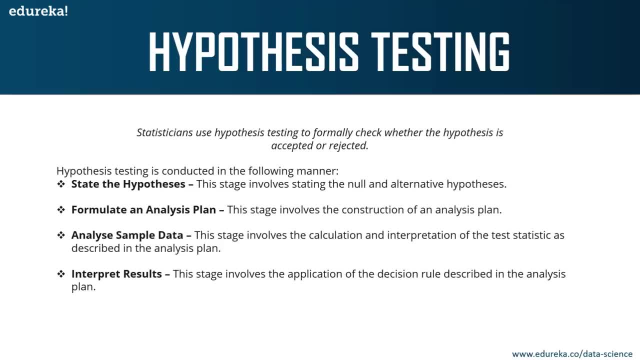 depends upon the percentage value that we get from the hypothesis. Okay, so to better understand this, let's look at a small example. Before that, there are a few steps that are followed in hypothesis testing. You begin by stating the null and the alternative hypothesis. all right, 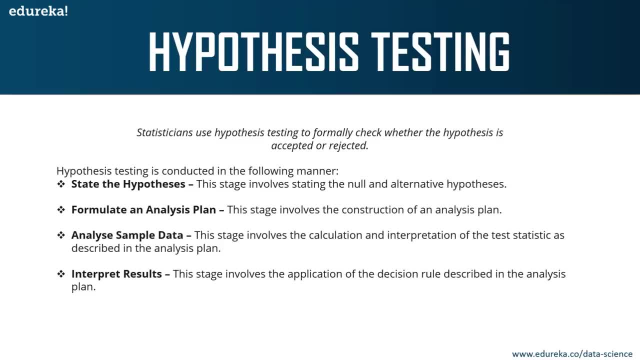 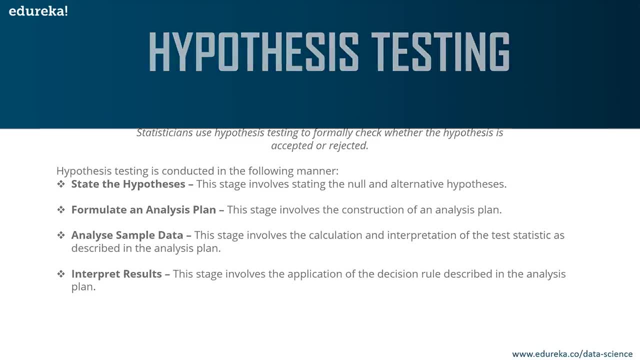 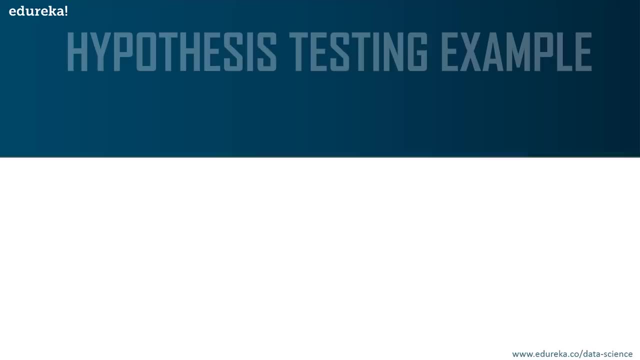 I'll tell you what exactly these terms are, and then you formulate an analysis plan, all right. After that, you analyze the sample data and finally, you can interpret the results right Now to understand the entire hypothesis testing. we look at a good example, okay. 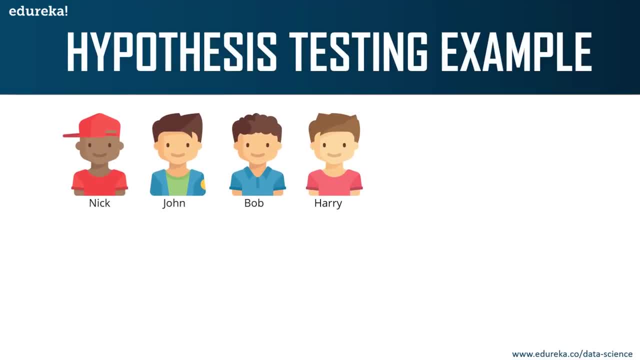 Now consider four boys: Nick, John, Bob and Harry. These boys were caught bunking a class and they were asked to stay back at school and clean their classroom as a punishment, right. So what John did is he decided that four of them. 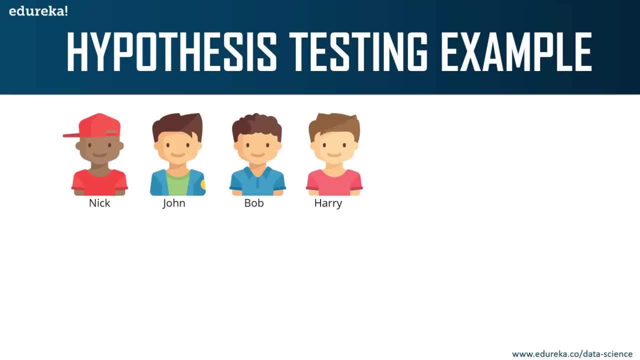 would take turns to clean their classrooms. He came up with a plan of writing each of their names on chits and putting them in a bowl. Now, every day they had to pick up a name from the bowl and that person had to clean the class. right? 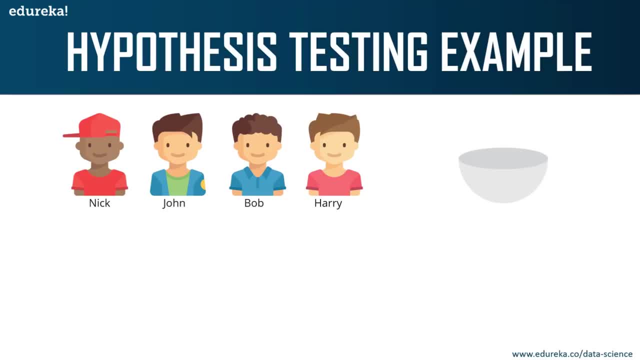 That sounds pretty fair enough. Now it has been three days and everybody's name has come up except John's. Assuming that this event is completely random and free of bias, what is the probability of John not cheating, right? What is the probability that he's not actually cheating? 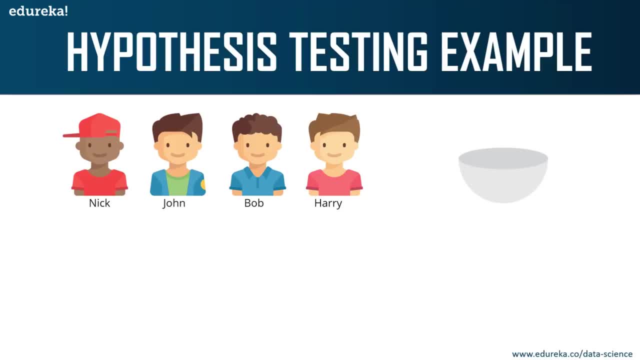 This can be solved by using hypothesis testing. okay, So we'll begin by calculating the probability of John not being picked for a day, right? So we're going to assume that the event is free of bias, So we need to find out the probability. 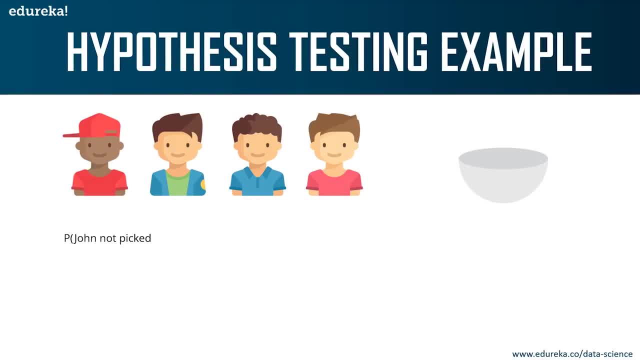 of John not cheating right First, we'll find the probability that John is not picked for a day right. We get three out of four, which is basically 75 percent. Now, 75 percent is fairly high. So if John is not picked for three days in a row, 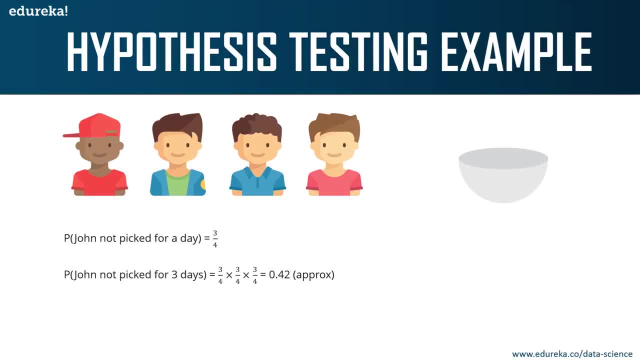 the probability will drop down to approximately 42 percent. Okay, so three days in a row, meaning that is, the probability drops down to 42 percent. Now let's consider a situation where John is not picked for 12 days in a row. 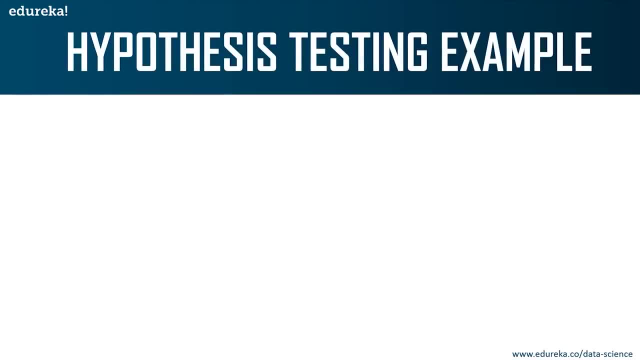 we'll look at a good example. okay, now consider four boys: nick, john, bob and harry. these boys were caught bunking a class and they were asked to stay back at school and clean their classroom as a punishment. right? so what john did is he decided that four of them would take turns to clean their classrooms. 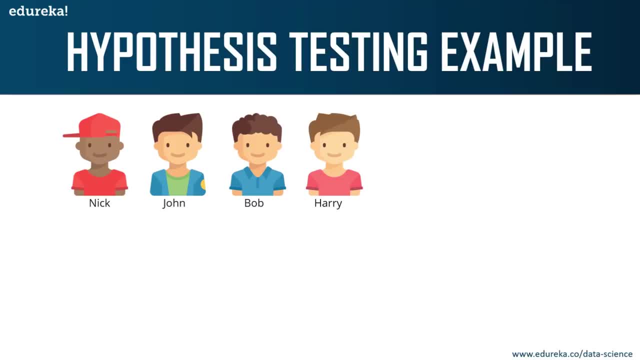 he came up with a plan of writing each of their names on chits and putting them in a bowl. now, every day they had to pick up a name from the bowl and that person had to clean the class. right, that sounds pretty fair enough. now it has been three days and 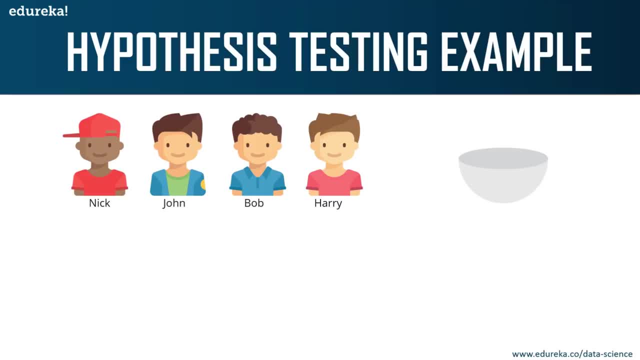 everybody's name has come up except john's. assuming that this event is completely random and free of bias, what is the probability of john not cheating, right? what is the probability that he's not actually cheating? this can be solved by using hypothesis testing. okay, so we'll begin by. 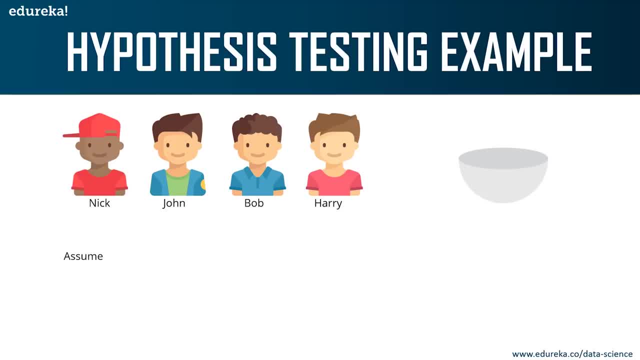 calculating the probability of john not being picked for a day right. so we're going to assume that the event is free of bias. so we need to find out the probability of john not cheating right first. we'll find the probability that john is not picked for a day right. we get three out of. 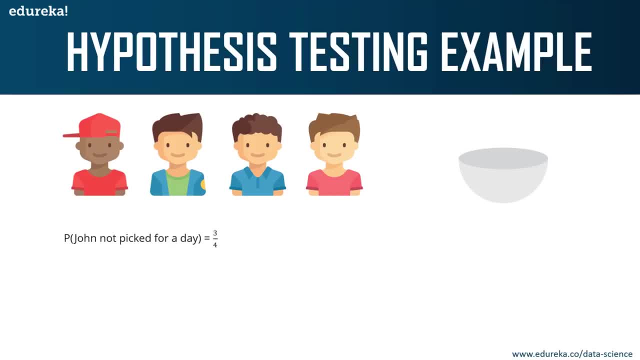 four, which is basically 75 percent. now, 75 percent is fairly high, so if john is not picked for three days in a row, the probability will drop down to approximately 42 percent. okay, so three days in a row, meaning that is, the probability drops down to 42 percent. 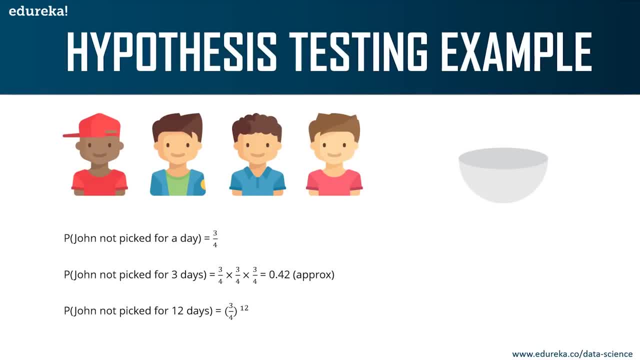 now let's consider a situation where john is not picked for 12 days in a row. the probability drops down to 3.2 percent. okay, that's, the probability of john cheating becomes fairly high, right? so in order for statisticians to come to a conclusion, they define what is known as the threshold value. 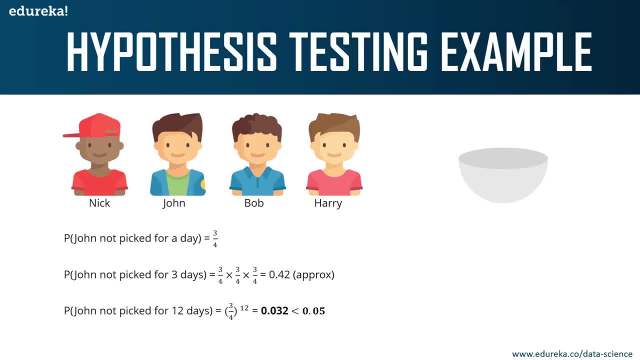 right, considering the above situation, if the threshold value is set to 5, it would indicate that if the probability lies below 5, then john is cheating his way out of detention. but if the probability is about threshold value, then john is just lucky and his name isn't getting picked. so the probability and hypothesis testing give rise to two important 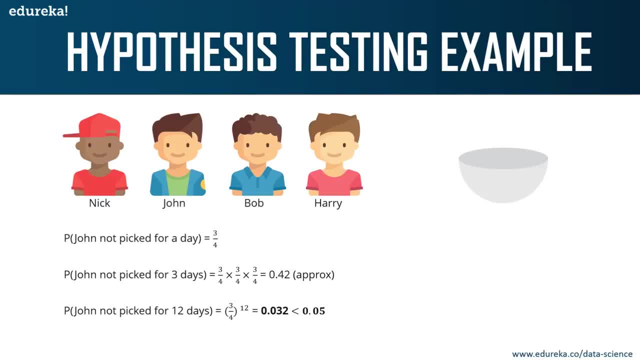 The probability drops down to 3.2 percent. okay, That's, the probability of John cheating becomes fairly high, Right? So in order for statisticians to come to a conclusion, they define what is known as the threshold value, right? Considering the above situation, 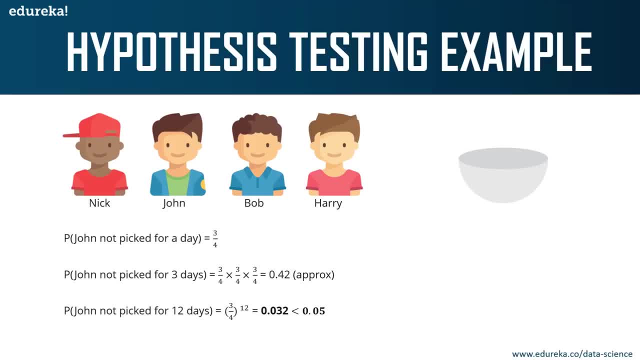 if the threshold value is set to 5 percent, it would indicate that if the probability lies below 5 percent then John is cheating his way out of detention, But if the probability is above threshold value, then John is just lucky and his name isn't getting picked. 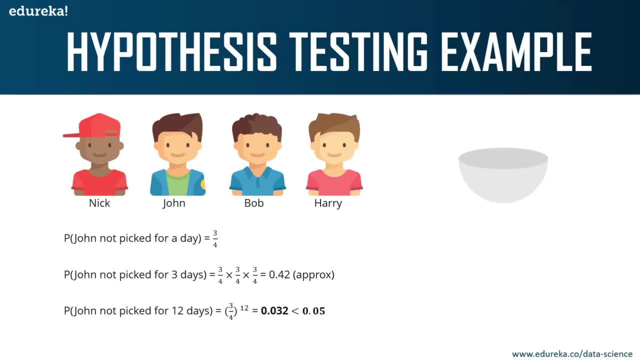 So the probability and hypothesis testing give rise to two important components of hypothesis testing, which is null hypothesis and alternate hypothesis. Null hypothesis is basically approving the assumption. Alternate hypothesis is when your result disapproves the assumption. Right. therefore, in our example, 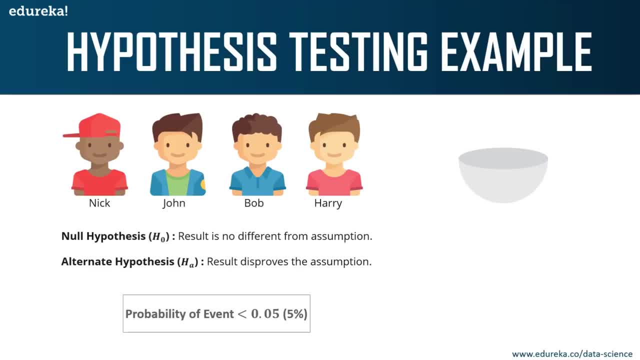 if the probability of an event occurring is less than 5 percent- which it is- then the event is biased, Hence it proves the alternate hypothesis. So, guys, with this we come to the end of this session. So before I wrap up, 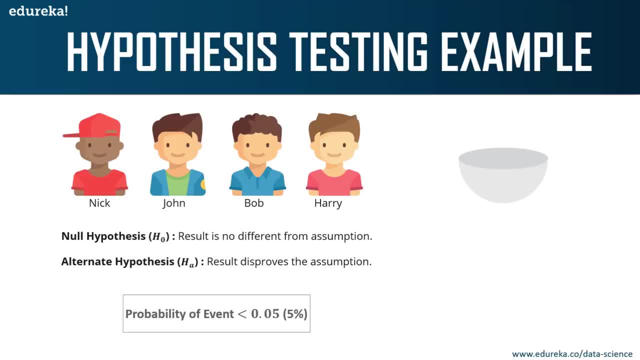 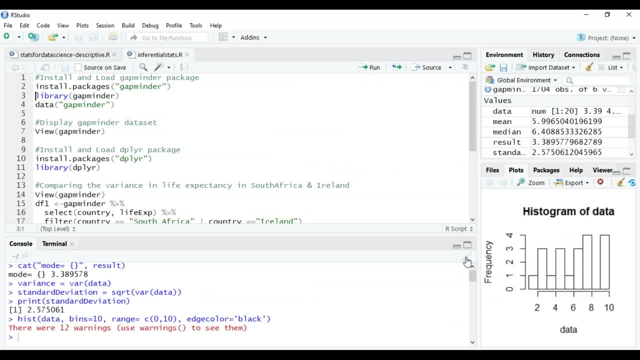 we're going to run a quick demo, which is based on inferential statistics. Let's quickly open up RStudio Again. I'll be running this in R language and those of you who don't know R, it's okay. I'm gonna leave a couple of links in the description. 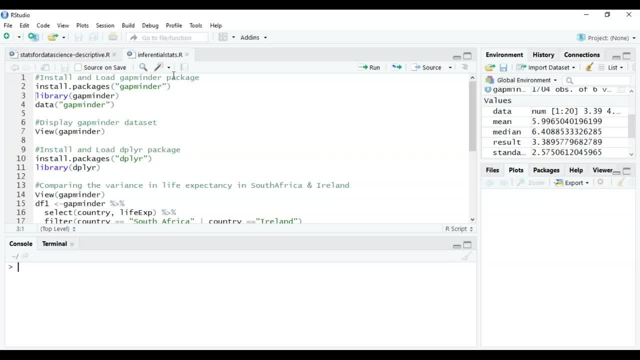 and this is pretty understandable. This is just basic math. right Now, in this demo, what we'll be doing is we'll be using the Gapminder dataset to perform hypothesis testing. Now, guys, the Gapminder dataset contains a list of 142 countries. 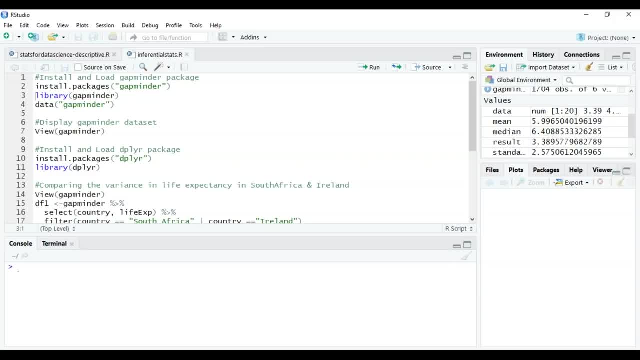 with their respective values for life expectancy, a GDP per capita and population, every five years from 1952 to 2007.. Okay, don't worry, I'll show you the dataset. So what we'll do is we'll begin by installing. 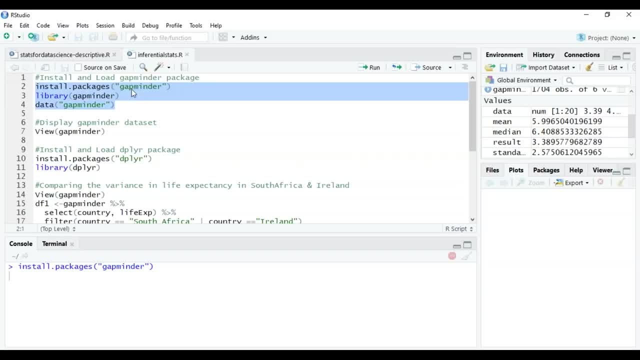 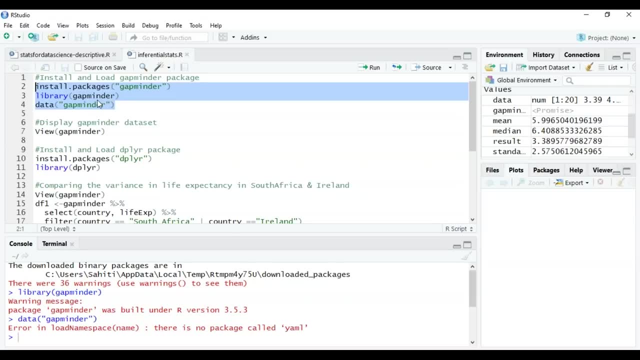 and downloading the Gapminder dataset. So this installpackages will basically install the Gapminder package and this library. Gapminder will just load the Gapminder library. all right, So we've successfully loaded our Gapminder package. 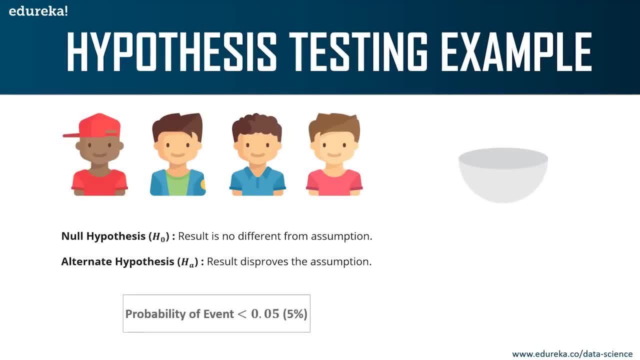 components of hypothesis testing, which is null hypothesis and alternate hypothesis. null hypothesis is basically approving the assumption. alternate hypothesis is when your result disapproves the assumption right. therefore, in our example, if the probability of an event occurring is less than five percent, which it is, then the event is biased, hence it proves the. 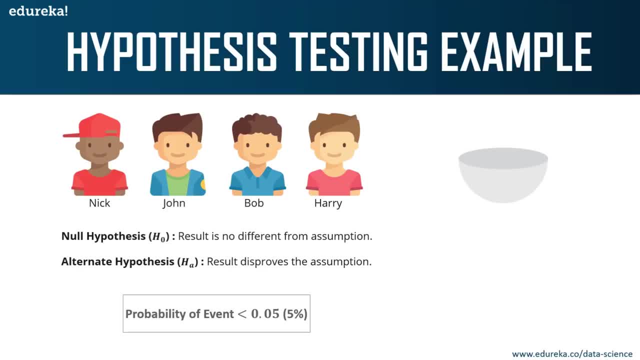 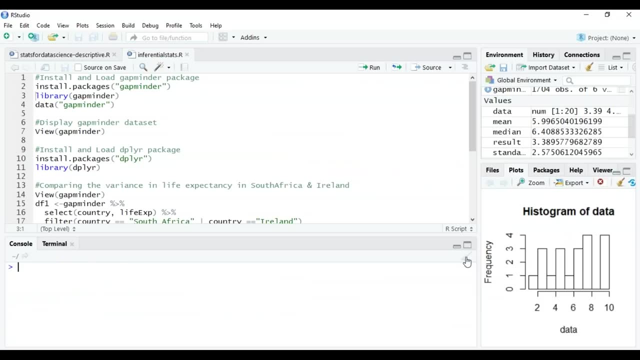 alternate hypothesis. so, guys, with this we come to the end of this session. so before i wrap up, we're going to run a quick demo, which is based on inferential statistics. let's quickly open up our studio again. i'll be running this in our language and. 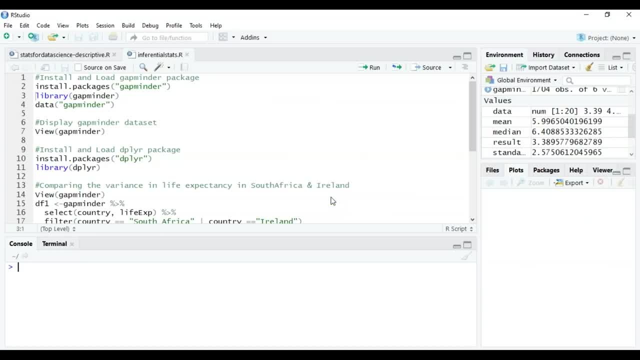 those of you who don't know are. it's okay, i'm going to leave a couple of links in the description, and this is pretty understandable. this is just basic math. right now, in this demo, what we'll be doing is we'll be using the gap minder data set to perform hypothesis testing. now, guys, the gap minder. 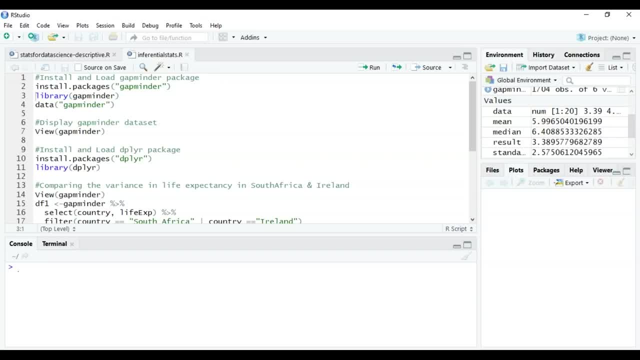 data set contains a list of 142 countries with their respective values for life expectancy, a gdp per capita and population every five years from 1952 to 2007. okay, don't worry, i'll show you the data set. so what we'll do is we'll begin by installing and downloading. 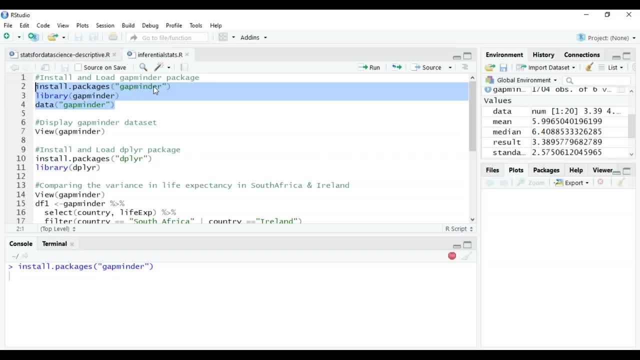 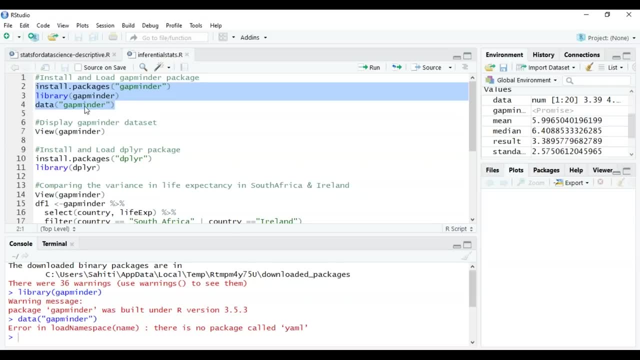 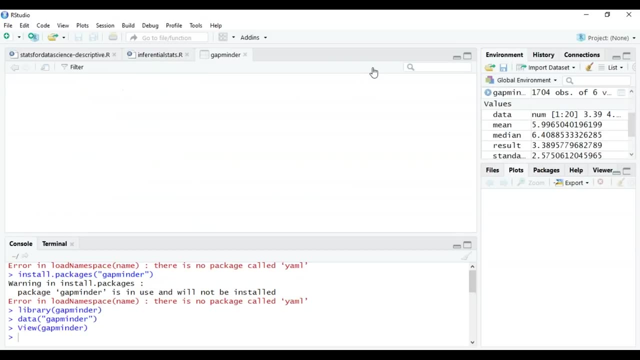 the gap minder data set. so this installpackages will basically install the gap minder package and this library. gap minder will just load the gap minder library. all right, so we've successfully loaded our gap minder package. now let's view this data set. 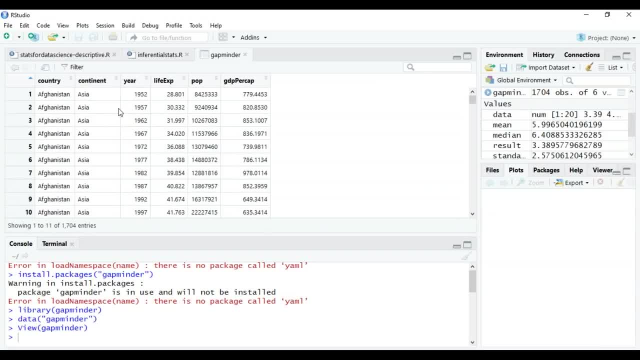 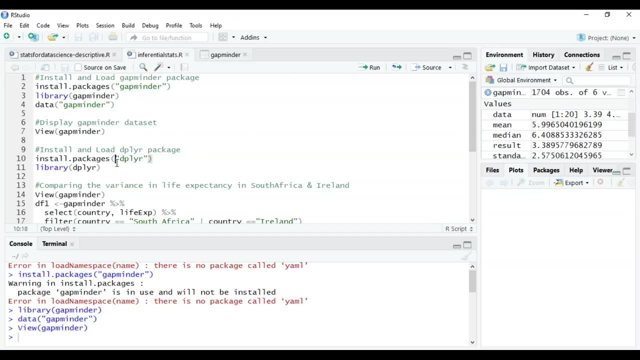 these are the countries. all right, different countries, and you have the continents, the year, the life expectancy, the population and the gdp per capita. okay, so, each of these countries. we have this information right now. the next step is to load the famous deployer package provided by. 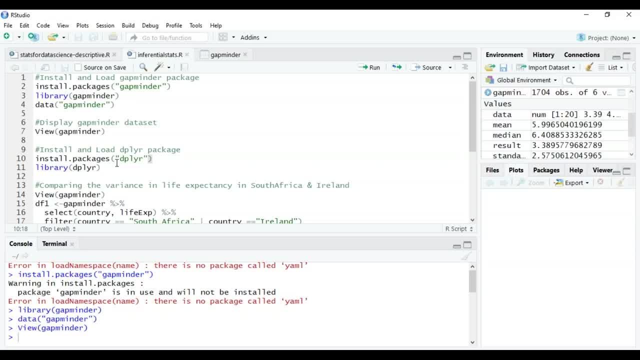 our. we're specifically looking to use the pipe operator in this package. okay, now for those of you who don't know what the pipe operator does, this is a pipe operator. right now. the pipe operator, uh, allows you to pipe your data from the left hand side into. 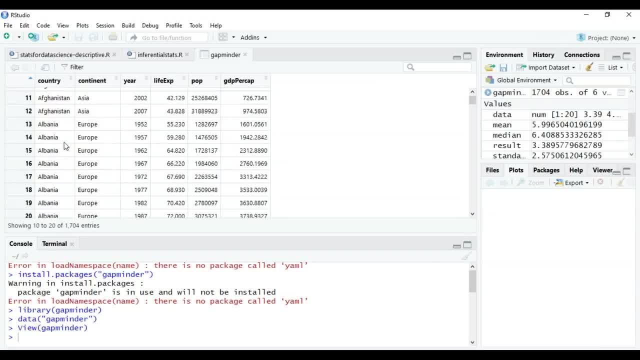 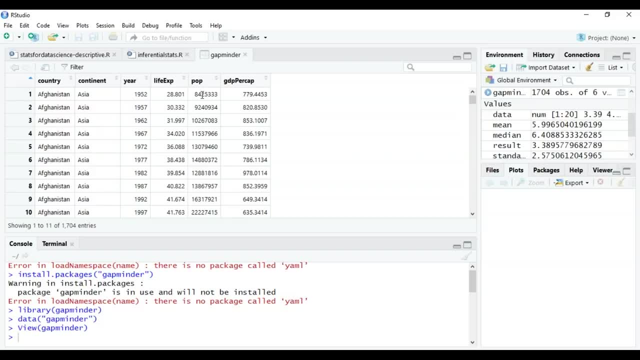 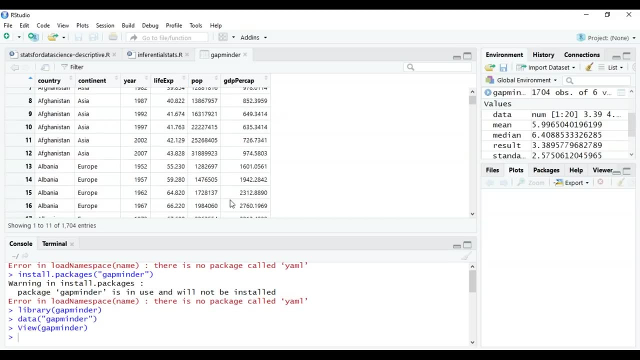 Now let's view this dataset. These are the countries, all right, different countries, and you have the continents, the year, the life expectancy, the population and the GDP per capita. Okay, so each of these countries. we have this information, right. 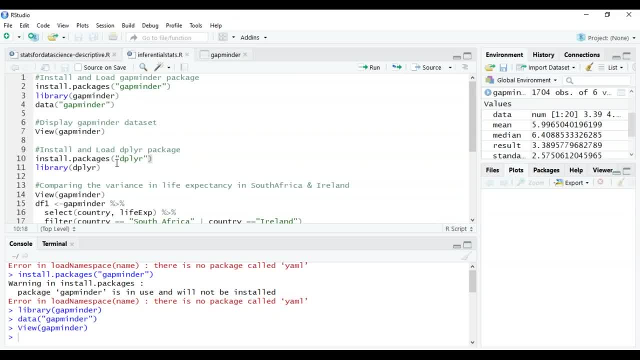 And the next step is to load the famous deployer package provided by R. We're specifically looking to use the pipe operator in this package. okay, Now for those of you who don't know what the pipe operator does, this is a pipe operator, right. 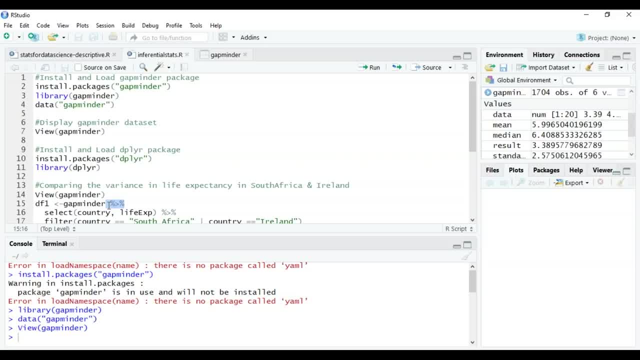 Now the pipe operator allows you to pipe your data from the left-hand side into the data at the right-hand side of the pipe. Okay, it's quite self-explanatory: It's a pipe which connects two data points, right? So let's install and load this package. 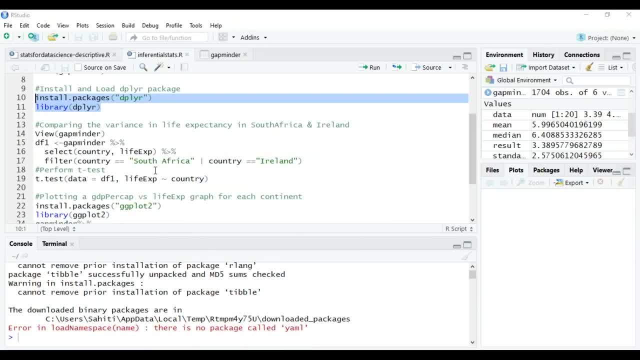 All right, now our next step. what we're gonna do is we're going to compare the life expectancy of two places. Okay, we're gonna compare the life expectancy of Ireland and South Africa and we're gonna perform the t-test to check. 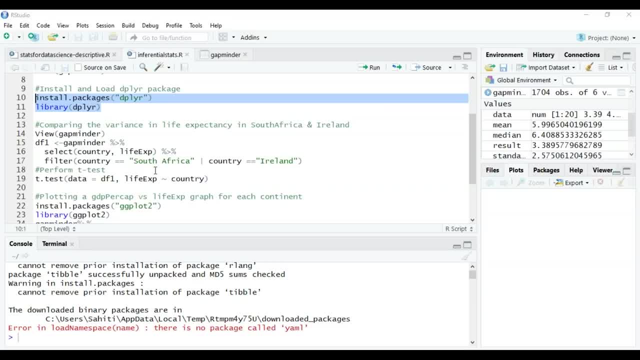 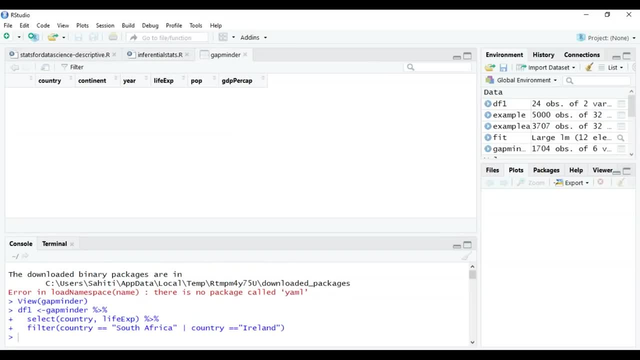 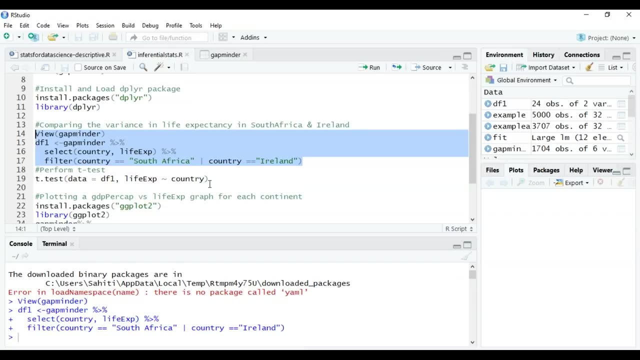 if the comparison follows a null hypothesis or an alternate hypothesis. okay, So let's run the code. Okay, so now we'll apply the t-test and we'll compare the life expectancy of these two places. All right, let's run this. 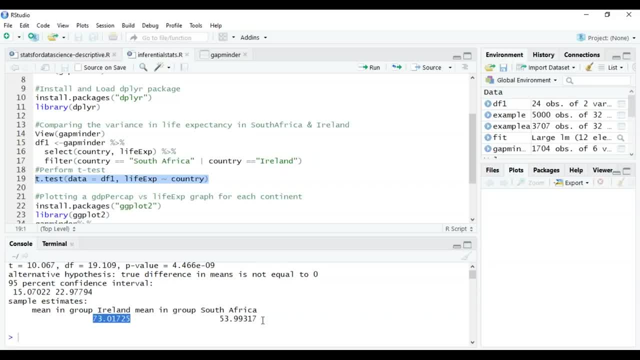 Notice the mean in group Ireland and South Africa. right Here is the mean. You can see that the life expectancy almost differs by a scale of 20.. Now we need to check if this difference in the value of life expectancy in South Africa and Ireland. 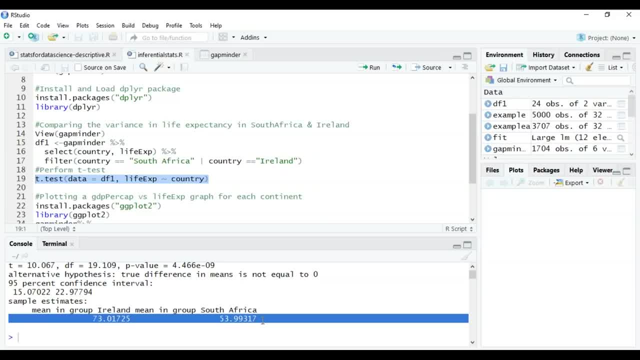 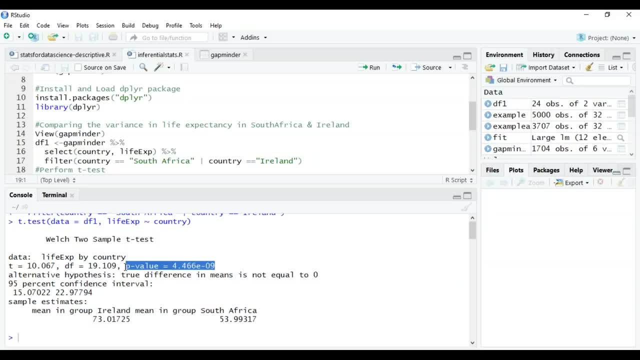 is actually valid and not just by pure chance. okay, For this reason, the t-test is carried out. So pay special attention to this p-value over here. This is also known as the probability value right. The p-value is very important measurement. 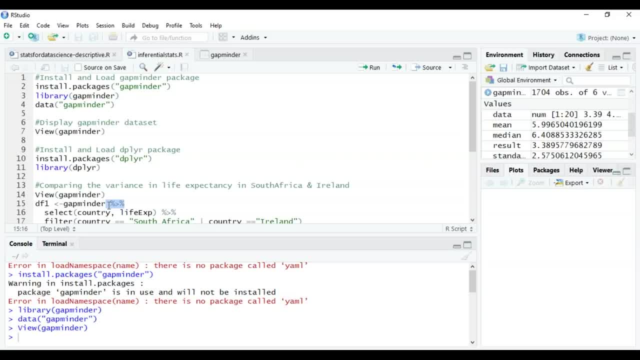 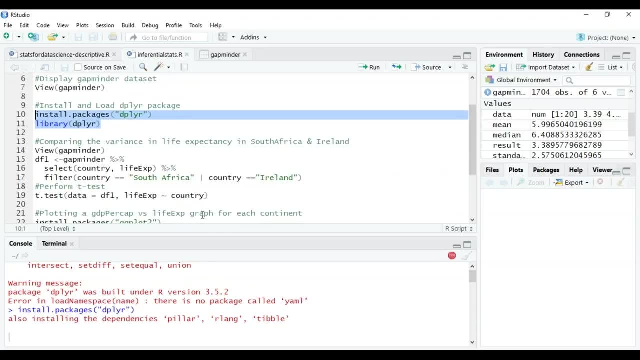 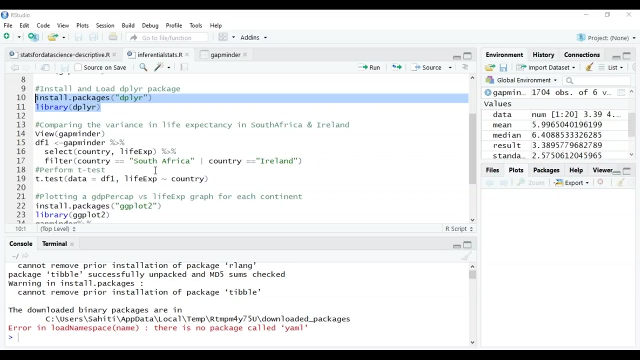 the data at the right hand side of the pipe. okay, it's quite self-explanatory: it's a pipe which connects two data points. right? so let's install and load this package all right. now. our next step. what we're going to do, is we're going to compare the life expectancy. 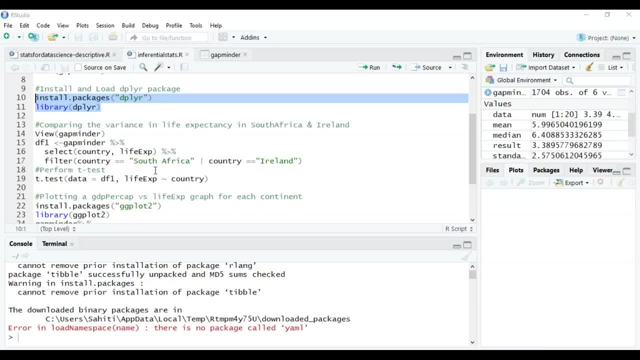 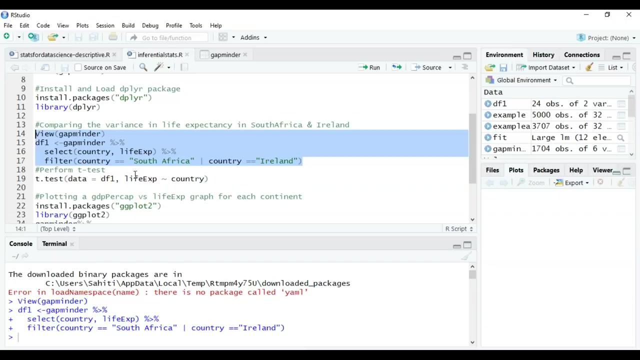 of two places. okay, we're going to compare the life expectancy of ireland and south africa and we're going to perform the t test to check if the comparison follows a null hypothesis or an alternate hypothesis. okay, so let's run the code. okay, so now we'll apply the t test and we'll compare the life expectancy of these two places. 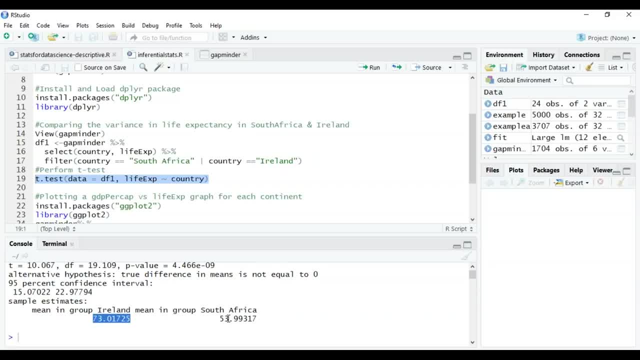 all right, let's run this: notice: the mean in group ireland and south africa. right here is the mean. you can see that the life expectancy almost differs by a scale of 20.. now we need to check if this difference in the value of life expectancy in south africa and ireland is actually valid. 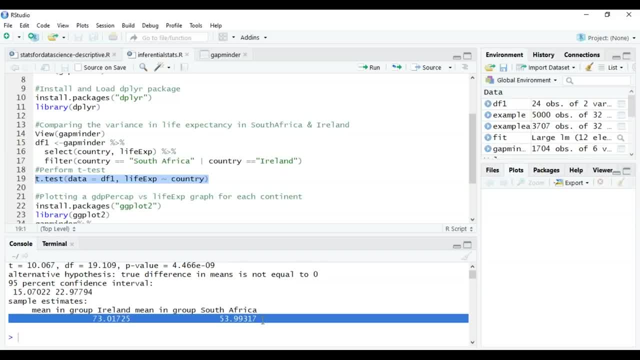 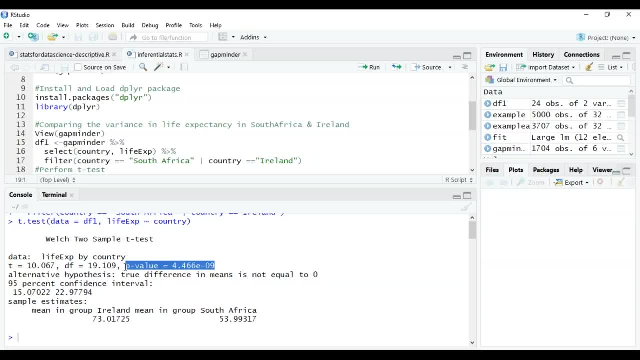 and not just by pure chance. okay, for this reason the d test is carried out. so pay special attention to this p value over here. this is also known as the probability value right, very important measurement when it comes to ensuring the significance of a model. a model is said to be statistically significant only when the p value is less than the predetermined. 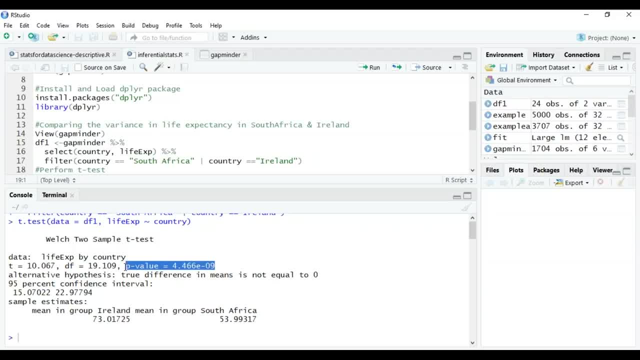 statistical significance level, which is ideally 0.05, right? so your p value has to be much lesser than 0.05. as you can see from our output, the p value is very, very lesser when compared to 0.05, right? it is an extremely small value, which is a good thing. now, in the summary of the 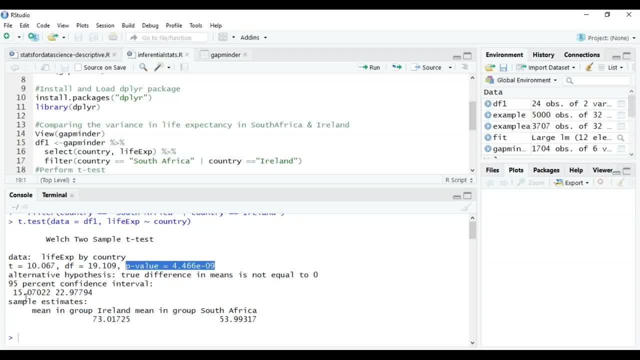 model. notice another important parameter called the t value. right, i've been talking about the t test, and what exactly is this t value? you can see it over here: it is 10.067 now. a larger t value suggests that the alternate hypothesis is true and that the difference in life expectancy 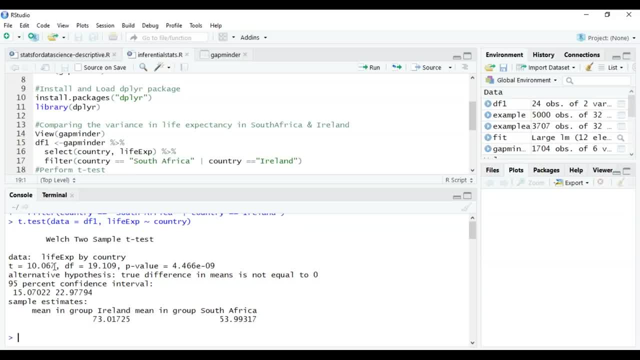 is not equal to zero by pure luck. hence, in our case, the null hypothesis is disapproved. so to prove that the null hypothesis is true, we have to use the null hypothesis to prove that the null hypothesis is true and that the difference in life expectancy is not equal to zero by pure luck. 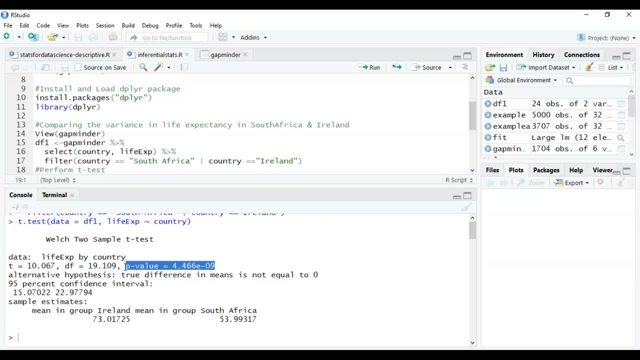 when it comes to ensuring the significance of a model. A model is said to be statistically significant only when the p-value is less than the predetermined statistical significance level, which is ideally 0.05, right, So your p-value has to be much lesser than 0.05.. 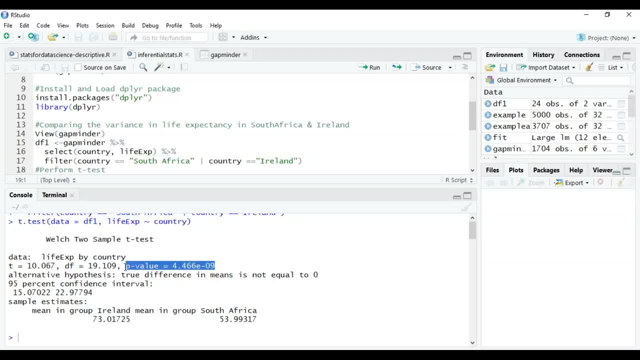 As you can see from our output, the p-value is very, very lesser when compared to 0.05, right, It is an extremely small value, which is a good thing. Now, in the summary of the model, notice another important parameter called the t-value, right. 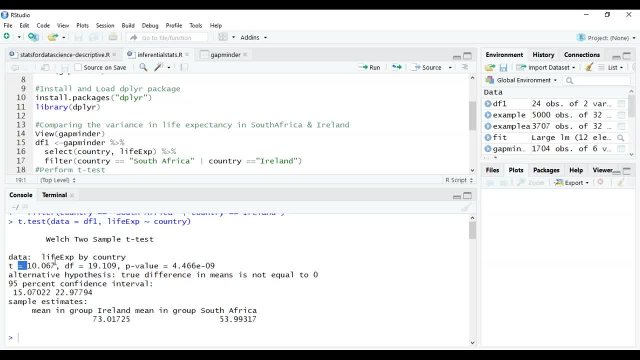 I've been talking about the t-test. and what exactly is this t-value? You can see it over here: It is 10.067.. Now, a larger t-value suggests that the alternate hypothesis is true and that the difference in life expectancy is not equal to zero by pure luck. 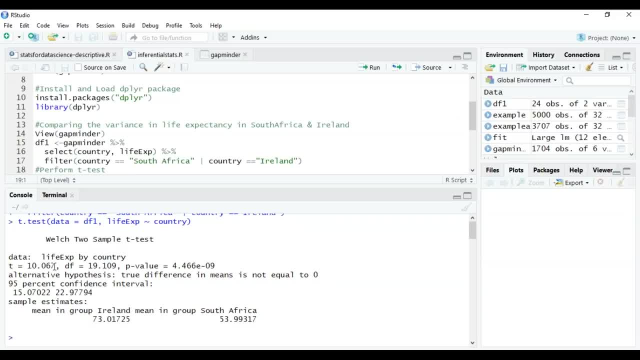 Hence, in our case, the null hypothesis is disapproved. So to conclude the demo, we'll be plotting a graph for each continent, such that the graph shows how the life expectancy for each continent varies with the respective GDP per capita. Just to add a little bit data visualization. 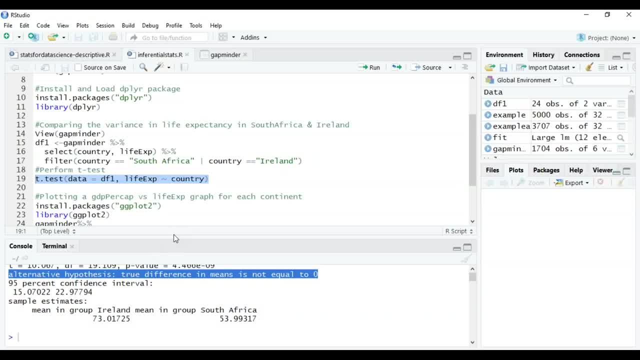 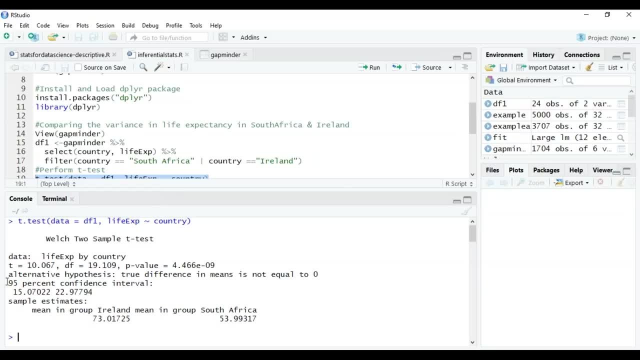 I am performing this last step. So, guys here, we can clearly see from the output that the alternate hypothesis is true. all right. So this is calculated with a 95% confidence interval, right? You get what I'm saying when I'm talking about. 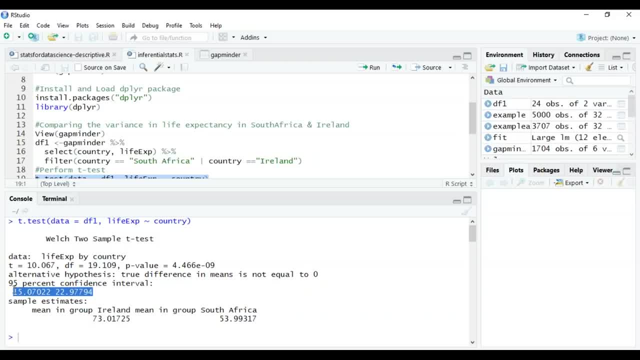 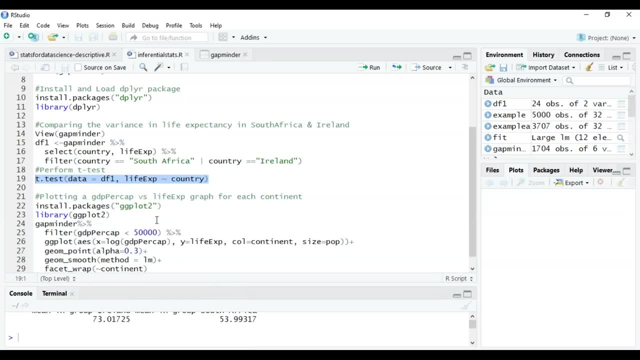 a 95% confidence interval. right? This is our confidence interval: 15 to 22,- and our confidence level is 95%. This is exactly what we discussed a couple of minutes ago. Now, just to end the demo, I'll show you a small visualization. 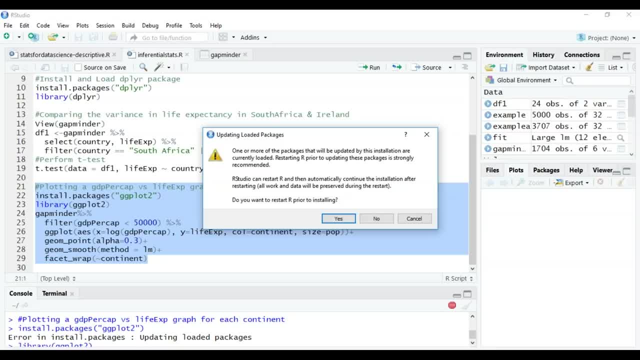 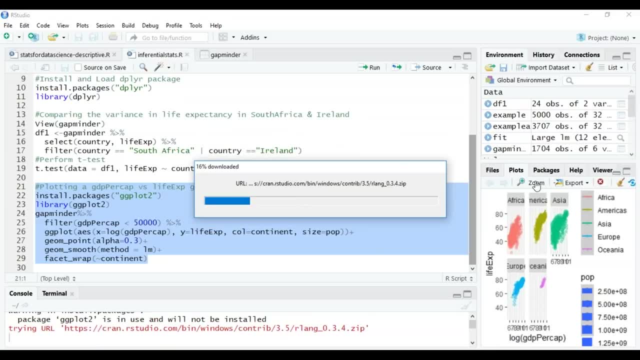 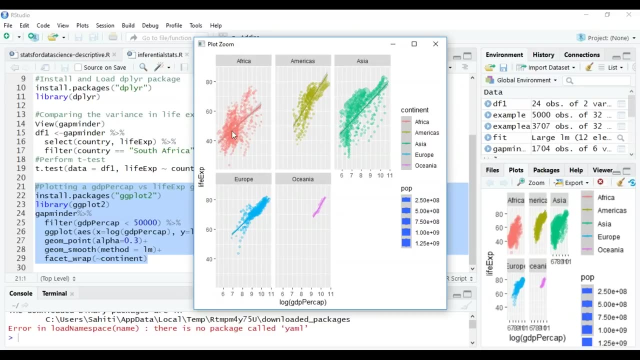 Here. what we're doing is we're showing how the life expectancy for each continent varies with respect to the GDP per capita For that continent. okay, so this is our plot. Okay, if you look at the illustration, you can almost see a linear variance, right? 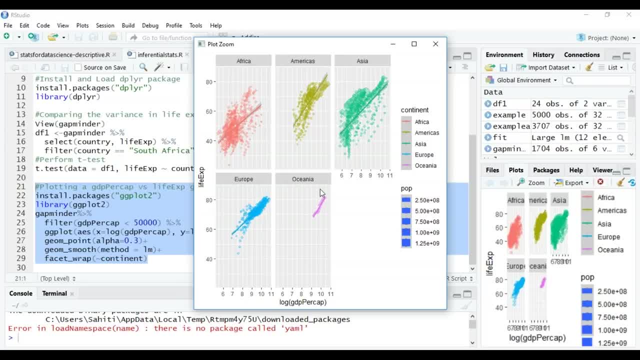 You can almost see a linear line in the life expectancy for each of the continent with respect to the GDP per capita. Now this also shows how well the R language can be used for statistical analysis. right, Look at how pretty the graph looks and also how well they show that. 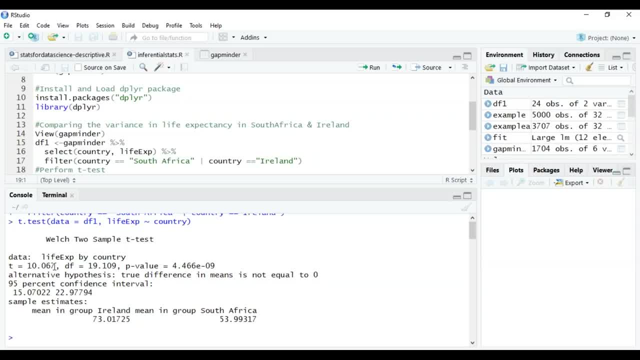 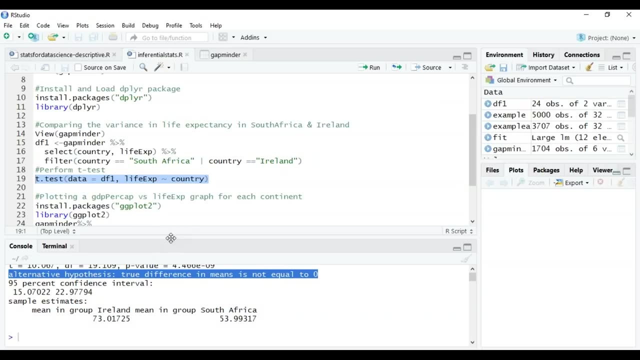 conclude, the demo will be plotting a graph for each continent, such that the graph shows how the life expectancy for each continent varies with the respective gdp per capita, just to add a little bit data visualization. i am performing this last step. so, guys, here we can clearly see from the output. 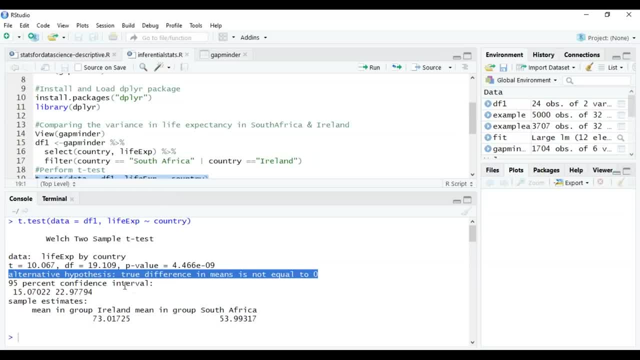 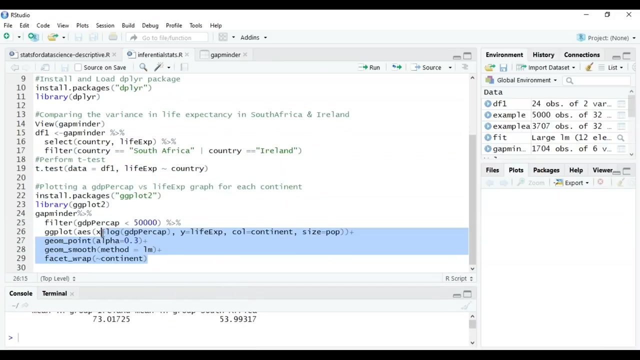 that the alternate hypothesis is true, all right. and also, this is calculated with a 95 confidence interval, right? you get what i'm saying when i'm talking about 95 percent confidence interval, right? this is our confidence interval- 15 to 22- and our confidence level is 95. this is exactly what we discussed a couple of minutes ago. now, just to end the demo, i'll 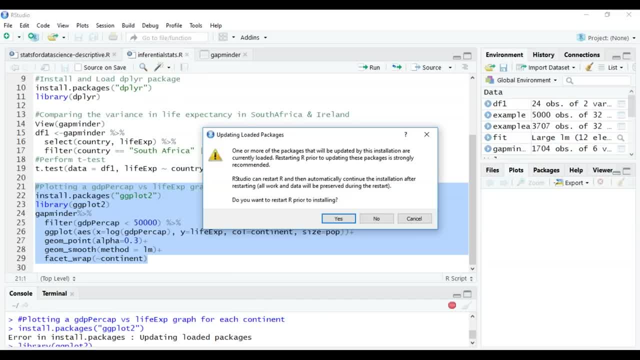 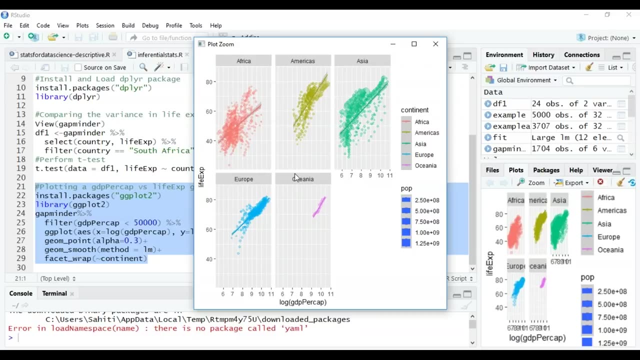 show you a small visualization here. what we're doing is we're showing how the life expectancy for each continent varies with respect to the gdp per capita for that continent. okay, so this is our plot. okay, if you look at the illustration, you can almost see a linear variance. right, you can almost see a linear line in the life. 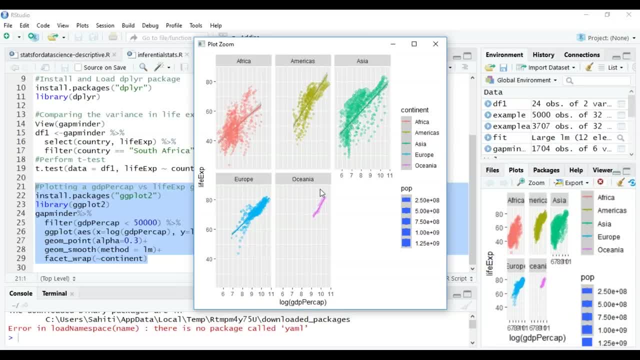 expectancy for each of the continent with respect to the gdp per capita right. this also shows how well the r language can be used for statistical analysis right. look at how pretty the graph looks and also how well they show that there is almost a linear dependency between. 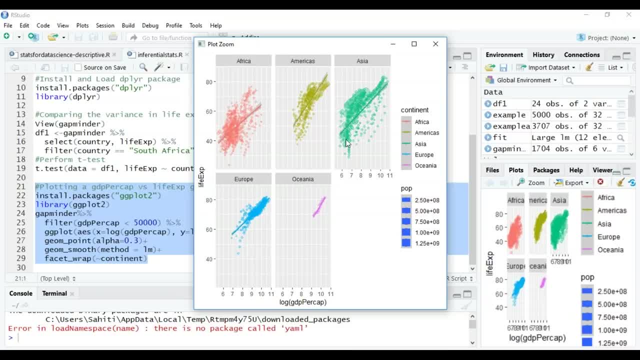 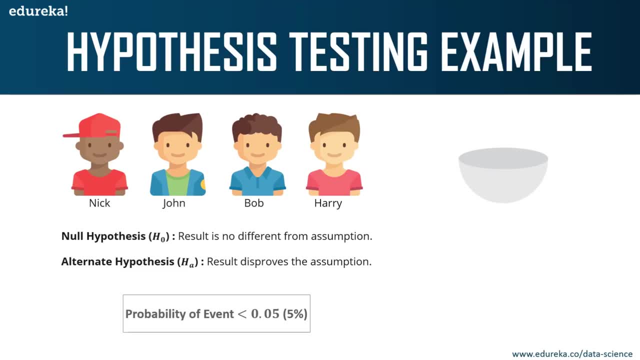 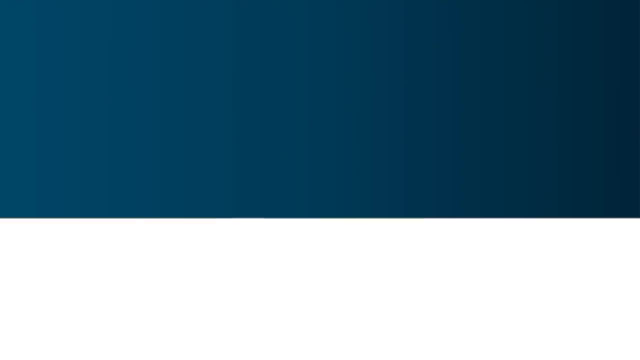 the gdp per capita and the life expectancy. right? so in this demo, i showed you how hypothesis is, testing is done, which is actually one of the most important part of statistical inference. we also saw confidence interval and the confidence level in the same example, right? so, guys, if you 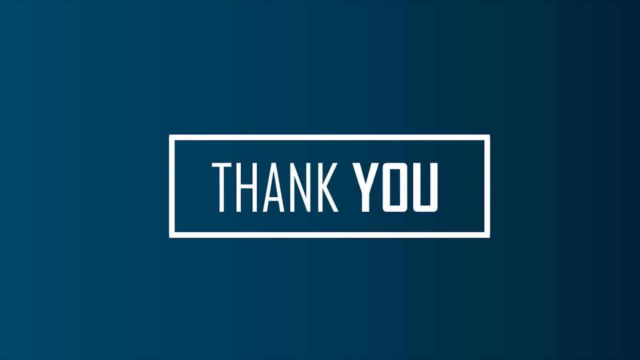 have any questions regarding the session? please leave your questions in the comment section. i'll try and answer all of your questions. so, guys, thank you so much for watching this video. have a great day. i hope you have enjoyed listening to this video. please be kind enough to like it and you. 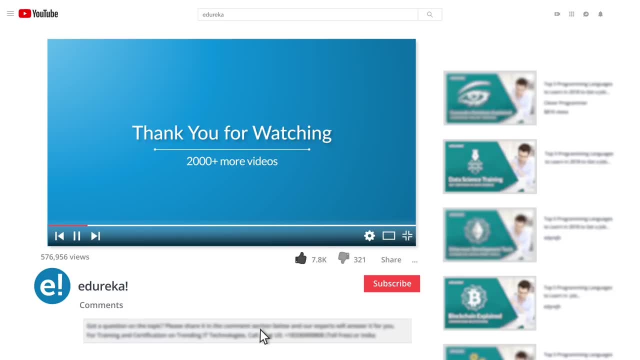 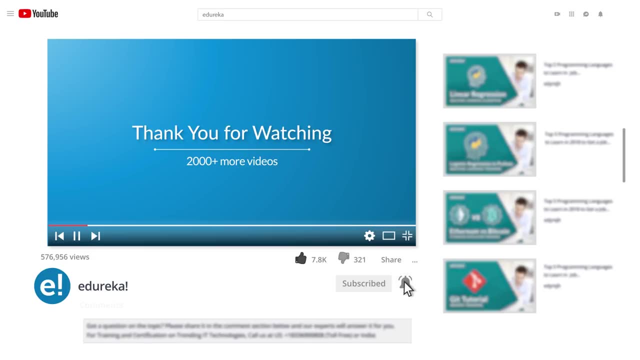 comment any of your doubts and queries and we will reply them at the earliest. do look out for more videos in our playlist and subscribe to edureka channel to learn more happy learning.